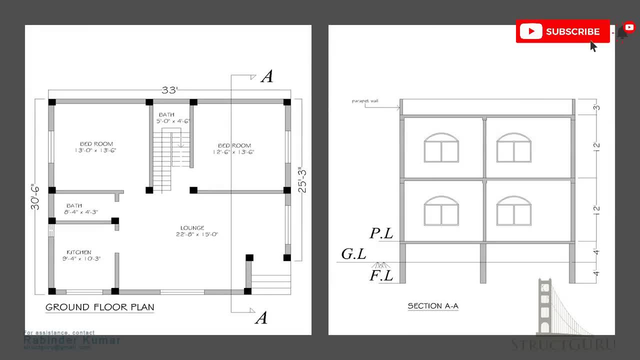 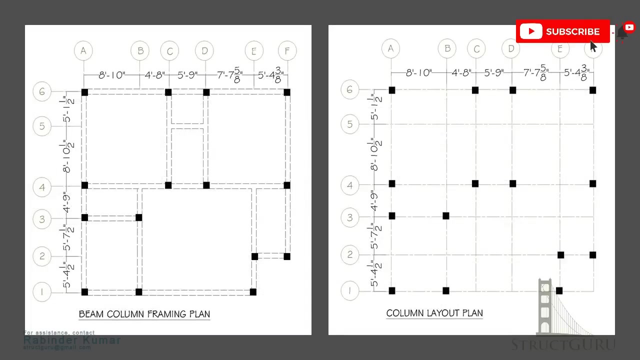 The structure we are going to model is a residential building. It consists of ground plus one storey building. You can see various plans on the screens. The architectural plan and section elevation is given to you from architect Or, if you are good in planning, you can also draw it by yourself. And the beam column layout is designed by a structural engineer. 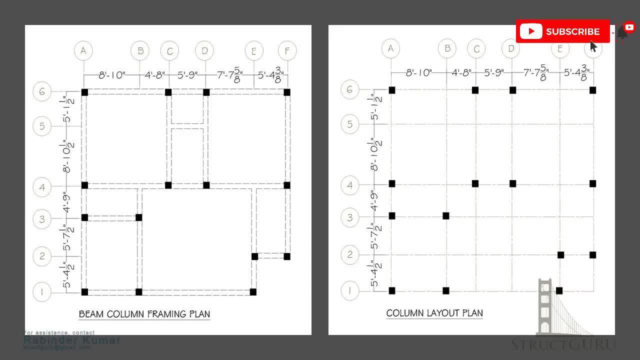 Now the question is: how do you design a building, How to decide the positions, orientations and sizes of columns and beams? So I will discuss this in my next video in detail. Today we will focus to the basic: modeling and defining the structural elements. So let's begin. 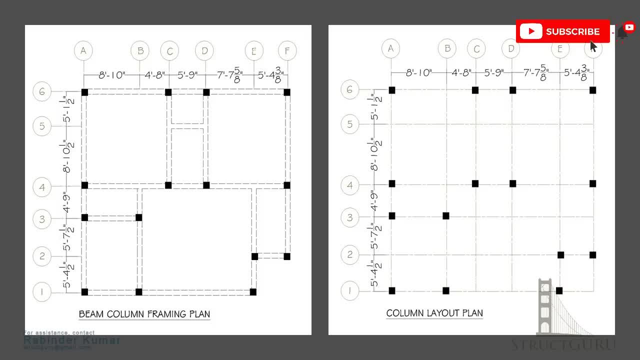 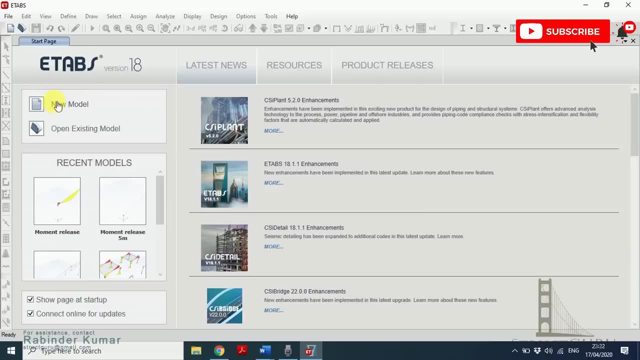 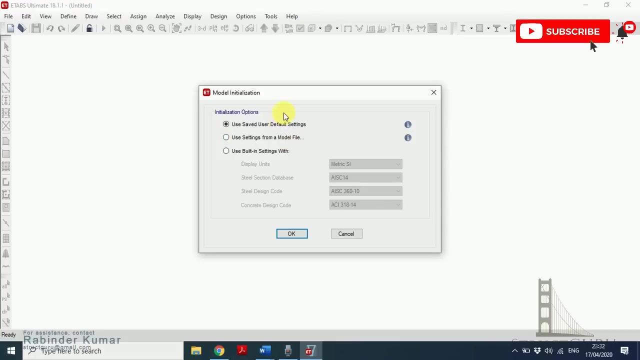 Open your E-Tabs application. So to create a new model, click new model Or you can also create a new model. You can also create a new model by clicking on the file menu and select the new model. A window will pop up. If you want to go with default settings, then click the first option. 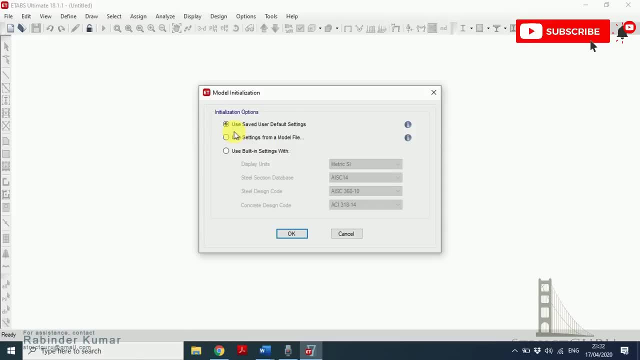 If your country requirement is to work with different set of units, then go to use built-in settings, So from there you can choose the different set of units And also you can choose the code codes. for our case, I am going to use ACI 318 2014 for concrete design code for 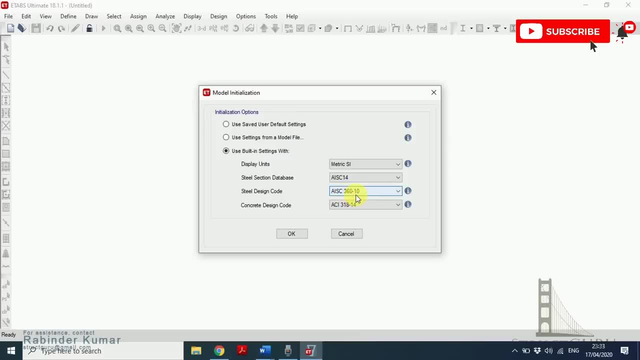 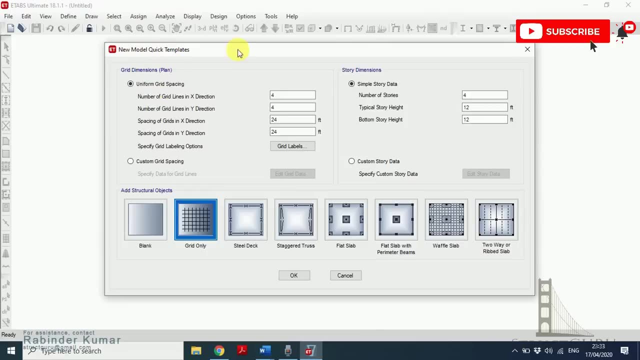 steel design code. I will be stick to AISC 360. to click OK bring you to the new model and quick templates. I will discuss this panel in detail as it is very important to model a structure. so first understand why we have to define the grids and story data at the start. so grid lines are reference central lines. 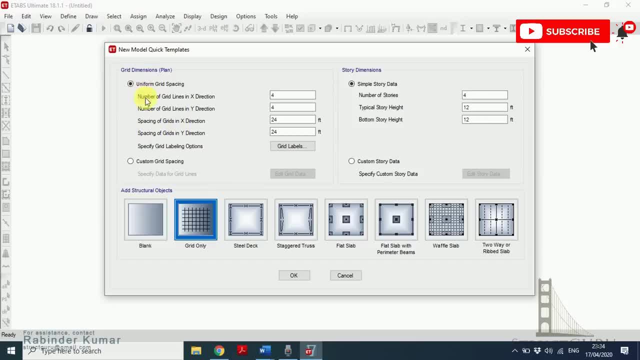 of your structure. so grid dimensions are categorized into two panels: a uniform grid spacing and custom grid spacing. the uniform grid spacing is used when the size of grid is same in X and Y direction. most of the time our center line spacing is not constant along X and Y direction, then we go with. 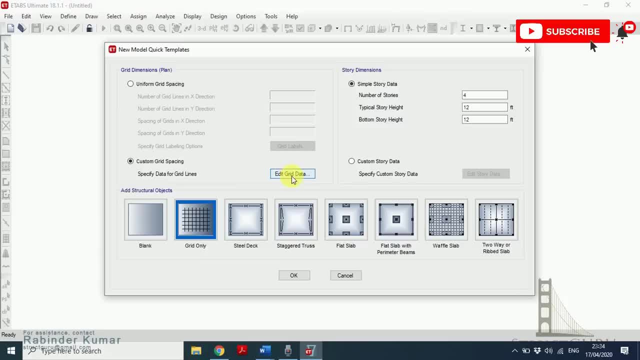 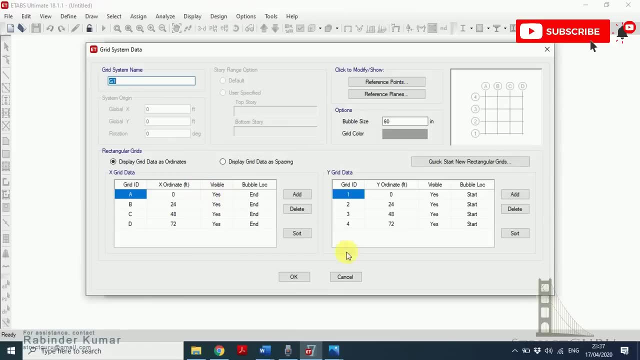 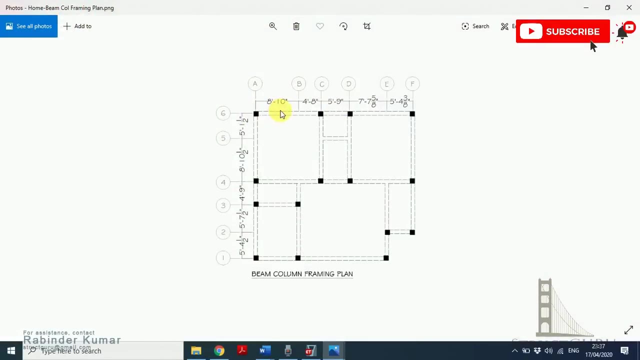 custom grid spacing. so click custom grid spacing and click on edit grid data. before entering the value of grid spacing, let's have a view to our beam column layout or grid layout plan. so this is the beam column layout. the position of column is marked here. so along X axis there are six grids and along Y axis 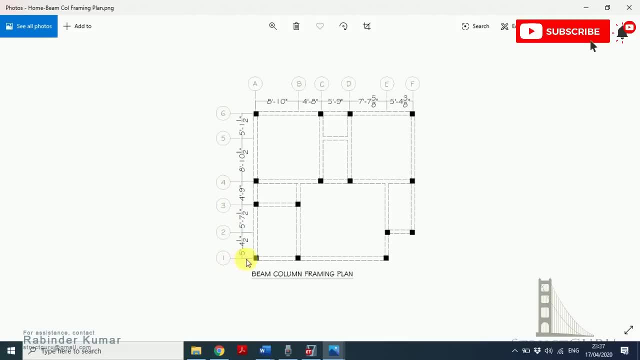 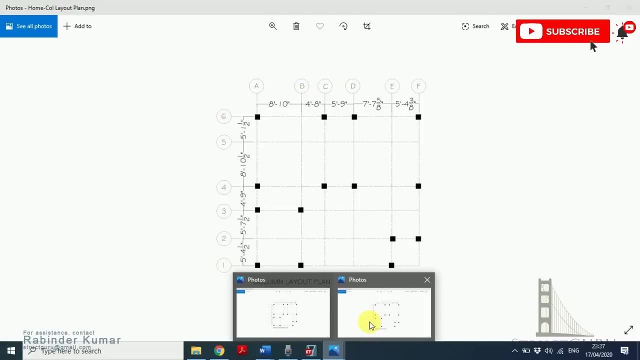 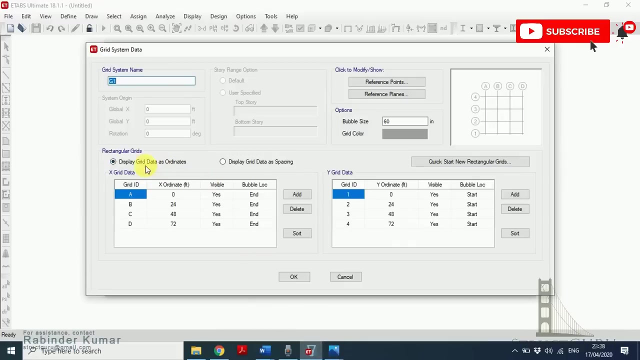 there are also six grids. the dimension between each grid is mentioned here, so I have. so I have divided this into a grid layout plan so it will be easy to mark all the dimension in our ETABS model. so let's begin in your ETABS model, you can. 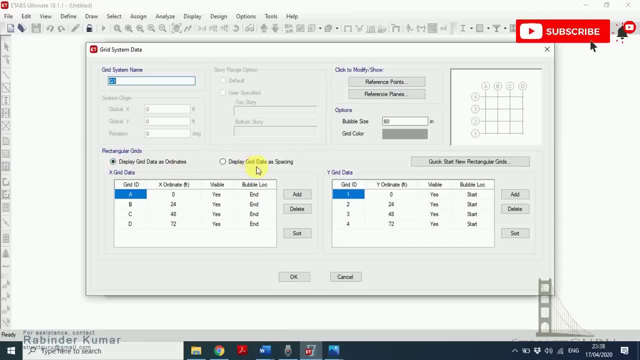 see display grid data as ordinance or display grid data as spacing. so what is difference between them? so if you choose this option as ordinance, that means all this. whatever the value you choose between the crates, you have to always follow from your origin. for example, if the distance between grid 1 and 2 is 2. 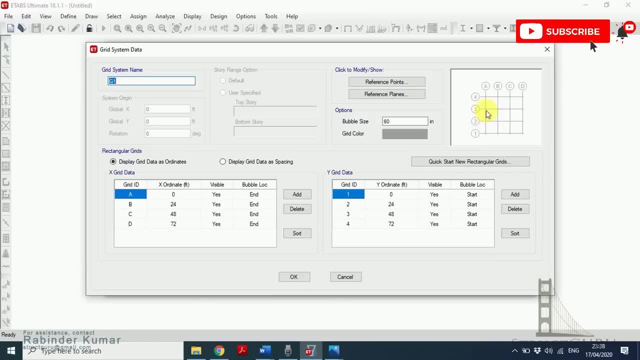 and the distance between grid 2 and 3 is 2. so if you choose this option, so for 1 and 2 you will put 2 and for 2 and 3 you will put 4. but if you choose this option- display grid data as spacing- so in this data you have to put the value between. 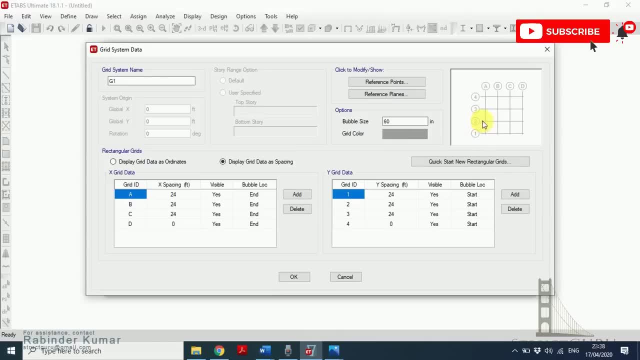 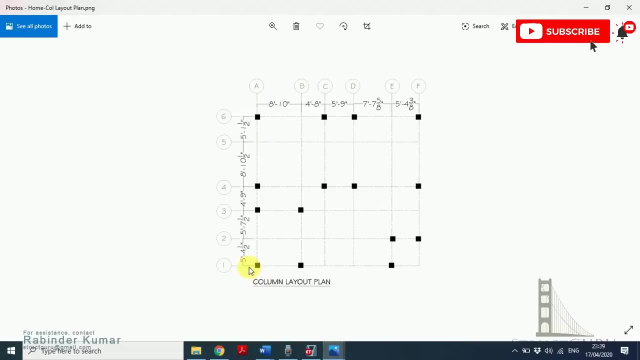 A and B, whatever the value is between 1 and 2, and for 2 and 3, whatever the value of dimension is between 2 and 3. so I will tell you in a moment. so I'm choosing display. grid. data is open, our column layout plan. so, from 1 to: 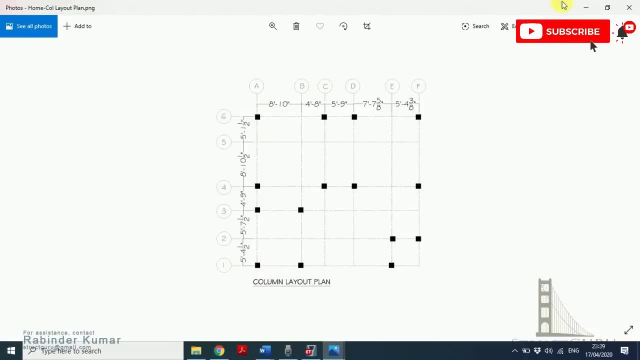 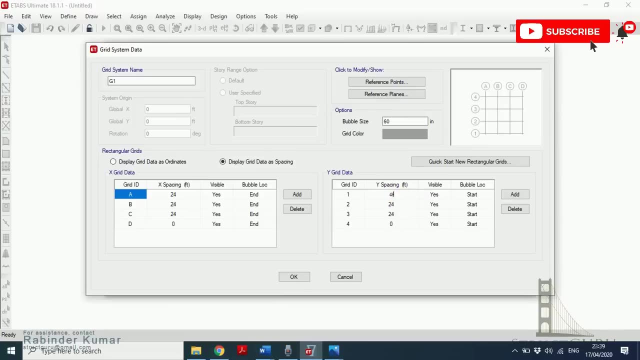 2 is 5 ft 4 and half inch, so let's put this value in ETABS, so one and two full fit and 1.5 inch, or you can use 4 feet, and so ETEPS is smart and it will automatically convert the. 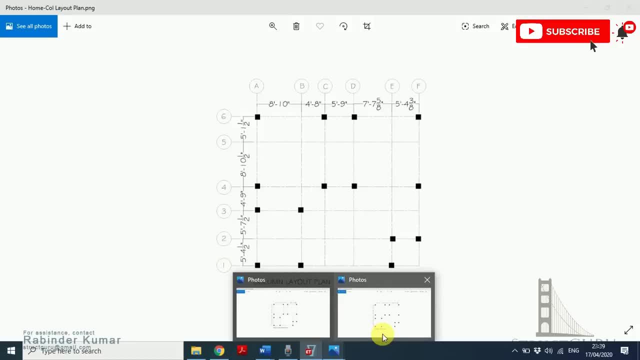 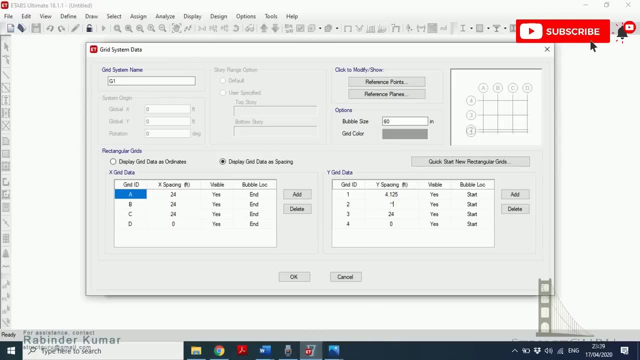 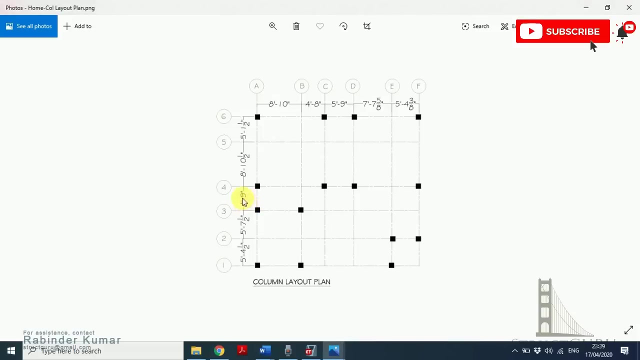 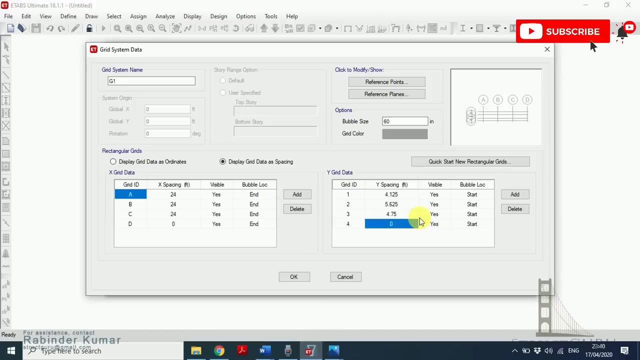 values now begin from 2 to 3. so for 2 to 3 is 5 feet 7.5 inches. go to your ETEPS model. so 5 feet 7.5 inches, again 4 feet and 9 inches. 4 feet 9 inches. you can add or delete the grid data. 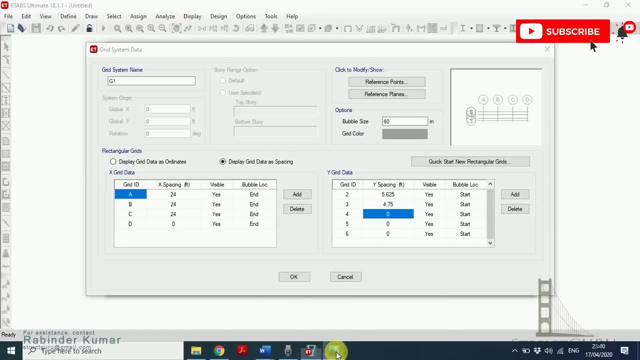 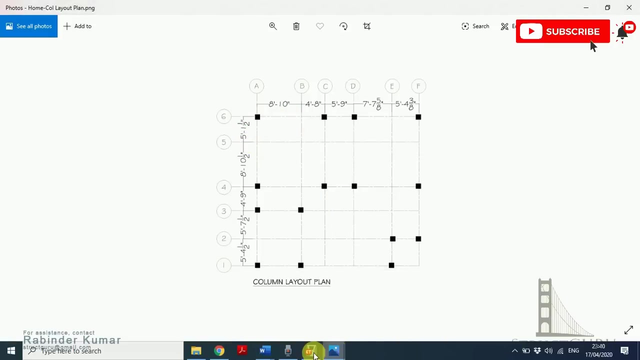 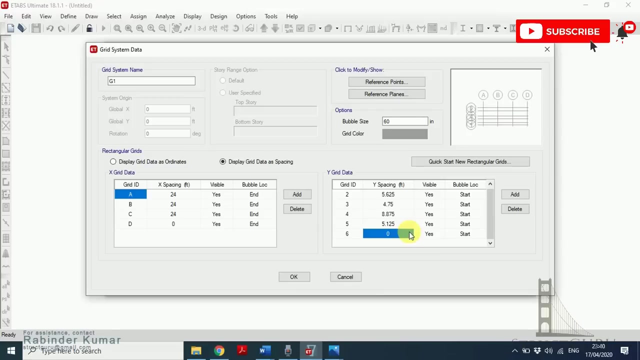 from these buttons: 8 feet and 10.5 inches, 5 feet and 11.5 inch and 5 feet and 5 to 6 to 0. now change the x axis data from a to b. value is 8 feet 10 inches, so 8 feet 10 inches. 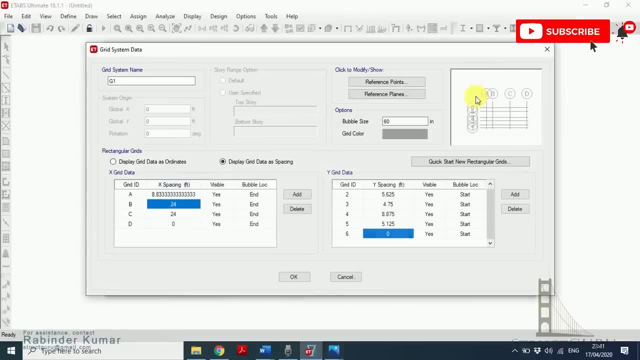 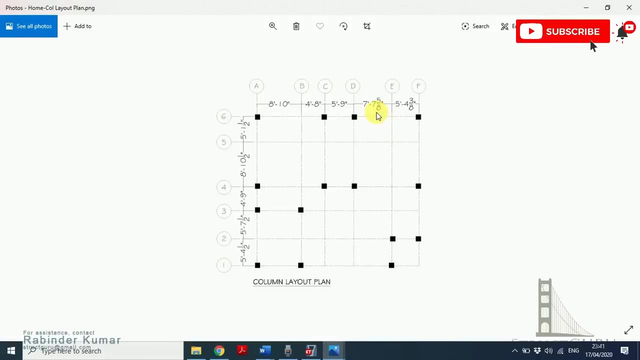 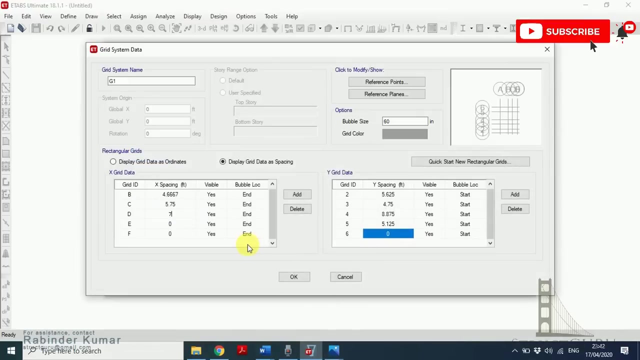 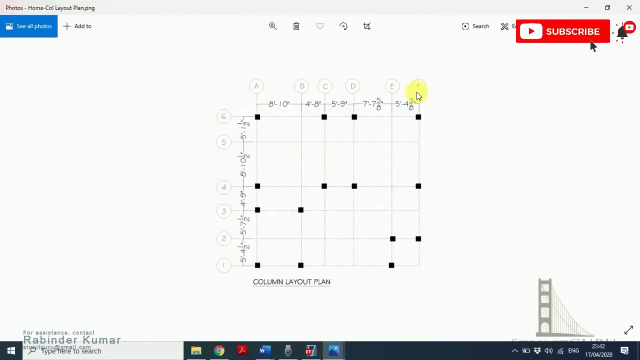 4 feet, 8 inches. 5 feet, 9 inches. 4 feet, 8 inches, 5 feet, 9 inches. 7 feet, 7, 5, 5, 8, 5 feet, 4, 3 by 8, so 7 feet, 7.6 to 5 inches. okay, and three by 3 by 8 is equal to 0.375 inches, so 5 feet. 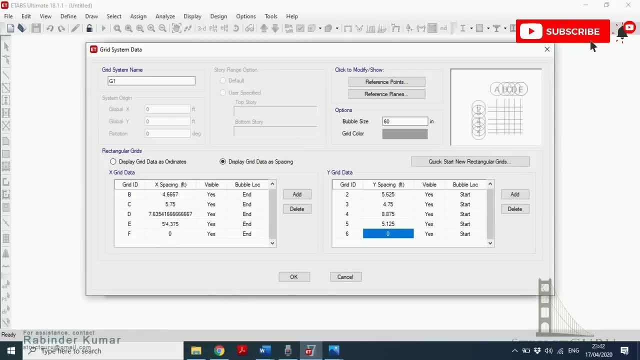 5 feet four point three, seven five inches. okay, so we have added our grid story data. as you can see, the bubbles are overlapping. to reduce the size of bubble, you can insert the different values over here. so 60 inches inch is higher, so start from the 20 inches. so 20 is fine, the no bubbles. 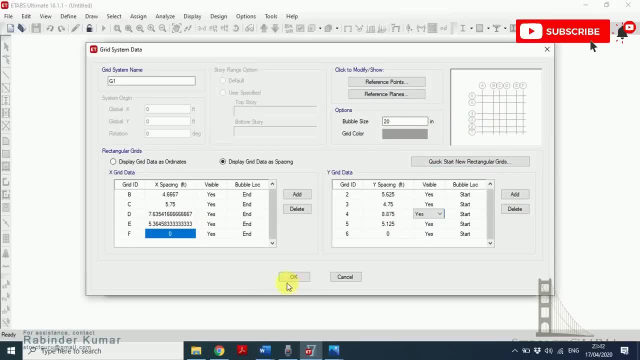 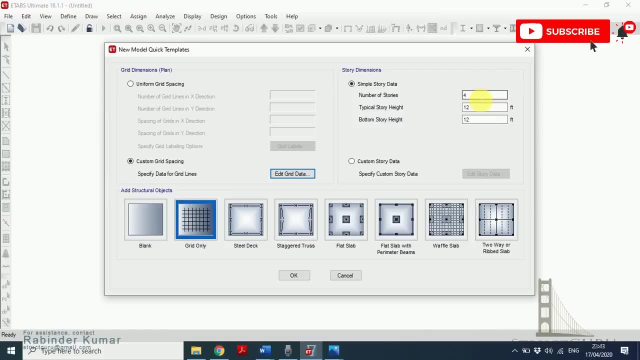 are overlapping, so this grid data is added, so please click ok, now we have to go and change the story data. for story data in etabs we have to provide the story data from the foundation level, so, for example, from foundation to plinth level, we have got a certain value. from plinth to first floor level and from the first to roof level. so it will be a three level, three story building. so from foundation, foundation is generally kept at one and one and a half meter below the ground level. so i'm considering, let's suppose, four feet or five feet below the ground. 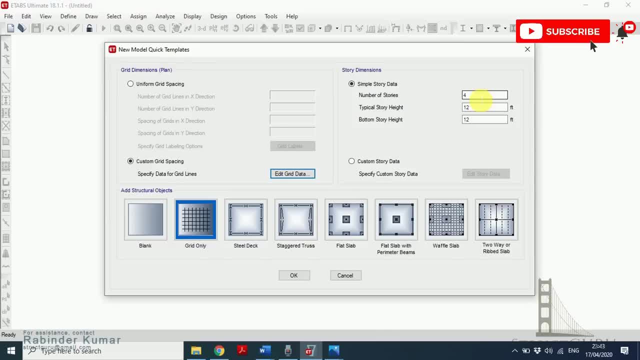 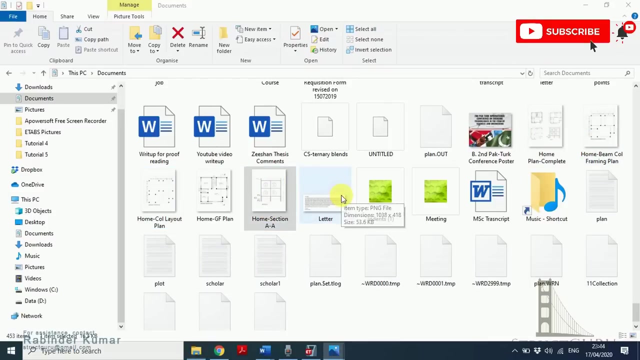 level three feet. our plinth level is three feet or three and a half feet above the ground level and our first floor level is 12 feet and the second floor level is 12 foot. so this all data will be given from sectional plan, which is given to us from an architect. so let me open. 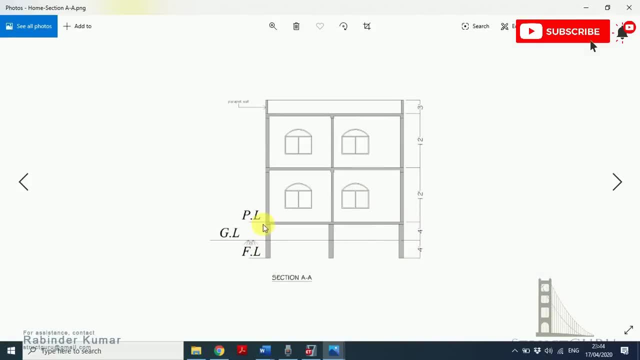 and sectional plan. so, as you can see, from foundation level to plinth level it is eight feet. from plinth level to first floor level, which is 12 feet. from first floor level to roof level, again 12 feet. so we have got three stories: first story, second story and the third story. 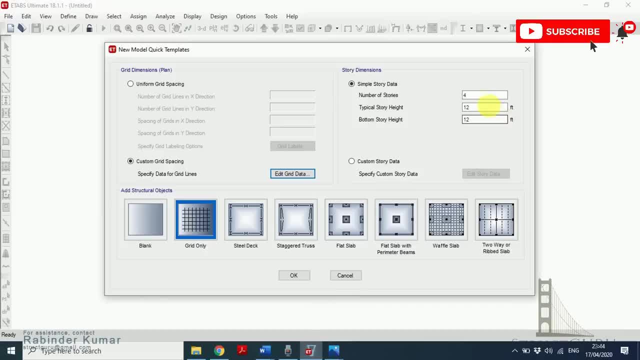 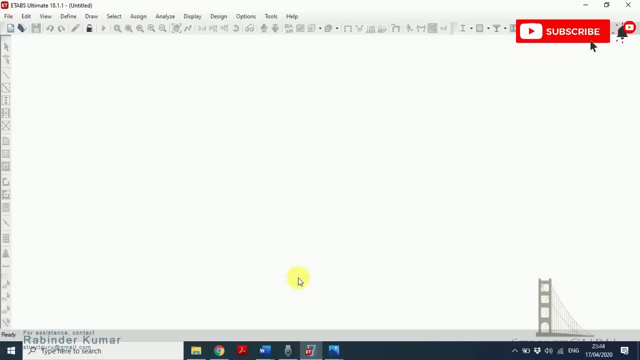 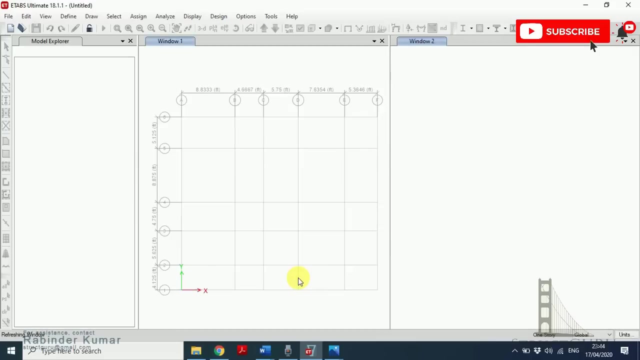 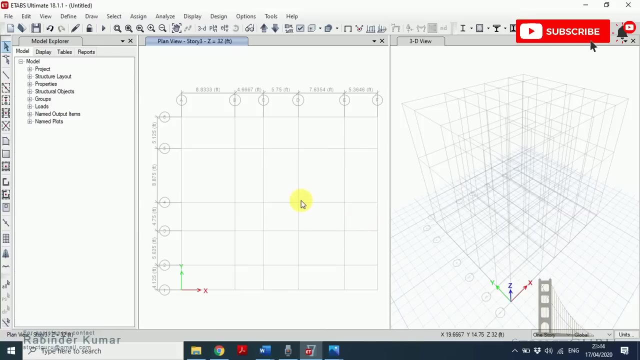 story and third story. so let's put this data into the ETIPS model. so we've got three-story building. typical story height is 12 feet and the bottom story height is 8 feet. so we have done with all the data, click OK and, as you can see, the gridline layout is being generated. so, first and foremost, 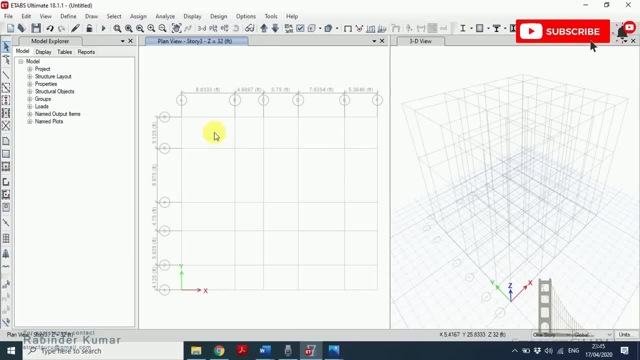 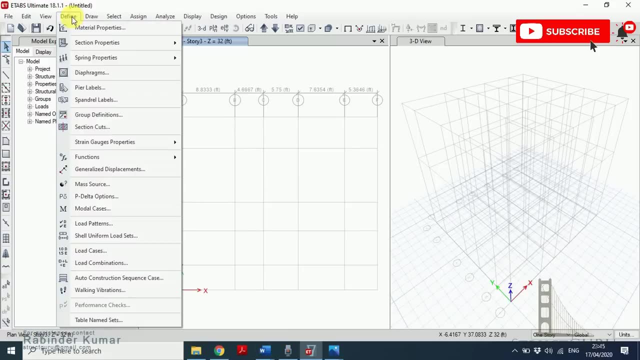 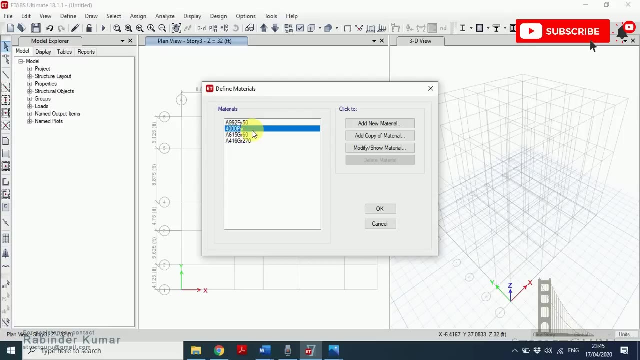 option is: we have to define the material properties. so this is it. we are going to design a concrete structure, so we have to define the concrete material property. so go to the define menu- material property properties. so ETIPS by default has defined different material properties for 60 grade steel, for 50 grade steel, F5 yield strength 4000 psi, which is the 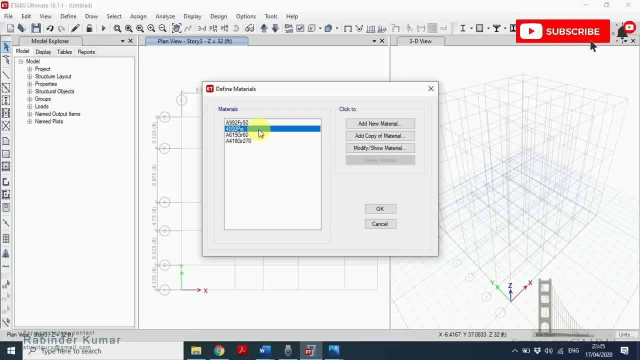 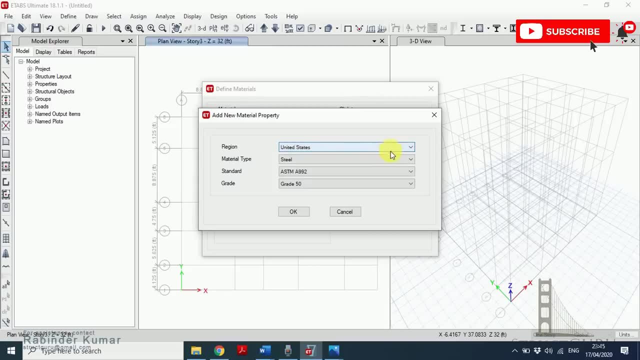 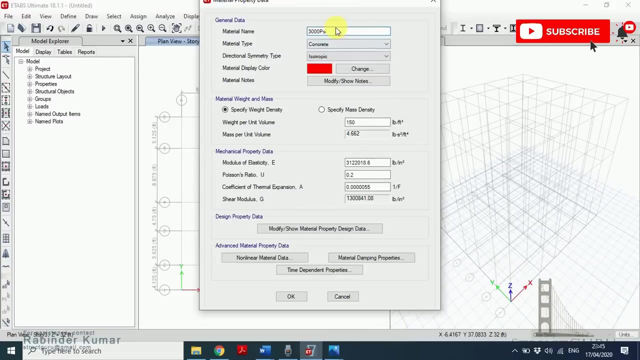 compressive strength of concrete at 28 days. so you can modify these options. if you want to add new material, you just click to add new material. okay, region- whatever the region you want to select, click concrete. if you want to change this data, click 3000. okay, so this is 3000 psi concrete isotropic. the density. 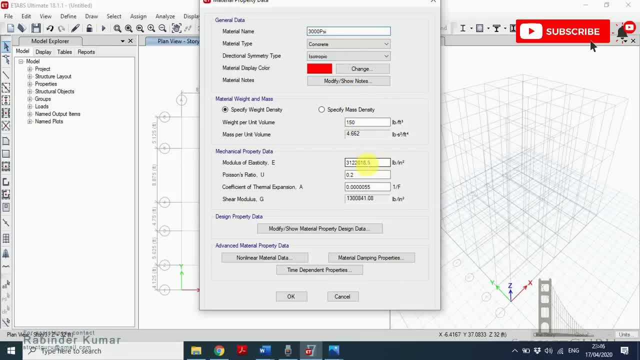 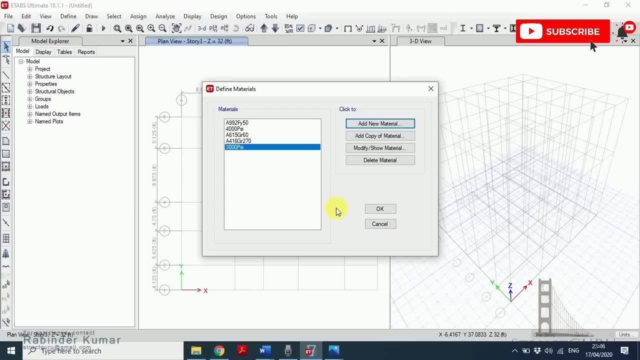 of concrete is 150. the default ETIPS calculated the models of elasticity. we don't have to worry about that. click OK if you want to eight different materials, because in general practice we assign different types of concrete amount structure. for example, for column we use 4000 psi. sometimes for slabs we use 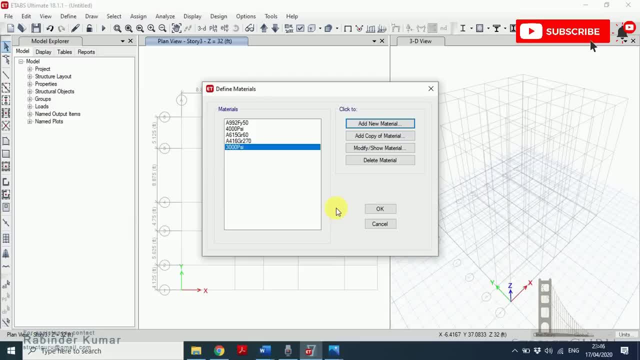 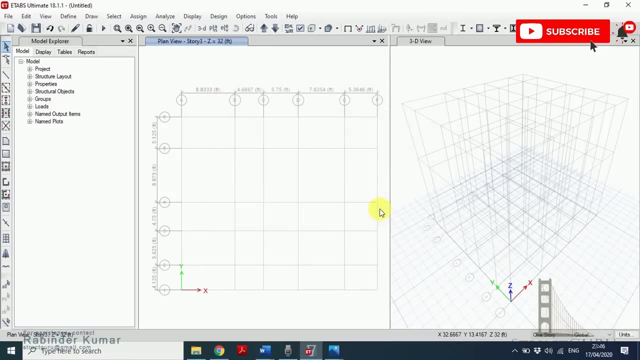 3000 psi. for beams we use 4000 psi. so in this way you can define different types of materials or the different properties of same materials and this model. so click OK o. after defining the material properties, we have to define the section properties. sections means works, how sections we are going to use in our structure. so there 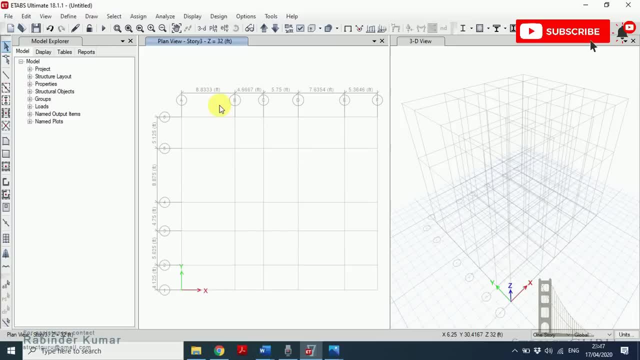 can be beam sections and column sections. so column sections can be rectangular, circular, square. but mostly these all information is given from structural engineers. you have to decide it by yourself What type of column is suitable inickers, and this particular calculation points the material to reach high level. this can also be used to track if this material- as you just knew that the material- will sit for hours parallel to higher level or later. 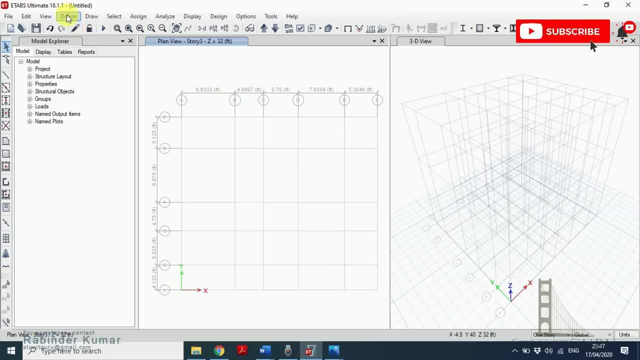 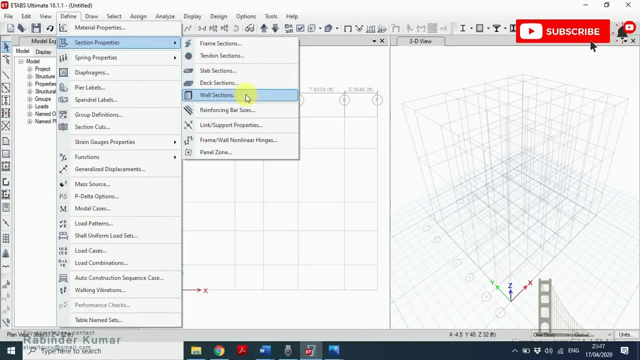 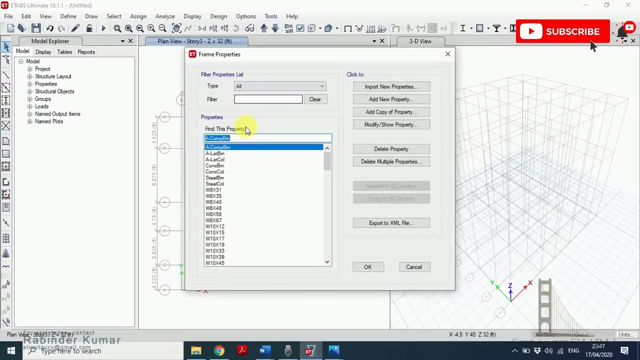 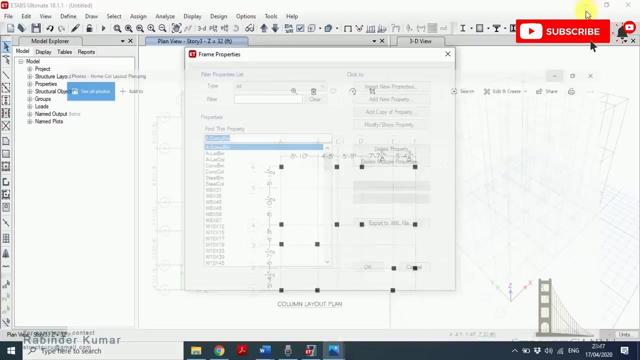 type of column is suitable in this building. so go to the define menu. from section properties you can define frame sections, slab sections, wall sections, reinforcing bar sizes and these other options i will discuss one by one in my future videos. so go to the frame sections options. so in our case columns are rectangular, so the size of column is kept as 12 inches by 12 inches. 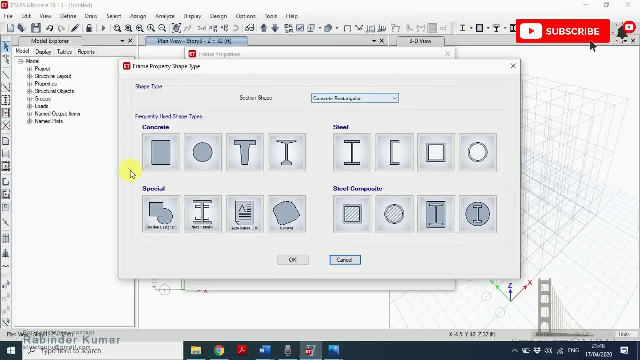 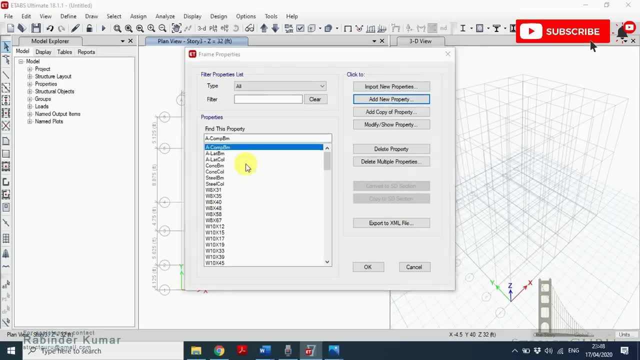 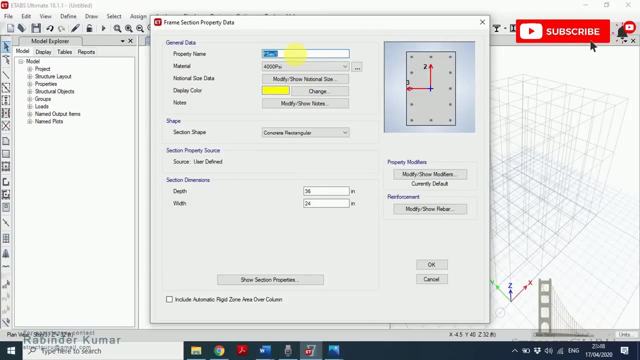 so go to the add new property, click recting complete rectangular section. so our column size is 12 inches by 12 inches. so you can name your column as c dimension is 12 inches by 12 inches and this way we can identify our size of column. so 12 inches by 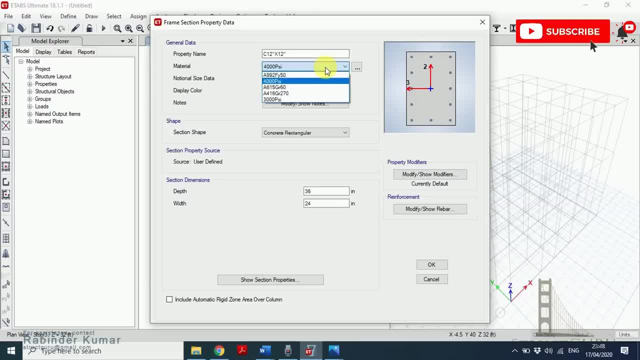 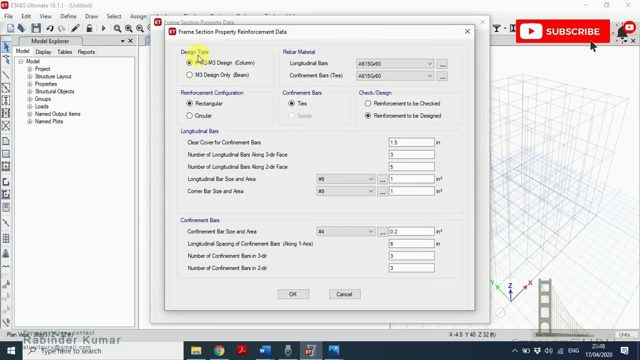 12 inches. i want to keep uh 4000 psi for my column. to change the dimension here: 12 inch. 12 inch. go to the modify show rebar. if you are going to design your define the column, click here column longitudinal bars you can change. 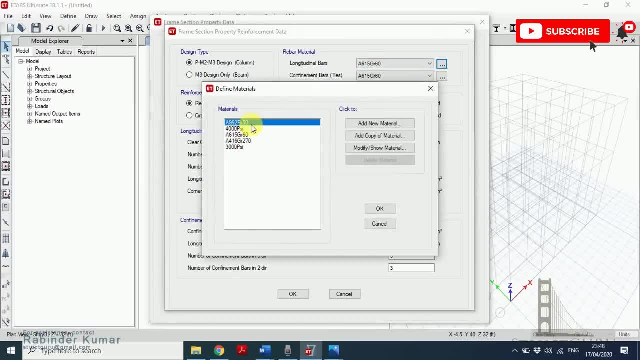 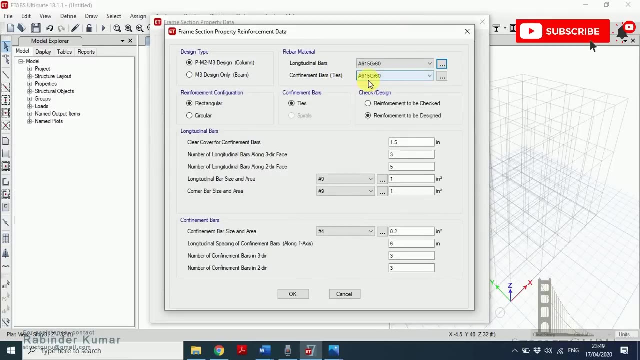 the type of bars from this section. if you want to use 50 yield strength bar, you can click here. if you want to use 16 strand bar, you can click here. so i'm just keeping the default value. and for confinement ties- lateral ties- you might have seen in columns, so i'm also 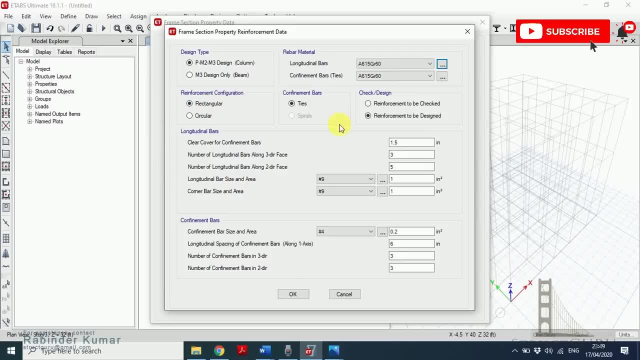 60 graded steel. so our column is rectangular and this option- reinforcement to be checked, reinforcement to be designed- always go for reinforcement to be designed, because reinforcement to be designed: that means e-tabs will tell us the total area of steel needed to resist the load which is assigned on the structure. reinforcement to be checked: that means if you click reinforcement. 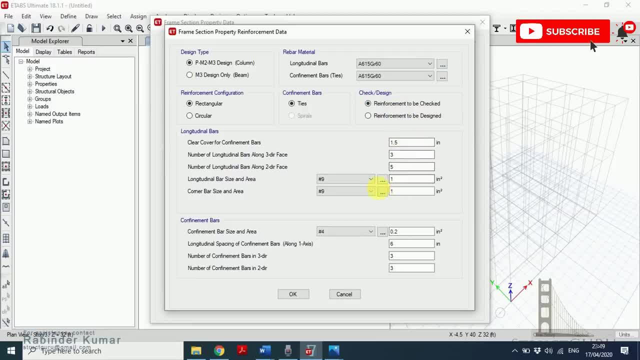 to be checked, you have to provide all these information. you have to provide the bar size, bar number, number in x direction, number in y direction, what spacing you are providing. so in this way, e-tabs will check your given data according to your given data. so always go with. 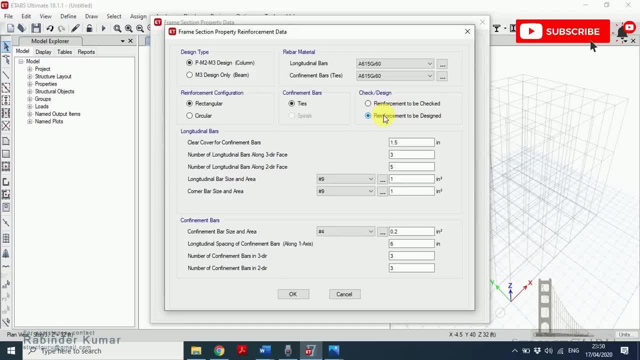 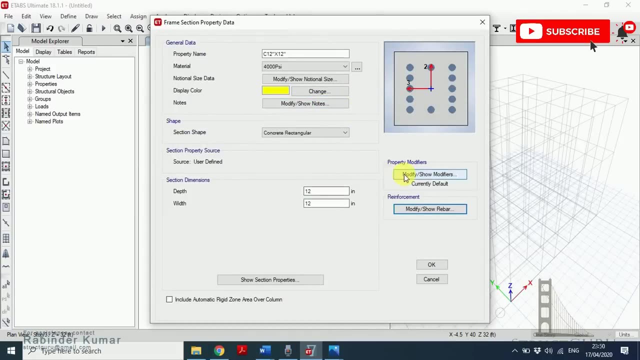 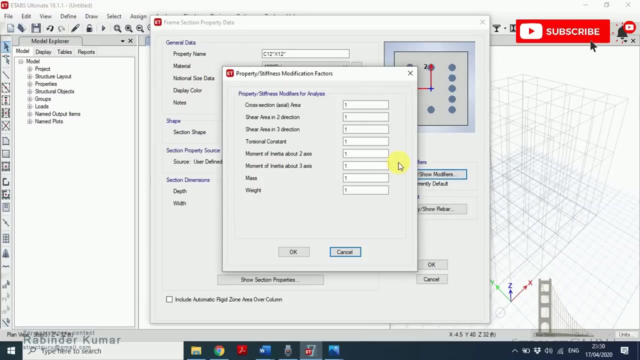 reinforcement to be designed. that's why we are using the software. if everything is given by a user, then there is no use to use this software. so reinforcement to be designed, click ok. now we have to define a beam section after. okay, let me go with the modify show modifier, as we are using ACI 31814 code, so in this code we have to change: 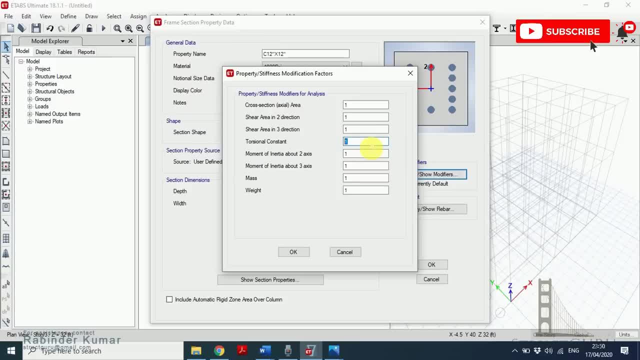 these values. I will explain the purpose of changing these values in the end of my video. so for torsional constant, the code recommends the value of 0.0. 1. for moment of inertia- about 2 X's for a column: 0.7- 0 and moment of inertia- about 3 X's for a. 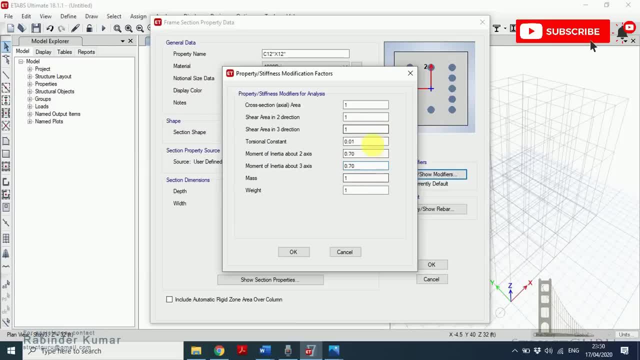 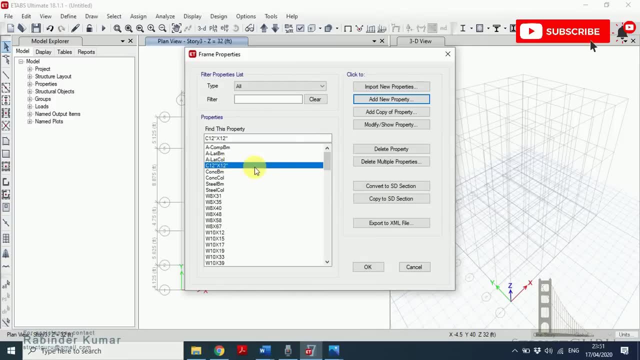 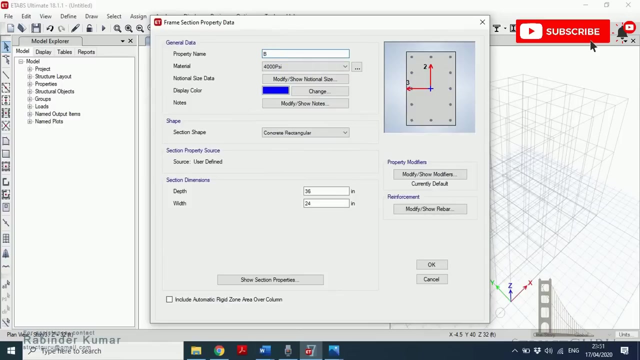 column 0.7, 0. after modifying these values, click OK, click OK. so we have successfully defined the column. after defining the column, we have to define the beam. the beam is normally rectangular, so this is the beam. start with P. so I am using b12 by 24 inches, so I am assuming this dimension. so depth of 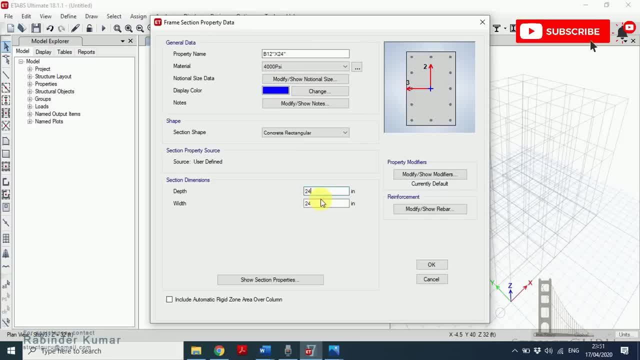 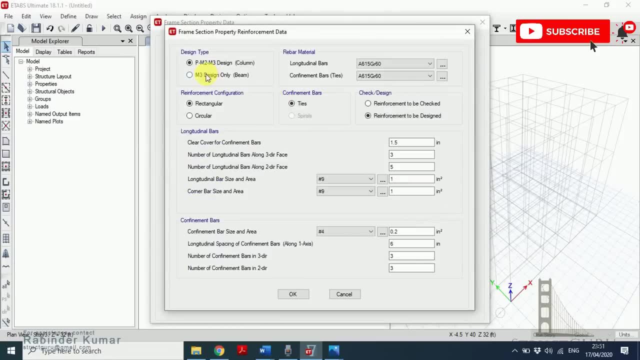 beam is 24 inch and the width of beam is 12 inch. again go to modify show rebar. column click beam, because we are going to define a beam over here. beam space is 12 inch, so you have to modify this dimension. so for that, we are going to define a beam by 12 inches. so again go to modify show rebar. 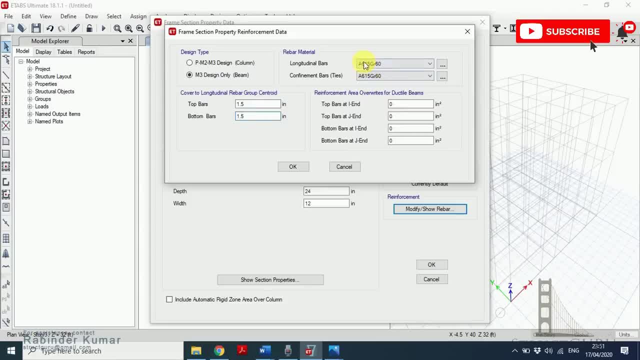 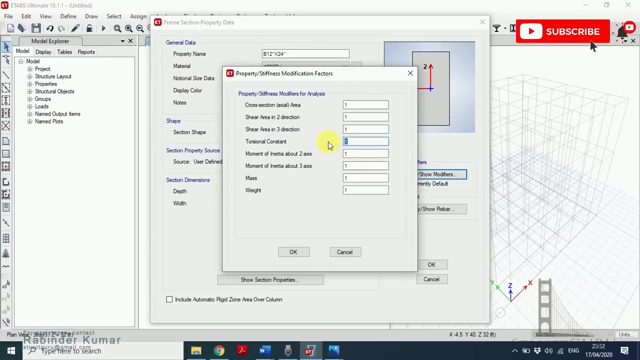 1.5 inch, which is kept normally. again the longitudinal bars and using 60 grade steel bars. for the confinement bars, again I'm using 60 grade steel bar. click OK then go to the modifiers. for torsional constant, ACI code recommends the value for a beam should be 0.01. moment of inertia about x-axis is 0.35. 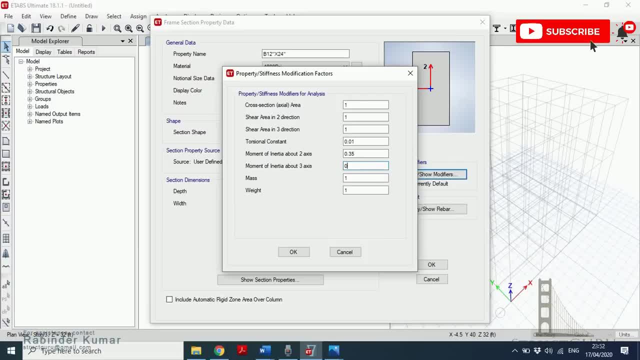 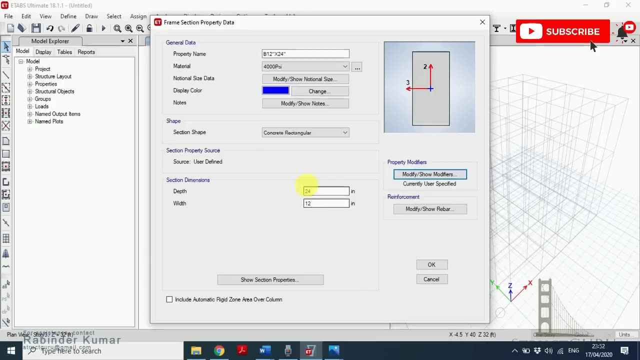 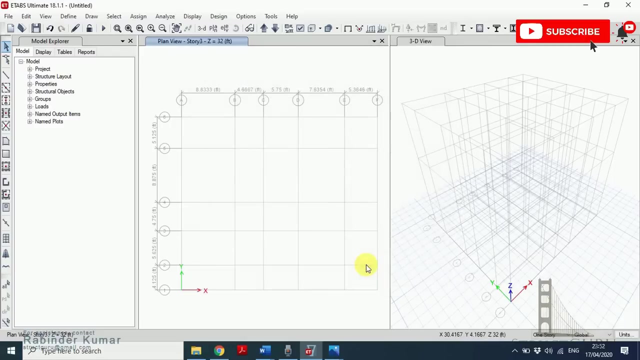 moment of inertia about 3x is again, the value is 0.35. what does it indicate? I will explain later in the end of this video. so all the parameters are defined. click OK, click OK and we have to define the slab as well. go to the define menu. 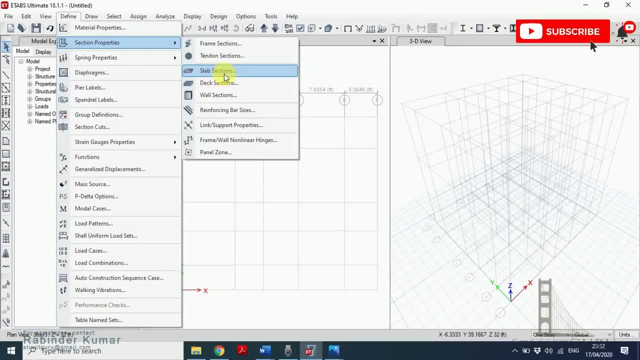 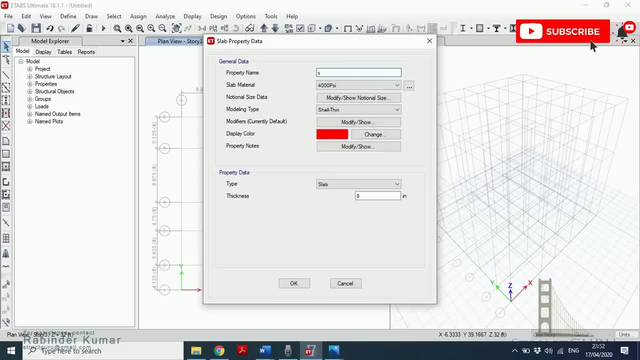 and section properties. the third option is slab sections. so slab. add new property: slab. normally slab is assumed with six inches thickness. so for slab we are going to change the material. we are keeping it as 3000 PSI also change dimension over here six inches, click OK. 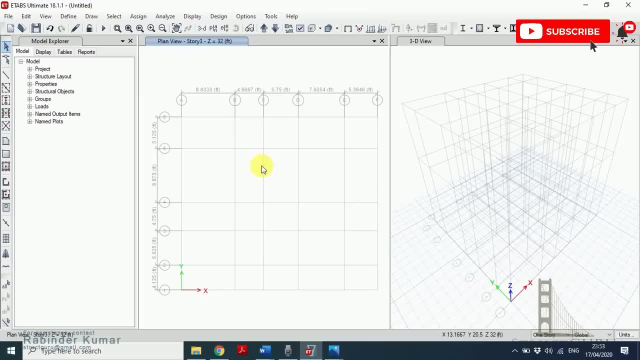 as we have successfully defined the material properties, now we will assign the material properties. so for assigning, as you can see, there are several elements over here. this is element. this icon is used for drawing a beam column width, and the description is also written when you put the cursor on this. 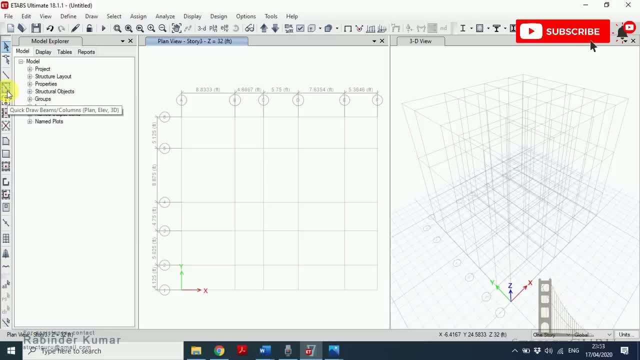 icon. similarly, this is the quick draw tool. if you want to draw the beam in a grid in this grid, just click this option. by default it will draw a beam between these two grids. another option is on the bottom of this tab. you can see one story, all story. 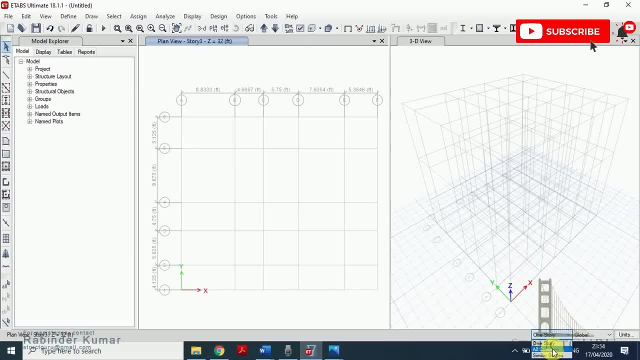 similar story story. normally our column goes throughout the building. so in order to reduce our effort, we always work with all story building. so I'm using all story building, so I'm using all story. first, we will draw the column. so I've selected the column from property. we will select the property we have just defined. so 12 by 12 inches. 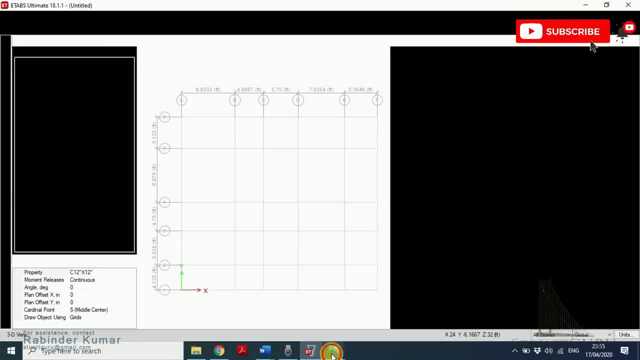 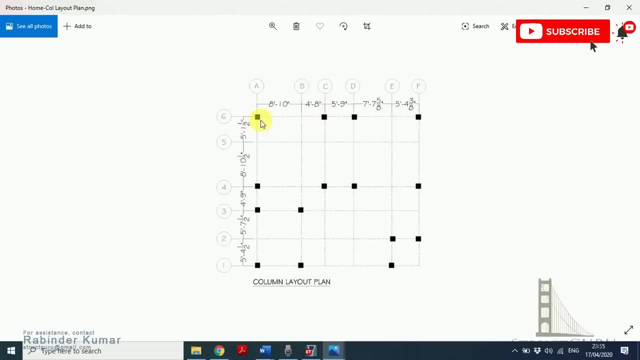 go to your column layout plan and said the location A. so along grid a6 there is one column long grid c6 there is one column long grid d6 there is another column. along grid f6 there is another column. as you can see, the center line of this beam is not passing through the central line of this column. 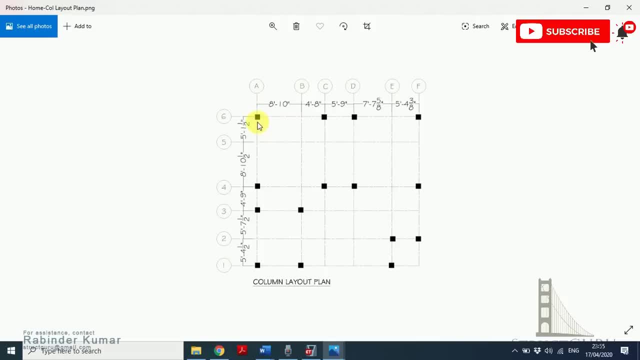 but for our case we are considering the. both lines are passing from the center. so why i am considering this? to consider the simple case, to model our structure in actual. whatever the position is given here, you have to model the same position in your etabs software. so for how to do this, for example, this is one and half inches away from the center line. 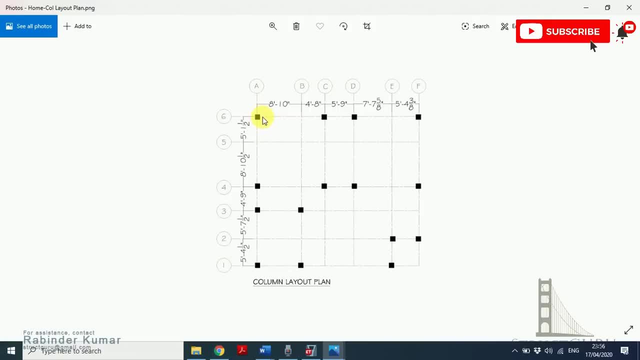 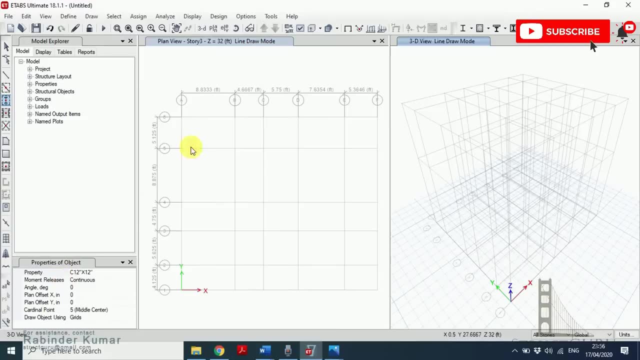 okay, and this is approximately one and half inches below from the center line of this column. so for this case, how we will model. so as you can see, in property section there are different seats. if you want to roll the column by certain angle, you have to put some value over here and automatically. 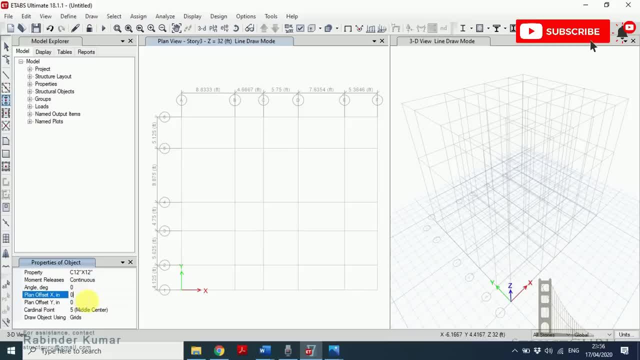 your column will be rotated if you want to place your column at a certain distance from this grid line in x direction. so you have to put some value over here. so this will mark your column away from the center line in positive x direction or negative x direction. 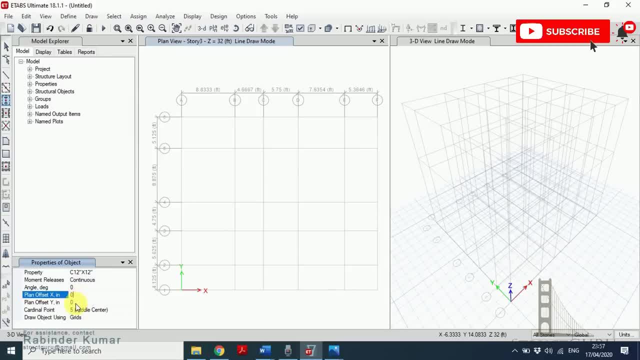 similarly, if you want to do the same in y direction, just put some value over here. if you want to keep model the pure column away from the grid line in positive y direction or negative y direction, just put some value over here. so for our case, we are considering both. 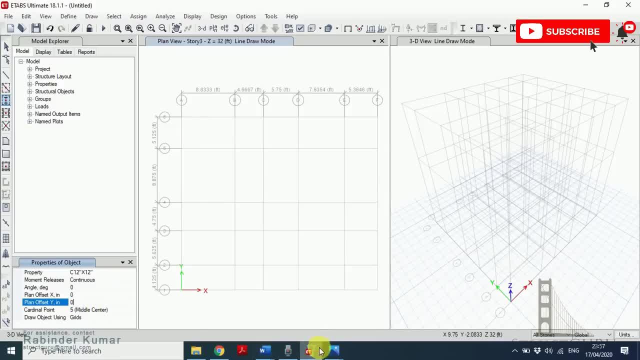 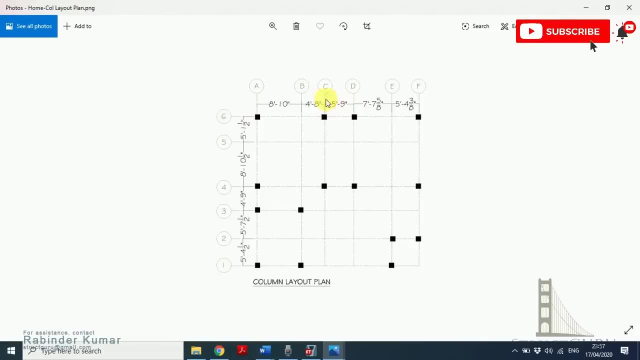 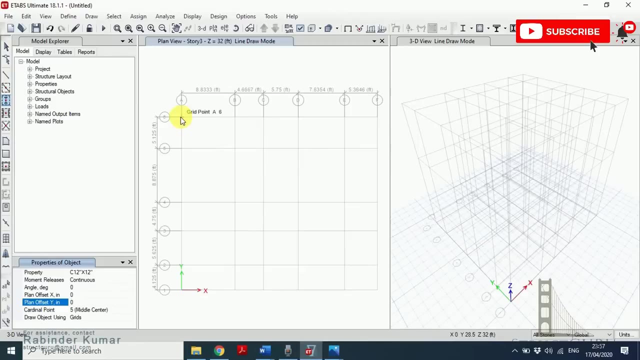 lines are passing from the same center line. so as we have seen from our column layout plan, so along along a6, c6, d6 and f6. there are four columns, so along a6, a6, c6, d6 and f6. so there are four columns. so this is the column a6, c6, d6 and f6. 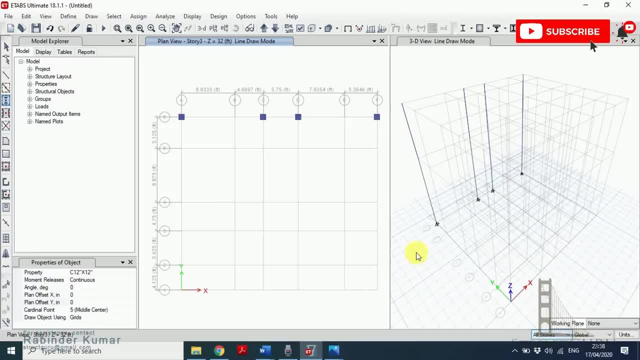 the benefit of clicking all stories because we are in story three. we are just inserting the column at story three and it is going to replicate on all other floors. for example, if you click only one story, we just click a column over here, it will draw for only one story. it will cost our time again. I'm 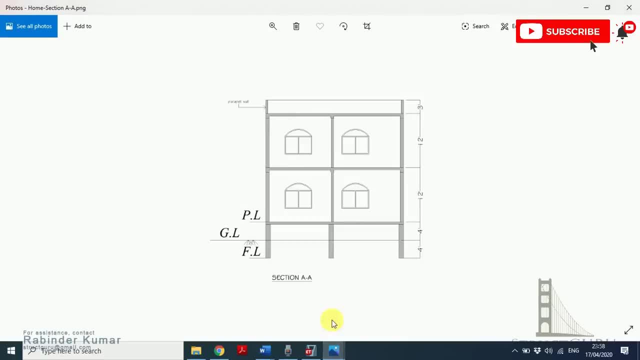 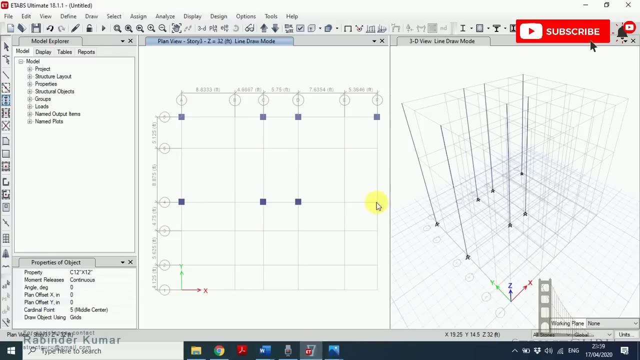 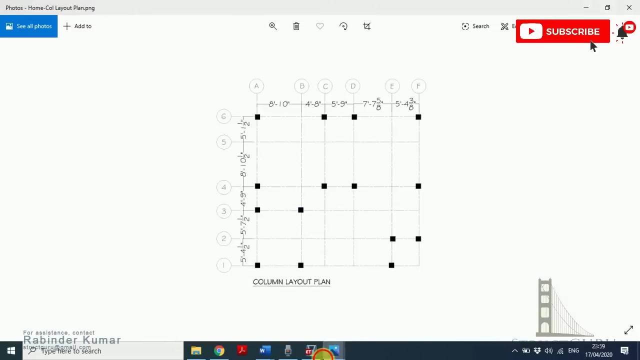 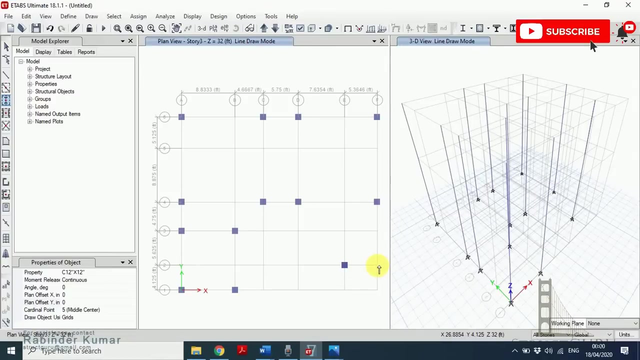 going to click all the story again. go to our central layout plan. so along a4, c4, d4 and f4 there are four columns, so they消 by single next column. as you can see, we have successfully placed all the world columns in our model along the grid line. now we will place the beans, so click this icon to. 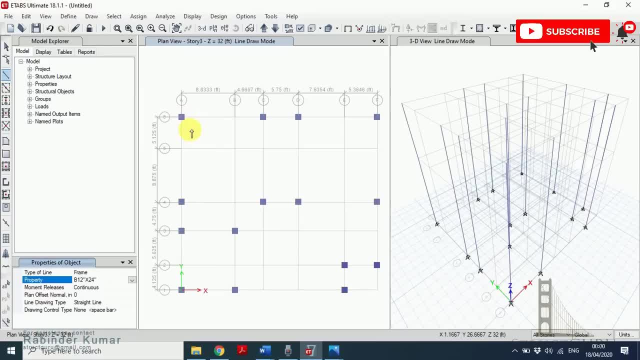 draw the beams from properties menu. change the property we have just defined. order to draw the beam, you have to click at the start point and you have to support the beam at other end of the column so our beam is drawn. similarly, do the same. so to know the exact location of the beam, we have to refer our beam. 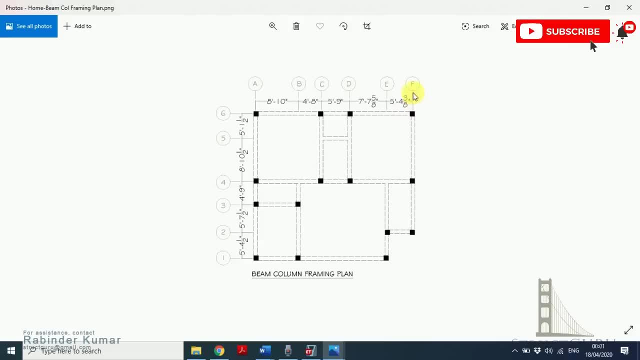 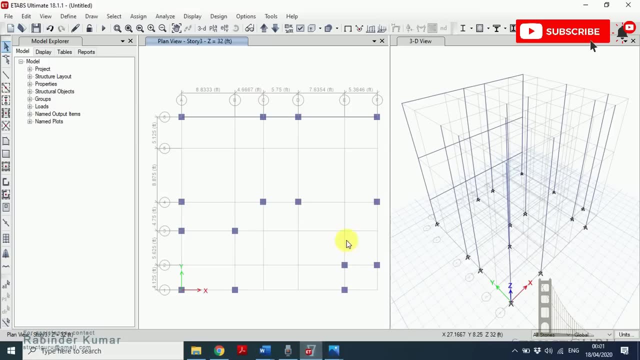 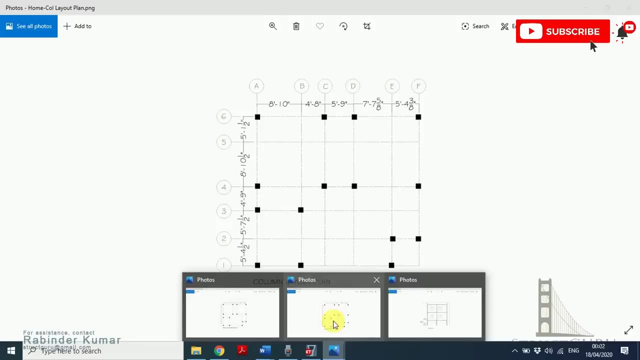 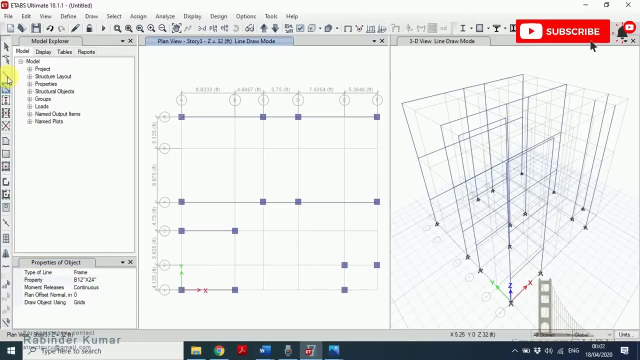 column layout plan. as you can see, from A to F, there is a beam. from F to grid 2, there is also a beam. so you have to follow this plan. you, you, as you can see, we've successfully model all the beams referring to our beam column framing plan. so these icons are used to move the. 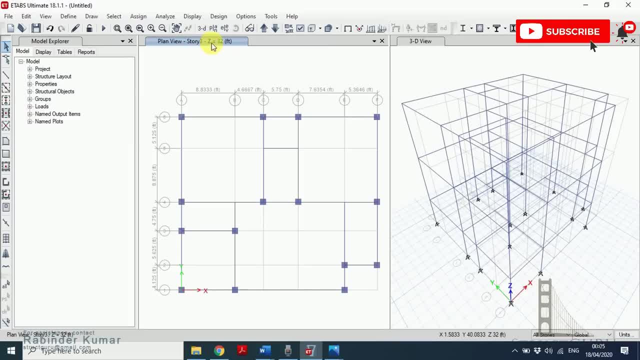 along the floors. as we are currently, we are on story 3. if you want to go blue- story 3, click this icon. so we are now at the story 2. if you want to go up, then click this icon. proof level: now we have to place the slabs, so this icon is used. 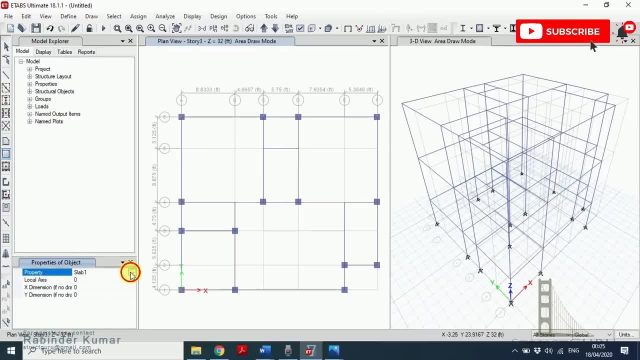 to draw the slabs from property menu. select the property. drag the slabs as we have selected all the store lease. so it will draw the Dean belong all these stories a piece view. like similar stories, it will probably skip the foundation devil. so, as you can see, there is no being drawn along the 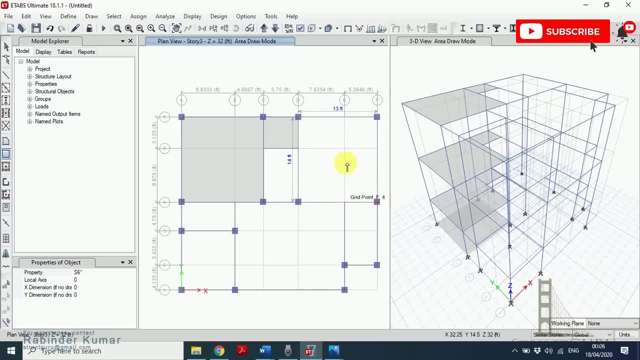 foundation level. so again, there is no slab is drawn at the foundation level. similar stories means the height of store is same. as we know, the height of story from the foundation level to first point level is 8 feet and for rest of the floors this height of the floor is 12 feet. so in this way you have to model. 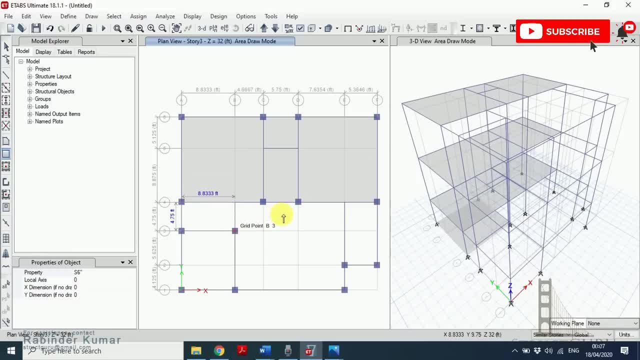 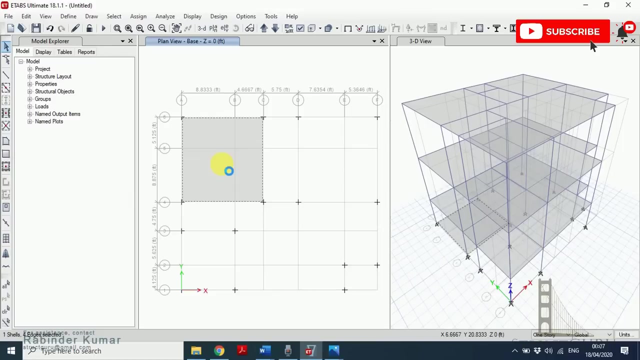 your slaves. so we have successfully placed all the slabs. go to the foundation level. we don't want slab here. so from smaller story click once this one story. click this slab and press the delete button from your key board. this slab will be vanished. also at the plinth level. we don't want slab. 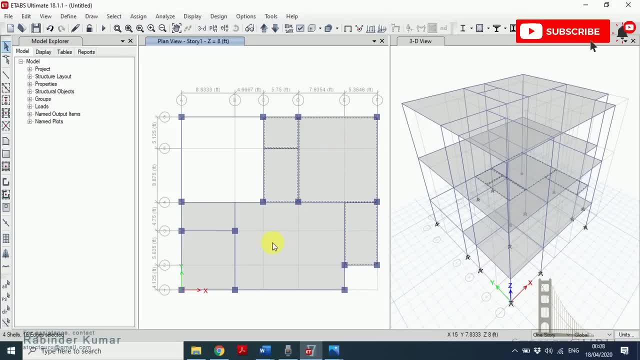 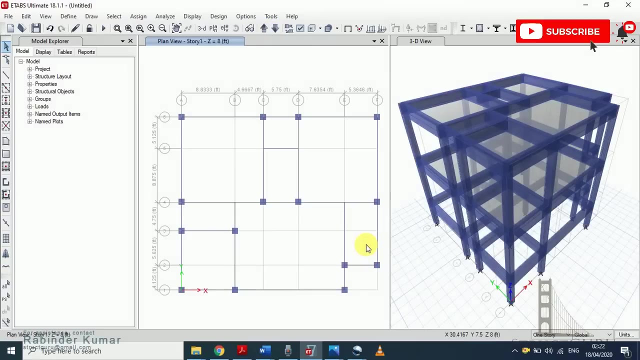 because click all the slabs on this story and delete it, because this is the first ground level. we just have to place the wall loads along these beams. so let me tell you why property modifiers are important. so property modifier are very important parameter in defining the section process. they are: 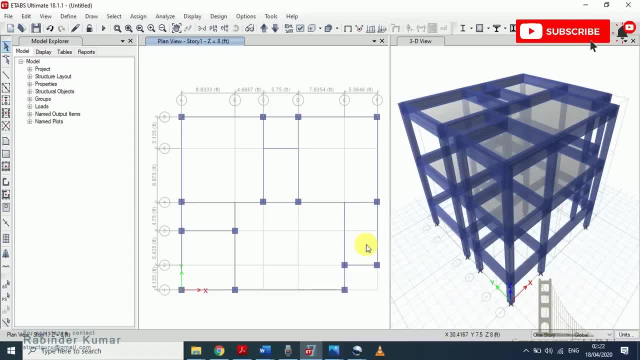 used to model correct behavior of concrete sections. as we all know that the concrete is weak in tension and strong in compression, property modifiers are only applied to concrete members only because of cracking. so if we are considering the rectangular section, the total moment of inertia is BD cube divided by 12. we all know that. 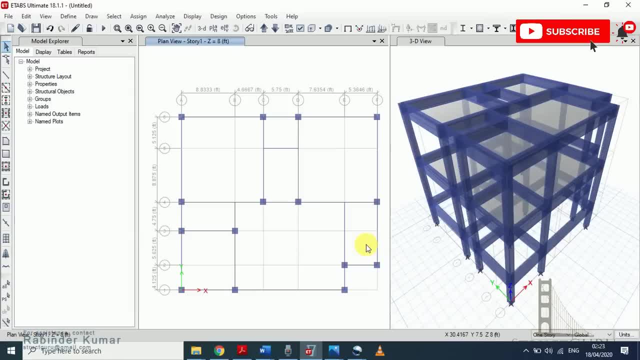 so if we are considering the rectangular section, the total moment of inertia is BD cube divided by 12. we all know that, But when you make this member of concrete, it will experience cracking when loading after some time. So this cracking will occur when concrete reaches its tensile capacity, which is about 7 to 10% of its compressive strength. 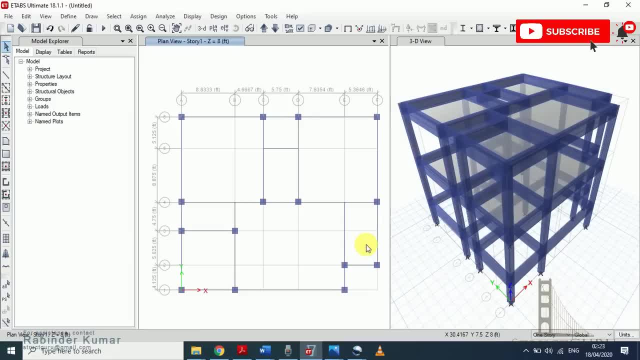 For example, 4000 PSI will have only 400 PSI of tensile strength, if we are considering 10%. After cracking, concrete is no longer able to carry tension, So steel starts taking the tension. So now, if concrete cracks after 400 PSI, the moment of inertia will be reduced because of cracking. 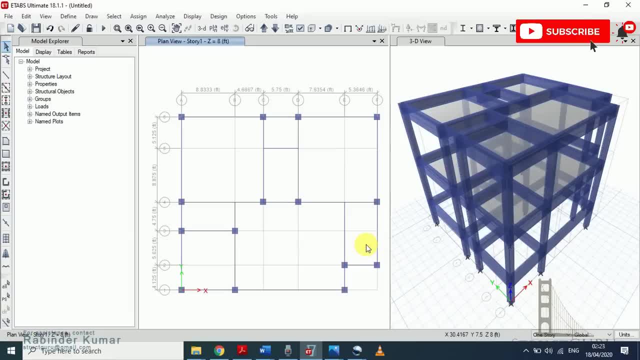 If the moment of inertia is reduced, the capacity of section to resist the bending is reduced, Its stiffness is reduced, The concrete will take less moments. Its deflection will increase due to less stiffness. So this moment of inertia which the crack beam is not taking anymore, 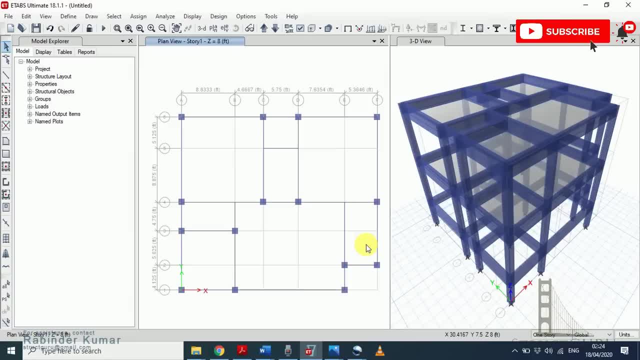 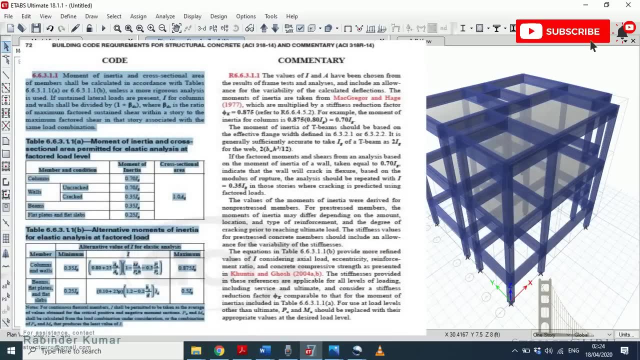 Will be redistributed to the other structural members based on their stiffness. That is why ACI codes suggest different values for property modifiers for beams, columns, slabs and wall sections. Capacity for beam section is reduced to 35% and capacity for column section is reduced to 70%. 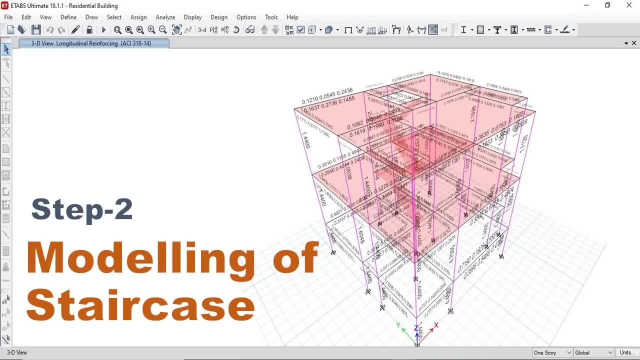 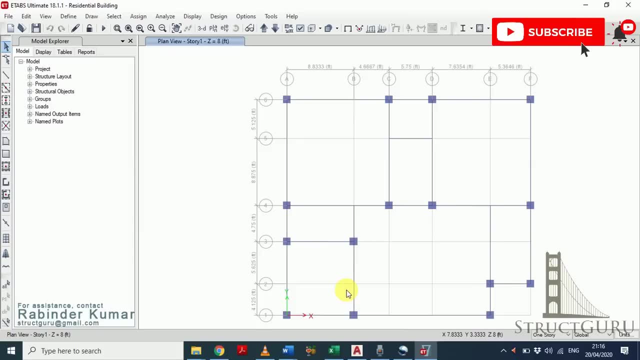 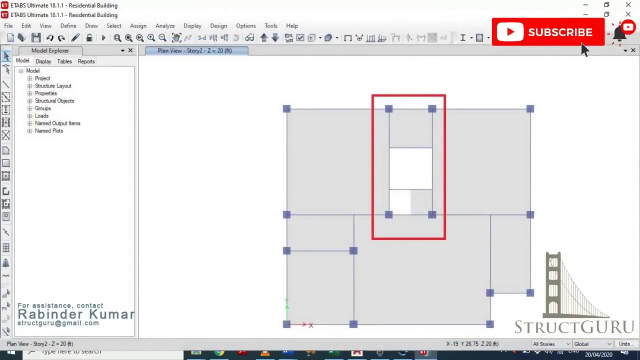 You might be thinking why we should consider modeling staircase in ETAPS, As there are other easy ways to find the reinforcement from manual methods and some charts available. So let me tell you why. to model a staircase into your structure? Because the columns on which the staircase is resting will experience maximum axial and shear and lateral forces. 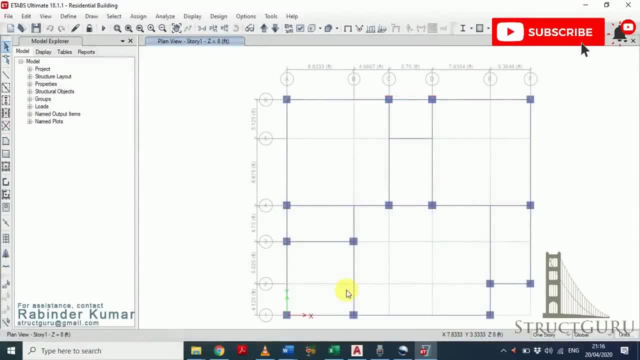 As compared to rest of the structural columns. So never skip modeling a staircase in structure. For resting the staircase system we need four columns and a beam on which our landing slab can rest. These beams will hold the staircase slab and transfer the loads on respective columns. 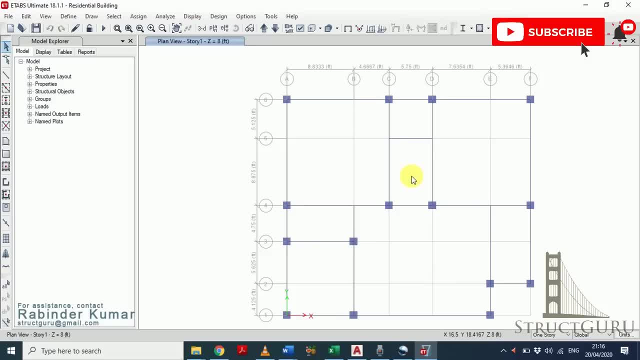 So let's begin to model a staircase in our structure. As shown in our architectural plan, Our staircase area lies in this region, So we have to remove the slabs from these areas. Choose all stories from bottom drop down list and select the slabs. 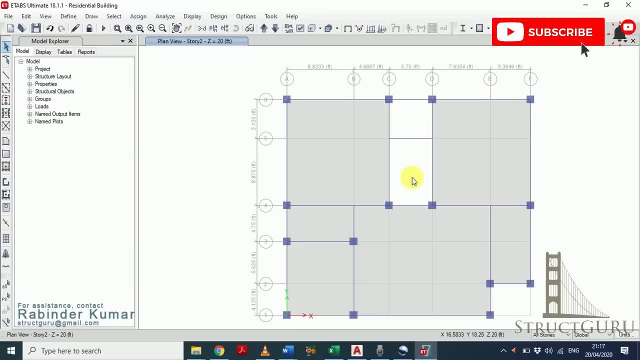 Delete them all, as we do not require these slabs between our stories. Select the beams and columns. So we have selected the beams and columns on which the staircase will rest. Right click and select. show selected objects only. In this way, we can only focus on this area. 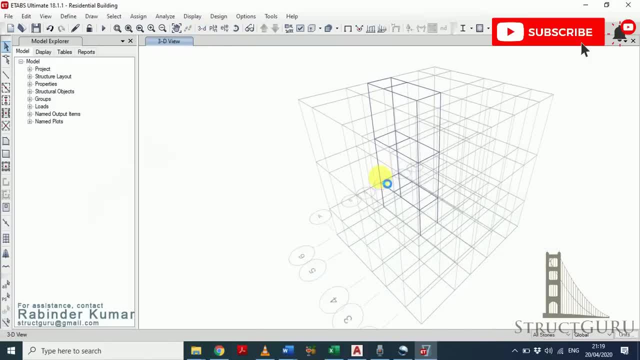 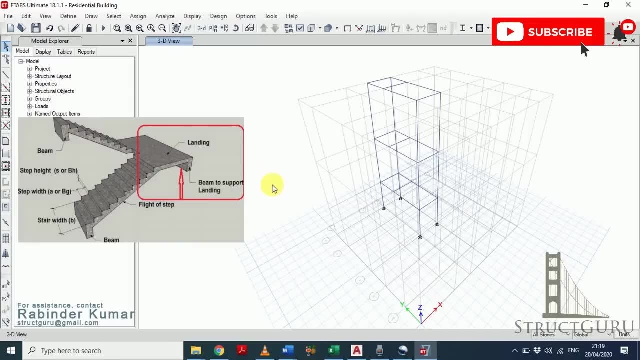 Now switch to the 3D mode. As you can see in this figure, We need a beam for the landing slab to hold the slab and transfer the loads on respective column. First we will draw the beams and landing slabs. To draw the landing slabs in midway of the story. 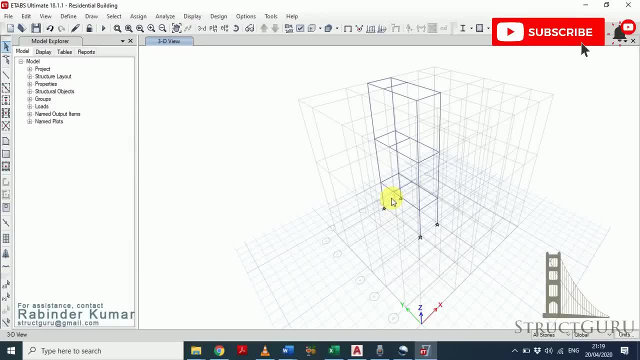 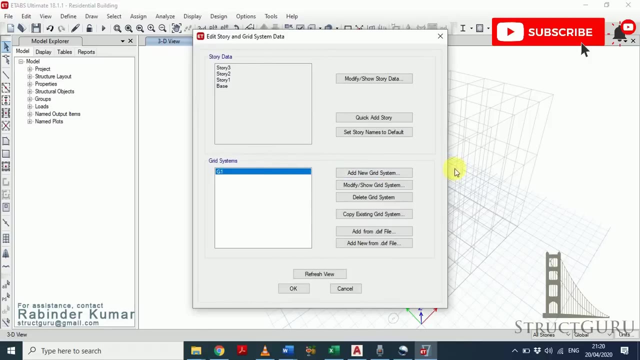 We need to define a reference plane So in this way we can reach between story 1 and story 2.. To create a reference plane, Go to edit menu And click on edit. Edit stories and grid data: Select- modify- show grid system. 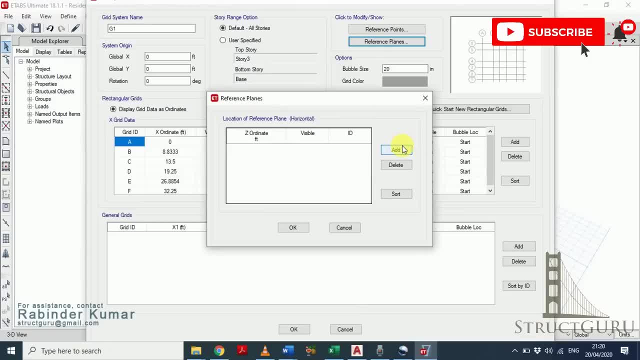 And click on reference planes. Click add. Now we have to enter a height at which we want to create our reference plane. The height will be made from bottom of the face. Our bottom story height is 8 feet And our typical story height is 12 feet. 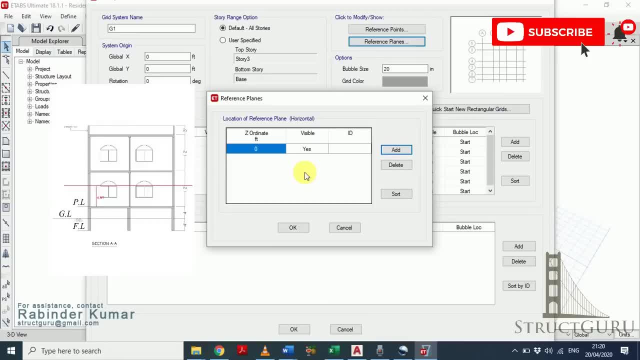 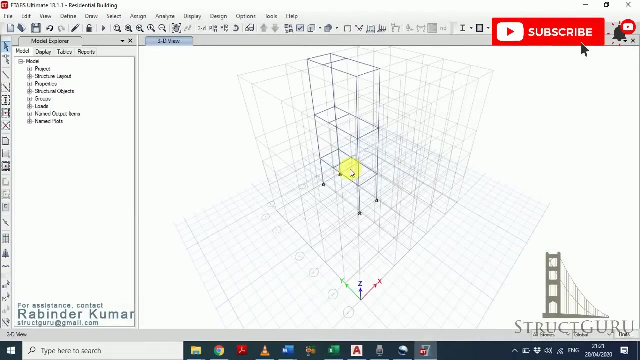 And our first landing height from the first story is 6.5 feet. So, varying from the base, Add height plus 6.5. It comes out to be 14.5 feet. Click ok, Click ok. As you can see, we have successfully drawn the reference plane. 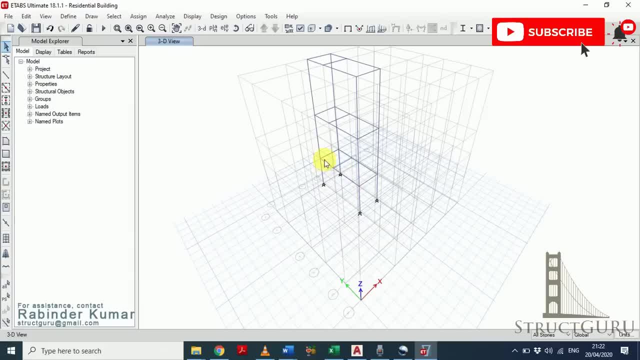 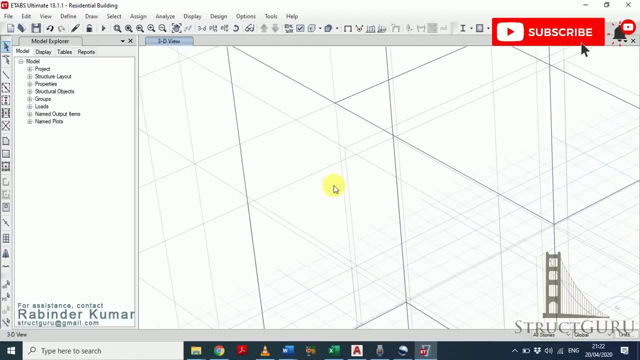 Let's draw the staircase for one story Between story 1 and story 2.. Then we will replicate it between story 2 and story 3.. So at reference level We need a beam to support landing portion of the staircase. So go to plan menu. 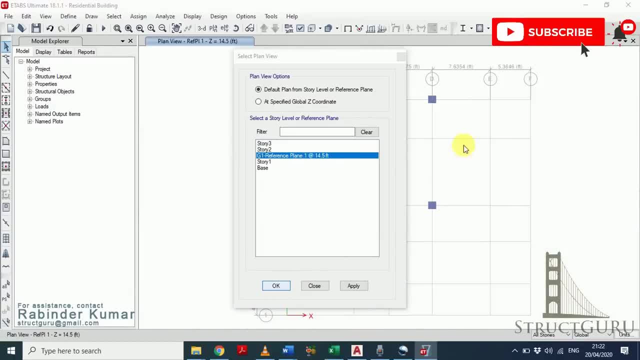 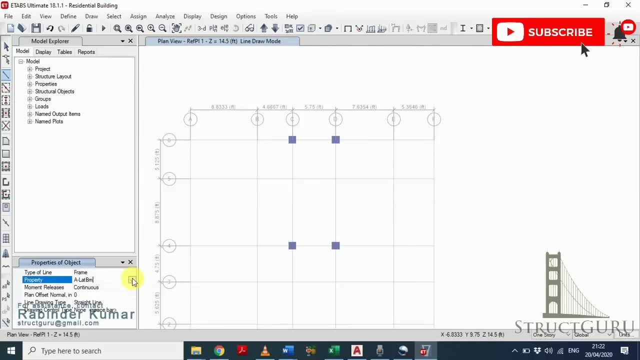 And select reference plane. Choose one story from this option. Choose a beam from property manual And draw the beam As we have to draw the landing slab at this section. Choose draw rectangular section. Select S6 slab. In this way, we have successfully created a landing slab. 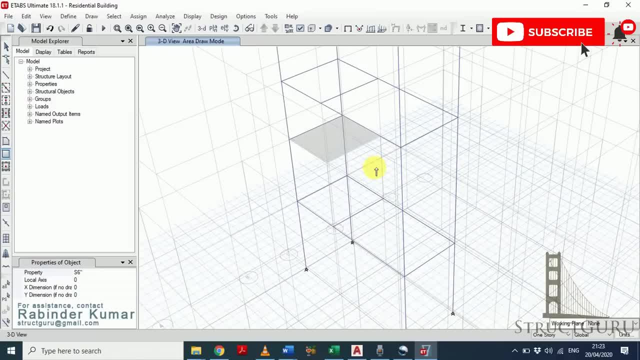 Switch to the 3D mode again. As our staircase is two legged stair, We have to draw two flights, Which goes from first story to landing And from landing to the second story. So go to plan view And click story 1.. 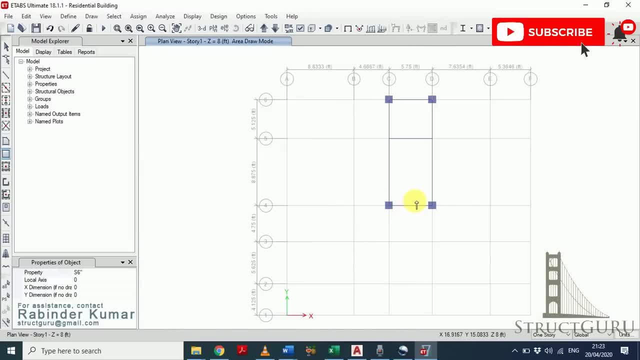 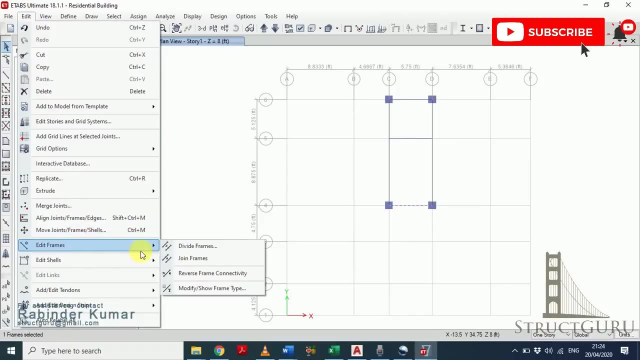 We have to divide this beam Into two halves. So we have reference points for making an inclined slab. So how to do that? Select this beam, Go to edit menu, Click edit frames. Divide frames. So we have to divide this frame into two halves. 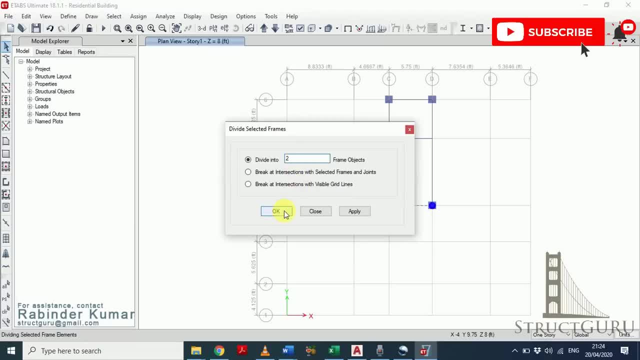 So press right 2 here And click ok. You have to do the same at this option as well. Draw a frame Now we have to do the same for the second story. As you can see from our architectural plan, Our stair is going to end. 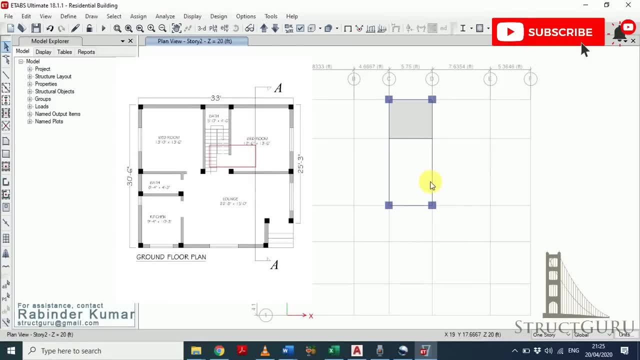 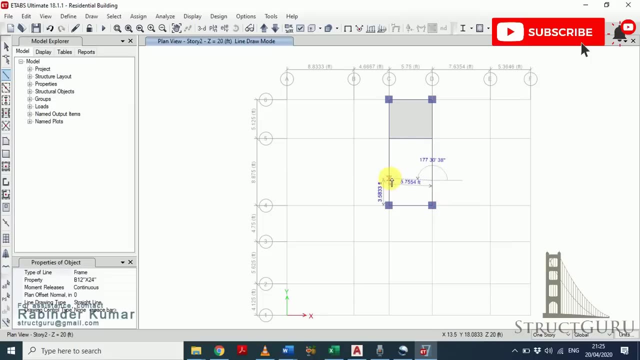 At this position. So this is approximately 3.25 feet away from this column. I will draw a beam at 3.25 feet Away from this column. Now We have to do the same for the third story. We have to do the same for the third story. 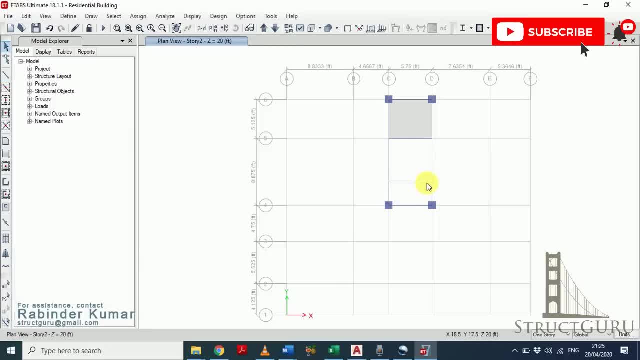 Now We have to do the same for the third story. Now Let's divide these two beams into two halves. So we are dividing these beams into two halves Because we have to create a reference point of inclined slab, To draw the inclined slab. 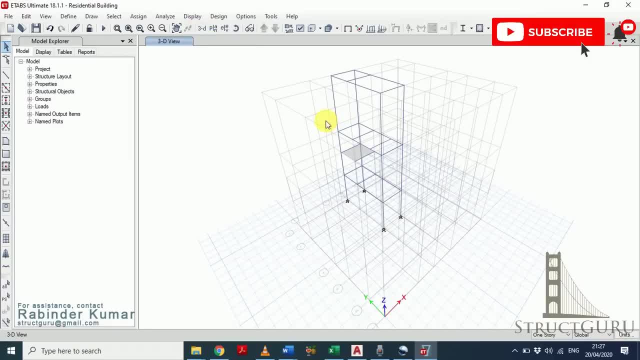 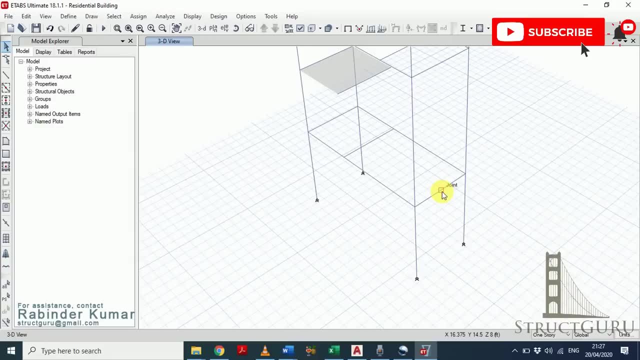 Switch to 3D mode For good. For clear visibility, I am going to hide these grids. First we have to create the inclined slab for story 1 to midway landing slab. To create a slab, click draw floor option. Click the first two joints on story 1 and click on the remaining two joints on landing. 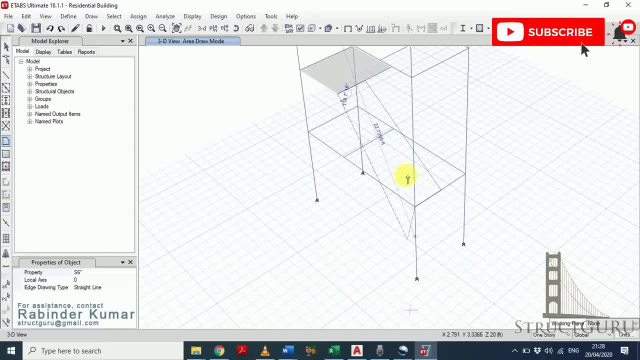 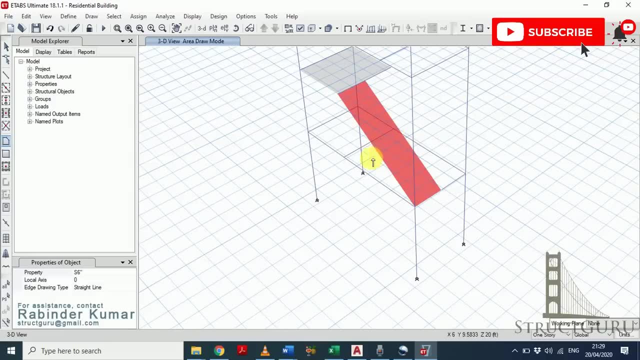 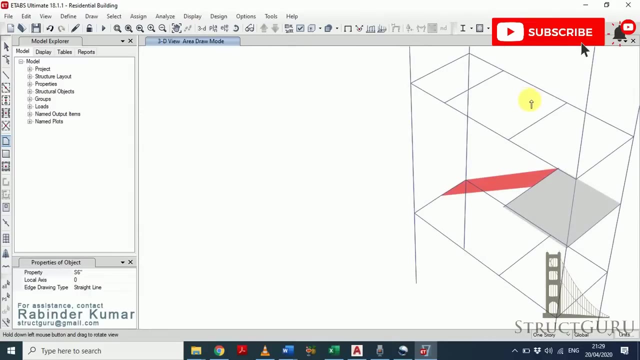 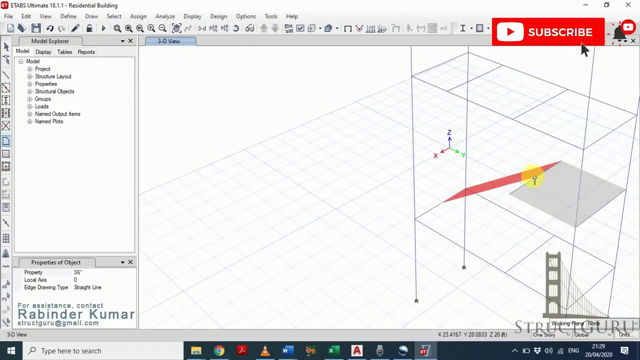 portion and click the first button again to complete the stair formation. And yes, our first inclined slab is created. Now rotate a bit and repeat the same process as we did to draw the first flight. Ok, Now assign a slab at the landing portion at story 2.. 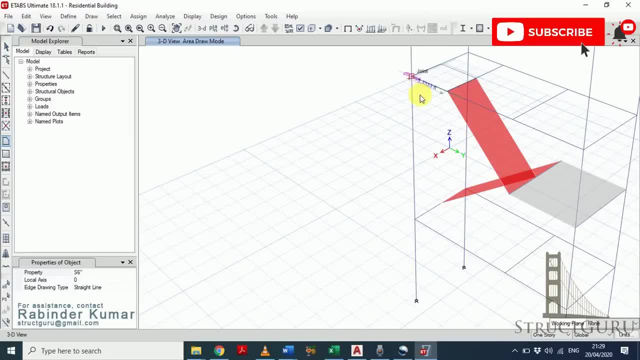 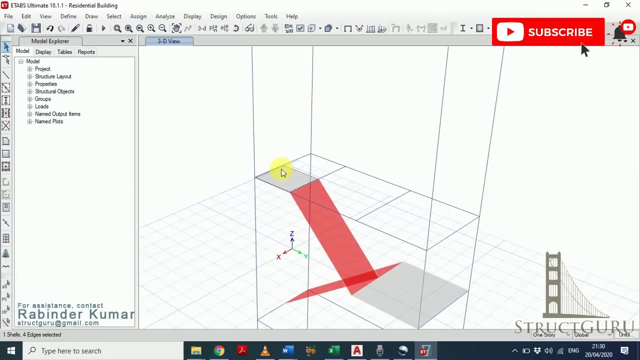 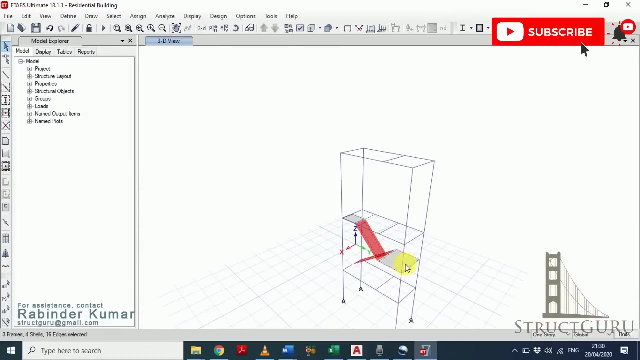 We don't want a beam at this portion, so delete it. As you can see, we have successfully drawn stair case between story 1 and story 2.. To replicate the stair for story 3.. Select all the elementary elements. Select all the elements of stair case. 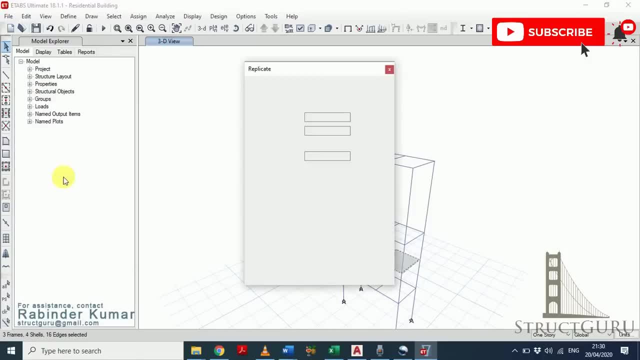 Go to edit menu and click replicate. Here you click story and we have to replicate the stair for story 3.. Click story 3 and then hit ok. As you can see, with a single click We have successfully drawn stair case for the entire building. 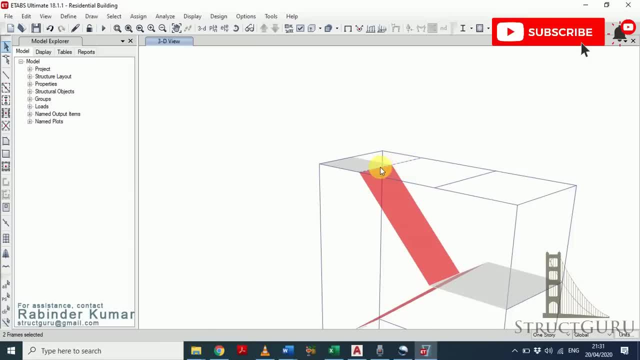 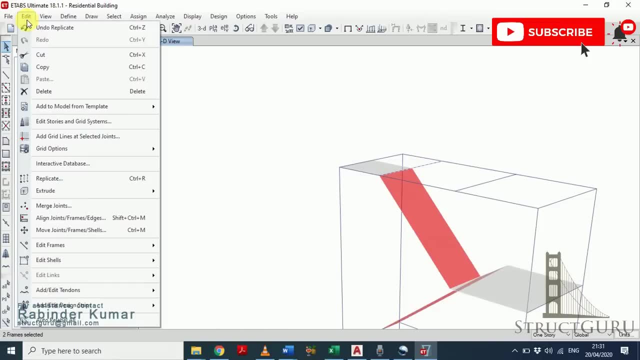 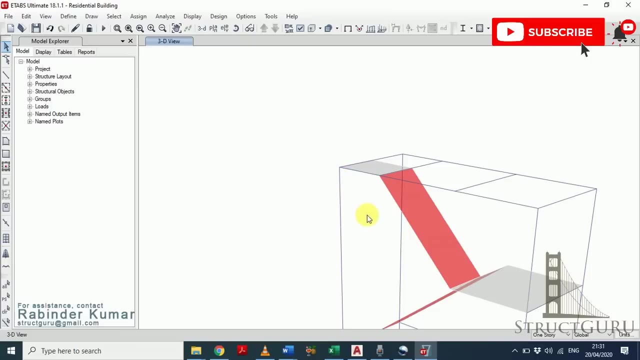 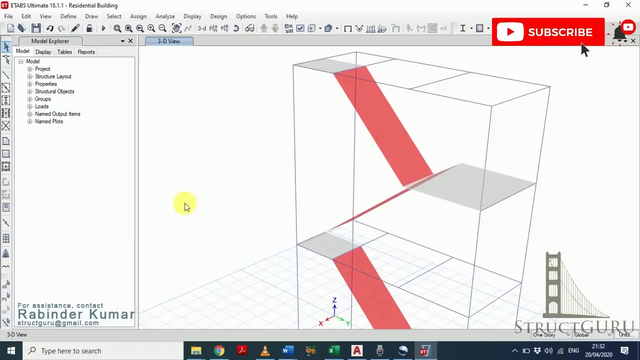 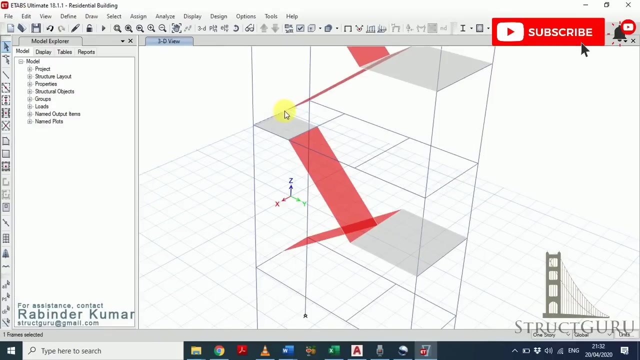 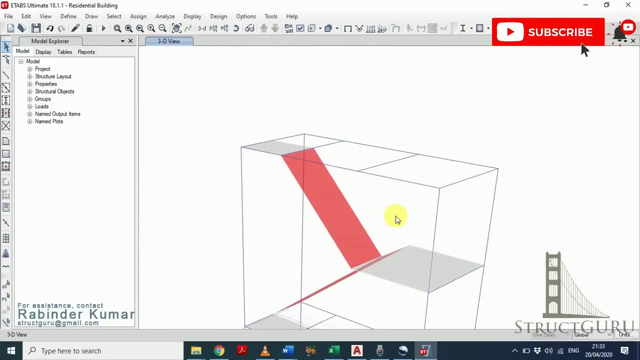 Now rejoin all the beams which we have splitted into two halves. So to do that, select the beams, Go to edit menu, Edit frame and join frame. We have to repeat the same process for all beams. Draw a slab at this portion. 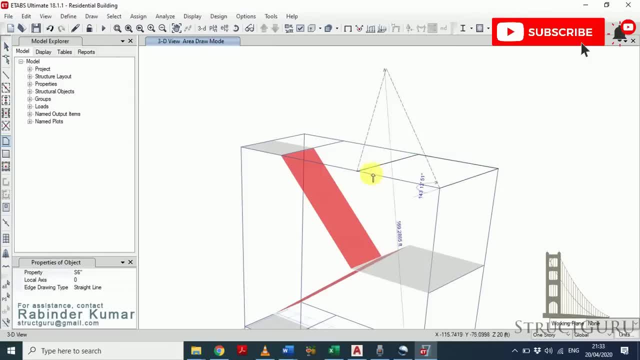 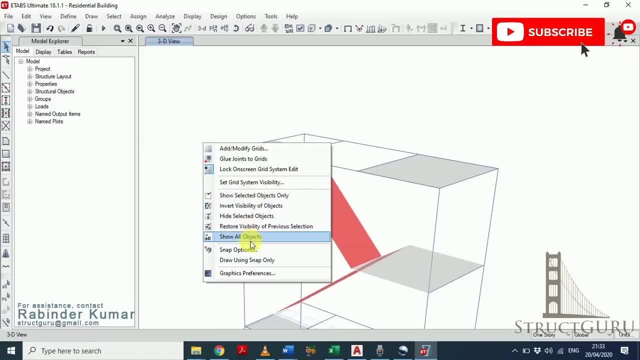 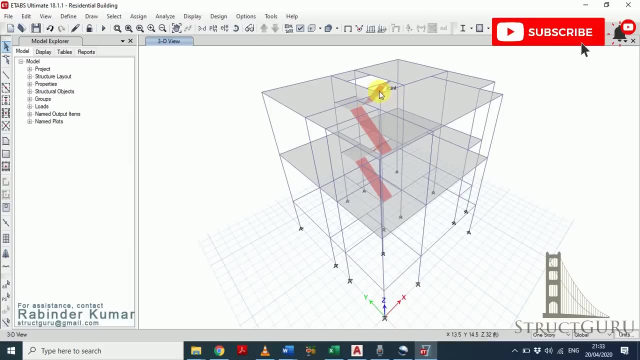 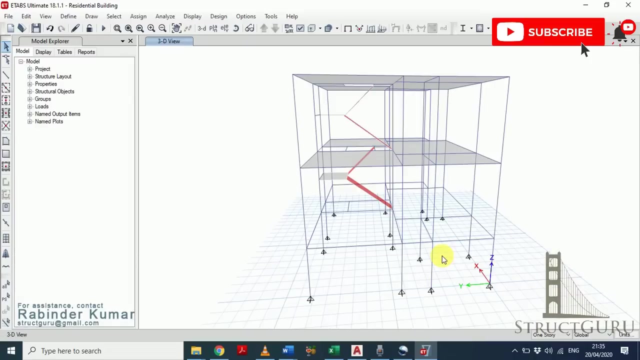 Now right click and select show all objects. Show all objects to see. We have to place a slab at this portion as well. This is our roof level. As you can see, we are done with modeling part of stair case. Now we have to calculate the dead load of steps on the inclined slab of the stair case. 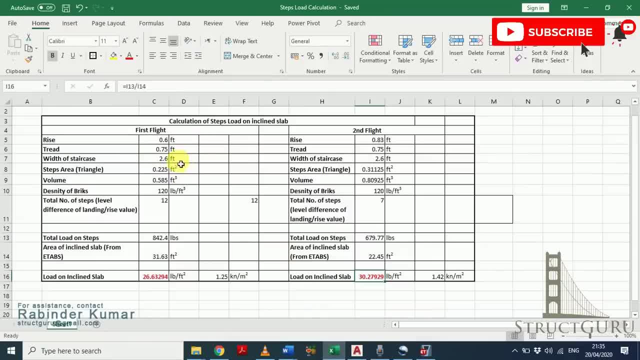 So let's go to the excel file. So here I have already calculated the step loads for first flight and second flight. The riser value in our case is 0.6 feet And freight value is 0.75 feet, So width of the stair case is considered as 2.6 feet. 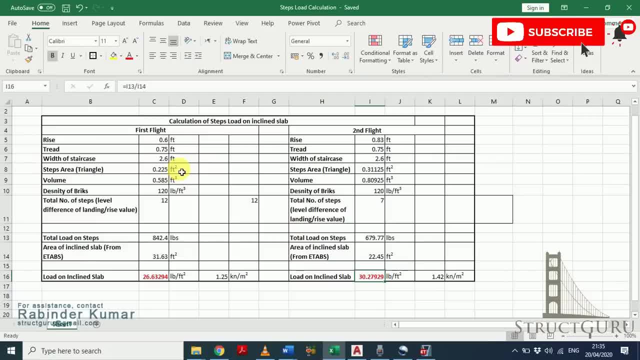 So area is calculated in a triangular shape, As you can see in this figure. So for area is half into rise into trade, which is 0.225.. For volume, you have to multiply this area with width of the stair case. Density of bricks: I have taken 120 pound per feet cube. 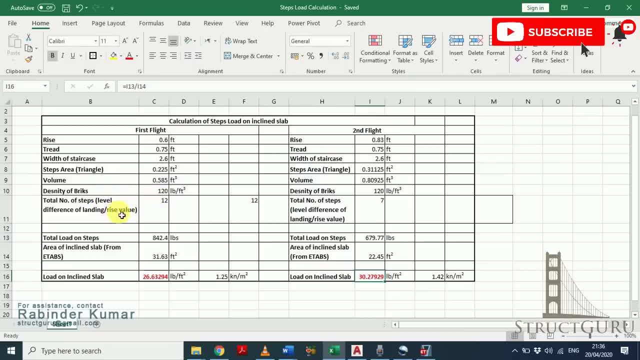 This is for the red bricks. Total number of steps can be calculated by the difference of level of landing divided by rise value. So rise value is 0.25 feet. So rise value is 0.5 feet. So total number of steps are 12.. 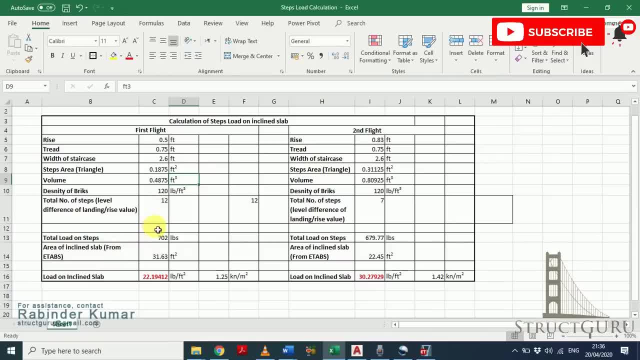 So total load on step is volume multiplied by number of steps and multiplied by density of a material. So it comes out to be 702 pounds. So area of inclined slab: you can calculate this. So we have to distribute this load into the entire area of inclined slab. 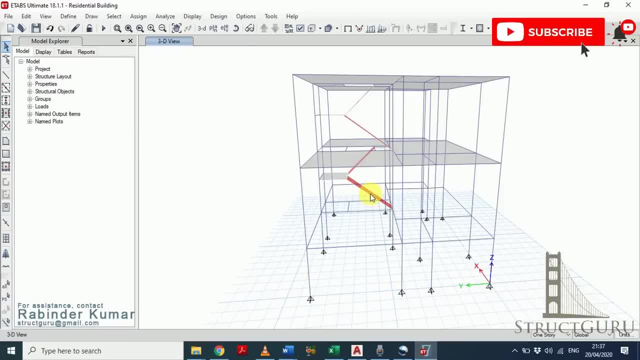 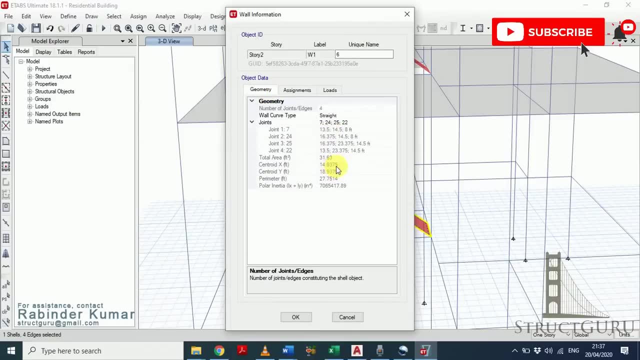 In order to find the area of inclined slab, Go to the ETABS menu, Select the first slide and right click on it, Go to the geometry section. So from there you can easily calculate area of the stair case, which is 31.63.. 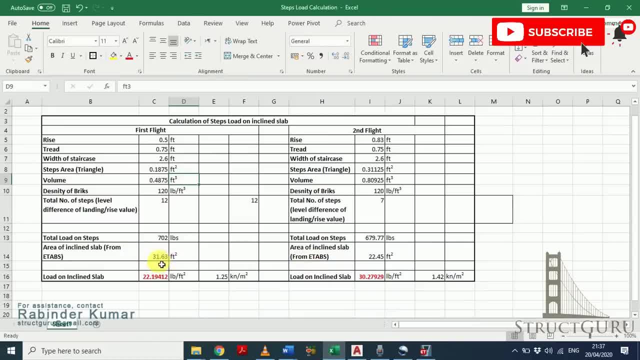 Come to the excel file again. So 31.63.. So divide 702 divided by 31.63.. So the final load on inclined slab is 22.19412 pound per feet square. And similarly I have calculated the loadings for the second slide. 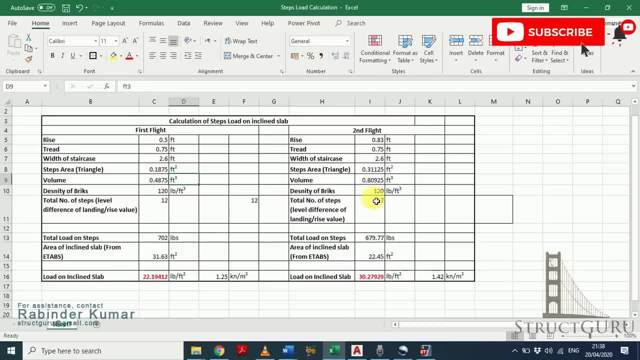 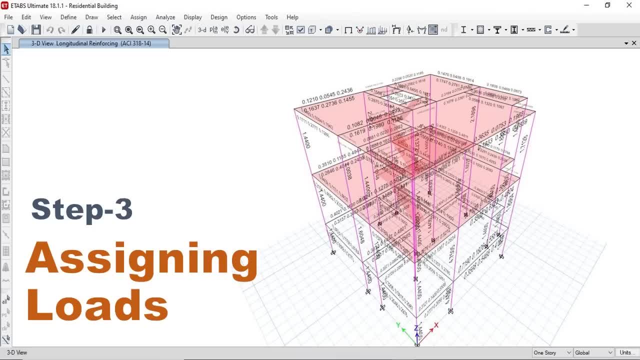 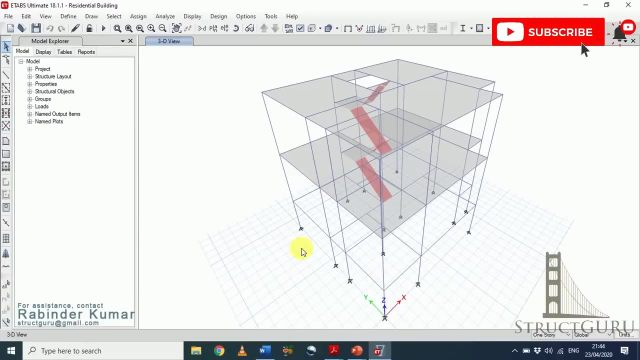 But here I have chosen different riser and tread value Because we have to adjust our stair in our architectural plan. So So, before assigning the loads, Let's look at some theory of the loads and classifications, As you can see in this slide. 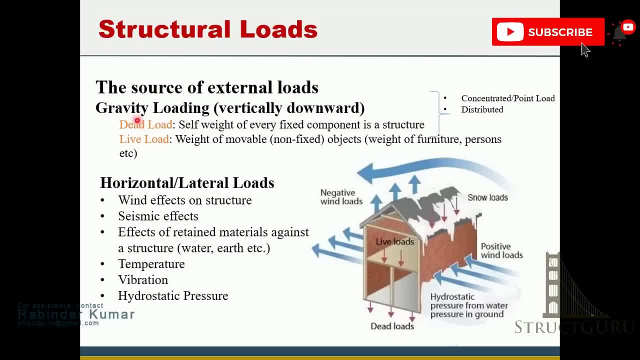 The loads are classified into two types. First one is gravity load Loads, which acts vertically downward, And lateral loads, which acts in horizontal manner onto the structure. So the gravity loads are further classified into two types. Number one is dead load. The examples of dead loads include self weight of structure. 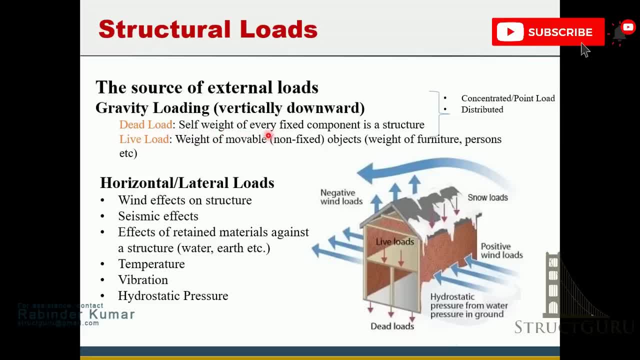 Or the weight of any permanent fixture in the structure. The example for the live loads are Wind effects on the structure, Seismic effects, Any retained material against the structure, Which could be water or earth, Temperature loads, Vibration loads And hydrostatic pressures. 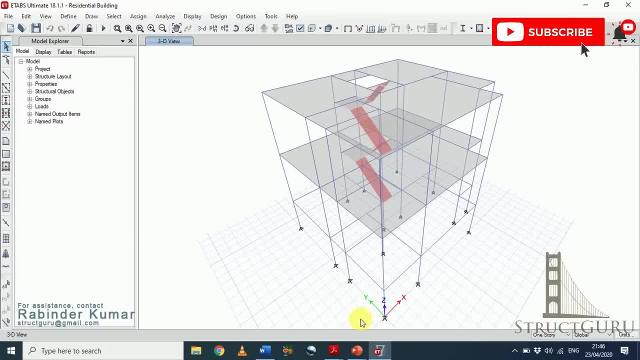 So in ETAPS You don't have to apply self weight of structure. ETAPS calculates it by its own. However, You need to apply any other dead loads and live loads which acts onto your structure. Now the question is How much weight or magnitude of weight we should apply. 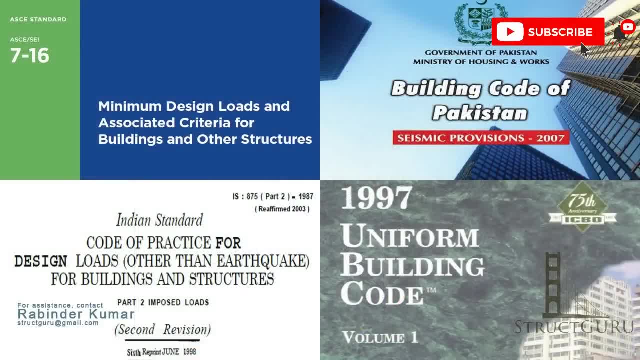 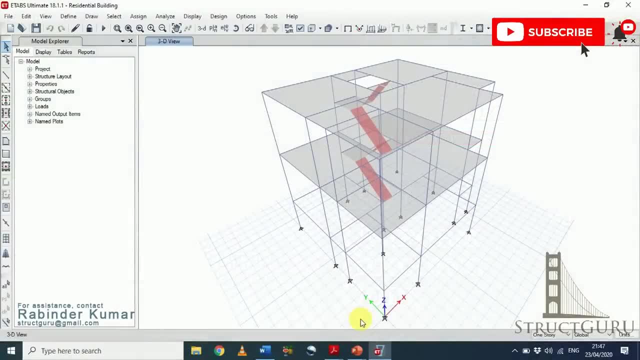 To answer this question, We need to refer code books, As I told earlier. I will refer four codes Just to teach how to read the codes And how to extract the information Of load data from the code books. And finally, We will use 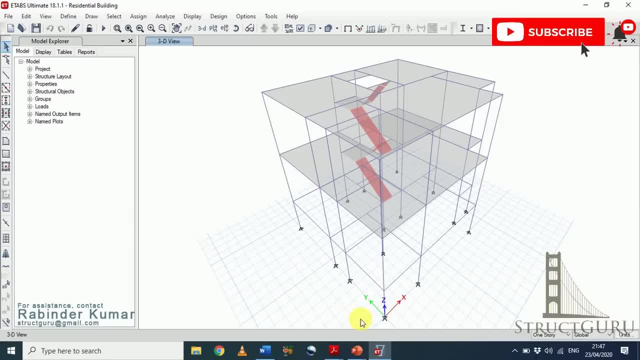 The load data from ASCE code And use in our model. So let's start from the Indian codes. In order to refer the dead loads value, We will refer to IS 875.. Part 1. For live loads, we will refer to. 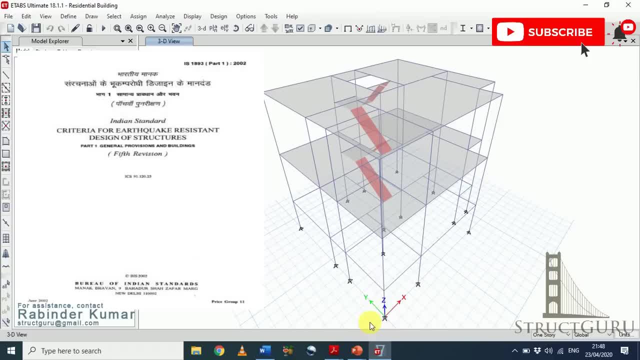 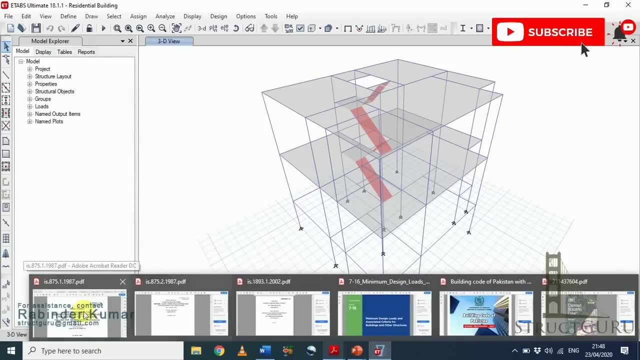 IS 875, part 2. And for seismic loads, We will take help from IS 1893, part 1.. So let's open the code book IS 875, part 1. For the dead loads. So, as I told you before, 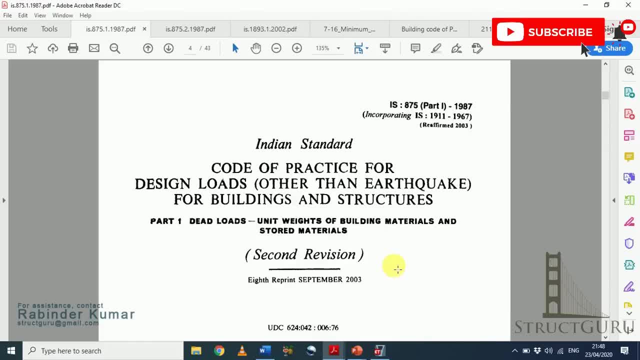 We need not to apply the self weight of structure But we have to apply permanent fixed objects On the structure. So the permanent fixed objects And dead load category Are: mortar screening Surface, finished Etc. The quick way to search. 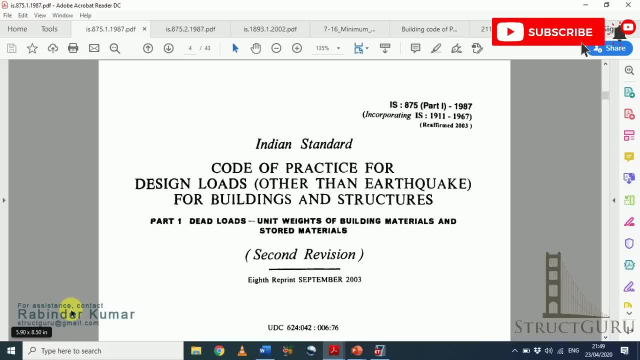 The desired data from the code book Is to press control F From your keyboard And type the T word. So we need The weight of mortar, screening And tiles. So let's find out. So just type mortar And click next several times. 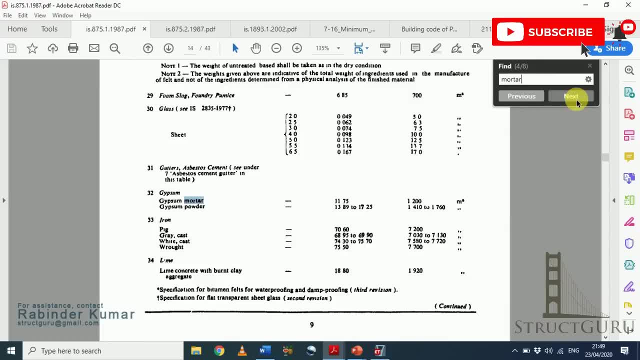 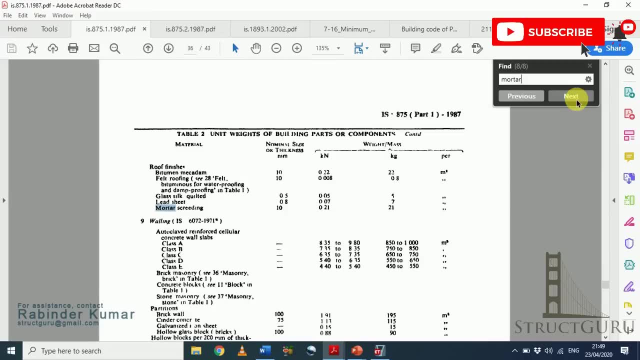 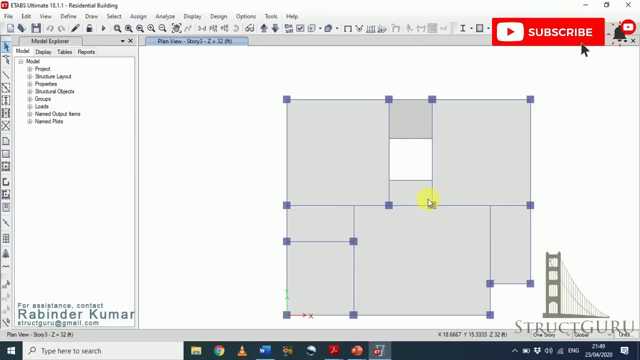 So, as you can see, There are several data available: Gypsum mortar, Lime mortar. We have to search for mortar screening. So here For mortar screening, The Either you select slab One by one, one by one, or you go to select menu from select, click select, then select object type and find out. 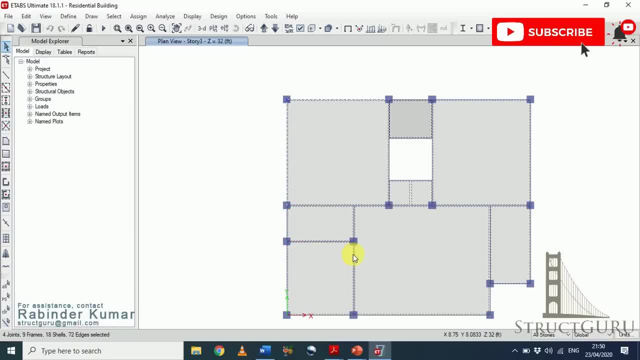 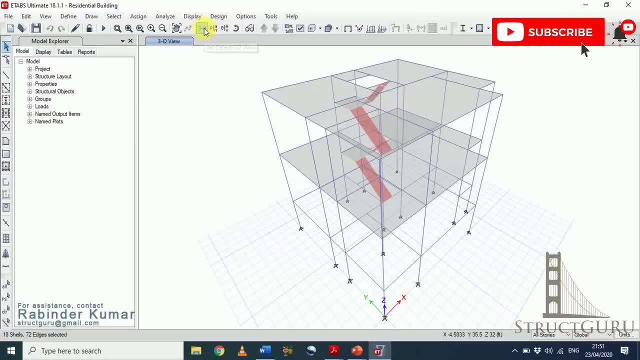 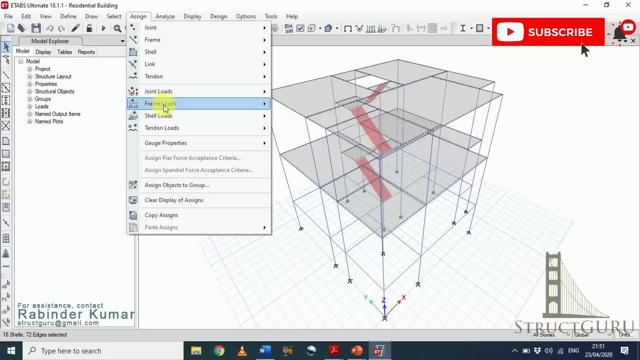 floors, then click select- close. this is a quick way to select all the slabs which are assigned into your model. as you can see, all the slabs in our model are selected. so in order to assign load, go to assign menu, click shell loads. as we are going to apply uniform loads, so click uniform. 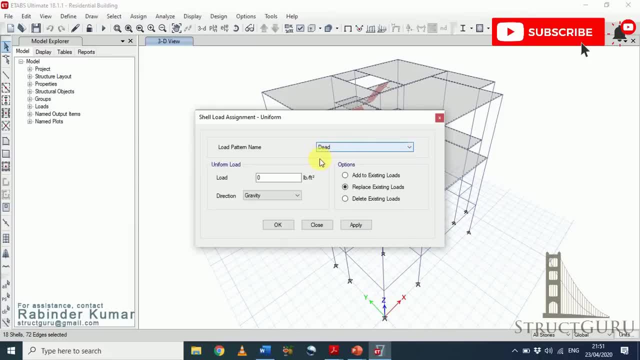 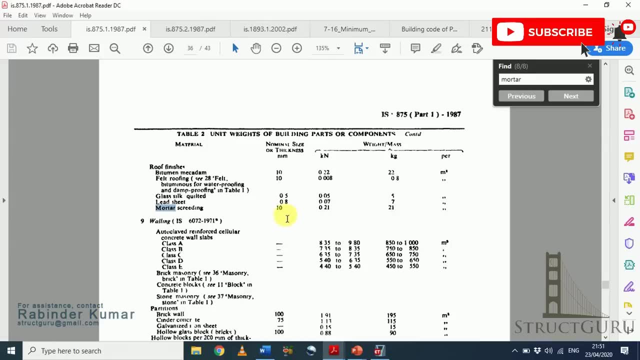 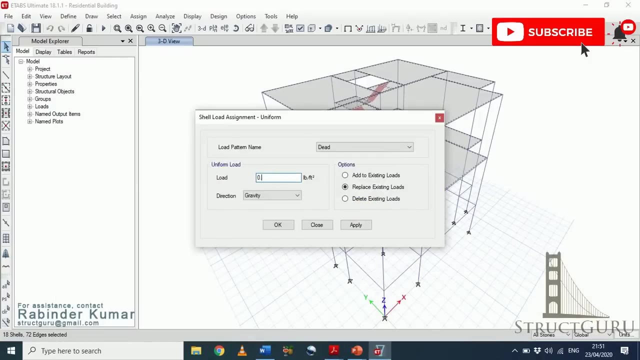 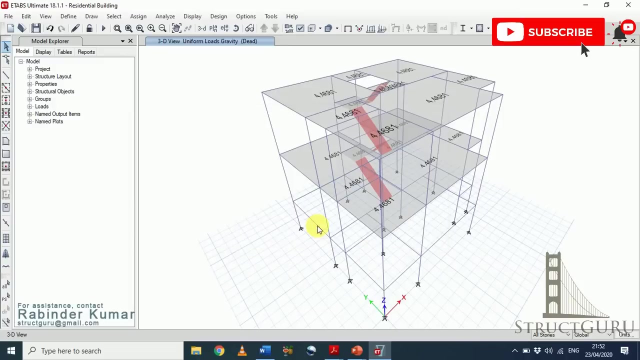 choose dead load and the value is 0.21 kilo newton per meter square- 0.21, so it comes out to be 4.46 pound per feet square. click ok. as you can see, the del load is applied on all the slabs which are modeled in our structure. after that we have to go and search for. 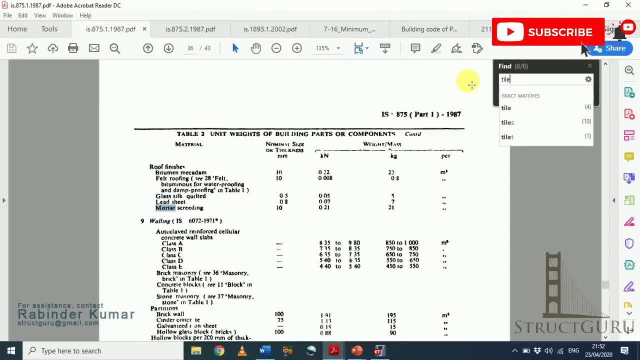 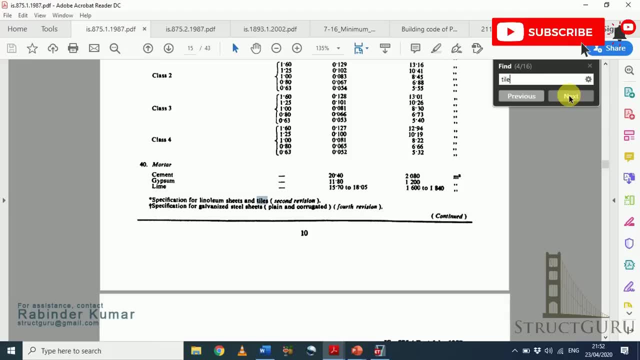 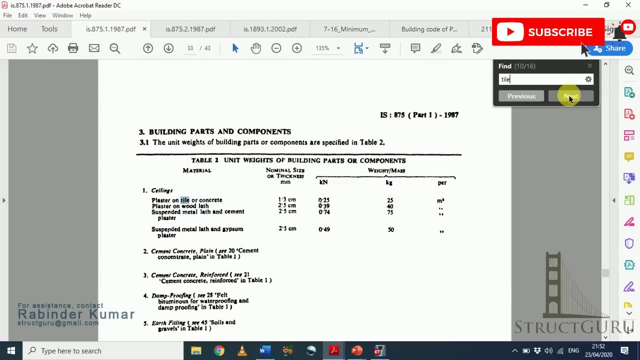 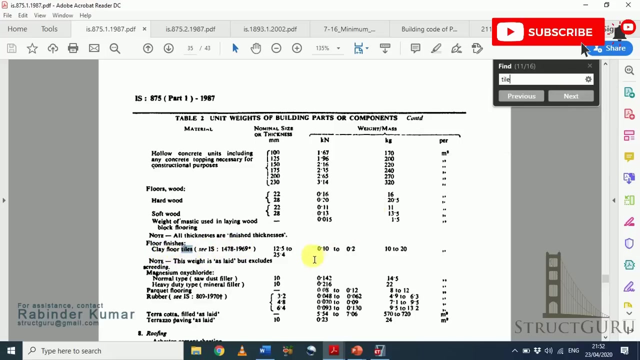 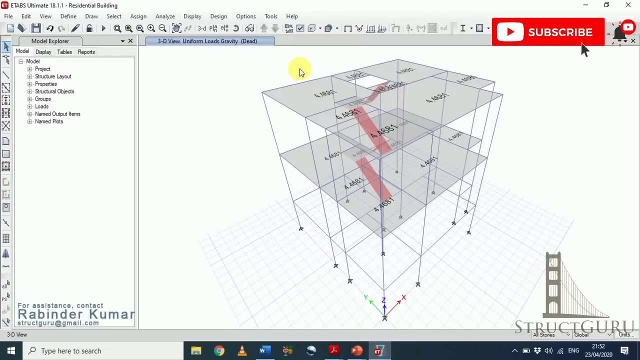 tiles, tile loads, type type. you can also assign marble or any other tile type or floor finishes. you are going to use it into your model, so tile. so let's search for clay floor tiles. so for clay floor tiles the value is 0.10 to 0.2. so we are choosing 0.2. so again go to select. 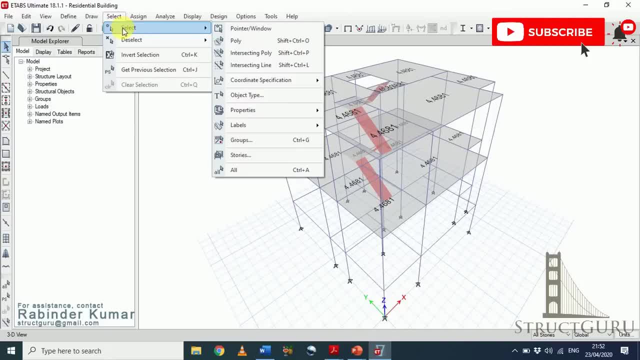 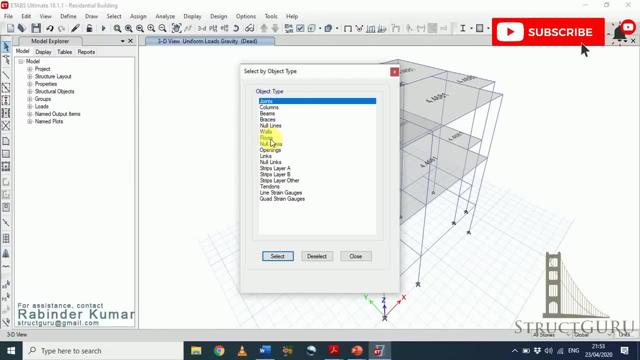 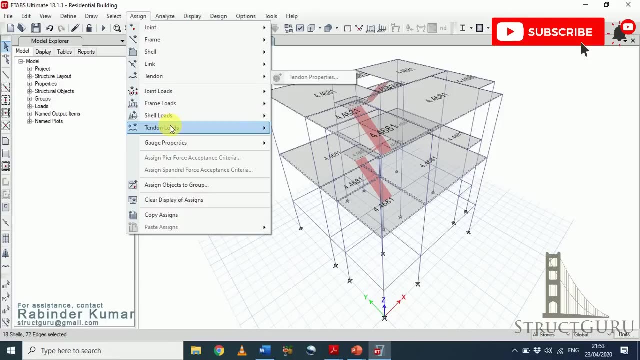 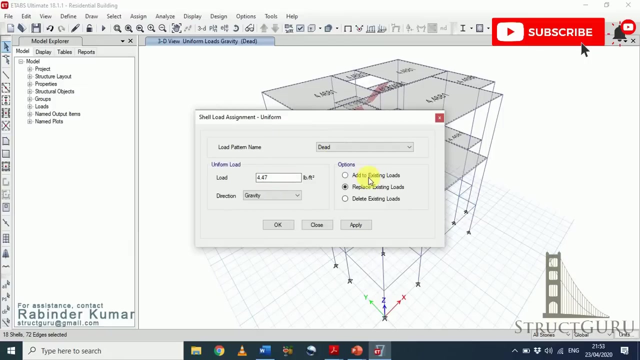 menu. in order to assign the load, you have to select the object first. for selecting the object, go to the select menu. object type: floors- select floors- click flows. go to the assign menu shell loads- click uniform. now we have already 4.47 earlier, so we have to add to. 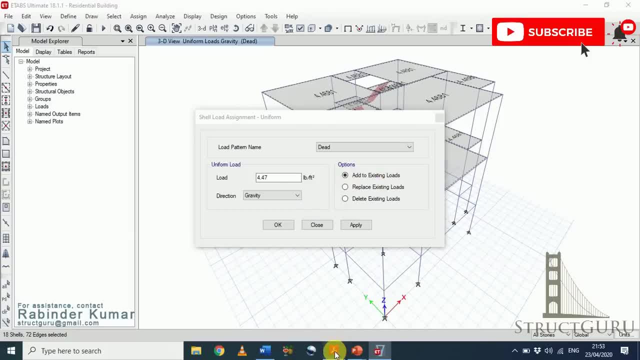 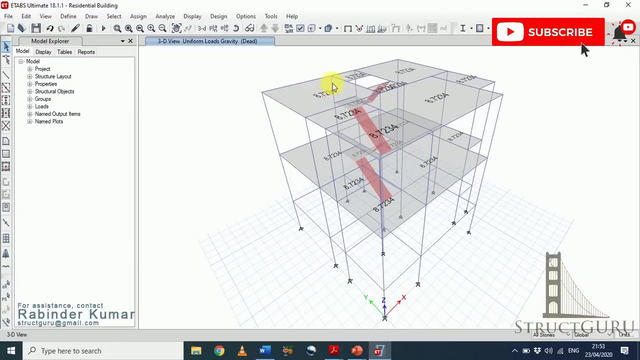 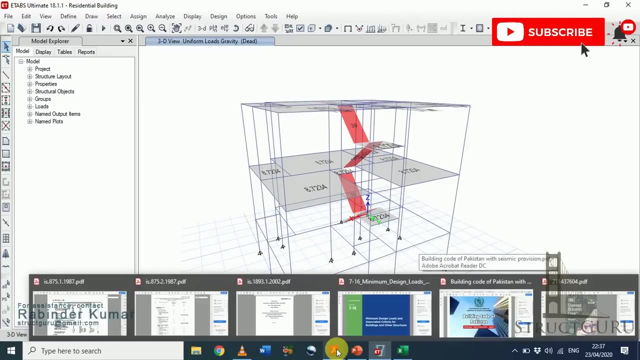 the existing load. so click add to the existing load and the value of load was 0.2, again 4.255. so it So ETAPS by default added the previous value and the current value which we have entered. In similar way, let's refer to ASCE code in order to see minimum design loads, which are 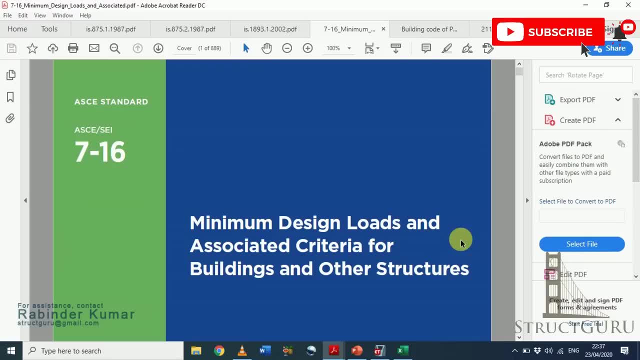 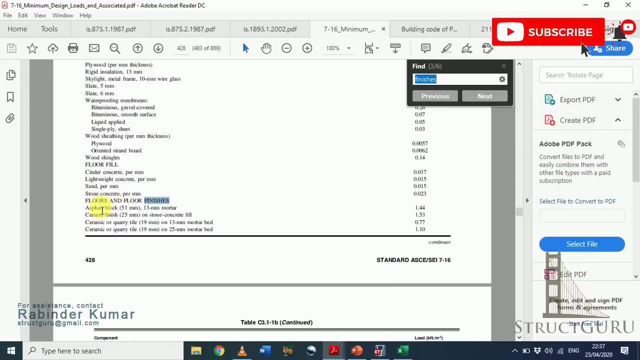 associated with buildings and other structures, Since we are designing residential building. so go and find the weight of finishes. Type keyword finishes. click several times as you can see. the load for floor finishes is written here: cement finish, which is 1.53 ceramit. 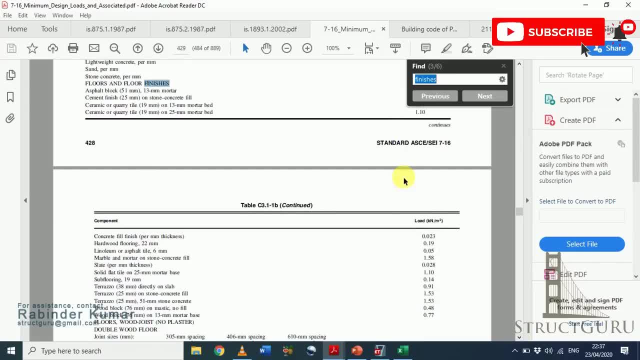 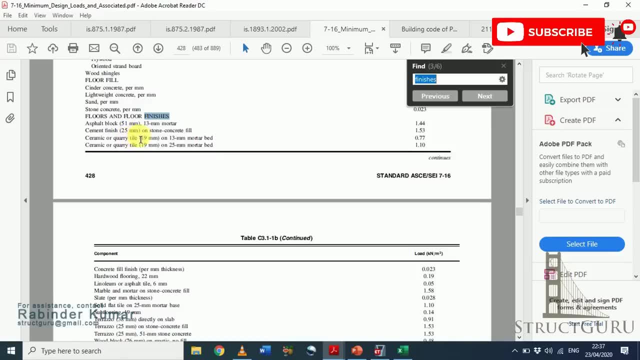 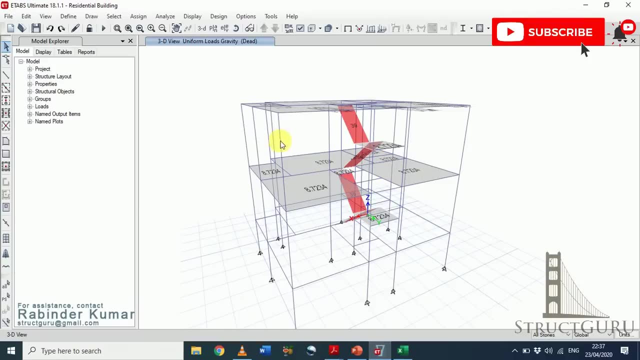 In this way. you have to choose the value from this code book. For example, I am choosing cement finish of 1.53.. 25 mm, which is 2.5 cm, it is 1.53.. So again you have to go to your ETAP model. select for the object type, choose all the. 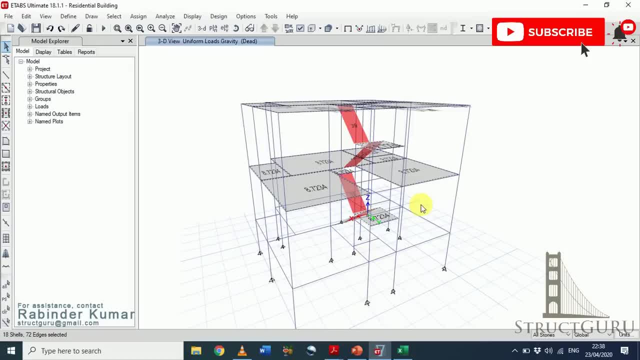 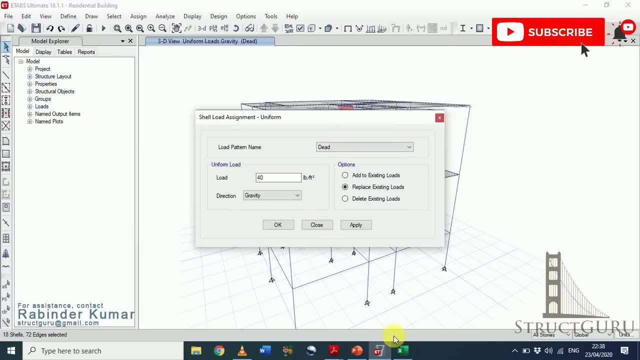 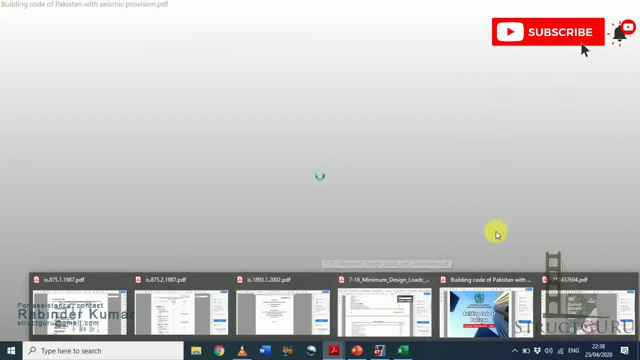 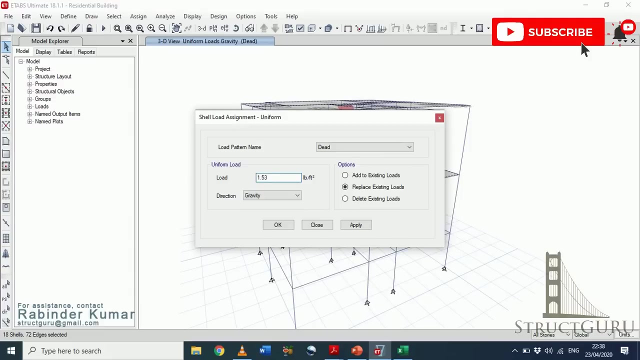 floor areas. go to assign menu shell loads, uniform loads. So the value was 1.53.. Okay, Value was 1.53 in the category of dead load. So 1.53 value was in kilo Newton per meter square. but we have to put the value in pound. 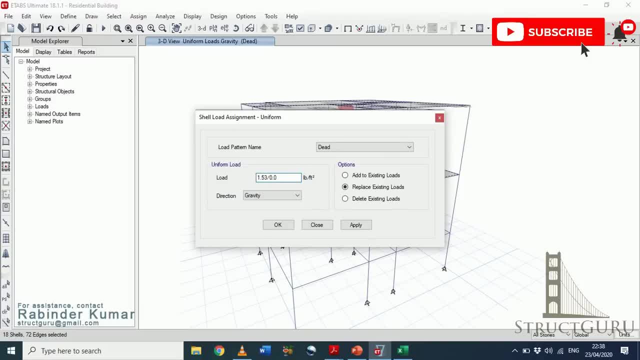 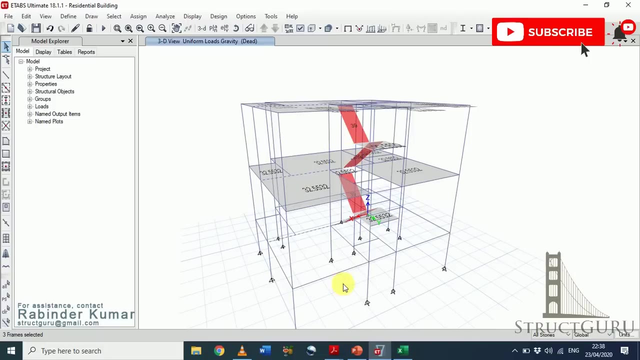 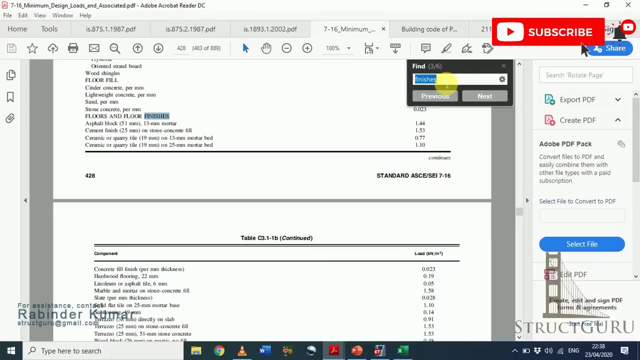 of it square. So divide this value by 0.047.. So it comes out to be 32.55.. Click okay. So in this way we can Apply the dead load. Similarly, you need to search out for live loads. refer to the code book again. 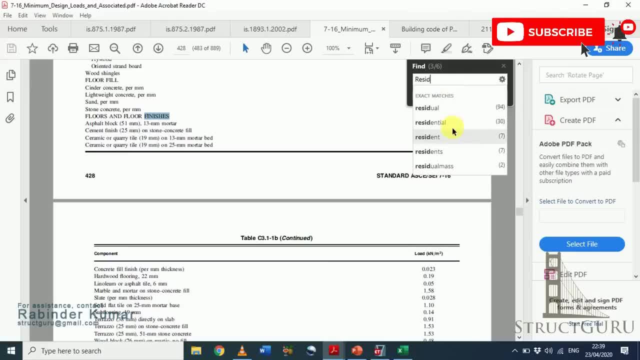 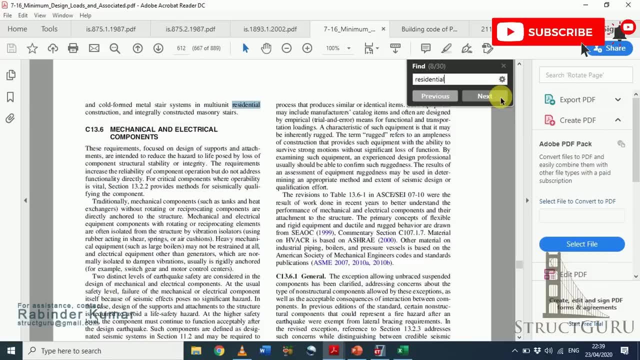 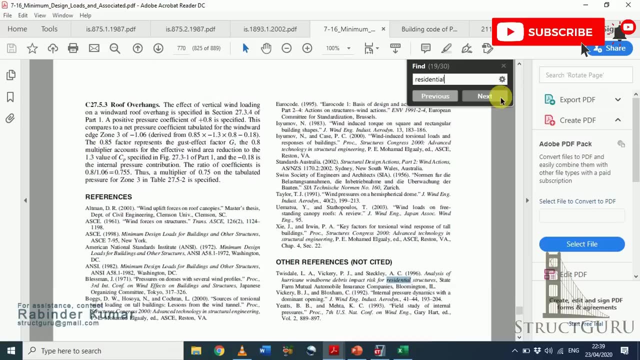 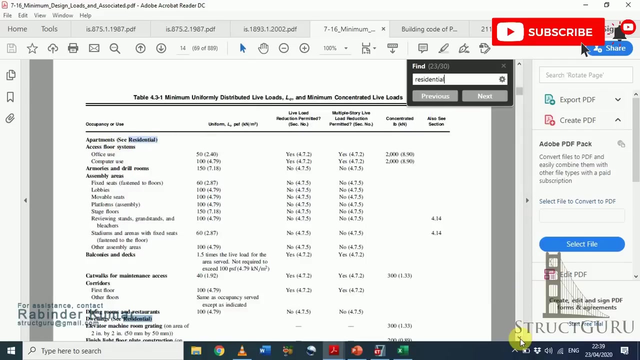 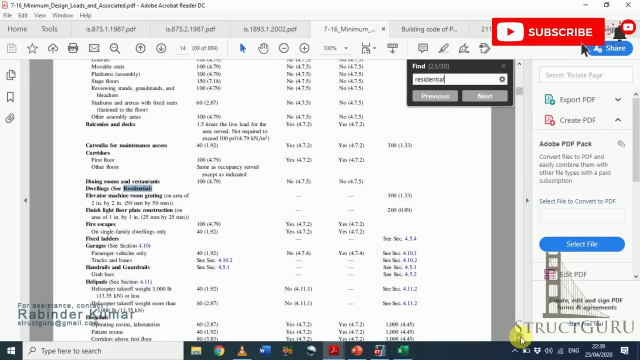 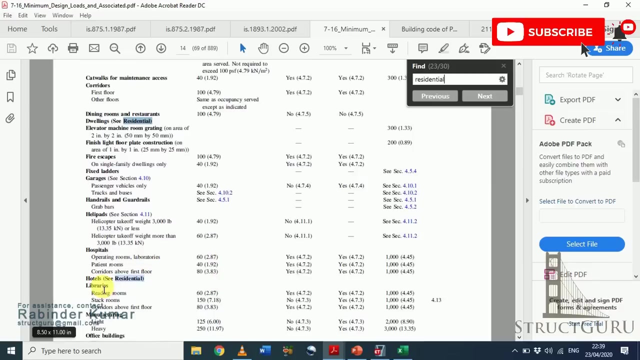 And type residential. Click next. Okay, Okay, See apartment. See residential. So various occupancy uses are written here. if you are designing office building, So you need to refer to this code book in order to see minimum design load. See for hospitals: the various loads are written for hotels, libraries. since we are designing 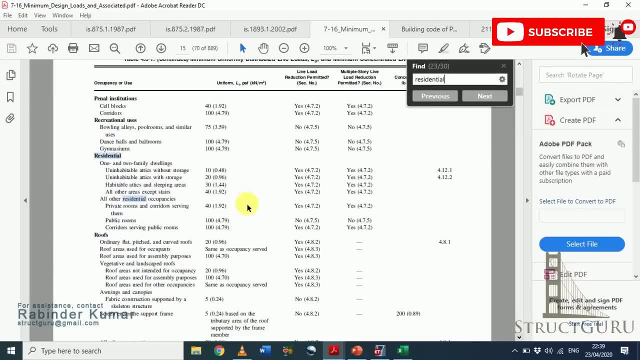 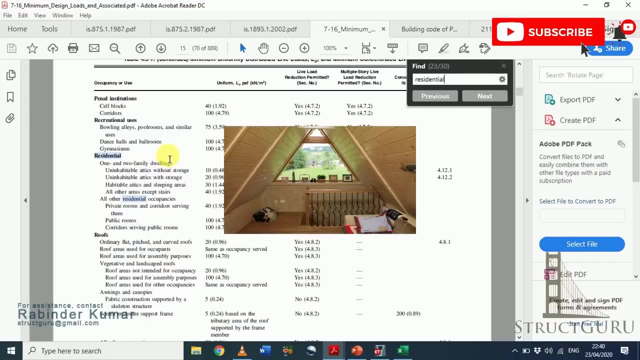 a residential building. So we have to look for residential. So uninhabitable attics without storage, And we'll Okay. So uninhabitable attics without storage. As you can see in this picture, there is a page screw. So if it is uninhabitable, so the loads are 10.. 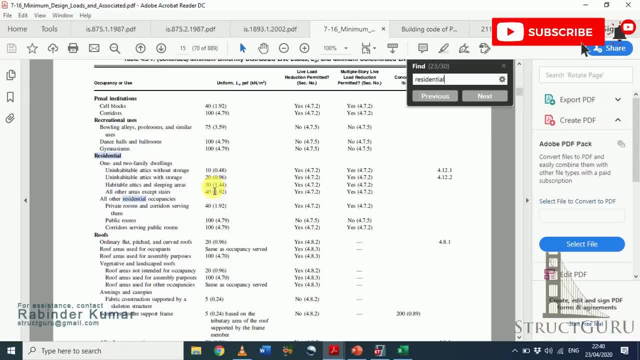 If it is habitable. so the load could be taken as 30. So all other areas except stairs- Again we have to choose. a similar value was written in IS code. All other residential occupancy, Private private rooms and corridors serving them- again we have to choose 40 for these categories. 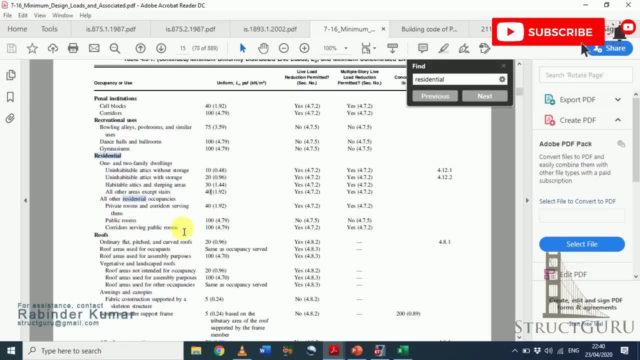 for public rooms we have to choose 100 PSF. for roof we have to choose 20 PSF, because we don't have lot of movement of people and objects there. so that's why the load value is reduced to half compared to the loads at other floor levels. so in this way again go. 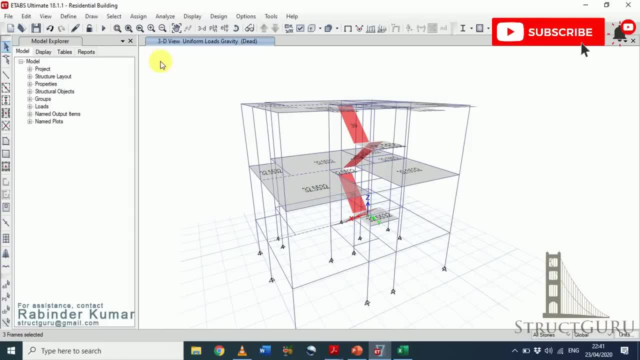 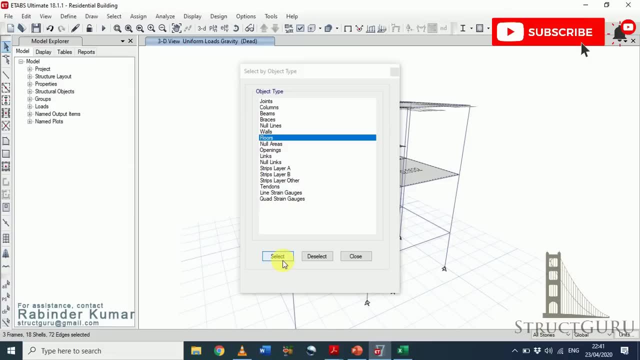 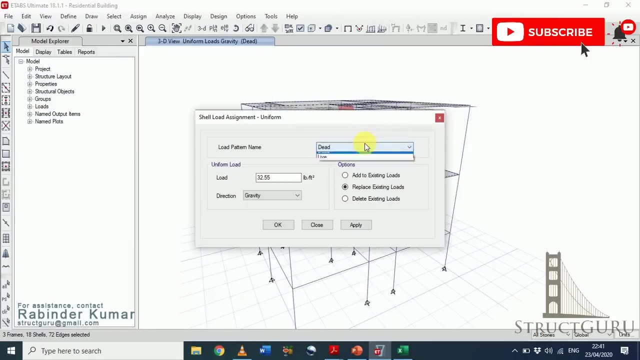 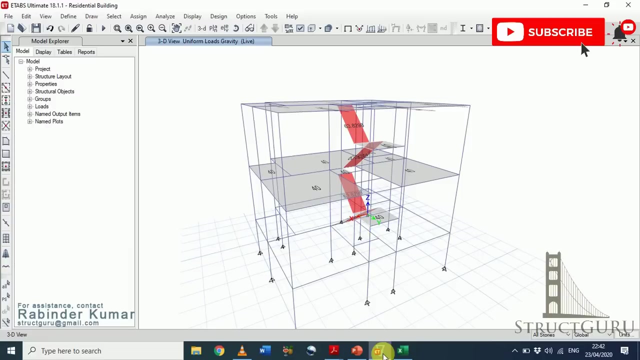 to your ETA model. you have to select all the objects. go to assign menu, shell loads, uniform loads. in the category of live loads you have to apply 40, click OK. so till now we have done with IS code and American code. now let's so, let's refer to. 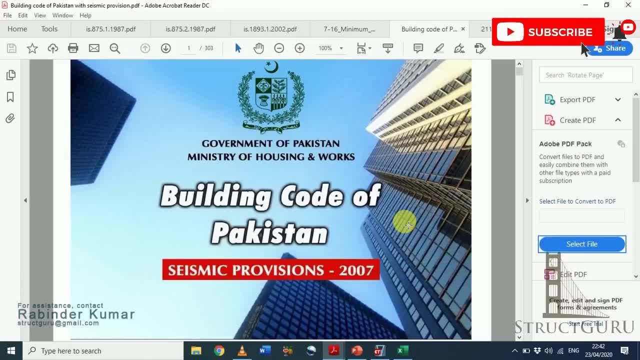 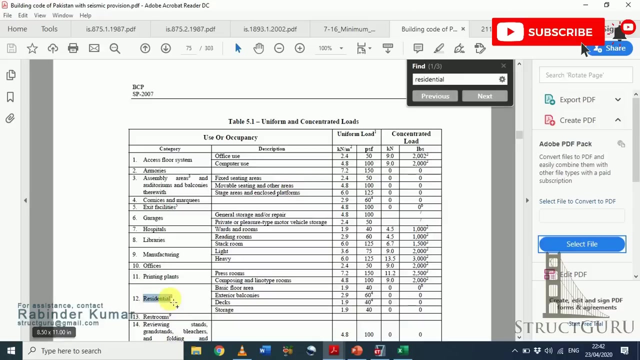 the Pakistan building codes to see what are the minimum design loads and given in the Pakistan code. so let's look for the live loads. so since again we are going to type residential: residential for basic floor area, we have to choose. 40 PSF for balconies, we have to choose. 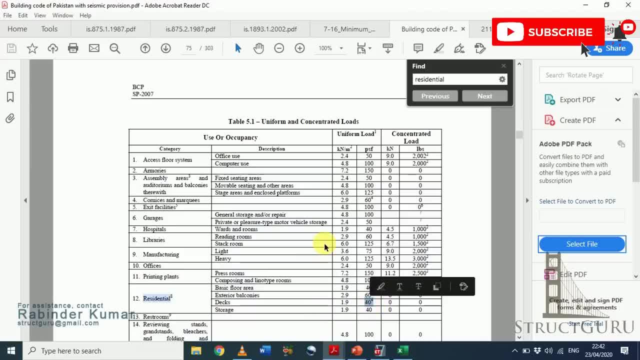 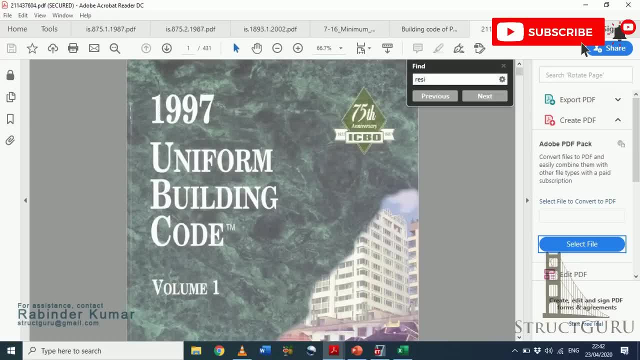 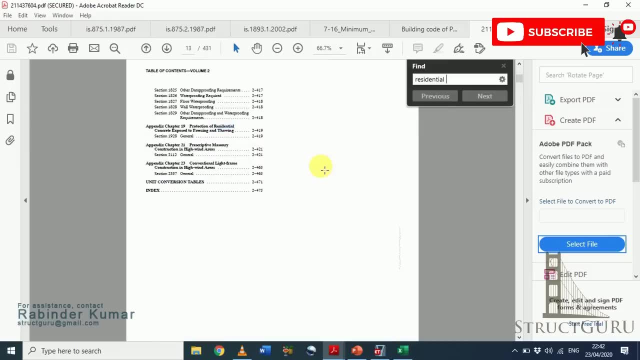 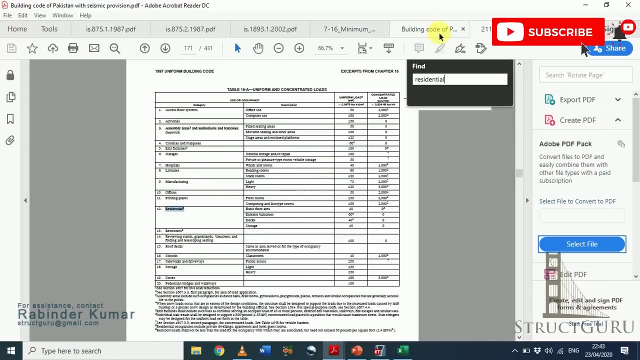 60 for decks storage, we have to choose 40 PSF for live loads. similarly for UBC code. if you refer to UBC code, the values will be same as given in Pakistan building codes. so let's see, if you refer to UBC, code for Pakistan is almost identical. values are almost identical as you can. 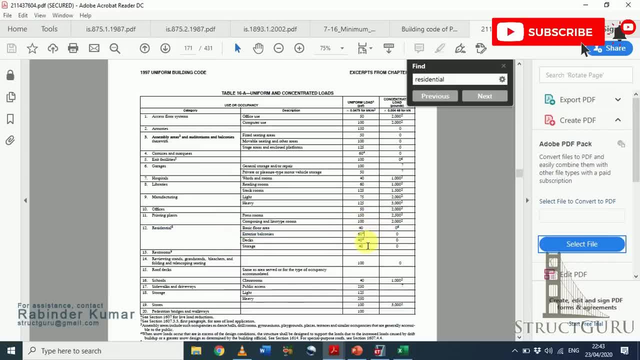 see for residential area. so it is given 40,, 60, 60 only the table is reproduced in other format, otherwise the load values are same. that's why I told you earlier the provision of building code of Pakistan are compatible with uniform building code. 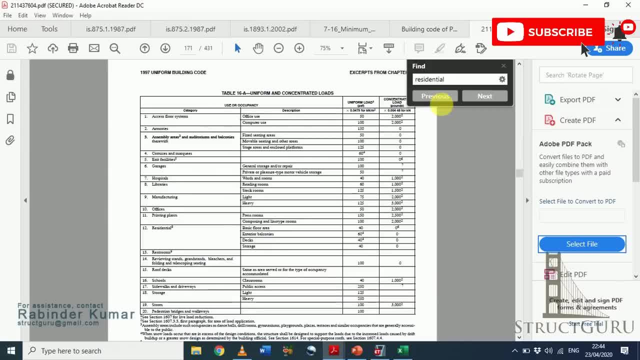 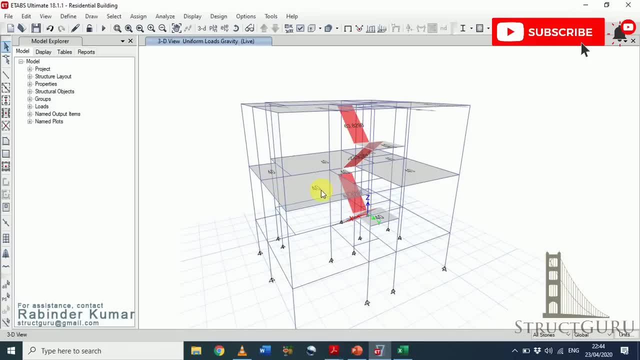 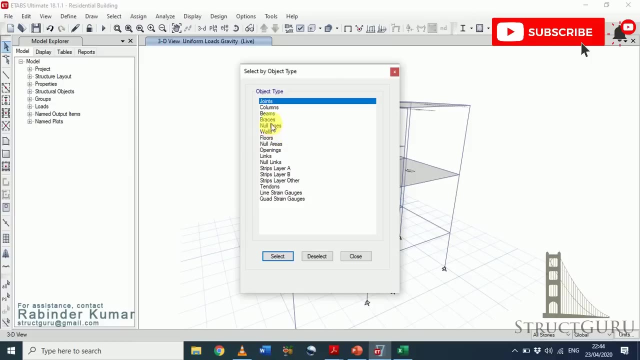 building code 1997. so in this way we can choose the values of dead loads and live loads. we can put it in our model. so, as I said, we will use ASC code values in our in our model. so go to again. select object type. select all floor areas. 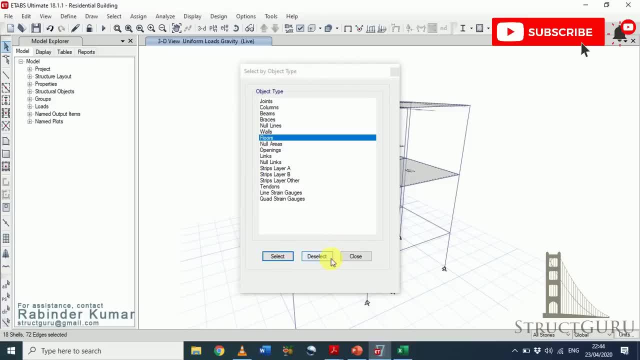 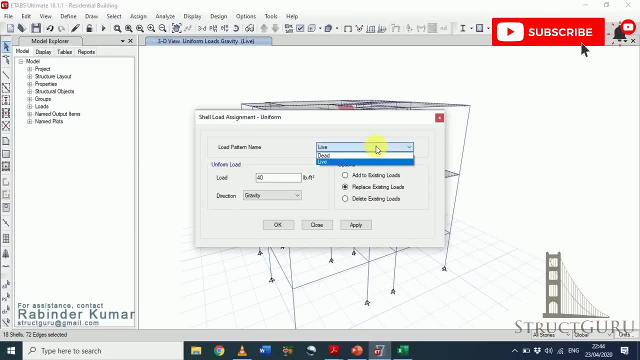 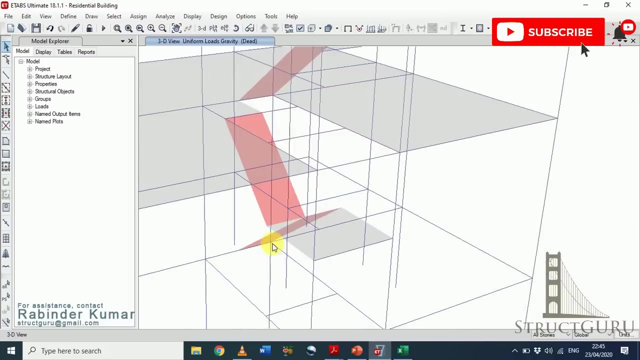 go to sign menu. shell loads the uniform loads. as we have seen from ASC code, the values for dead load comes out to be 33-pound, perfect square, so click OK. similarly, we have to do the same for staircases: select shredder. we are going to do it, so click ok. now we have the same values for the managers. 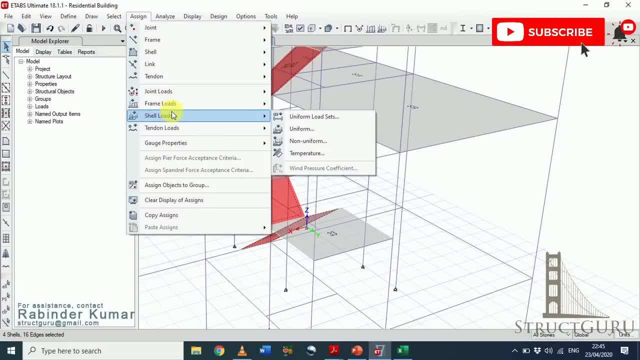 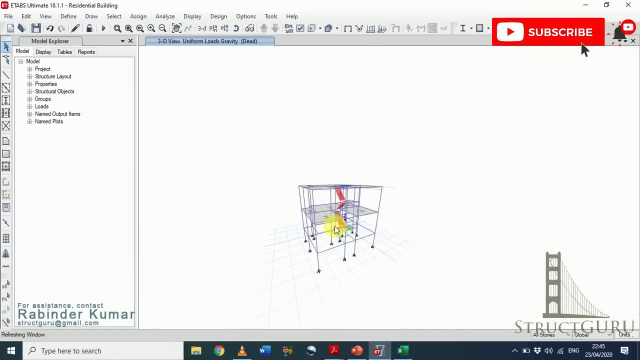 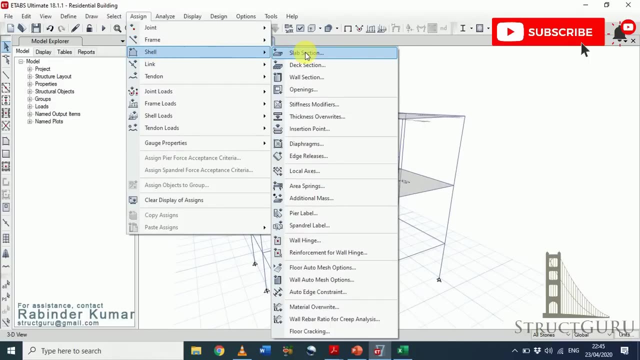 as we have seen from ASC code values for dead loads comes out to be 33 pounds, perfect square. so click, okay. similarly, we have to do the same for staircases like: so we assign shell loads, uniform 33. okay, now we have to assign live loads. assign shell loads. 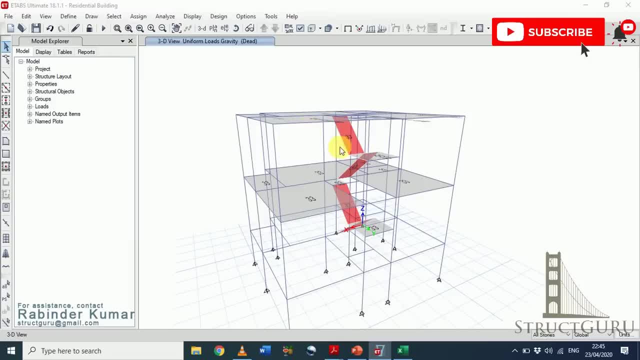 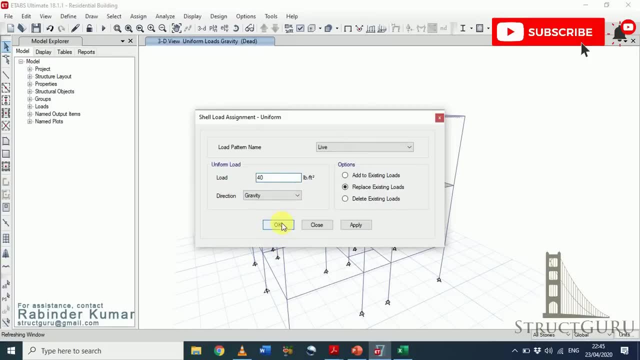 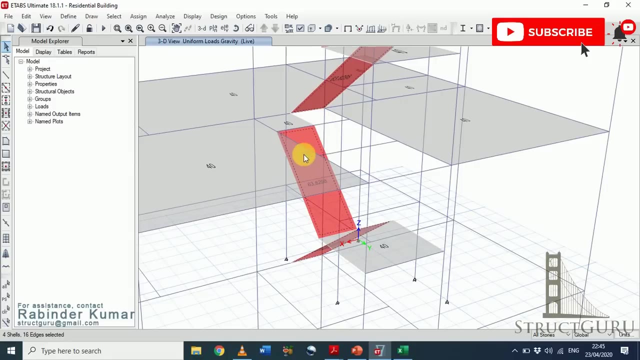 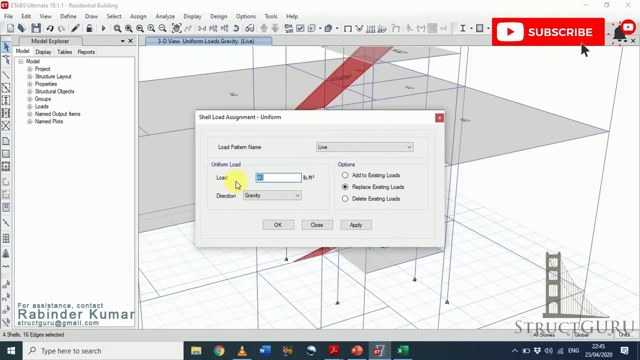 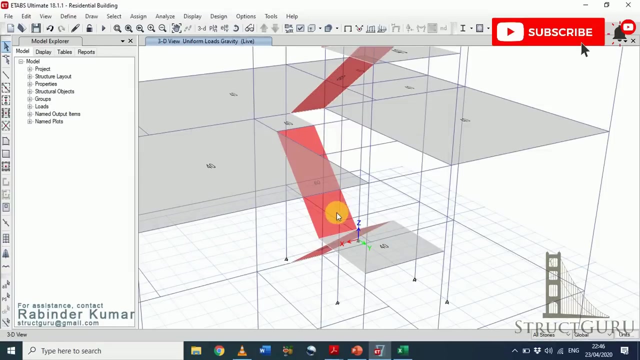 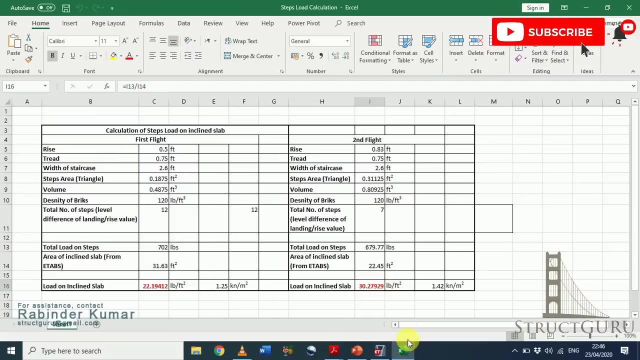 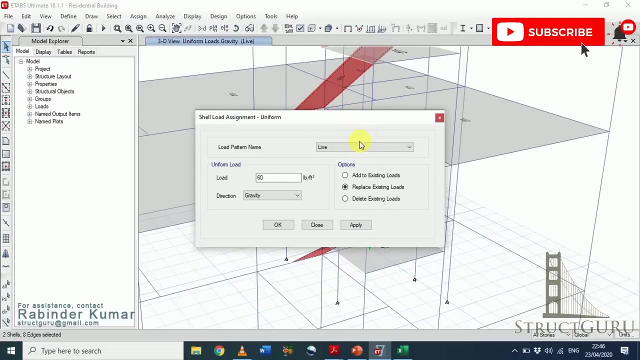 assign shell loads: uniform. choose live load from the down list type 40 and click OK. choose the staircase area. go to assign menu shell load: uniform load. so the live load was 60. add the dead loads on the staircase. select the first slide. go to assign menu shell loads: uniform. choose the dead. 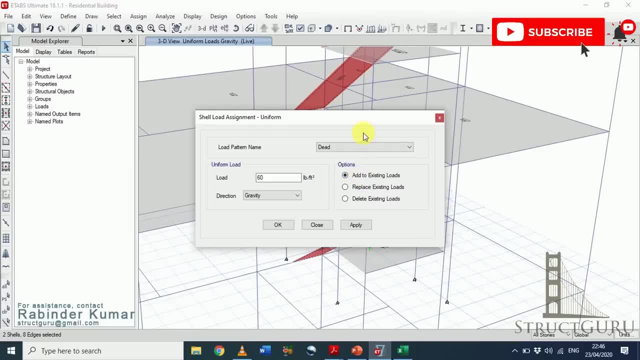 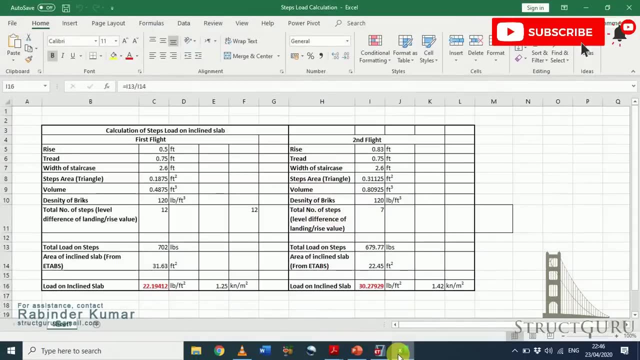 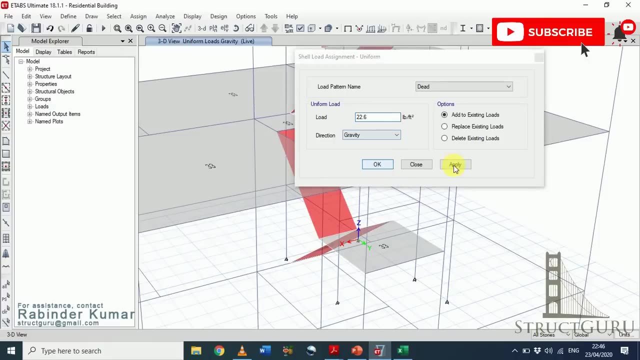 load click add to existing load because we have to add �� time الشARE surrounding edge to Not according to BTI step loads into the existing value of dead load which was 33 so the step load for first flight is 22.6 click OK close now select second flight go to sign 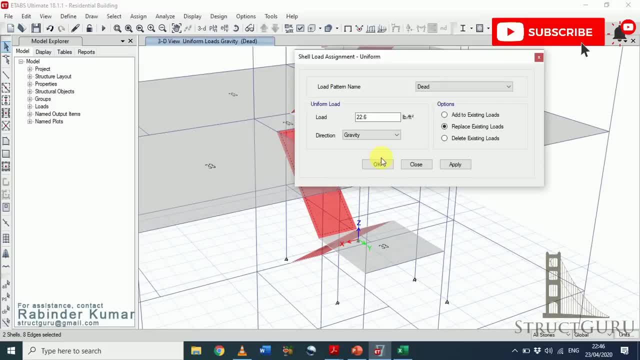 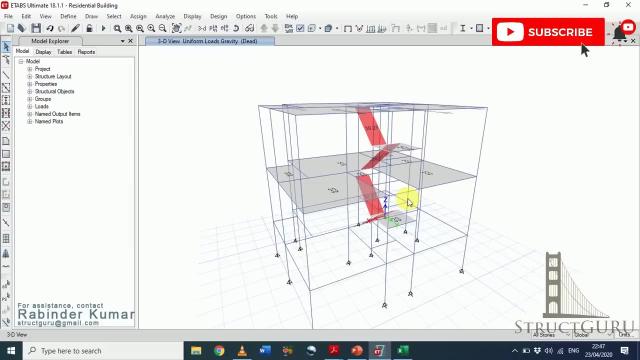 menu share loads: uniform 30.27- 30.27. click OK, as we are done with dead loads and live loads, now we have to assign wall loads. in order to assign the wall load, as we can see, the height of our floor is 12 feet and we have kept the 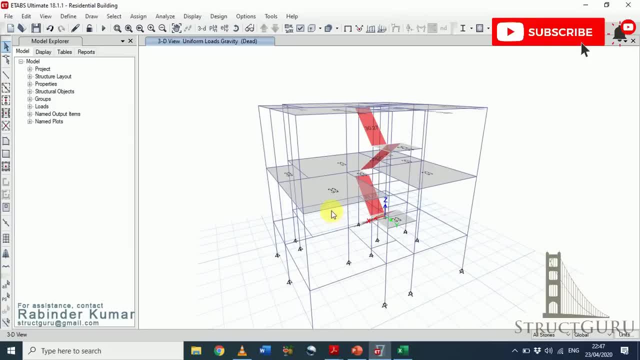 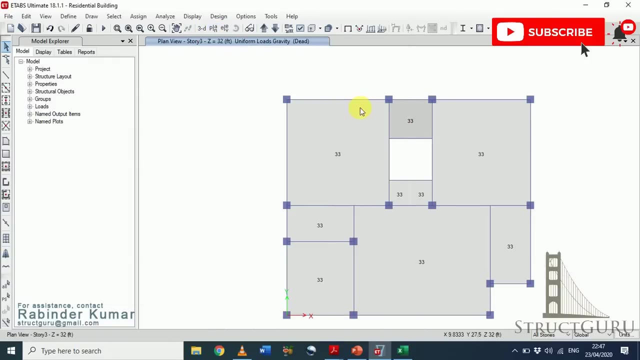 depth of beam as 2 feet. so 6 inches will be in the slip, so the total height for wall will be 10.5 feet. go to the plan mode. so our exterior walls are of 9 inches dimension and our interior walls are of 6 inches dimension and height of the 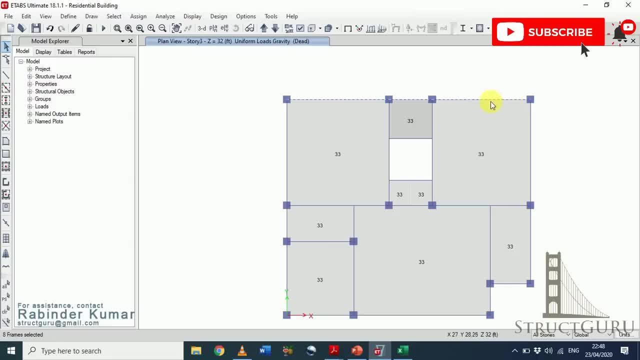 wall is 10.5 feet, I will centre location and move to side. so now our interior walls have a lot of beams, but we have to select some of them because we have to use these. so in this video i will show how to aíts fit, how to assign these. the 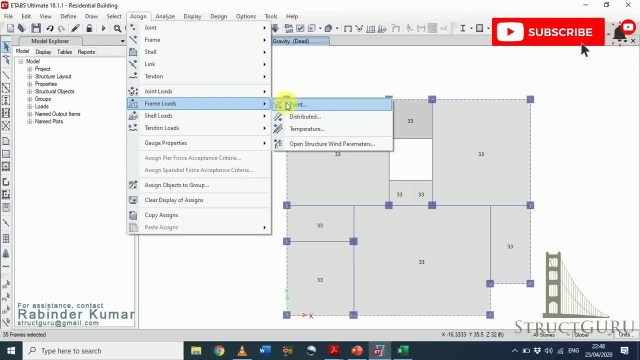 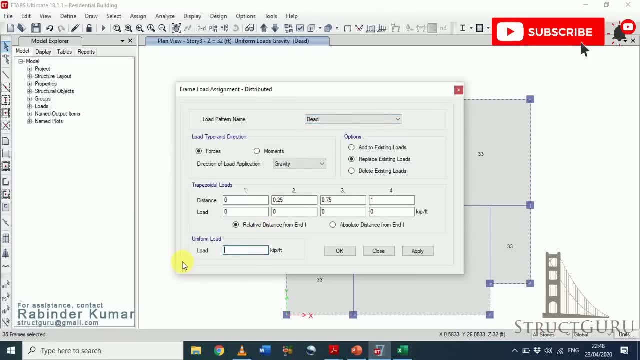 frameloads. first, select all the exterior walls, exterior beams. wall load is also in the category of dead loads. so how to calculate the wall, as we know that our height of wall is 10.5 feet multiplied by so density of wall, if i am considering concrete. 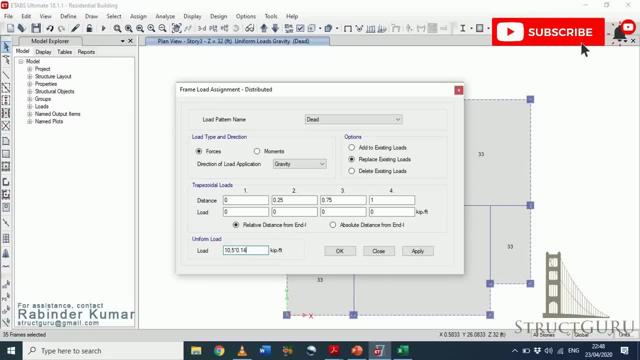 cement concrete blocks. so the density will be 0.45, 145 kip per feet cube, and our thickness of wall is 0.75 because our outer wall dimension is 9 inches. so exterior load of wall is 1.14. 1k. perfect, so click ok. 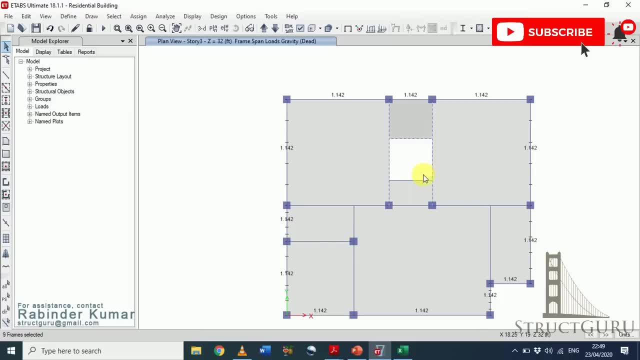 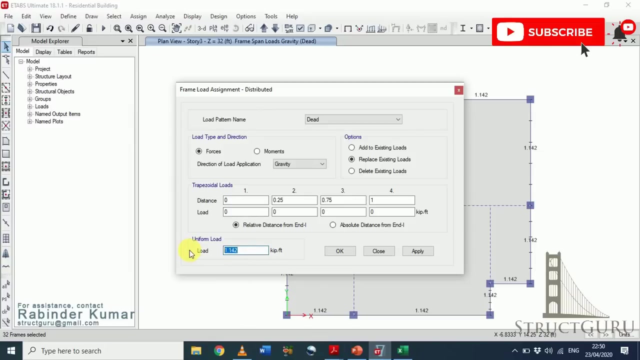 now choose the interior walls. so the thickness of our interior wall are 6 inches. so go to the frame line again, go to distributed load. now all the data will be same except the thickness of wall. so it will be 10.5 multiplied by 0.6, which is the width of wall multiplied by 0.145. this is the density of 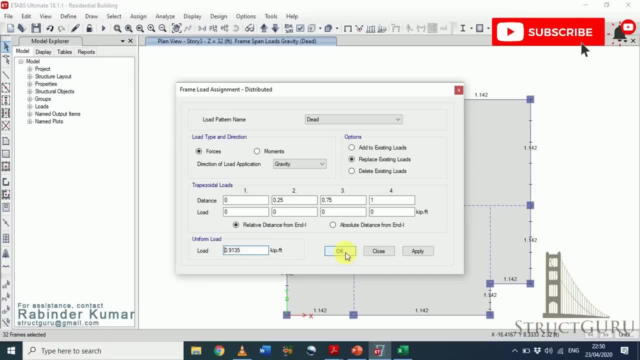 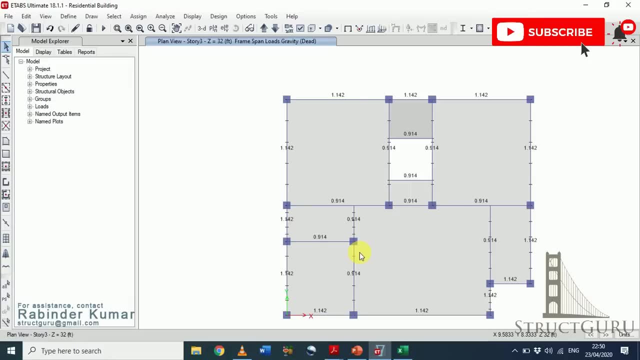 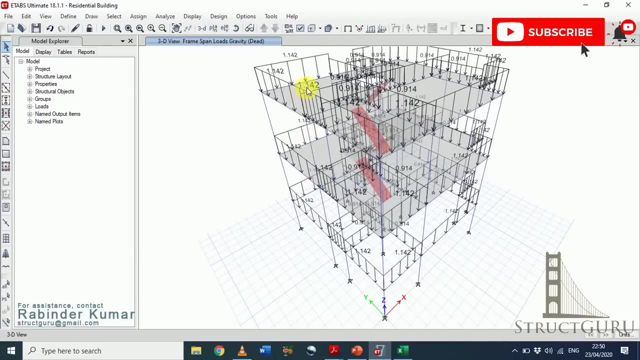 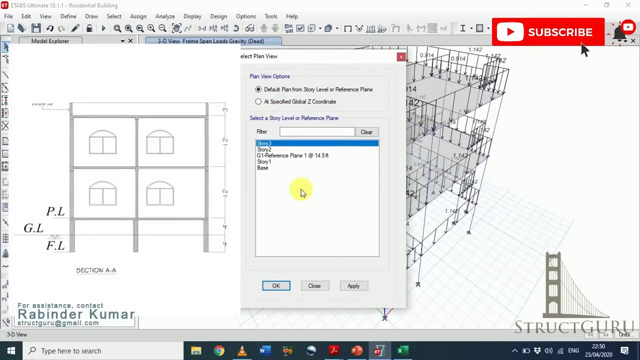 concrete, concrete block. click enter and click ok. so into the 3d mode. as you can see, we have successfully applied wall load. now we have to change the wall load at roof level because our parapet wall is of three feet. so go to the plan where view story 3, click. choose one story from drop down list. 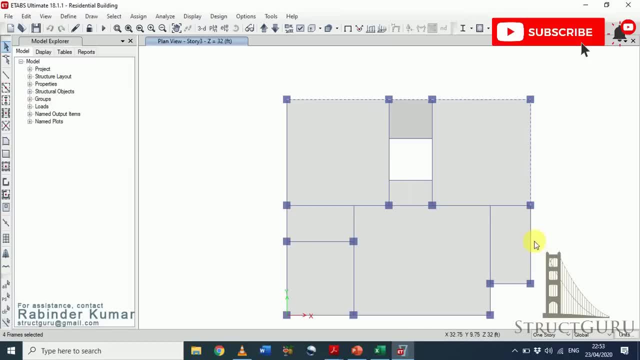 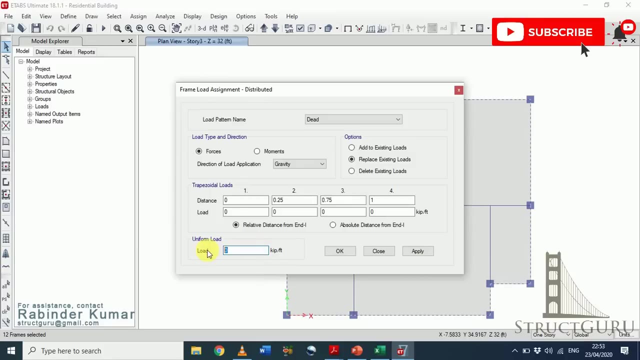 click the exterior wall, select assign frame line loads distributed. so now the wall loads will be: the height of wall is three feet multiplied by density of cement concrete block multiplied by thickness of wall, which is nine inches, 0.75 feet, 0.32 plus. click ok. so at the roof level there will not be any interior wall. 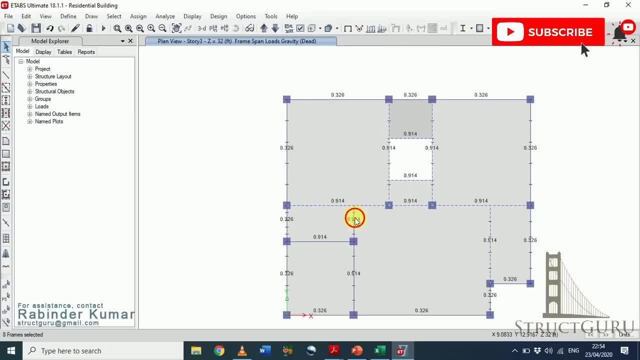 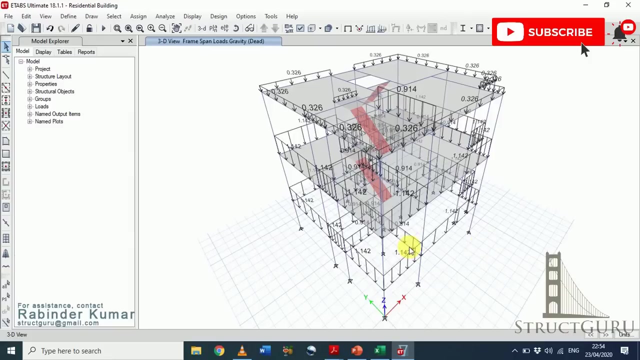 so select all the interior walls in order to remove the loads. go to assign menu: frame line loads, distributed load. click delete existing load. okay, switch on to 3d mode as we are done with assigning dead loads, live loads and frame line loads considering the kodal requirement be defined. 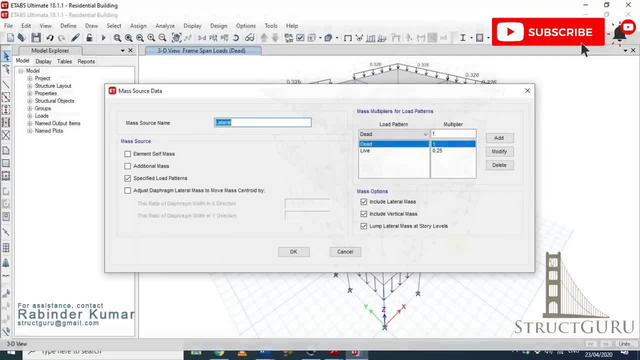 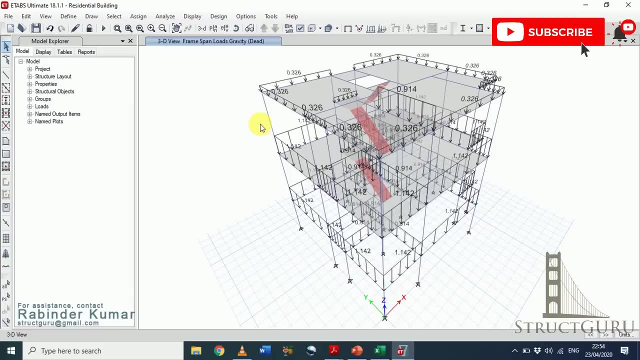 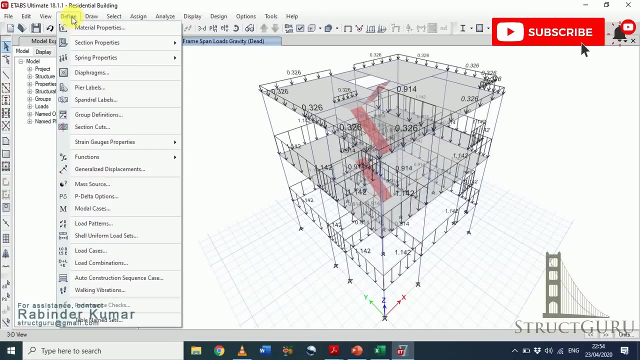 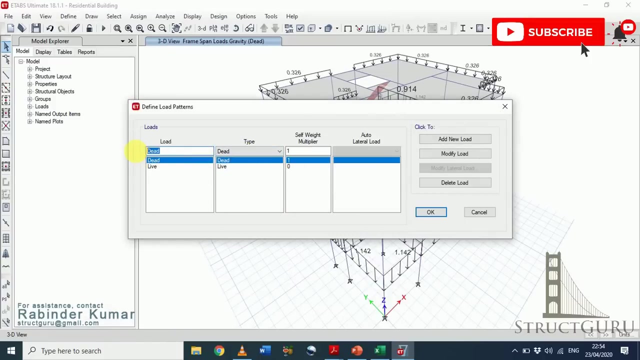 build. as we are done with assigning the gravity loads in our last tutorial, so we will move to assign the seismic loads. we will start with Indian standards. so how to apply the seismic loads? go to the define menu, choose load pattern. so seismic loads means they are the 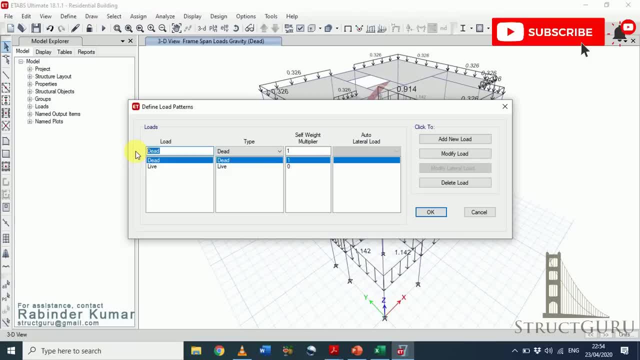 arctic loads either in X direction or Y direction, so we have to assign these bolts in both directions. so type EQ X: choose seismic. select is 1893 2016. click OK. similarly, earthquake in Y direction. type: seismic: similar code. add new. now we have to modify the parameters to modify. 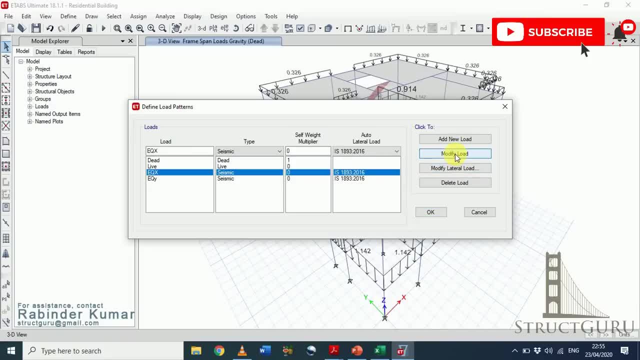 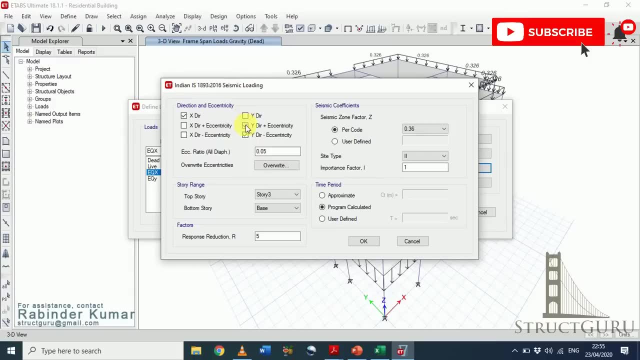 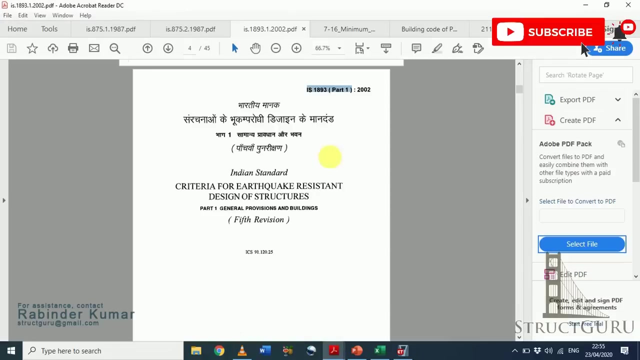 the parameters, click modify load, modify lateral loads and check all these parameters now from the code book. we have to define the zone factor, for example, if we are designing a building in a Bombay region, so go for Indian Standard 1893, part 1. so I have older version. 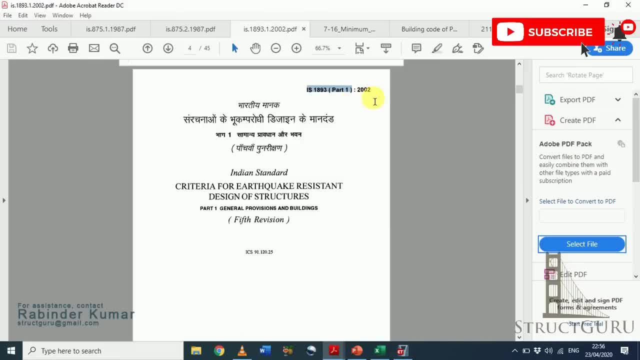 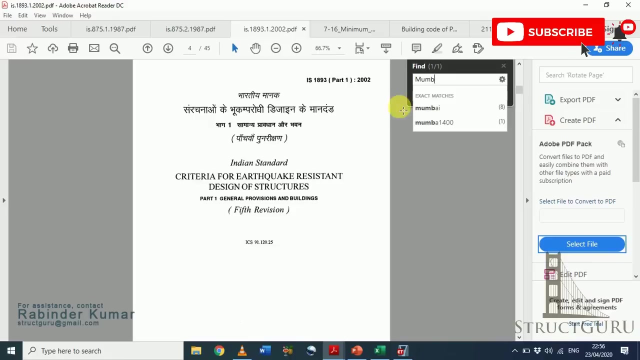 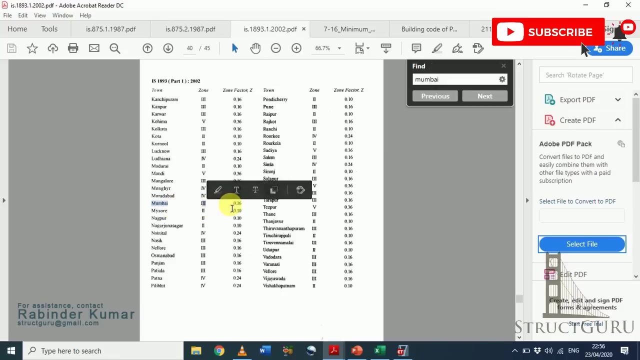 2002, but in ETABS we have selected 2016, so there will not be much difference. so if we are designing the building for Bombay region, how will we do? first, we have to define the zone factor. so type Bombay, type Bombay. so Mumbai is in zone 3 and the zone factor is 0.16. the value of Z is 0.16. 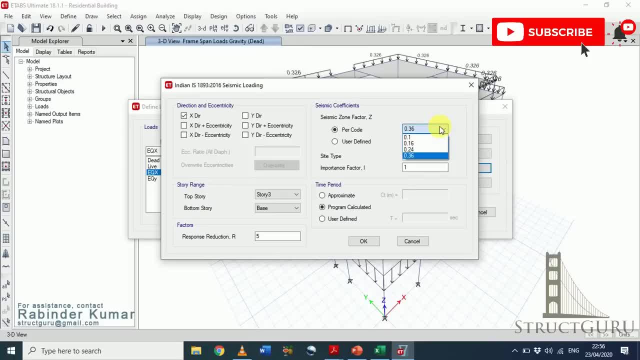 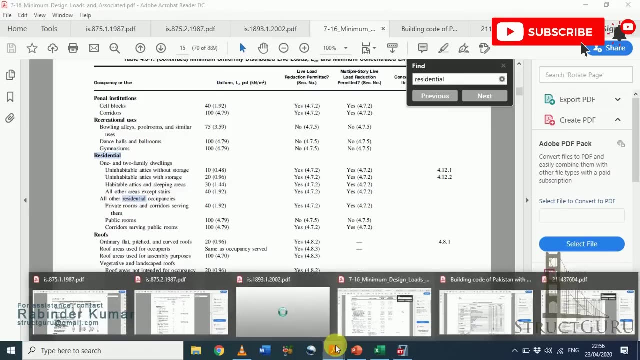 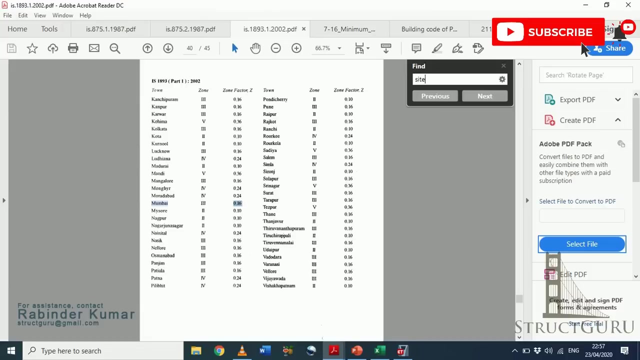 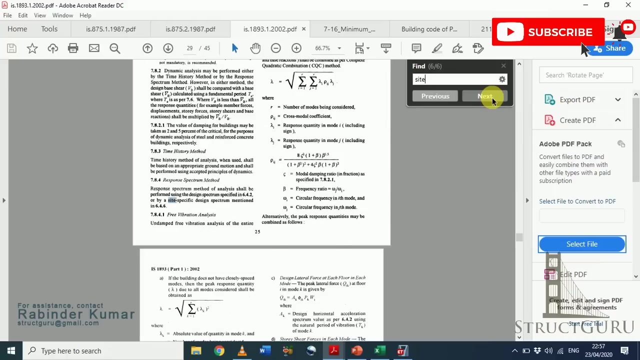 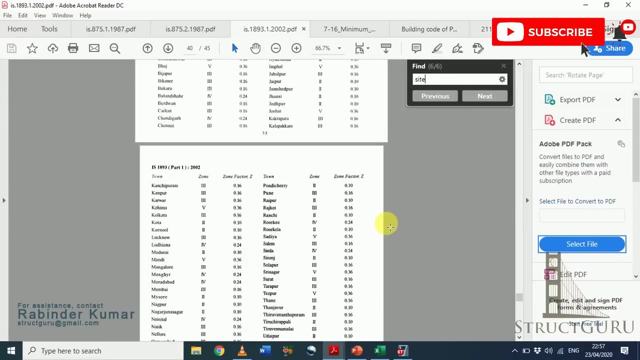 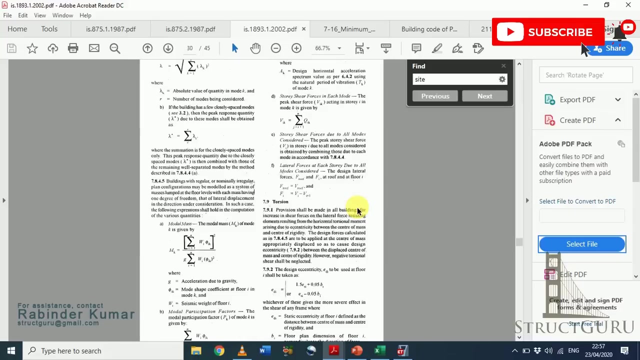 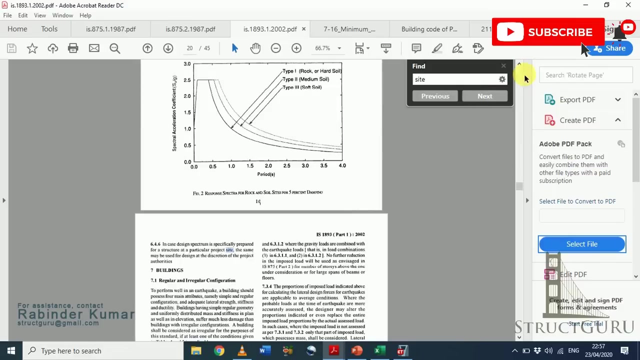 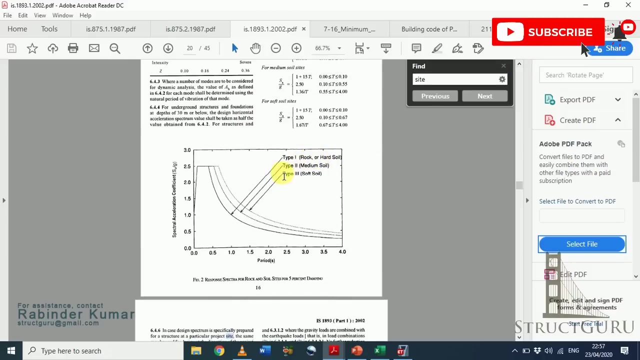 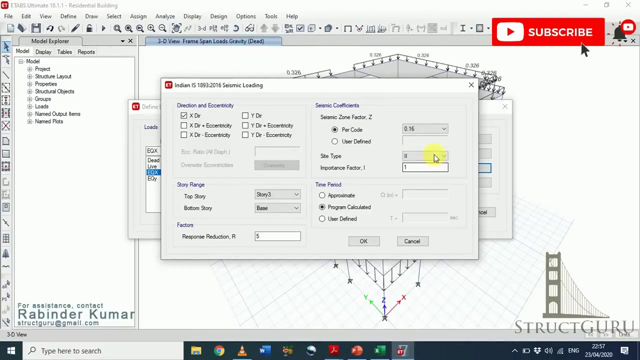 so go to ETABS model, select 0.16 site type. again go to the code book. again go to the code book, select site. select site or choose manually. or choose manually. yes, site type means weather. the soil type is rock or hard soil, so this data will be given to you from soil investigation. so, for example, I am 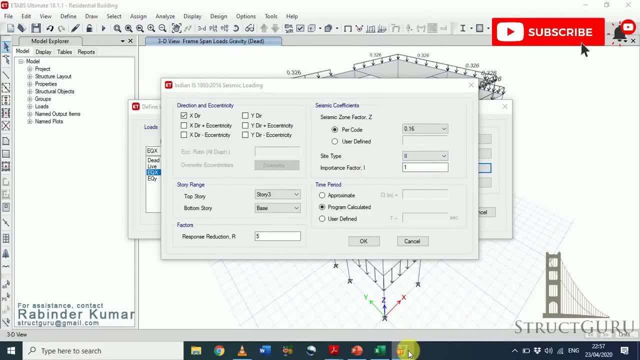 considering soil types. so importance factor. so important factors mean so important factor. so important factors mean so important factors. so important factors mean so important factors. and so if i pick soil type, Whether it is a residential building, school buildings, public offices, banks, hospitals, 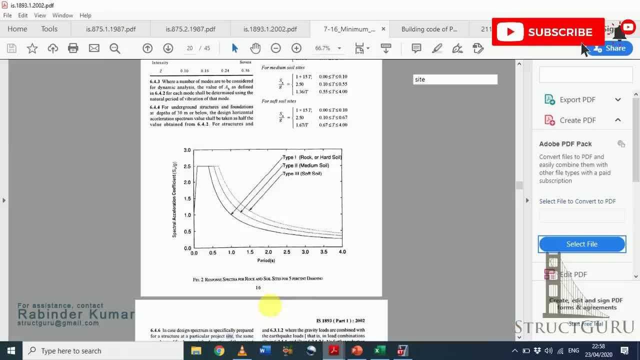 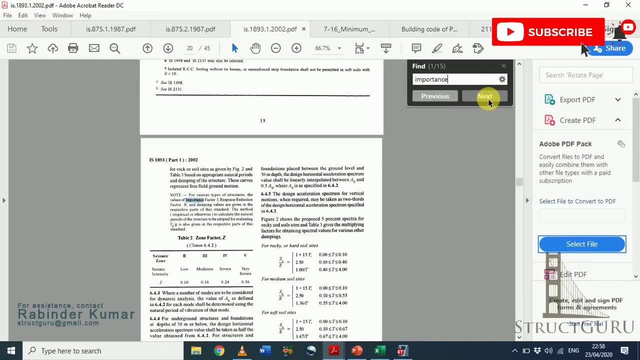 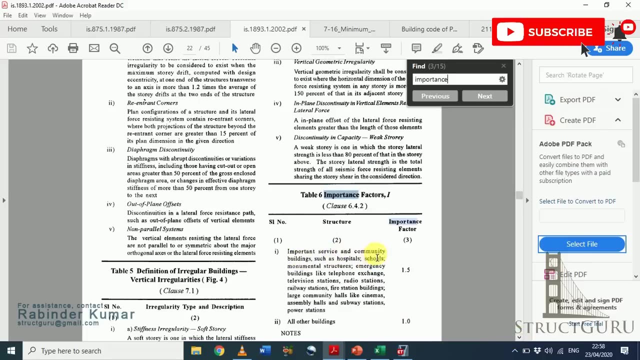 So in this way, the buildings are categorized based on their importance factor. In order to find the importance factor, just write importance and click next several times. So here you can read: important service and community building, such as hospital. our building is not hospital. our building is not a school building. 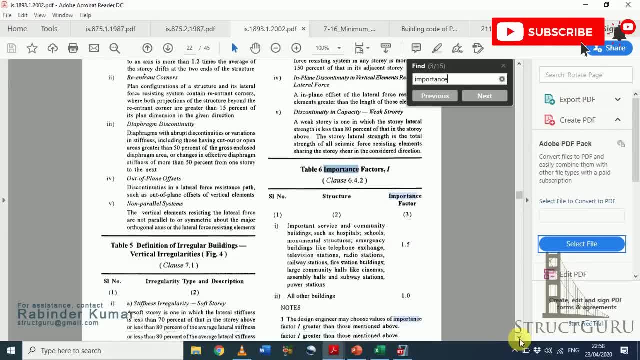 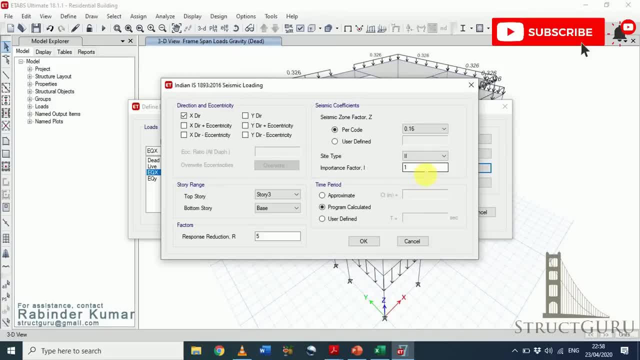 So for such cases we have to use 1.5, for all other buildings use 1.0. So our building lies in all other building category, so we will choose 1.. And now the response reduction factor. Again, the code has a structure. 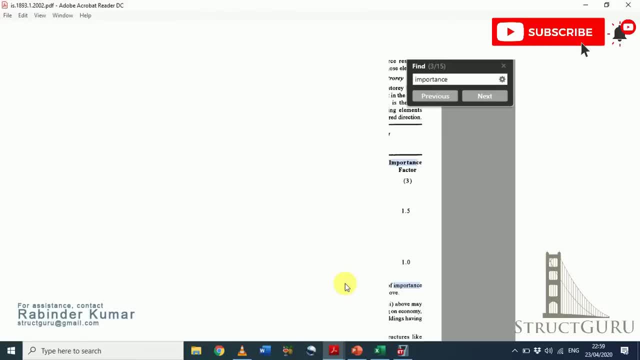 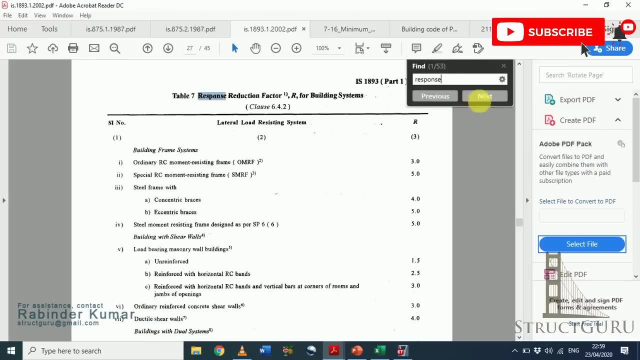 I have specified these values. Go to the code value again. type response. So first we have to define what type of building frame system is, Whether it is ordinary RC moment resisting frame or special RC moment resisting frame. In simple words, if I tell you, the difference between these two is of the shear reinforcement. 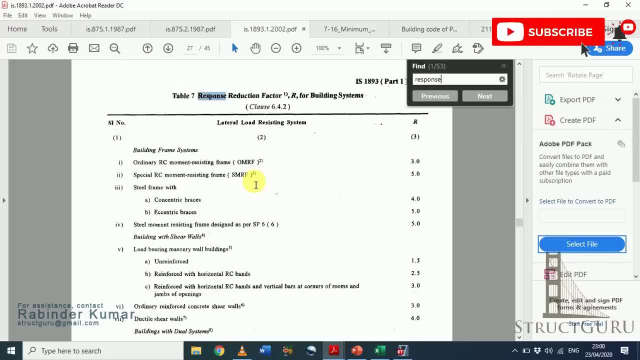 If the shear reinforcement is high, if the building is designed for high seismic zones, so we will go for special RC moment resisting frame. So for that the code suggests the value to take as 5.. For ordinary RC moment resisting frame, for example, if the building is to be designed. 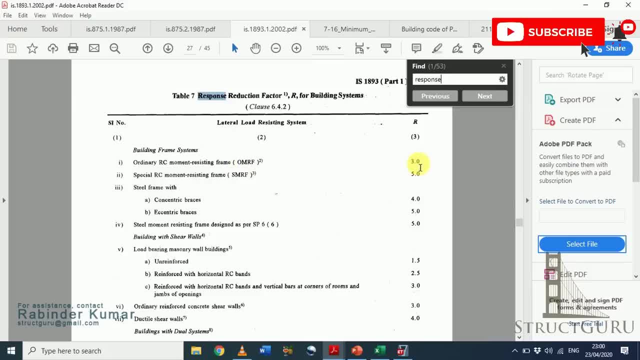 for low seismic regions, then we have to use reduction factor as 3.. So, as you can see, by default the value 5 is inserted here, Because each building is designed for low seismic regions, then we have to use reduction factor as 3.. So, as you can see, by default the value 5 is inserted here. 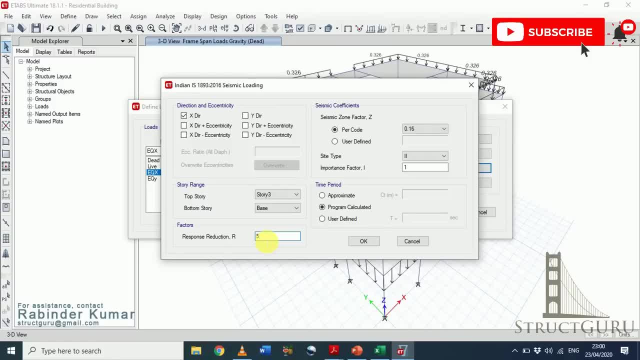 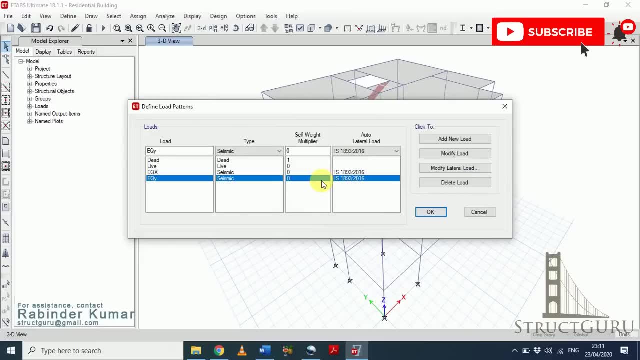 For any other KU station or any other RC được grant variants. consider: you are going to design special RCline cement energía as special RC moment resisting frame. so we are choosing 3 here. So in similar way you have to change the values in direct, it will. 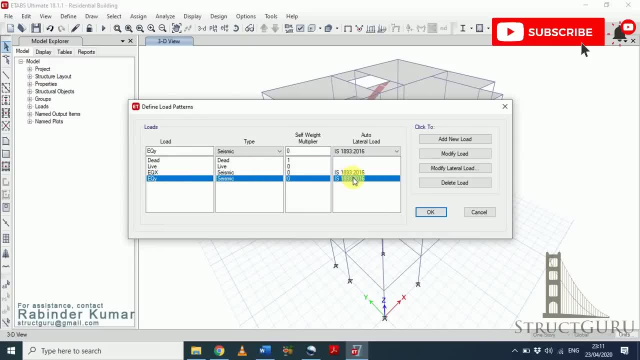 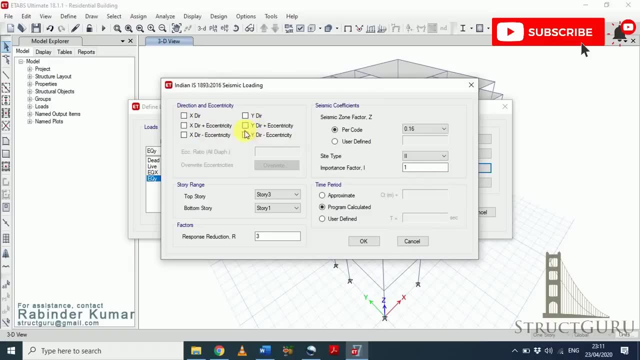 So to change the values in direct it will you have to click EQY, Click modify lateral load and you have to un check all these parameters. Check, LetsEít. Как Do Themyz interview From column to column, column section up to column to column. 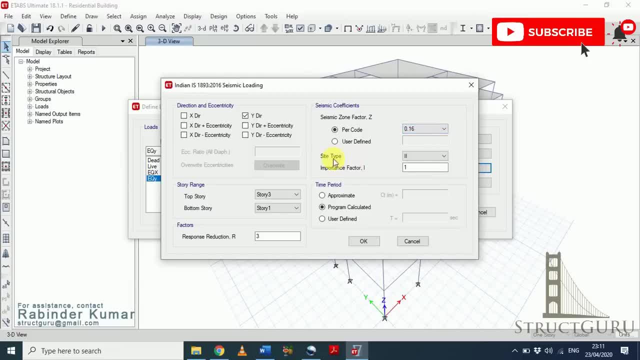 For y direction, As per the own sector, try to multiply by tick marketing c index With base rate for lowerскиmış that Ro good indicative parameters and never near以上 the electronic data base value one six. our site type we selected was two importance factor as we are dealing, 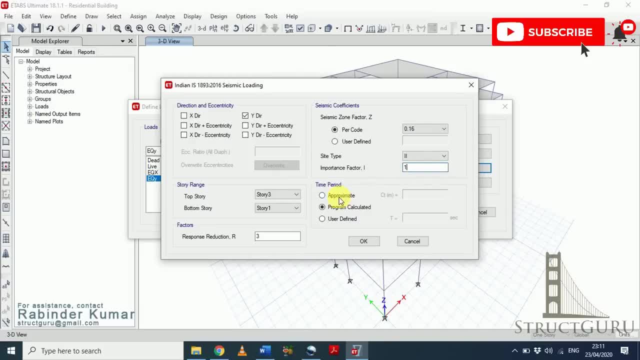 with residential buildings. importance factor is for for time period. I will always recommend you to go for program selected value. don't go for user define or approximate value because if you compare the value with manual calculations the values will be different, as the ETABs can see. the 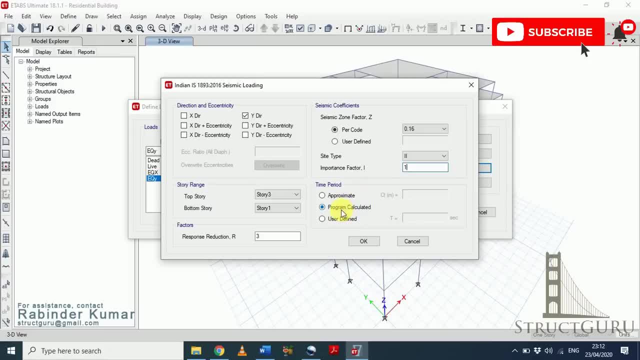 stiffness in the count as well. so always go for program calculated value. similarly, the story range. some users go from base to story 3 and some user go go from story 1 to story 3 because our base is embedded in the ground. so whether you choose from base or story 1, it is fine, so I will. I always choose from base to. 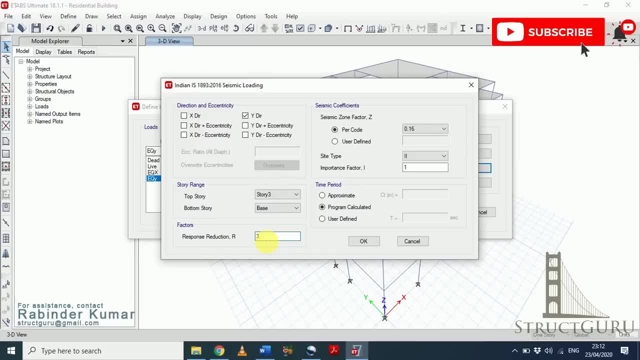 story 3 of a response reduction factor, as we saw from the code, value 3. so choose this value. now, what is the response reduction factor? let me define it. so it is the factor by which the actual base shear force is reduced. in simple words, it reduces the earthquake load which is encountered by the building, by the 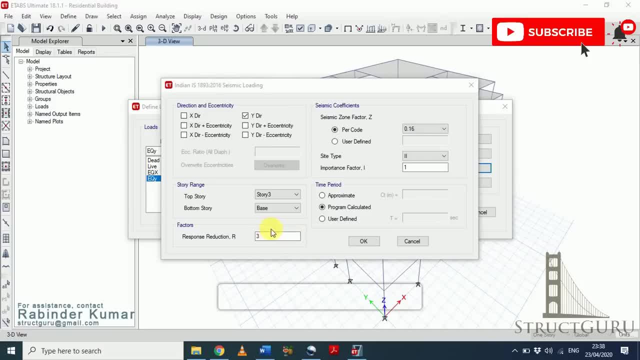 factor we input in this seismic coefficients. for example, if you have choosing response reduction factor 5 and the earthquake load is thousand units in actual, so this reduction factor reduces to one-fifth of the actual value and the building is designed to experience only 200 units of earthquake. now the question. 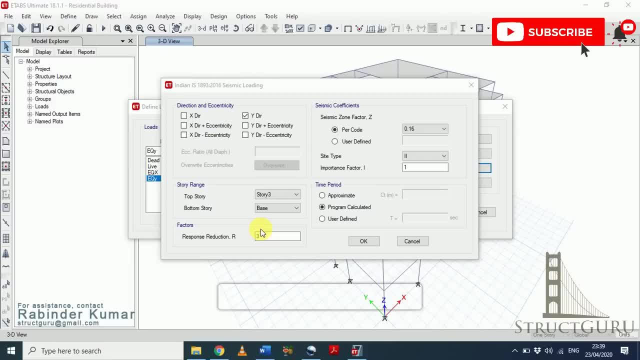 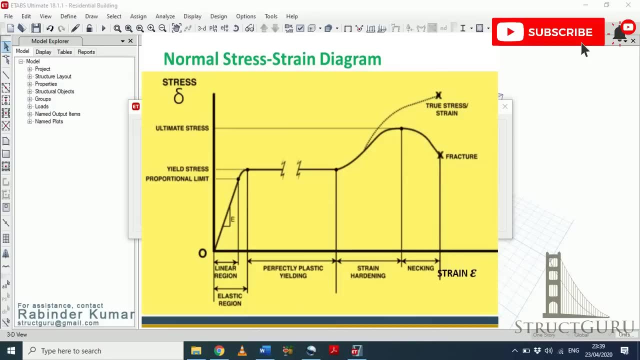 is why we do so, why we reduce it, as we know you can see from the strain stress diagram of a state. so, as we know, we always consider the properties of a material and linear elastic range and we always ignore the plastic strength of material. we always design our building considering the yield strength of. 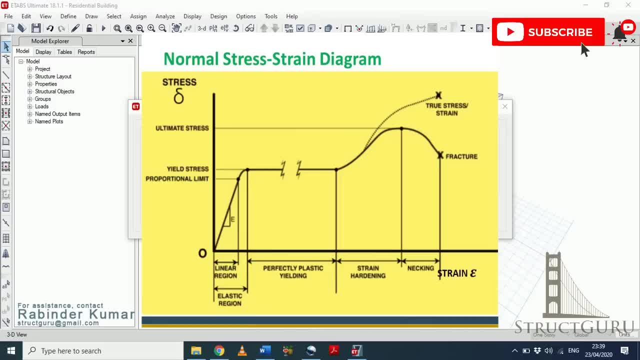 material but in actual the structure has capacity to take the load up to the strain hardening region. so that is why we reduce the actual base shear by certain values, because we know after yield point our structure has capacity to resist the earthquake and this makes our structure earthquake. 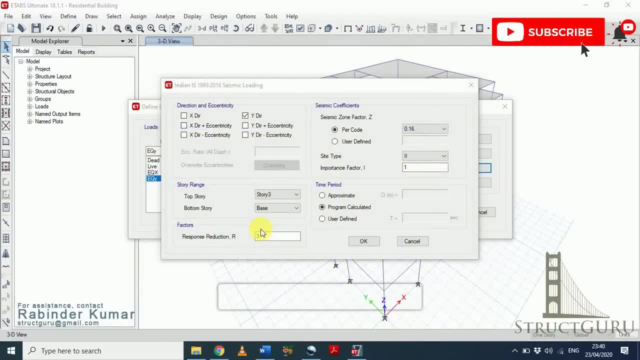 resistant. earthquake resistant structures means it can experience small cracks in the building or some building component may also collapse, but overall the structure will respond well against the earthquake. now if we say earthquake resistance, now the question is how we design earthquake proof structures so to do that, just type 1 in response, reduction factor input, but we don't go. 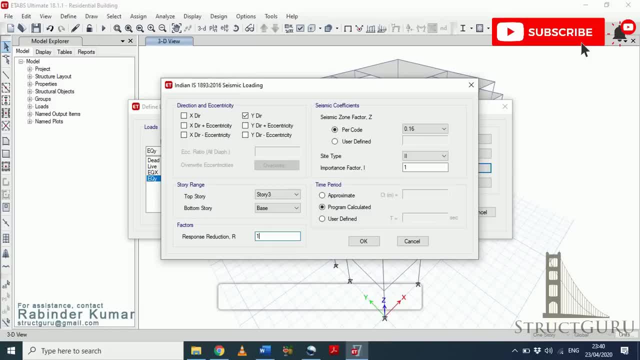 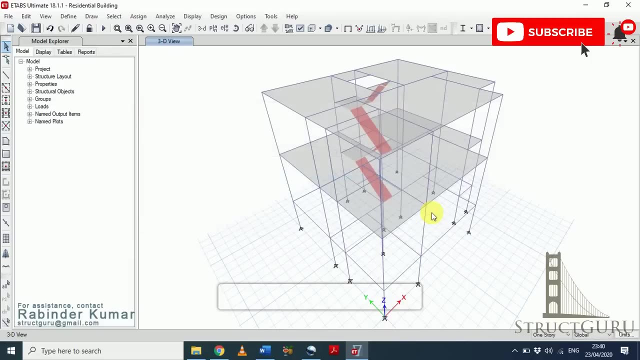 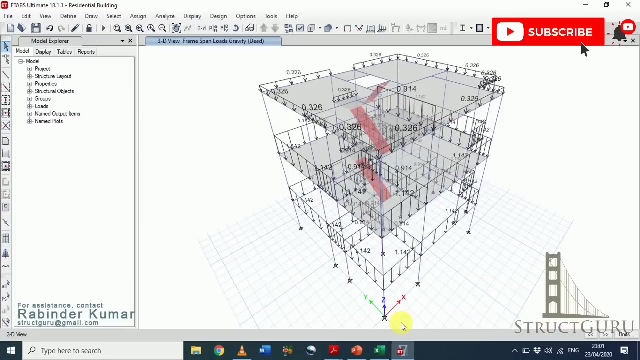 for this value, as it will give high reinforcement for our building and the structure will be uneconomical. so choose the value which is recommended by the code, click OK and okay. so we have successfully inserted all the parameters seismic coefficients using IS code. now I will refer to Pakistan building codes, but the problem is ETABS. 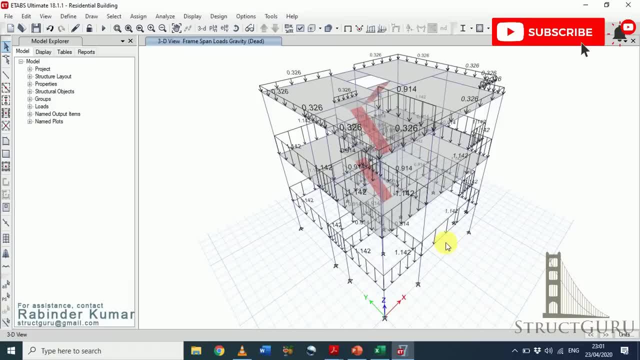 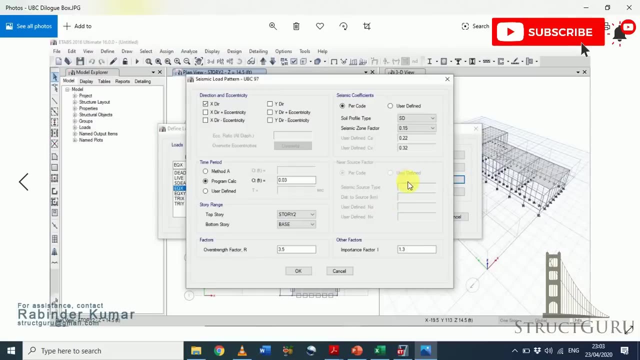 version does not support UBC code, so for those aspirants who use ETABS 2016. so first I will open a screenshot of seismic coefficients from ETABS 2016. so, as you can see in this picture, we have to define these parameters if we are 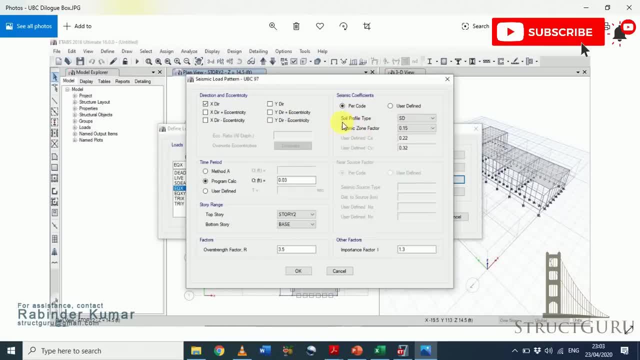 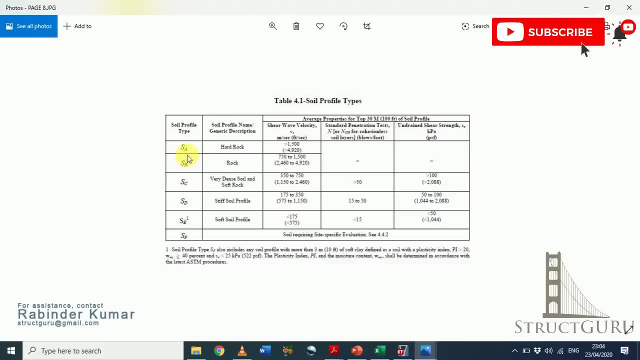 using UBC 97 code. first we have to define what type of soil is: 6 soil profile type SA, which is described as hard rock, SB, which is rock, SC- very dense soil and soft rock. SD refer to stiff soil profile and SC refer to soft soil profile. so you have to choose. this data will come out from soil investigation for 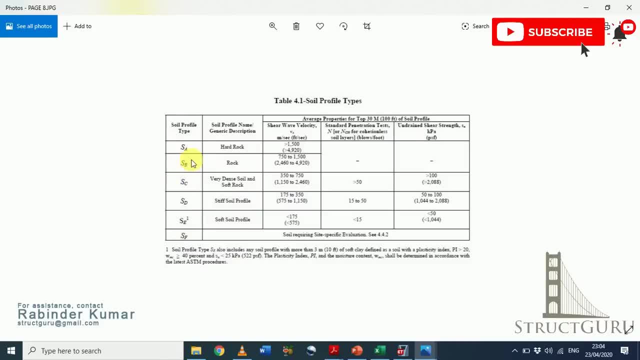 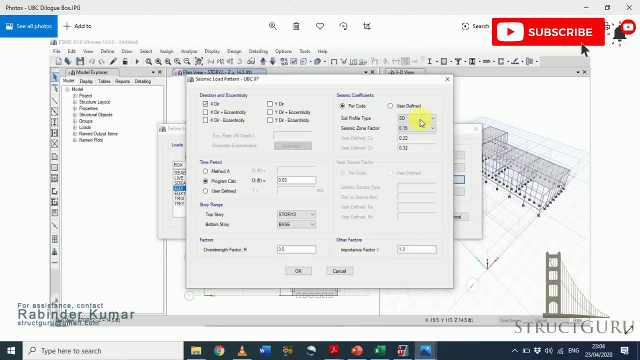 example, our building lies in SP region, so you have to choose SP here. now we have to look for the seismic zone factor, for example, if I have to design a building in Hyderabad region which is located in province Sindh. so first let's refer to Pakistan building. 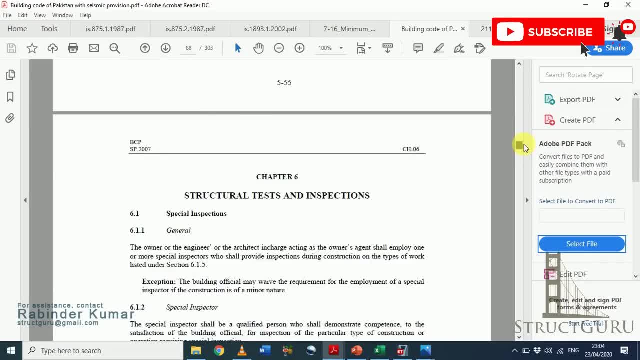 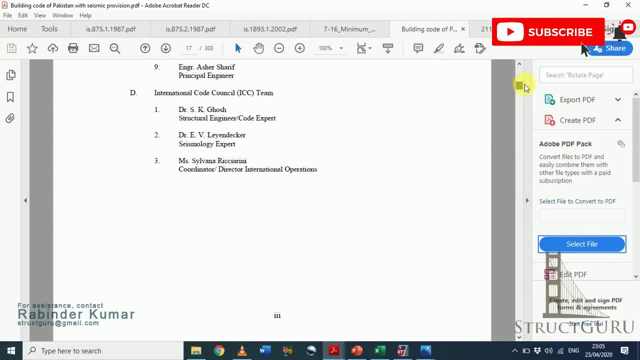 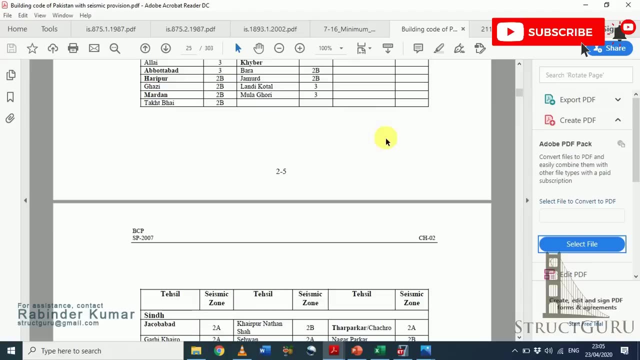 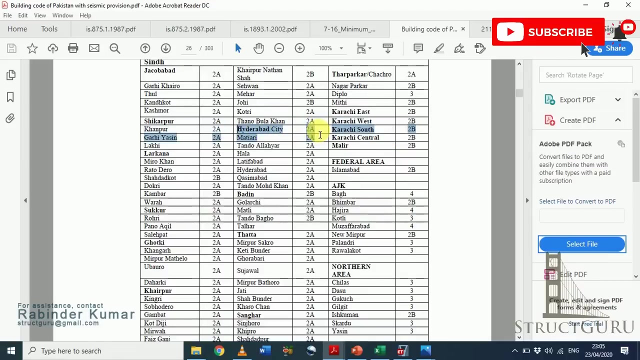 code. so first let's refer to Pakistan building code. so for Hyderabad region, first we have to see in which zone the Hyderabad lies. so Sindh in province, Sindh search for Hyderabad city. so Hyderabad city is in zone 2A. ok, now go and find zone factor. 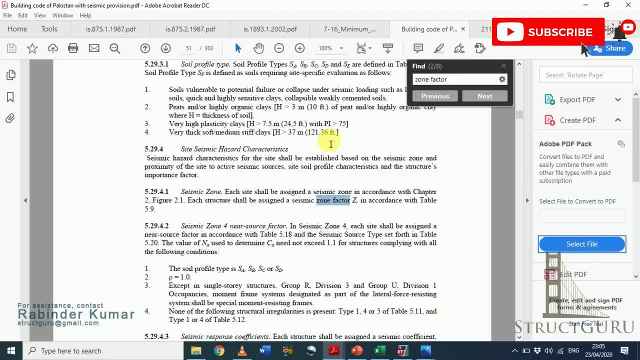 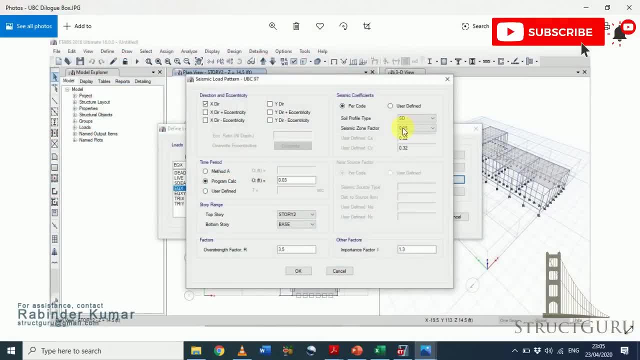 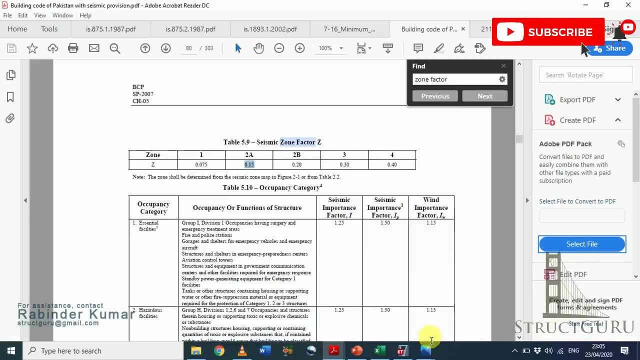 now go and find zone factor. so for 3A we have to put value 0.18. so in this dialog box we have to put 0.15. now you have to define the values of CA and CV. again we go to the code book for CA and CV. which we have to put as number and only in province Sindh. they are basically seismic zone factor. so for soil type B, zone 0.15. so the value of CV is 0.15 and the value of CA is 0.15, so you have to insert 0.15 in. 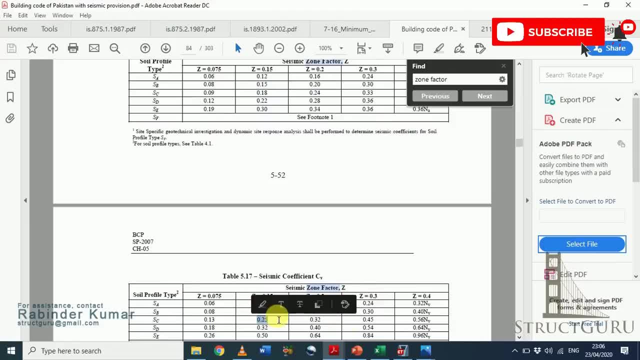 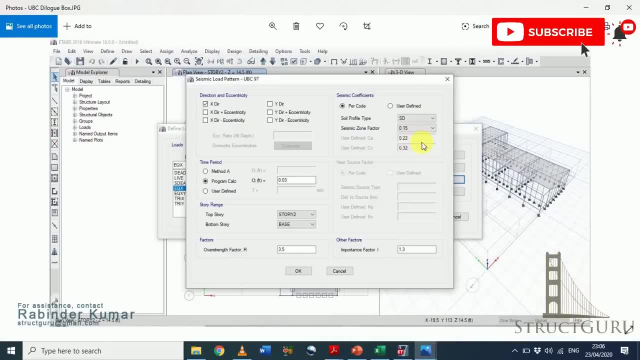 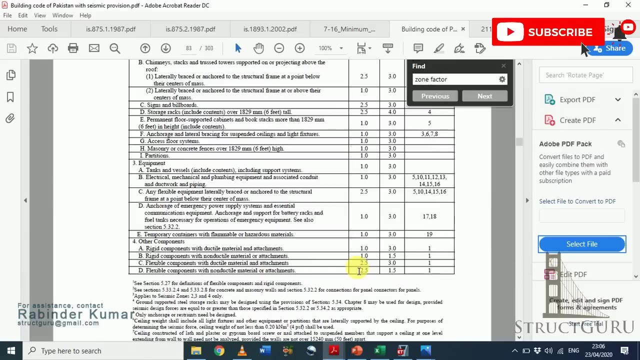 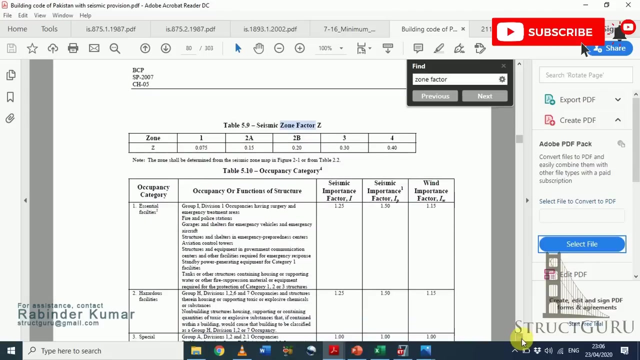 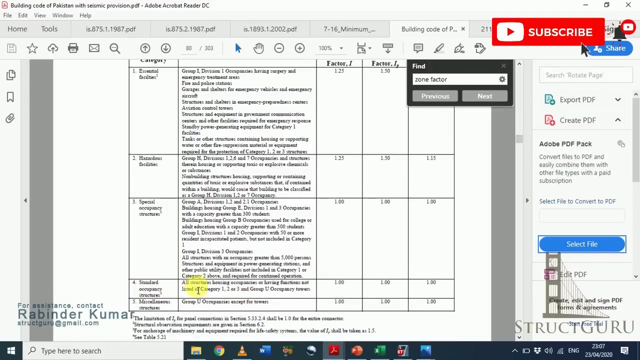 the section of CA and 0.15 as well in the section of CV. now importance factor. so important factor will be 1, because this is a residential building. we can also verify this from our code book. a standard occupancy, all structure housing occupancy, is in having function. 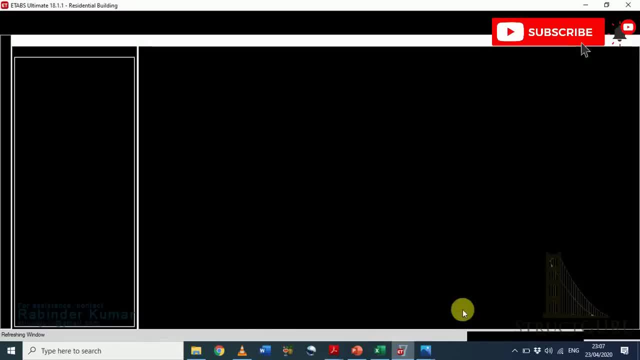 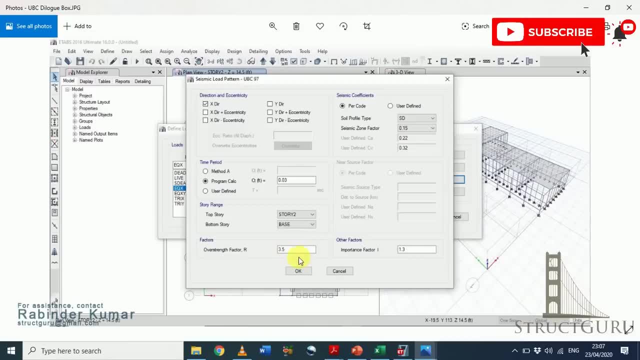 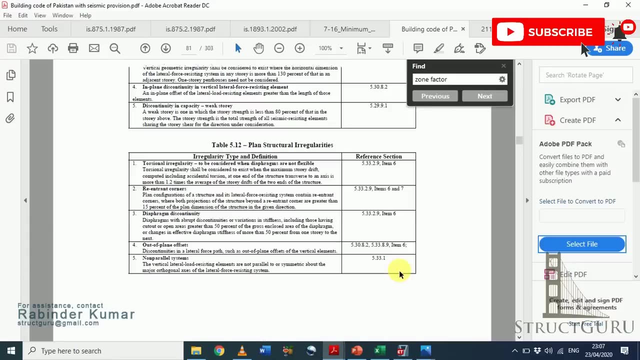 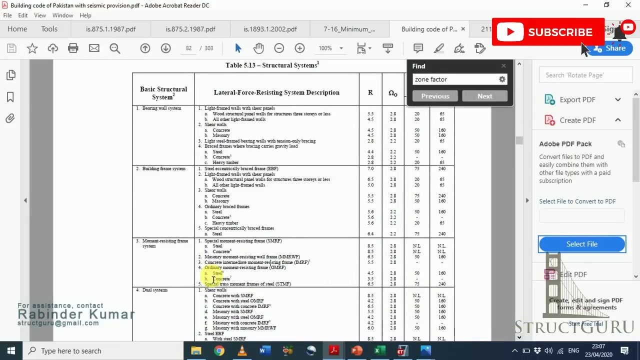 so I value is 1, so you have to insert 1 here over the strength factor are. I can refer to the code book. so for our building, our structural system is moment resisting frame and in the category of moment resisting frame it is an ordinary momenting, this moment. 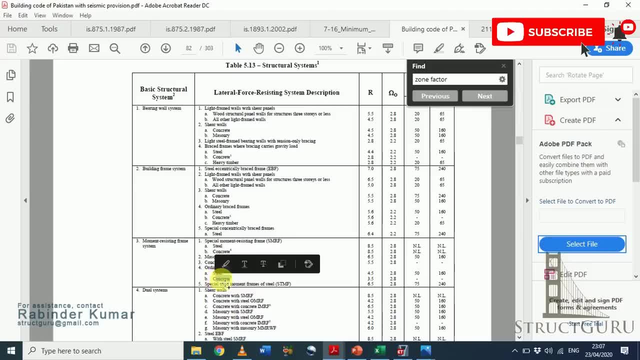 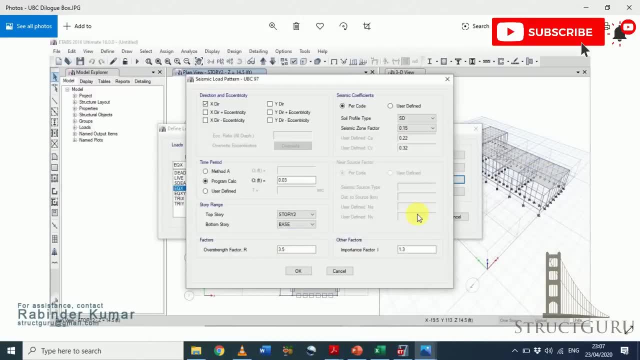 resisting frame concrete. so we have to choose 3.5. so just type 3.5 here. so in this way you have to use UBC code and find out all the coefficients from UBC code x in and insert all the values in seismic load pattern as we are going to design. 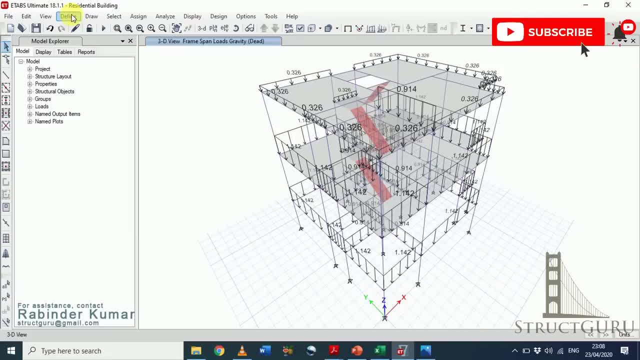 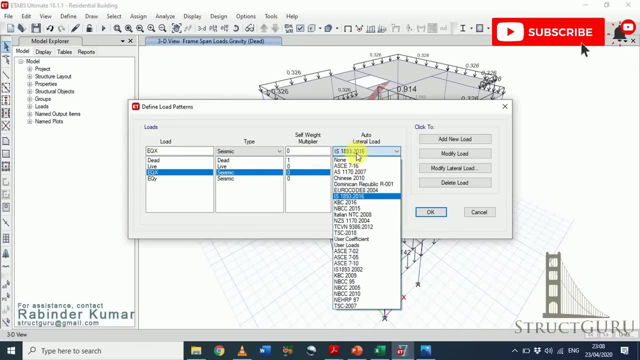 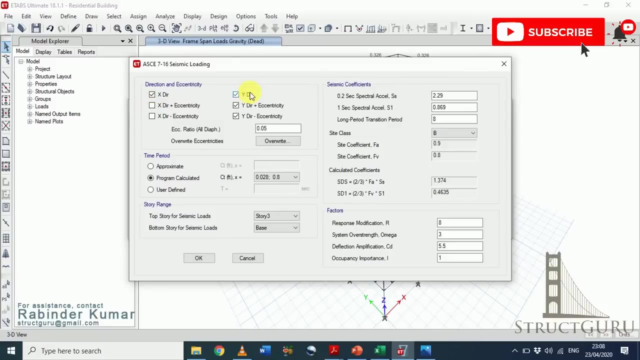 our building using ASCE ACI code. so go to the define menu. select load pattern. choose ASCE 716- click modify load. similarly, in right direction, choose ASCE 716, click modify load. uncheck all other parameters. I will discuss these parameters in advanced topics. now we have to look for these values first. 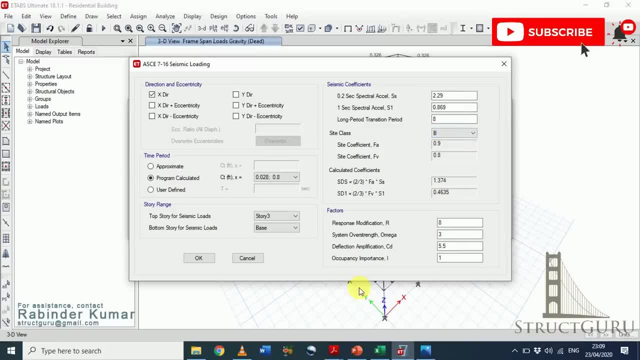 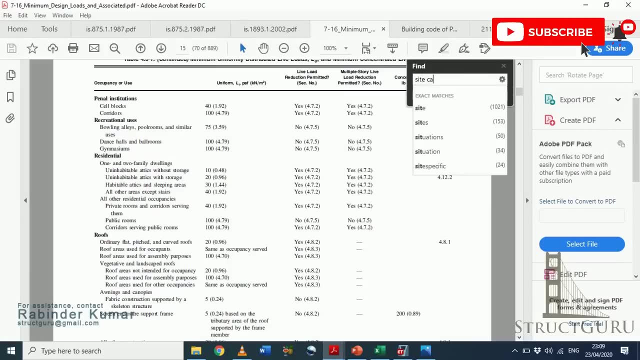 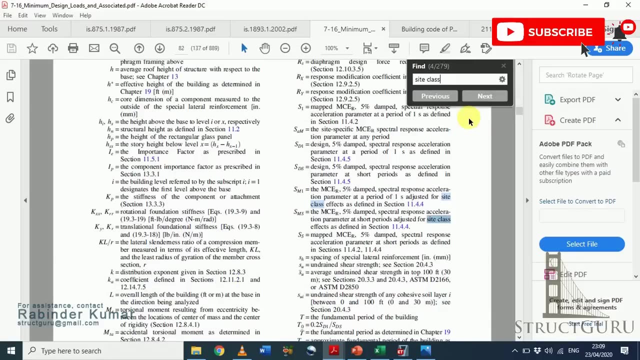 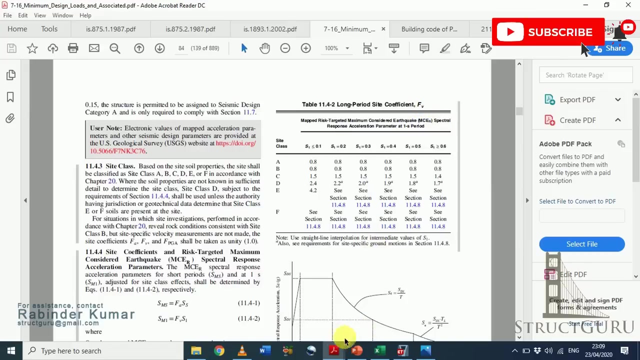 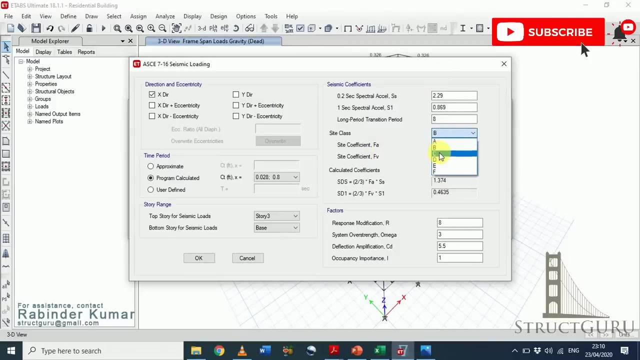 define site class. first we have to look for the site class from ASCE code, so site class, so side class. in side class we have to find the values of a, a and FB. if you just insert side classes, see so it eat ems will by default eat ems by default. 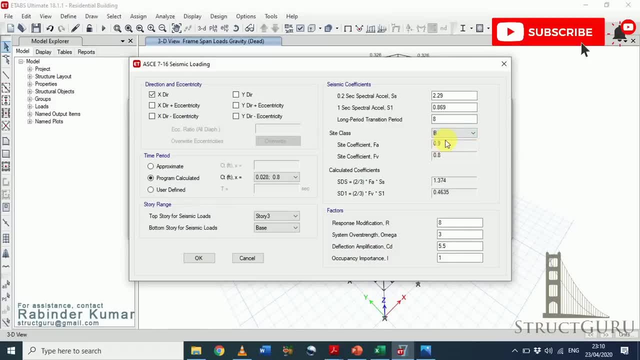 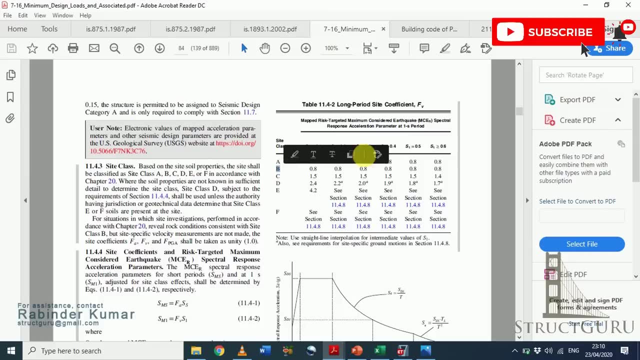 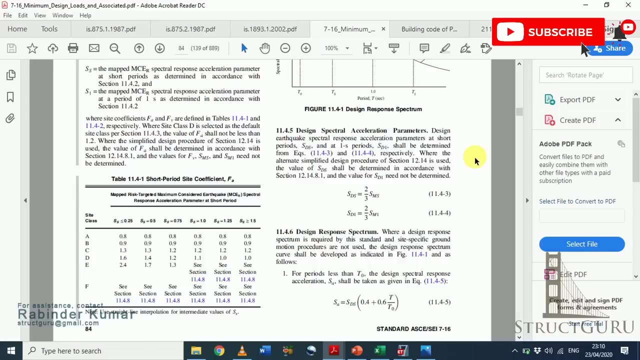 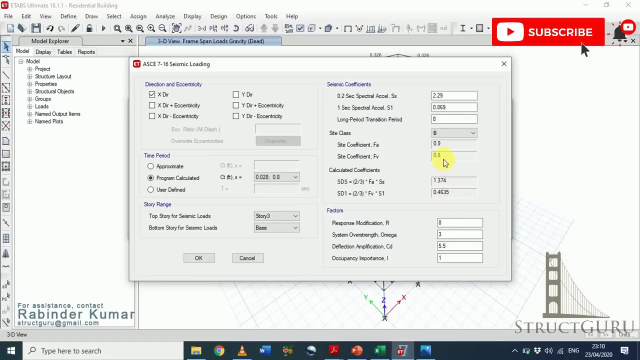 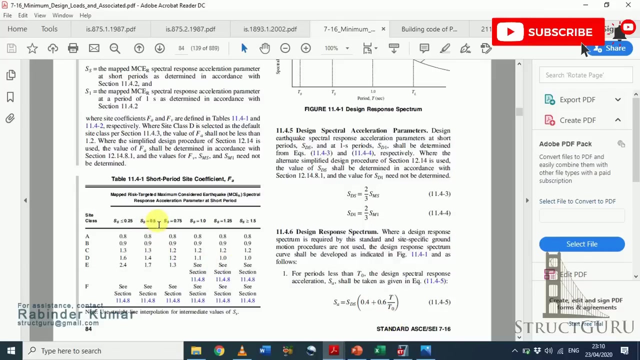 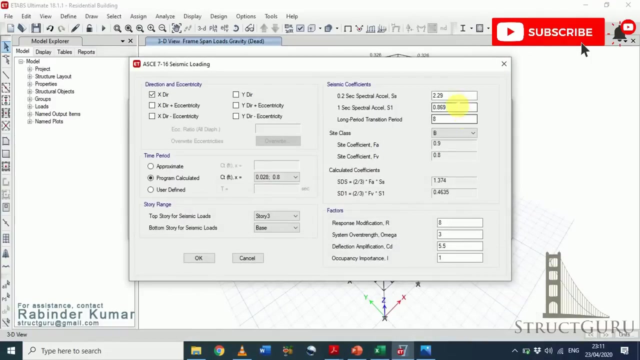 will take the value from code. so let's verify if you choose side class B to side class B. so if V is point eight and if a is point nine, if V is point eight and if a is point nine. so following this, we have to find the values of SS and s1. so SS is 0.5 and s1 is 0.2, 0.2 and 0.5. 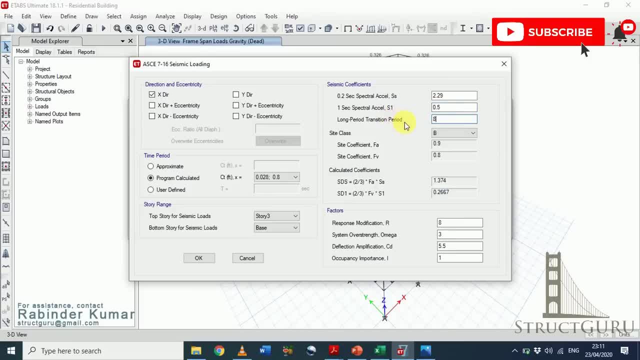 longer period. transition means chance of this value is used for high-rise buildings if it is more than four or five story welding. so you have to use whether you want to design a building for 10 seconds time periods or 11 seconds time periods. basically, this is advanced topic. you must have some basic. 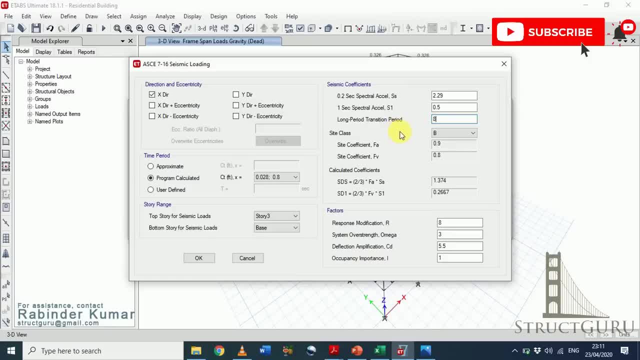 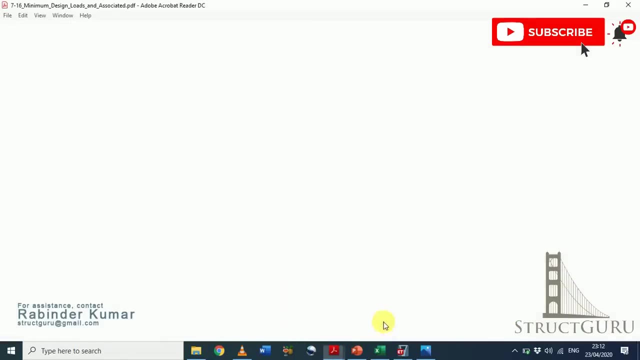 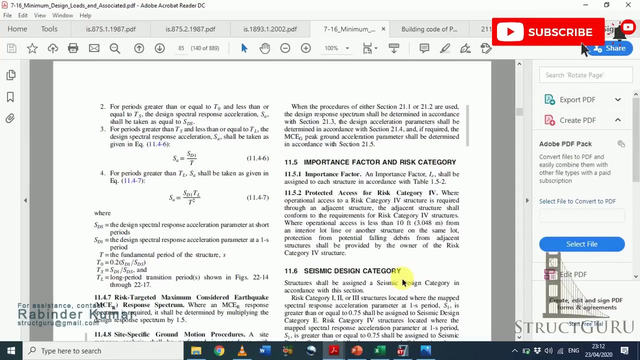 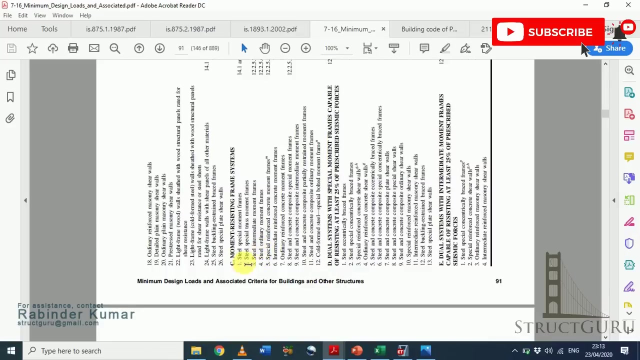 know-how about earthquake engineering. so just to just write eight here. you can also write them here, it's up to you. now. response modification factor again, as we did in, is code in Pakistan, building code. so for ordinary moment, resisting frame, so movement resisting frames. we are using ordinary reinforced concrete. 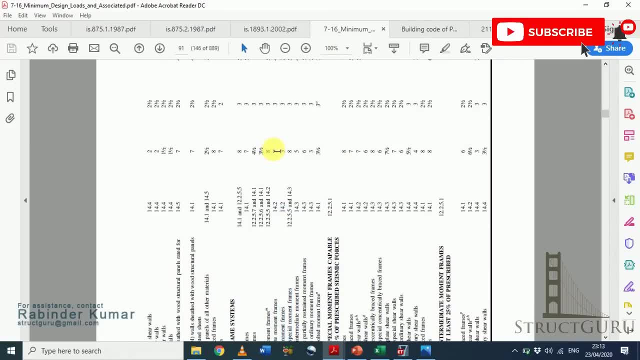 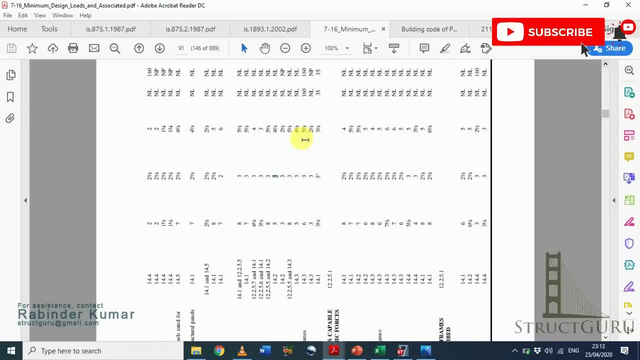 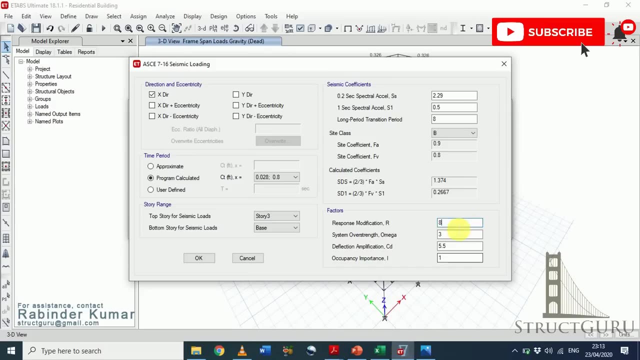 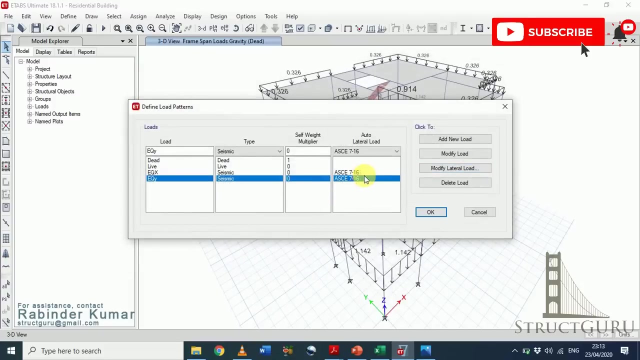 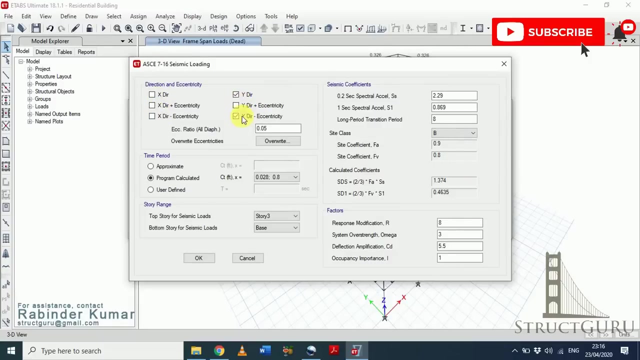 frames. for ordinary reinforced concrete frame, the value is five over a spring factor is three and deflection amplitude is four and half. deflection amplification is four and eight, three and four and a half. click. OK, and you have to do the same in right direction as well and check all these parameters: 0.5, 0.2, 3 and 4.5 click. 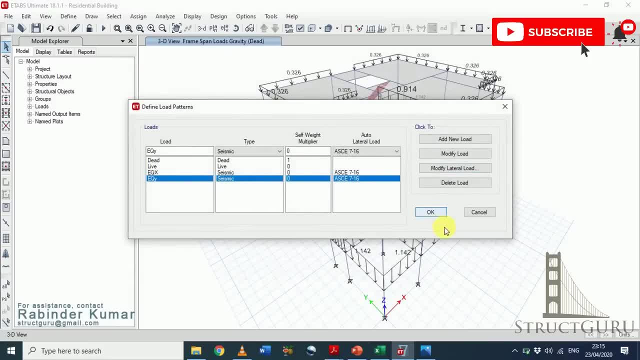 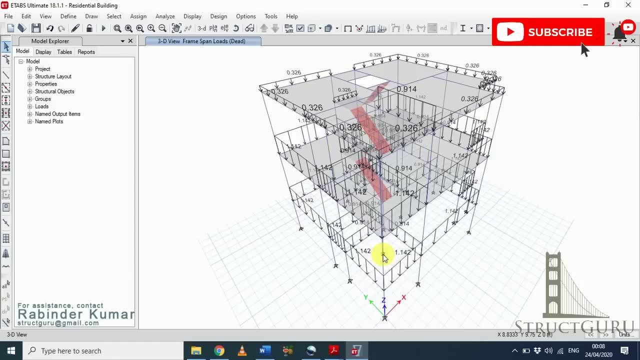 OK, now let's discuss about mass source. this is very essential for considering lateral load and seismic design of buildings. this means how much seismic weight should we include for calculating the base year? so let's see what are the provisions in ASCE 716 manual and is Indian standards building manual. so some 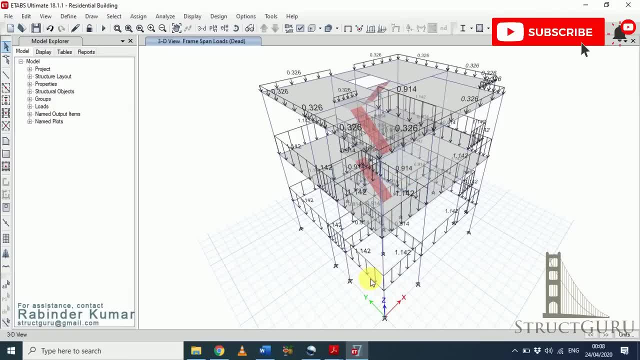 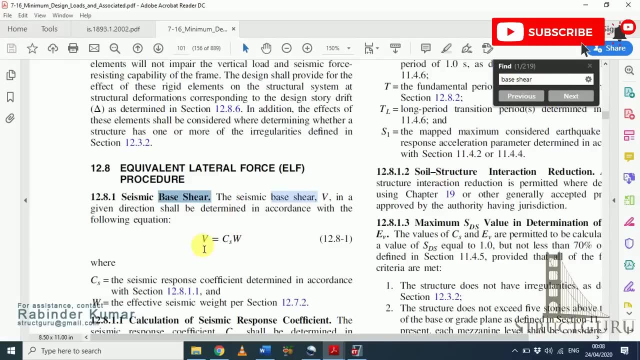 ones are very important for calculating the base year. so let's see what are the provisions in ASCE 716 manual and is Indian standards building manual. so some how the values are same in all the codes which you follow. but let's compare it. go and open ASCE manual. so first type the base year and you will be here. so 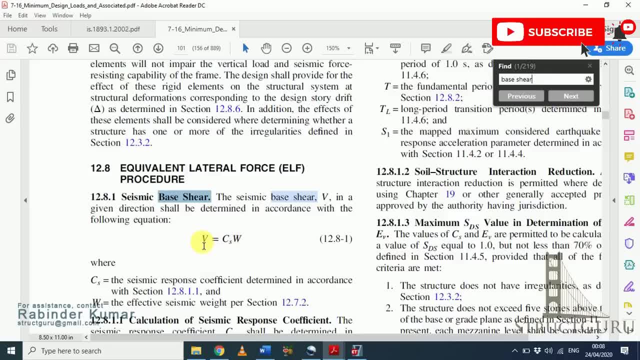 here you can see the equation for base year is written, which is: V is equal to CS, into W, where CS is seismic coefficient and W is seismic weight. so how much seismic weight do we have to include into our structure? so for this you have to click: W is the effective seismic weight for sections. how much weight should we? should we include for our lateral load calculations. so click this link so it will bring you to the section 12.7.2, where effective seismic weight criteria is given. so read this criteria. so the effective seismic weight W of structure should include all the dead load. include the dead load as defined in. 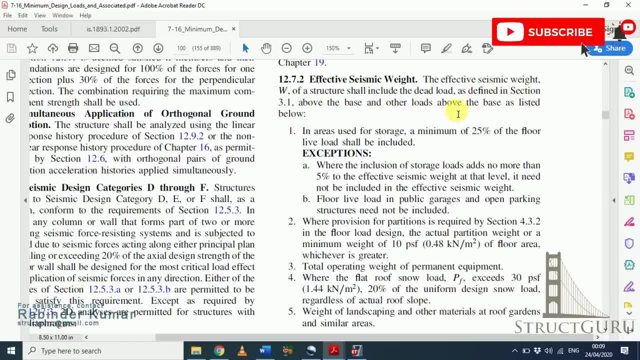 section 3.1, above the base, and other loads above the base are listed below. so you have to include all the dead load which is included in our structure for imposed loads. the conditions are given: an area is used for storage a minimum of 25% of. 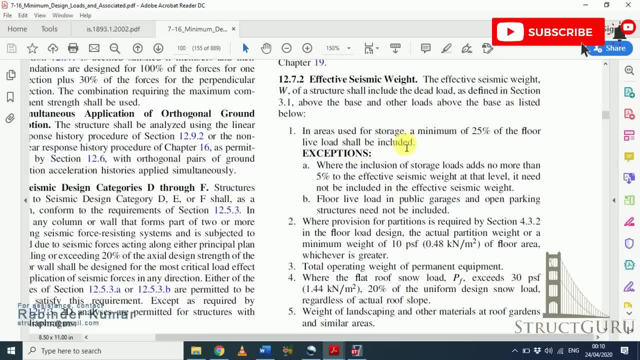 the flow live load should shall be included. so 25% live load you have to include. so there are some ten exceptions also written where the inclusions of storage load it's no more than 5%. so then you can neglect the seismic weight, so it need not. 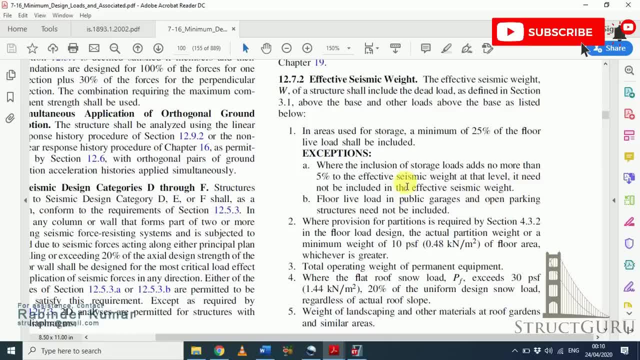 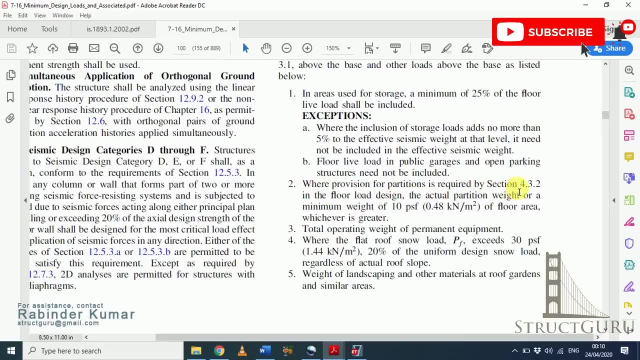 to be included in the effective seismic weights. as I said, you can neglect the value. similarly, live load in public garages and open parking structures need not to be included. so second isあ, where provision for partitions is required by section 4.3.2 in the floor load design, the actual 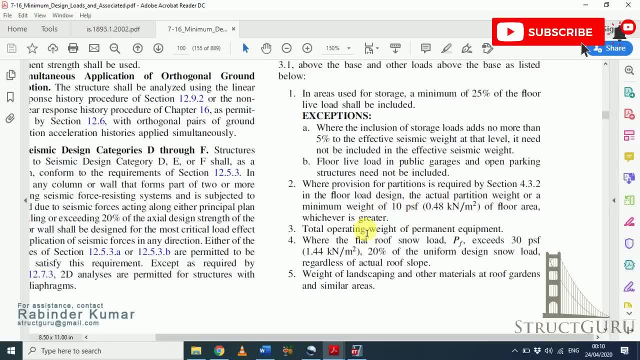 partition weight or the minimum weight of 10 PSF or floor area weight, shake or created from any wet or dry Writing is required for earthtime consuming product. very well, water storage and the Football dead 57, whichever is greater, so that you have to include in your masters, for example. so 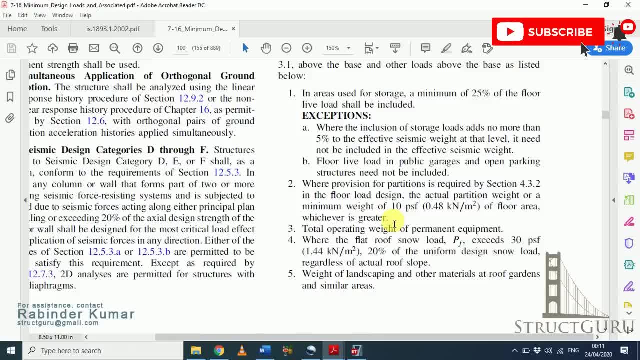 we might have seen wooden partitions and or glass partition in office building. so in that case you have to include 10 PSF of the floor area into the mass source calculations. total operating weight of urban recruitment is the if there is any machinery operated in the building. so you have to calculate the load of that. 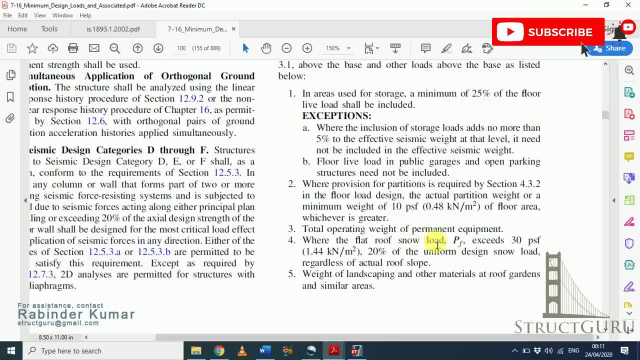 as well. so in case of snow load you have to take 20% and similarly weight of land escaping and other materials at roof gardens and similar area. so the conditions are written according to these conditions. you can define the parameters in mass, source option and ether. so I will tell you how to specify. 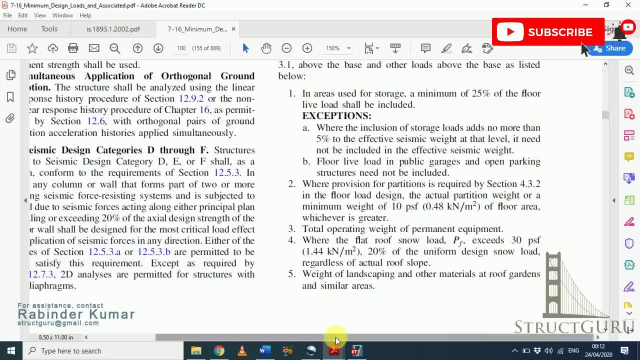 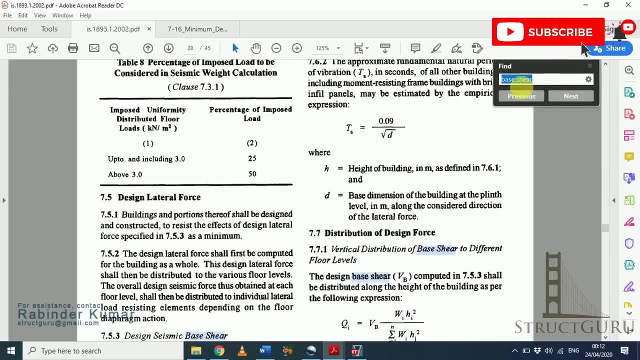 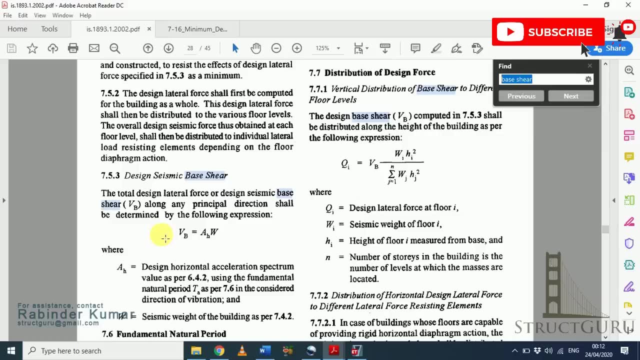 these conditions in mass source options. now let's compare with Indian codes. you so again for base here. just type base here in the search option, so it will bring you to this option again. the equation is same: VB is equals to a is W. the W is the seismic weight, H is the horizontal spectrum value. again, it is a. 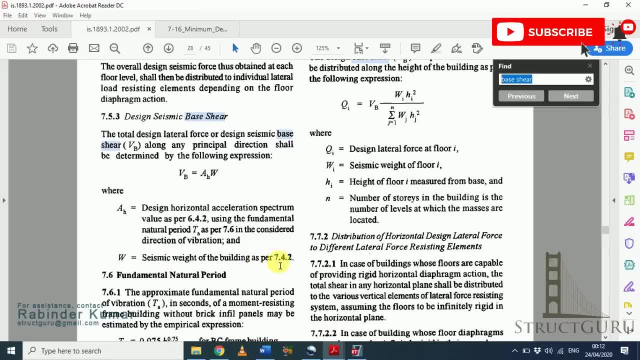 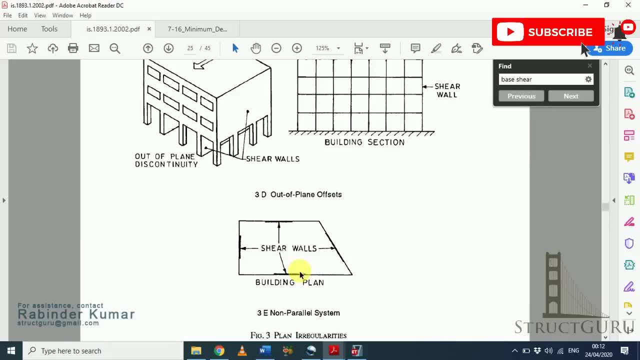 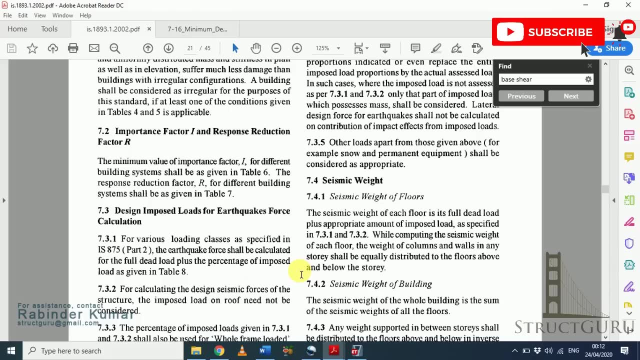 seismic coefficient. for W seismic weight, you have to refer to seven, point four, point two. so let's say it is 7.4.2.. so let's move to 7.4.2, 7.2, this is 7 point 4.2. seasumic weight of a building. 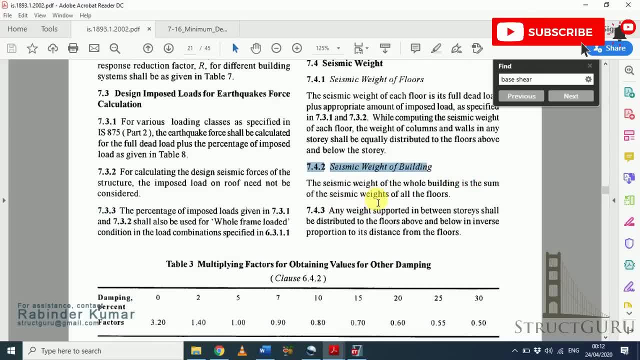 the chief equipment of the full building is the sum of seismic weight of all the närvaråð, all the funds dó pathway. easn't very easy to understand anyways. seismic weight of each floor is its full dead load plus appropriate amount of imposed load. so you have to include the full dead load in my source calculation. 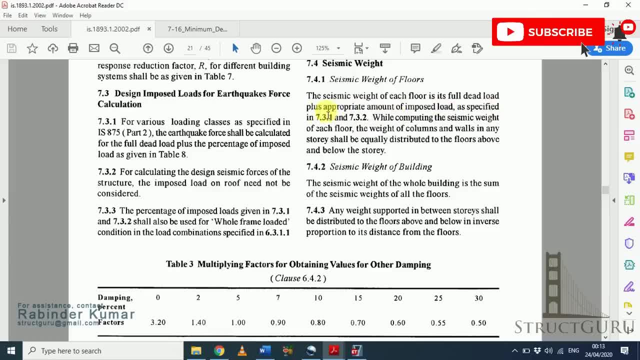 plus appropriate amount of imposed load, as specified in section seven, point three, point one, and seven, point three, point two. so let's go to these sections, for various loading classes is specified in is at seven five R to the earthquake force shall be calculated for the full dead load plus the percentage of 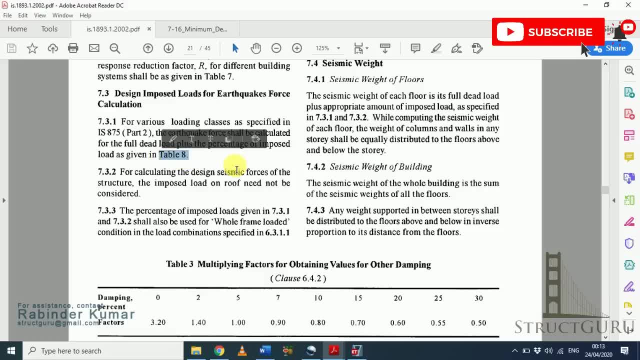 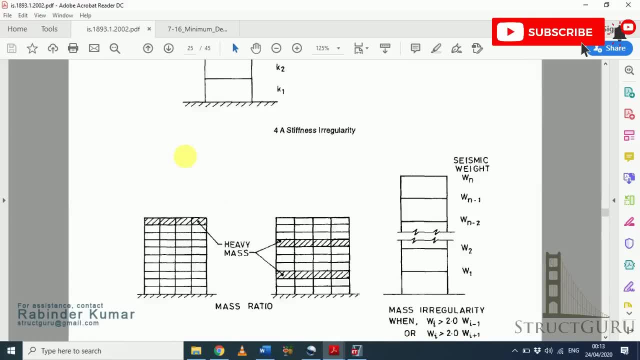 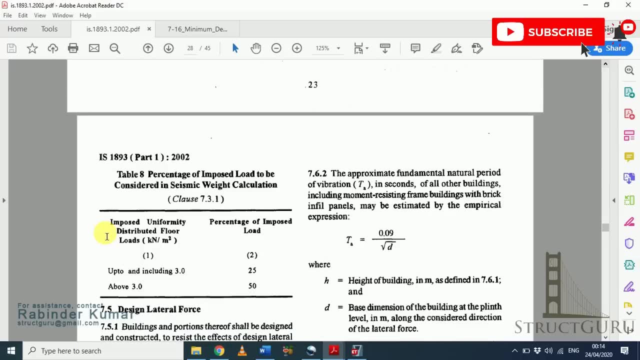 imposed load as given in table eight. so the person for the percentage of imposed load we have to refer table eight. so let's go to table eight. you have to move down a bit. so this is table eight: percentage of imposed load to be considered in seismic weight calculation. so if the live load 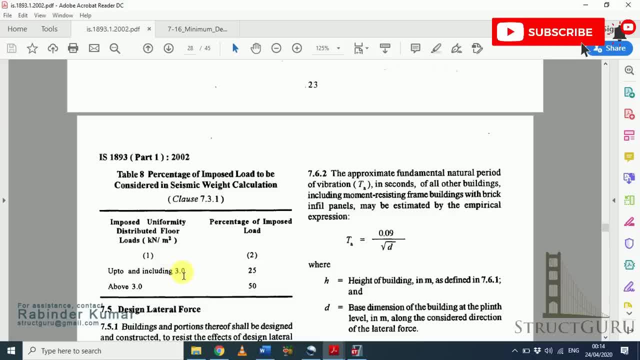 is given as given in table eight. so the percentage of imposed load to be is up to or including 3 kN per m2, you have to include 25 percent of 25% of lime load and the similar value of the specified in American code. if it is more than 3, you have to include 50 % of live load in. 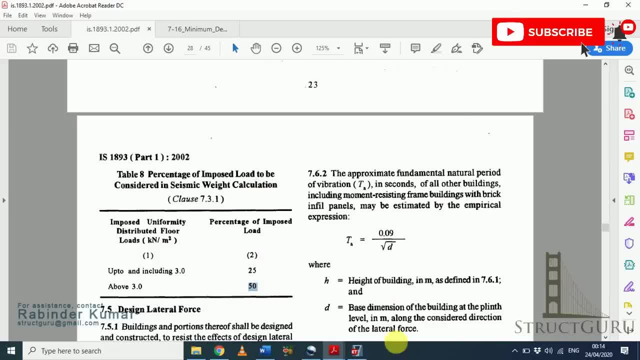 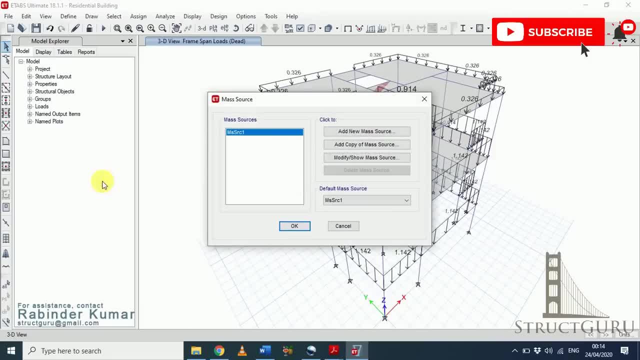 your base sheer calculation. so let's go to ETAB's and define the mass source over there. so go to define menu, click mass source. as you can see, ETAB by default is defined by the conventional evaluation type. find a mass source, but we have to modify the parameters into it. go to modify, show mass. 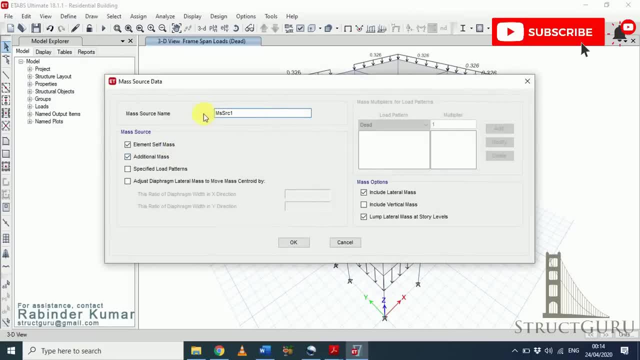 source. if you want to change the name of mass source, you can change by typing some name here. let's type lateral. as you can see, there are four checklists, parameters, so i will explain one by one. so number one is element self mass. that means all the self weight of structure. 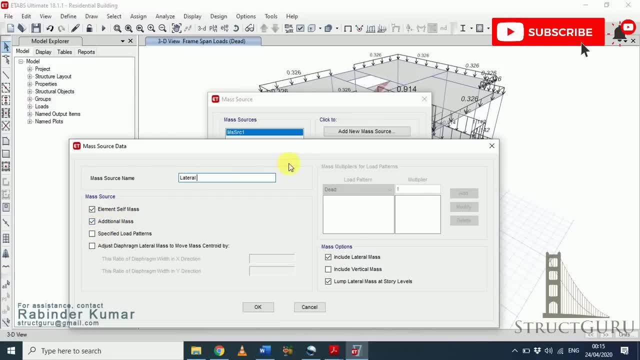 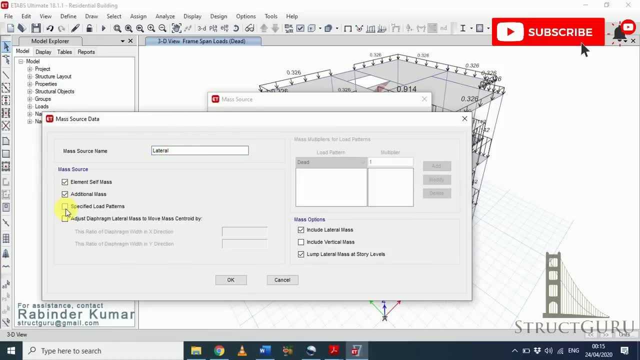 so that should be included. so yes, check this additional mass. any additional mass you want to include in the mass source. you have to check this parameter. the third option is specified load patterns. that means you have to specify the load patterns by yourself, referring to the code books. so if you are referring to indian standards, you have to refer indian. 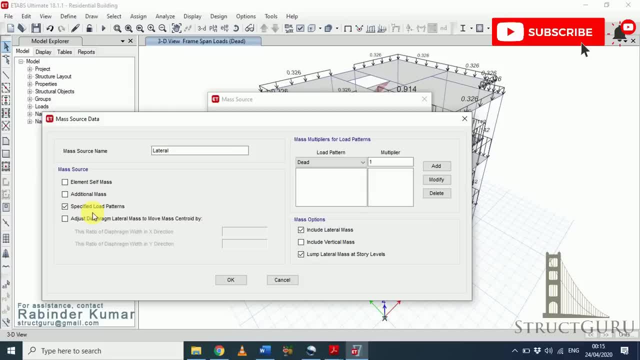 code books. if you are referring to any other country building codes, so you have to put the values accordingly. similarly, the fourth option is adjust diaphragm, lateral mass to move mass and quad bar. so this, this the dialog box, is basically related with the centricity. 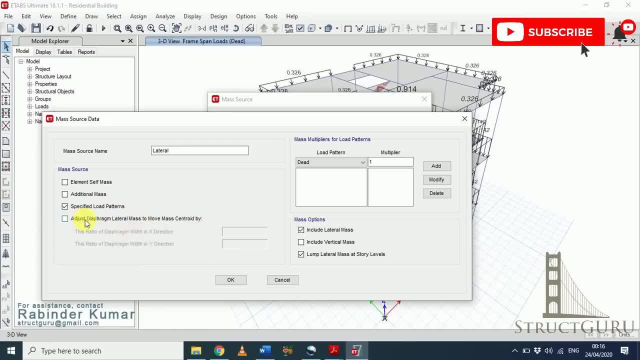 so normally we don't do anything with this dialog box as you want to. if you want to change the values, you can, but leave as it is for this stage. so let's specify the load: veteran as given in our ASCE and Indian code. so we have to. 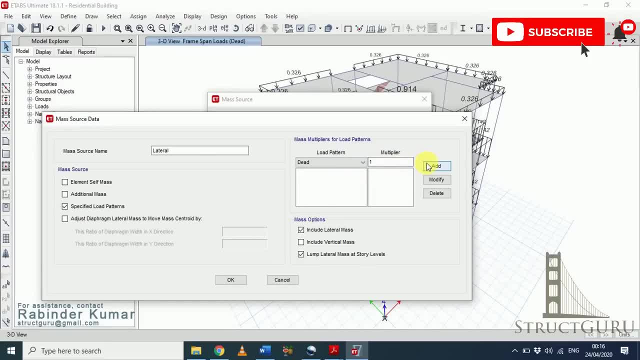 complete, we have to include all the dead loads of the building. so select dead from this option and click add, and 25% of the live load, right 0.25- and click add. so we are done now. there are other three options, so let me explain one by. 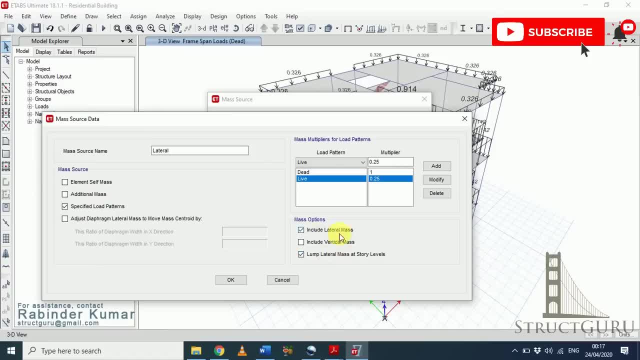 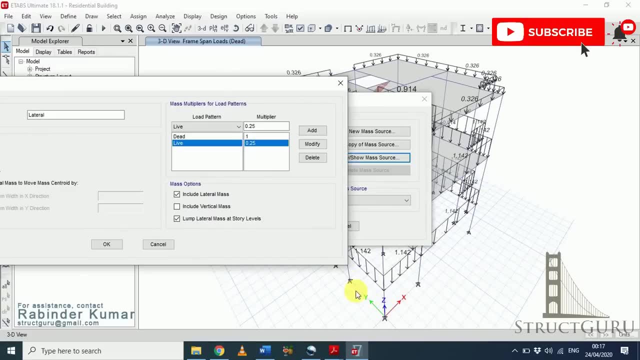 one. so first option is: includes lateral mass. that means the mass in x direction and y direction will be included. and the second option is include vertical man. this is unchecked by default because the letter motion this direction is so negligible so that's why it is not accounted in this option. and the third is lump lateral mass is story levels. 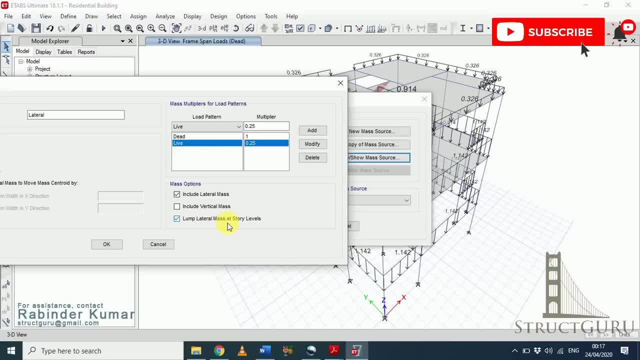 basically that means all of the surrounding data is counted in the. the self-weight and the mass force are considered to be accumulated as totally level, so you have to check this option. if you want to take these three, it's okay. it's not a big deal. this way we have to define the mass. 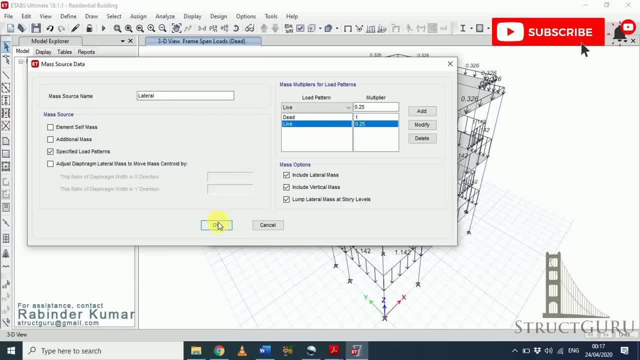 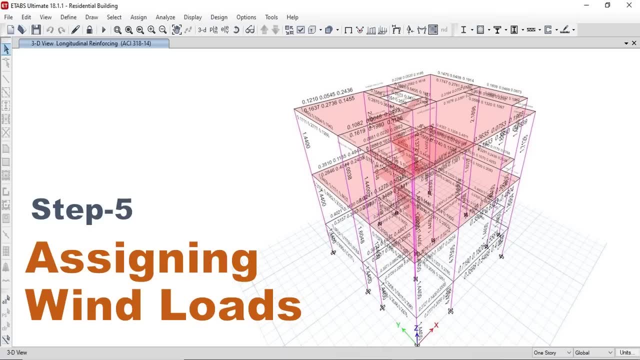 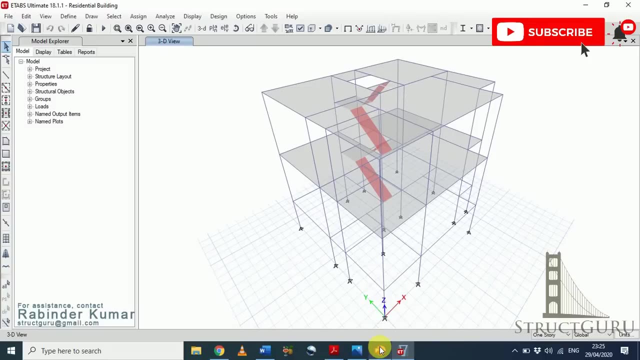 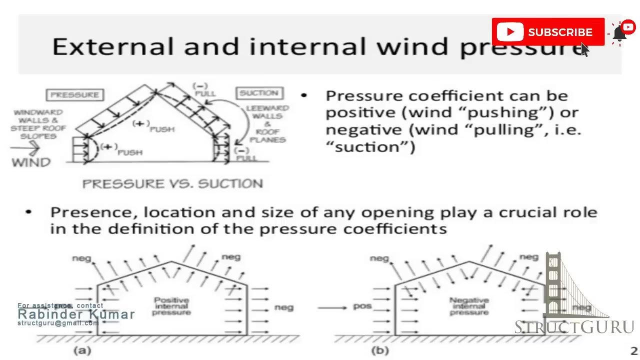 force theta in our model. so once we are done, click OK. so first understand how. when force I on a structure through a diagram. as you can see from this diagram, wind coming from left and side will create a pressure on the left-hand side wall and will create a section on right-hand side of the wall. 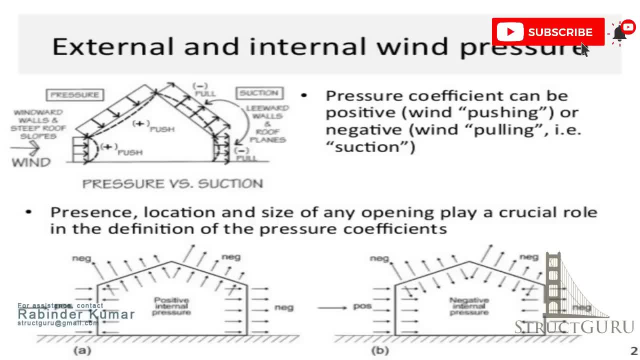 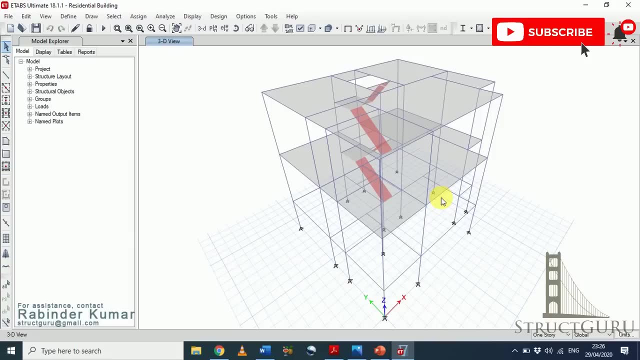 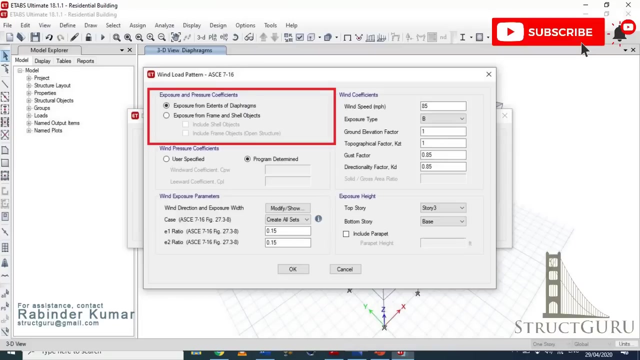 this is. this side of wall is known as windward direction, and this is section on the right hand of the wall, ok, known as leeward direction. so in ETABS you can apply wind loads in two different ways. first is exposure from extensive diaphragms and the second is 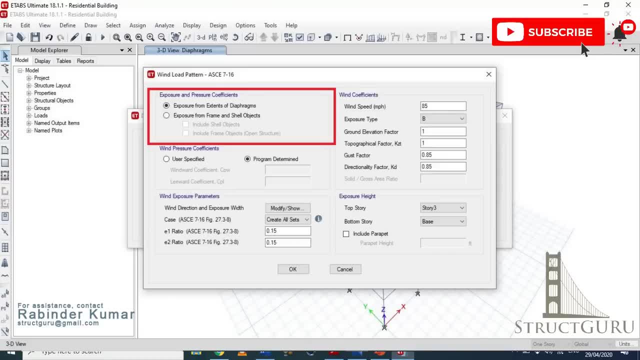 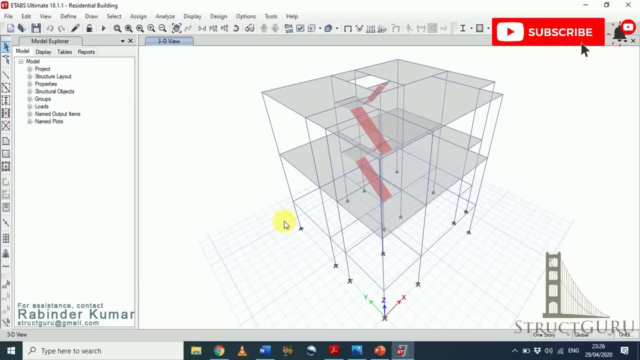 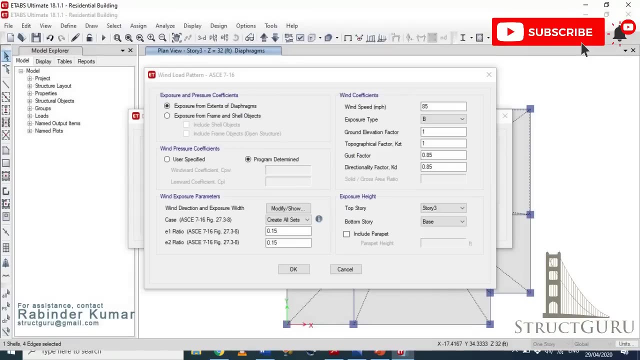 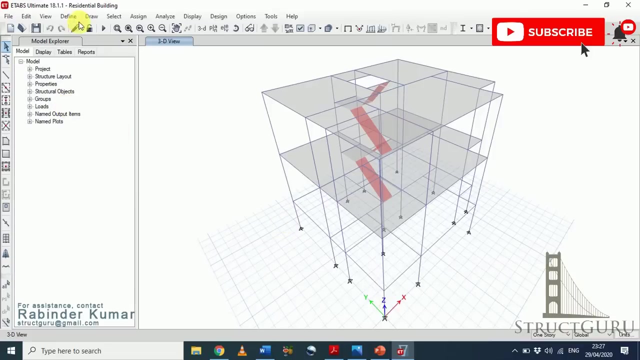 manually applying the wind pressure coefficients on the walls. for that you have to draw the walls. so first we will discuss what are the diaphragms, how to define them, and then we will talk about wind load patterns and discuss each terminology associated with that. to define the diaphragm, go to define menu. 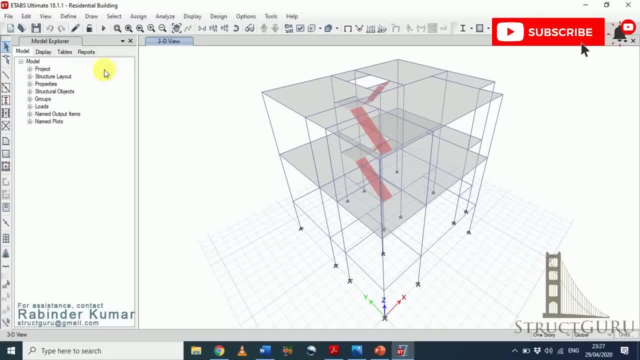 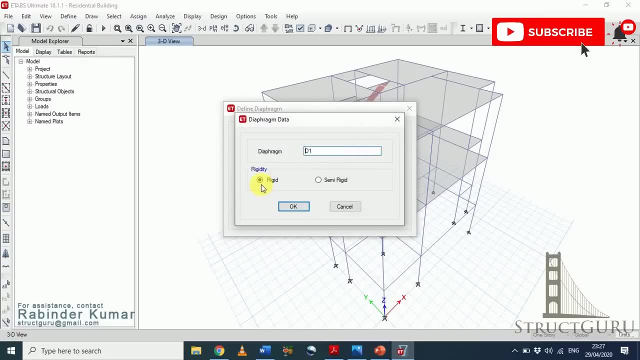 click the diaphragm, click modify, show diaphragm options. so here you can see two different options: rigid diaphragm and semi rigid diaphragms. so for rigid diaphragms you have infinite in plane stiffness and it does not exhibit any membrane deformation, and for semi rigid 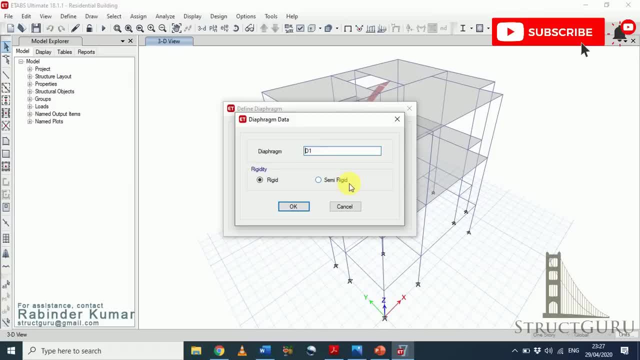 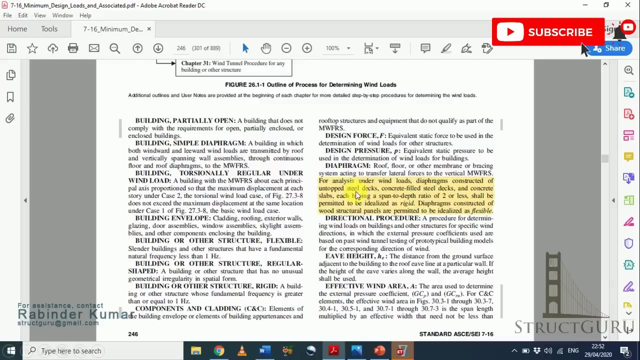 diaphragm. it simulates actual stiffness properties and behavior. basically, in both cases the loads will be distributed differently. now the question is when to choose rigid and when to choose semi rigid. in this case you have to refer a code book from the code book as it is written for. 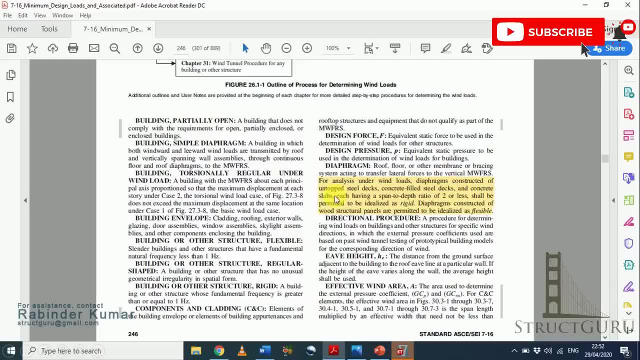 analysis under wind loads. diaphragm constructed of untapped steel decks, concrete-filled steel decks and concrete slab, each having a span to depth ratio of two or less, shall be permitted to be idealized as rigid. diaphragms constructed of wood structural panels are permitted to be idealized as flexible. 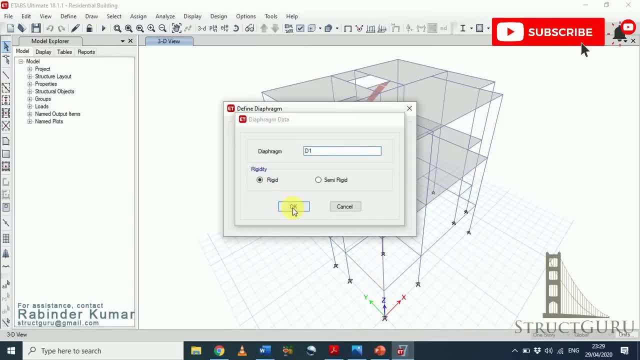 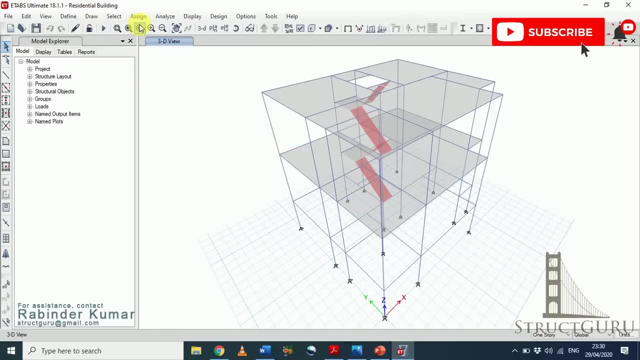 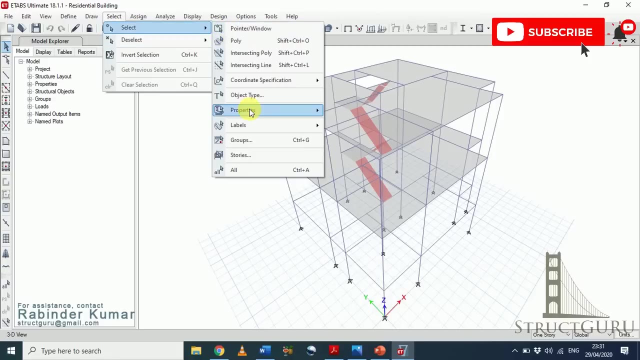 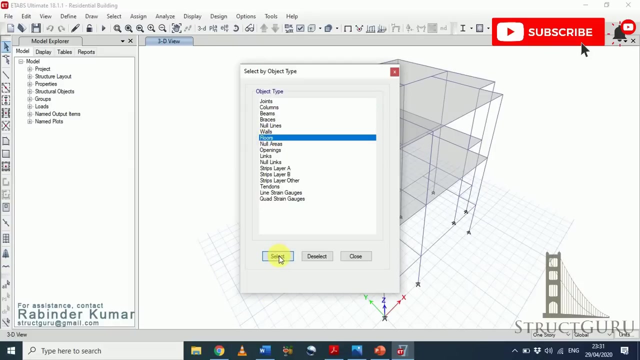 for our case we will select rigid diaphragm. so now we have to assign the diaphragm. so for this case you have to go to the assign menu first. you have to go to the select and then select object type. from here you have to select floors, then click. 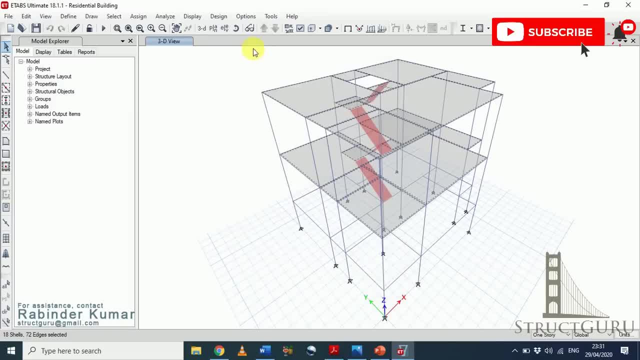 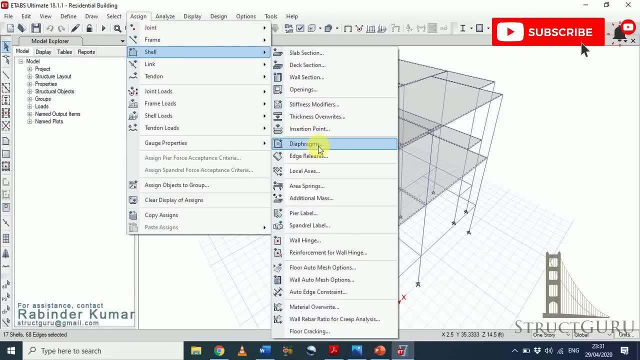 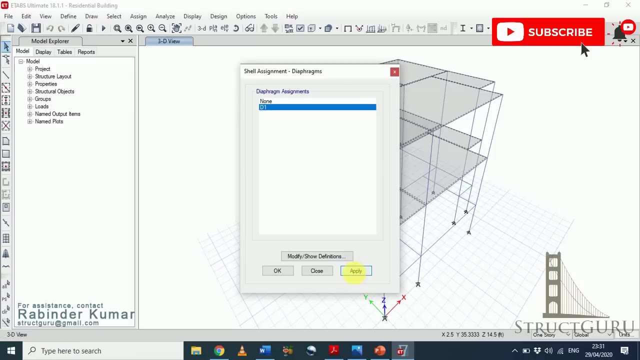 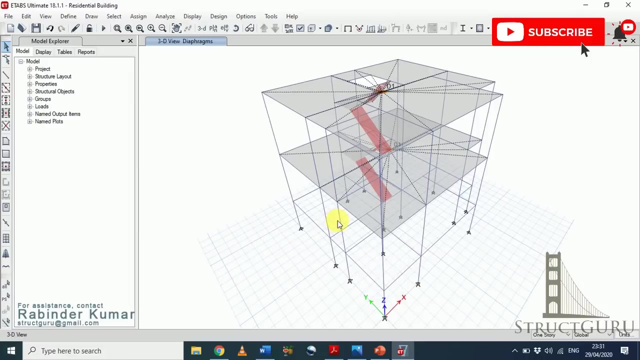 select close out to the 3d menu. now go to assign menu shell. from shell you have to look for diaphragms, click type on the diaphragm we have just assigned, then click apply, then ok. so now you can see here on a screen a kind of spiderweb image assigned to. the floors. so basically they represent here on a screen a kind of spiderweb image assigned to the floors. so basically they represent those the elements below thrown in the realism, meaning it was made a fine finishing floats. so basically the elements below fallen in this section, though, when we 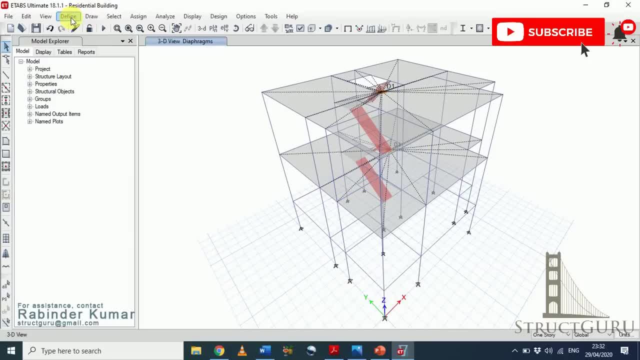 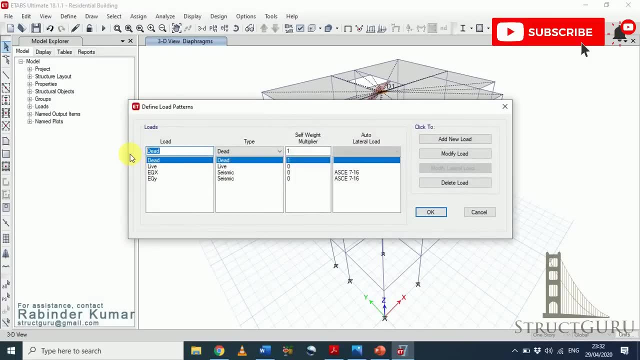 the diaphragm. so in order to define the wind load background, go to the define menu, select load background. so first I will discuss ASCE 716 code, how the wind load background are defined using American code. so write wind from X direction. we have to define wind load background in both the direction select. 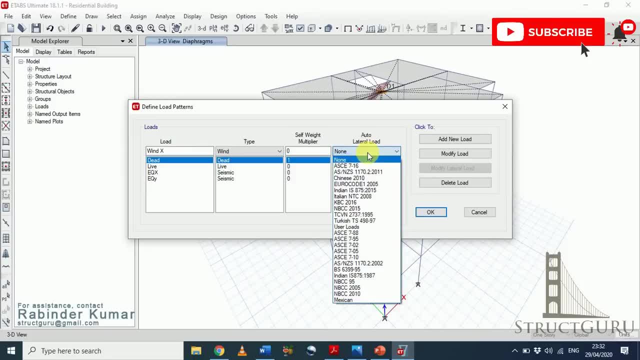 the type of load, which is wind, and, from auto lateral load drop-down list, select the code. so, for our case, as I am going to, as I am going to select ASCE 716- it's new- then, similarly, in wire direction, we have to do the same click. 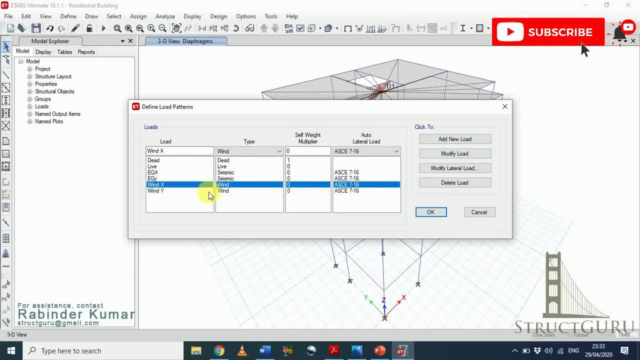 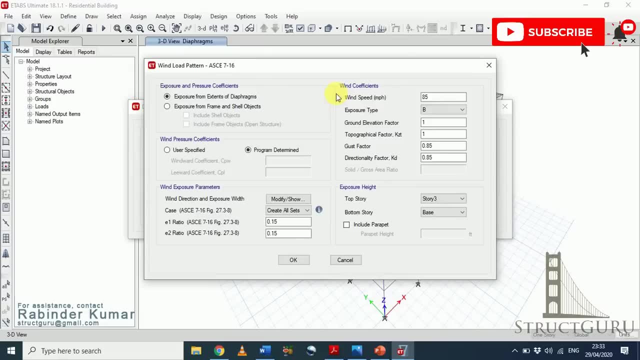 OK, now go to the, now select X direction and go to modify lateral load. so in this dialog box you will see lots of parameters are written, so I will explain one by one in detail. so as I X. so, as I discussed earlier, there are two ways to define the wind load parameters. number one is exposures from extents of 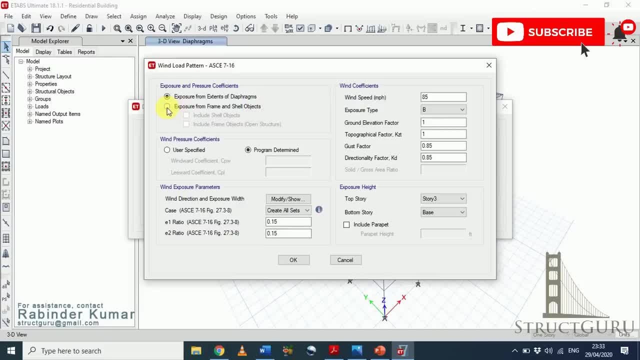 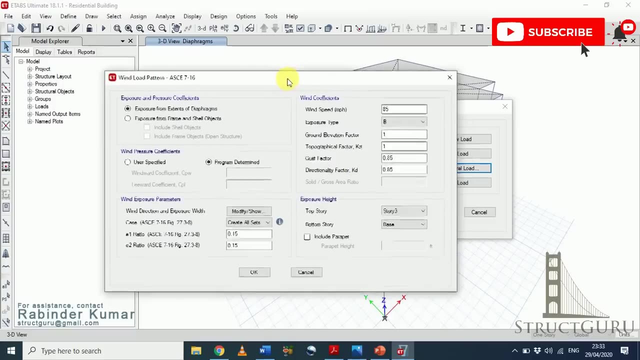 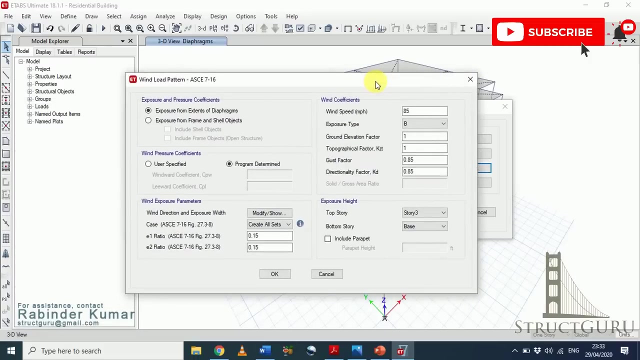 diaphragm and exposure from frame shell optics. I will discuss this. so first we will focus on this method, which is exposure from extents of diaphragm. so in this example we have to define wind load. so what does it mean? all our wind load will act on the center of mass of this structure. so after that you have to. 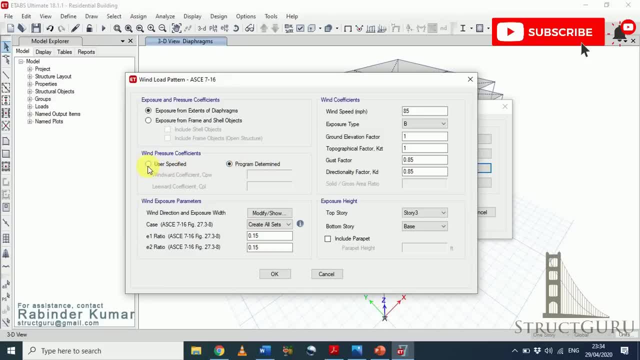 select wind pressure coefficients. so either you choose program determine or you choose user specified. if it is user specified, you have to put these coefficients from the codes. and leeward coefficient, which is CPL, other now wind coefficients. lets me define these one by one. so when the speed is the rate at which the wind is. 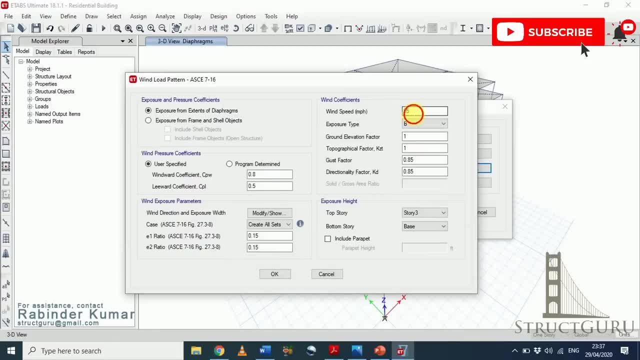 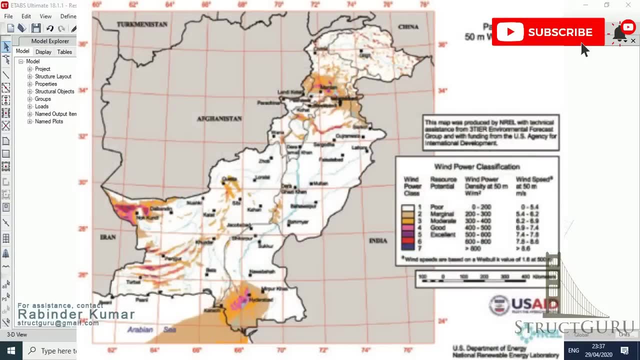 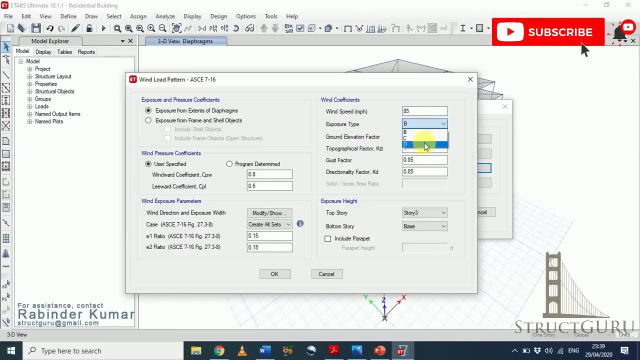 moving in a particular area. you can get this value from wind diagram of the can different countries, if you explore your time. then we have another option, which is exposure type. so there are three exposure type mentioned in American standards, which is B, C and D. so I will explain you one by one from the figures. 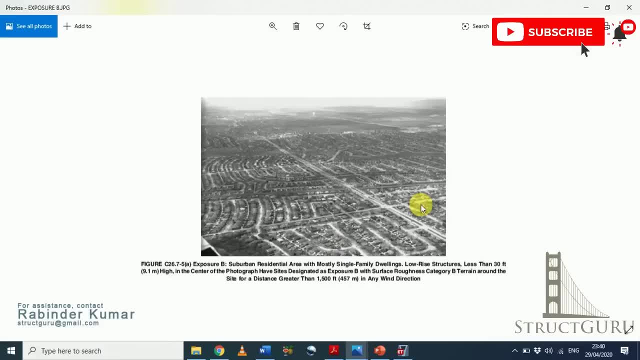 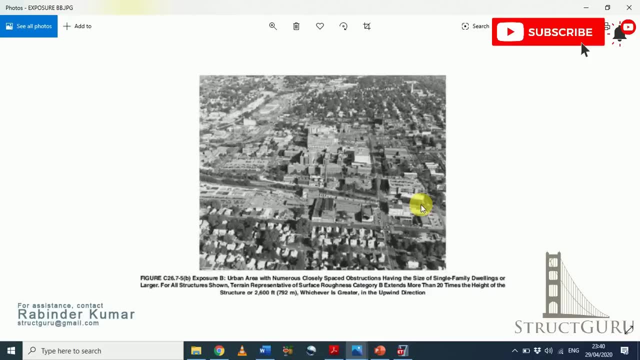 so exposure type B means a suburb residential area where mostly you will see single-family dwellings or low-rise structures. I can also explain you from another figure which is also exposure type B. so this is an urban area with numerous closely spaced buildings, obstructions having the size of single family dwellings. so these types of areas. 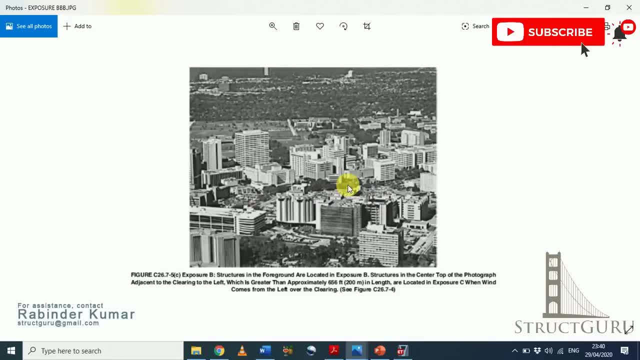 are known as exposure B type of area, or you can also differentiate exposure B from other two categories, which is, structures in the foreground are located in exposure B, so structures in the center top of the photograph, adjacent to the clearing to the left, which is greater than approximately 656 feet in. 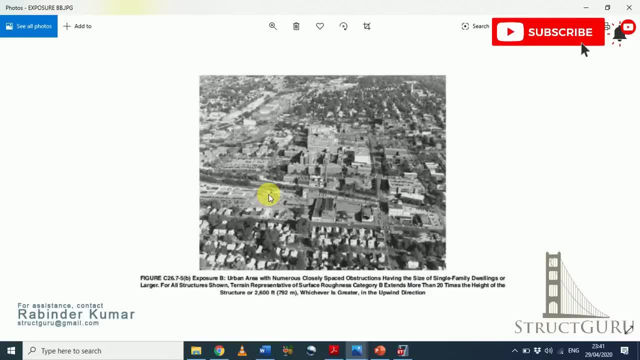 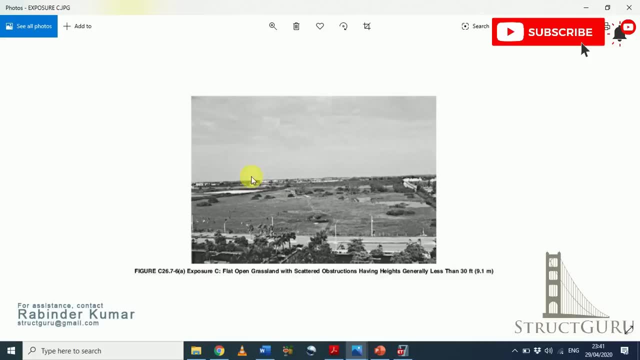 length. so these two categories are known as exposure B type of area, or you can also see the same in the second picture. so these kinds of areas is shown in these. three figures are referred as exposure B. similarly, exposure C type, that means flat, open grassland with the scattered obstructions having heights less than 30. 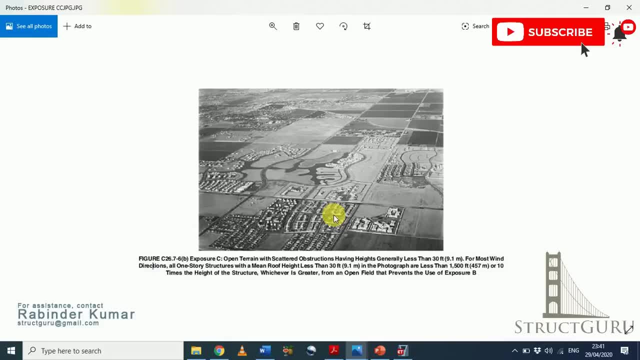 feet or 9.1 meter. another picture for exposure C, see open terrian with scattered obstructions is referred, the same as exposure B, so the height of the building is generally taken as less than 30 feet. now we will look to the exposure type T. 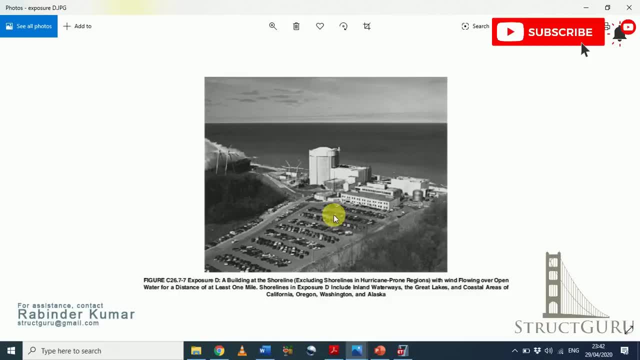 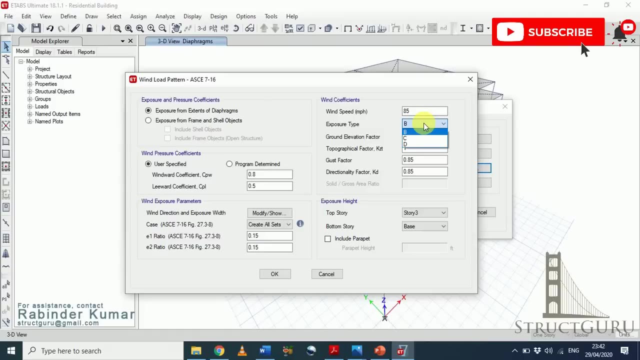 so the area of the buildings located near to this seashore, or near to the sea shorelines. they are referred as exposure T because they will experience heavy winds due to their pacing towards the seaside. from there, you will choose what kind of kind of exposure type your building is going to face. for example, i am choosing exposure type b. 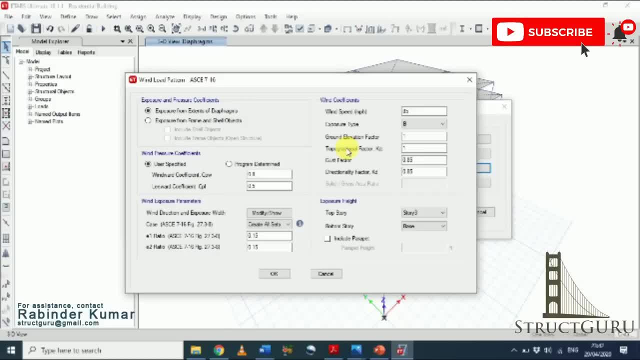 now. then you have to look for ground elevation factor. so the ground elevation factor is the ratio of air pressure and density at elevation related to the standard values. means level with constant temperature. so this level, this elevation, is determined with various formulas, but but if we refer to the code book, so this is. but if you refer to the code book, it says: 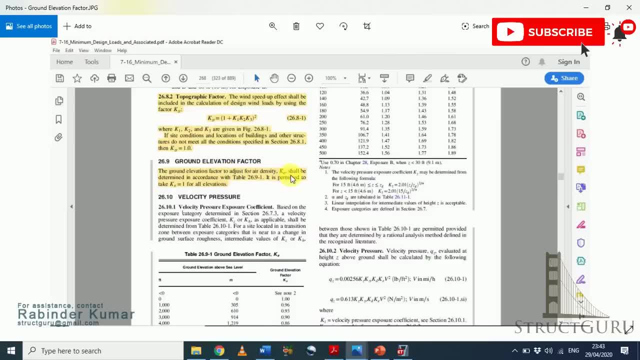 the ground elevation factor to adjust for air density, ke, shall be determined in accordance with table 226.9-1. it is permitted to take ke for all the elevation, for all the elevation. you can take this value or you can refer to this table in order to find the. 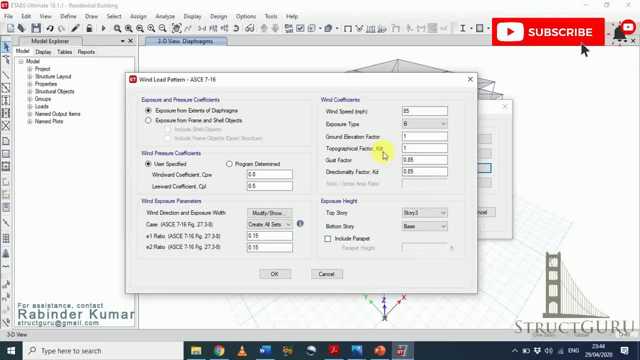 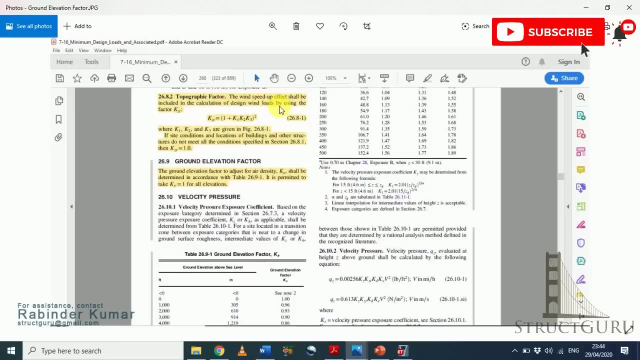 ground elevation factor. now we will see topographical factor. so topographical factor, it means your structures located in hilly areas or in plain areas. so again the code is specified. if site conditions and location of buildings and other structures do not meet all conditions- specialization, then k is taken as 1.0. then we will discuss gust factor. 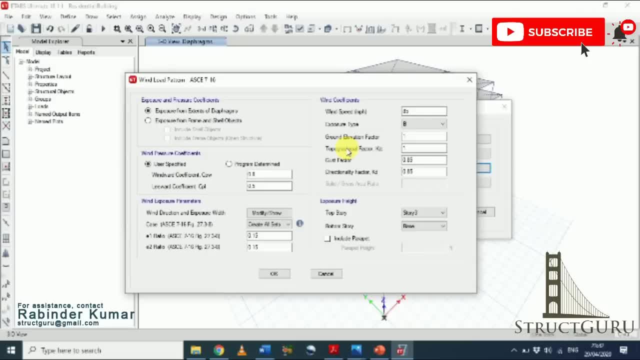 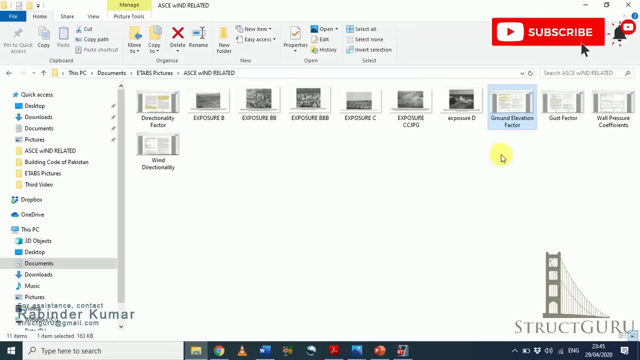 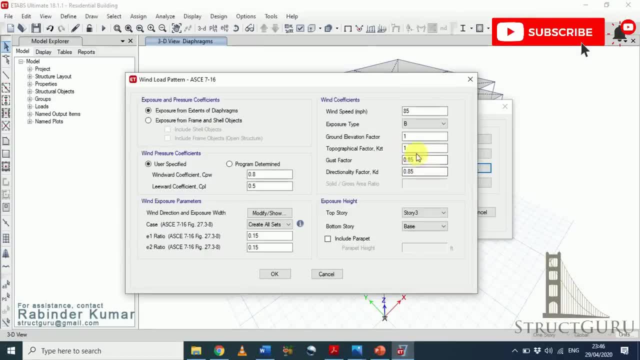 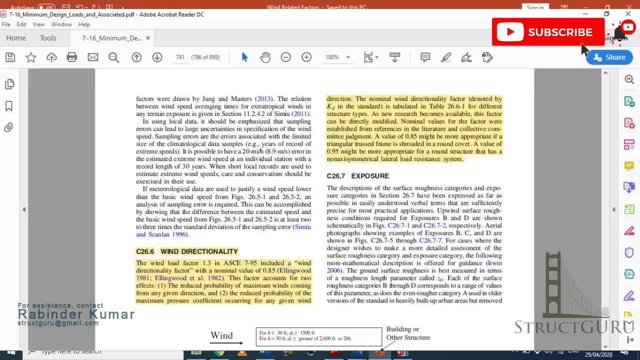 So you will see, by default it is 0.85. and the directionality factor, which accounts for the fact that the probability that the maximum wind may not impact the structural component or system in its weakest orientation- and this can mitigate over-conservatism by taking into 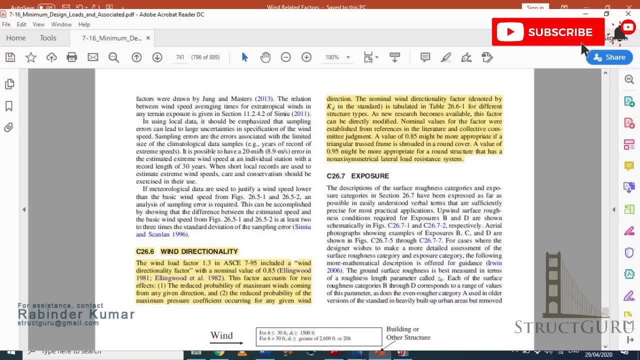 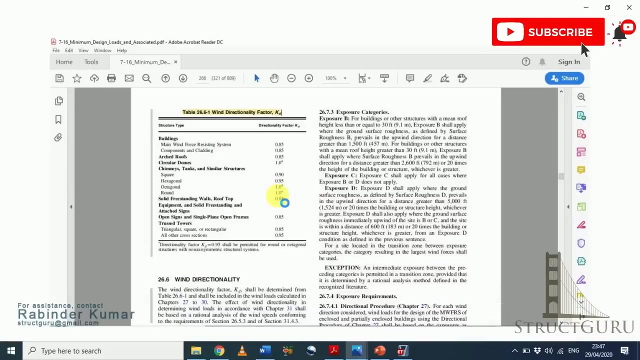 account the probability that the predominant extreme wind speed up may not coincide with least favorable orientation of the structural component. Again, if you refer to the code, the directionality factor is written as 0.85 earlier. or you can also refer to this table in order to specify the risk coefficient. so for buildings it. 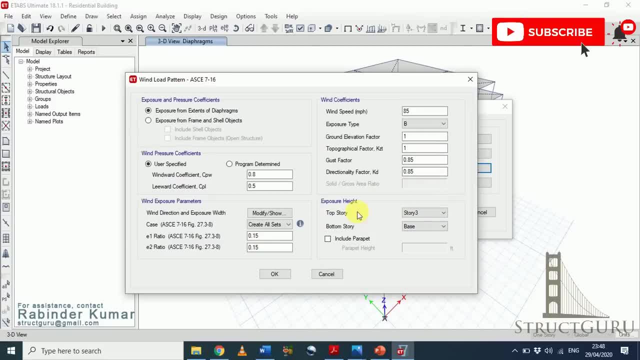 is 0.85, only in this form. Now, exposure height of building is obviously your building will face wind pressure from bottom to story 3, so just select base to story 3.. Now, as we have assigned the diagram, you can see automatically direction or the way the 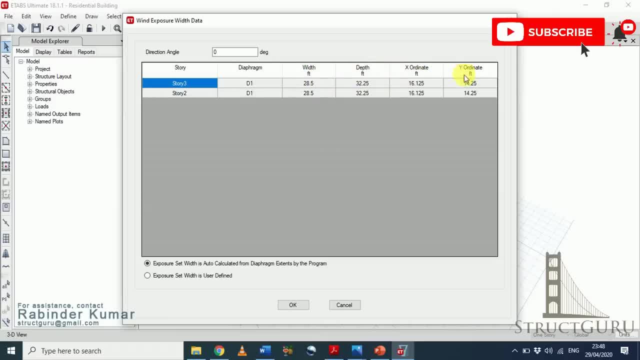 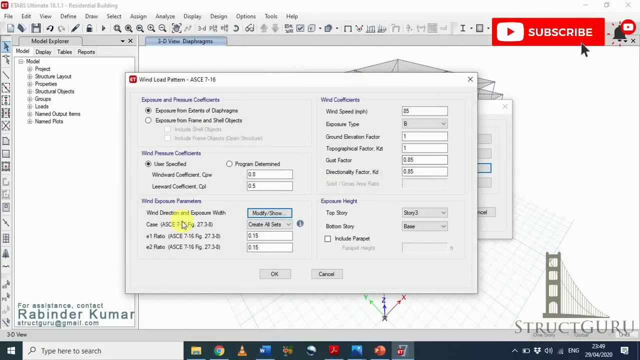 wind load will apply. the coordinates are calculated by the E-Tab. so direction 0 means wind load in X direction. So we have assigned the load in both directions. so for X direction you have to write 0 here, click ok. So these are the centricity ratios related to torsional cases. 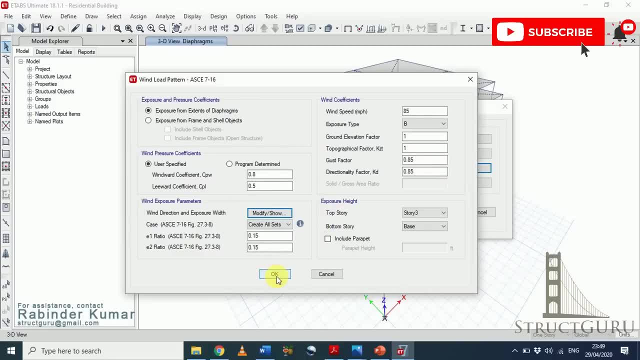 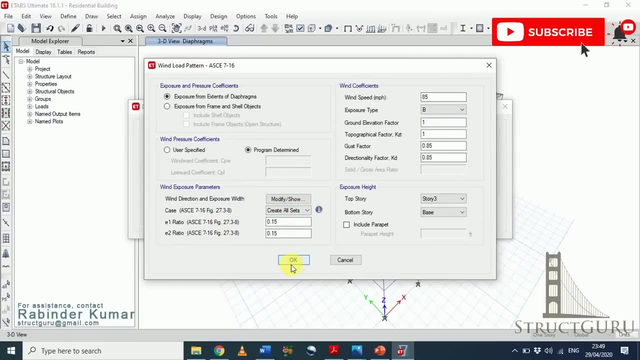 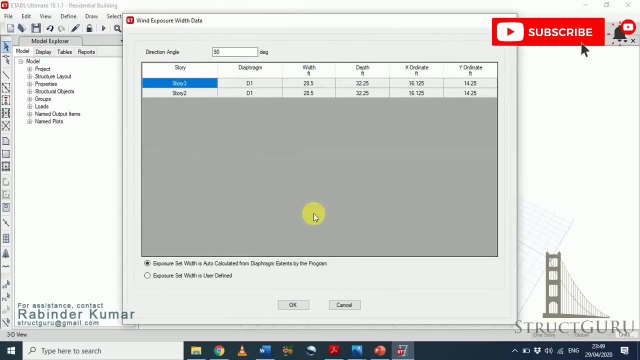 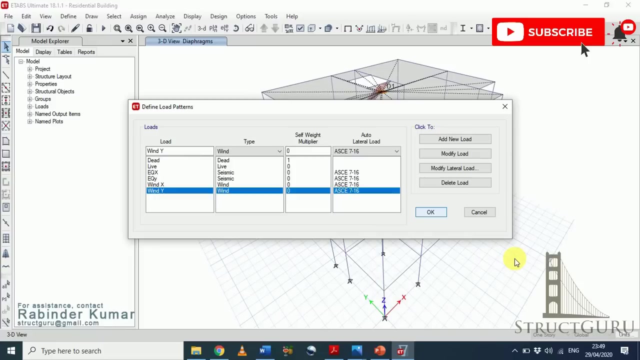 So in this case, you have to fill this form in order to define the wind load background. Similarly, you have to do you have to change all these values in Y direction as well, But you have to change the direction from this dialog box Now. put the direction as 90, so click ok, ok. 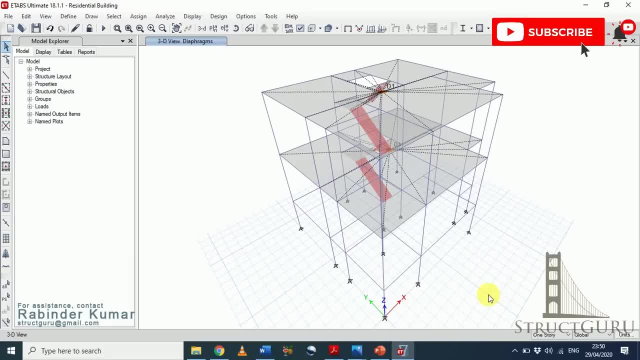 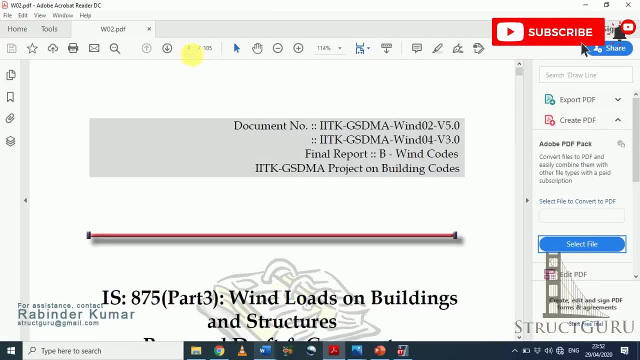 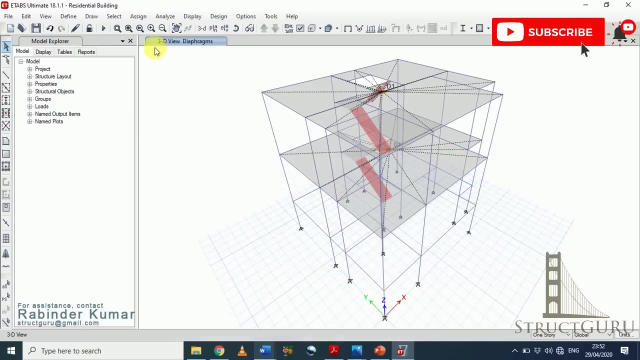 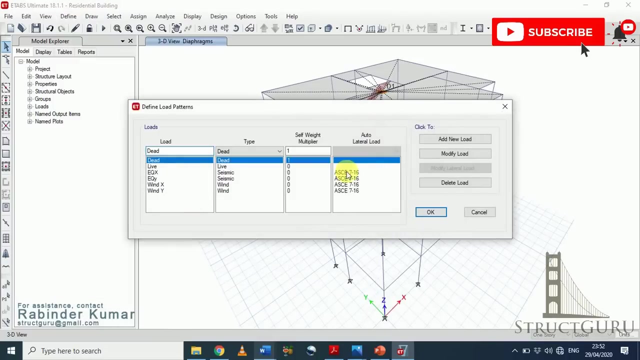 Now we will move to Indian codes and see how the wind loads are applied using Indian codes. So let's begin. Go to the Indian code book. So first we have to define the load pattern according to Indian standards. So go to the define menu, then click load pattern. 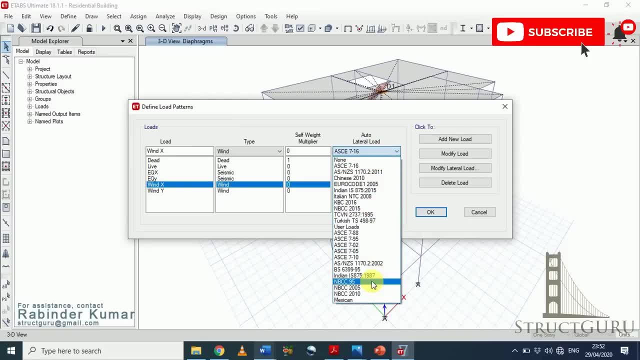 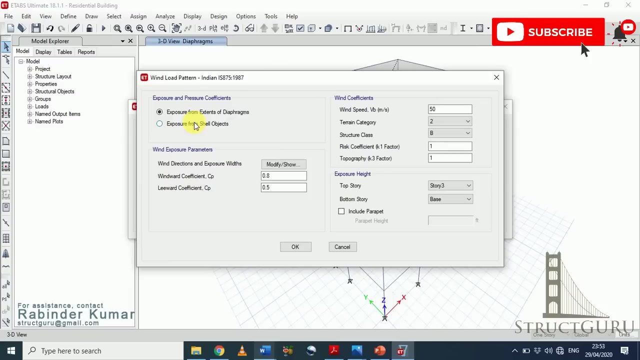 From here you just change to IS: 8751987.. Click modify. Similarly, you have to change it in Y direction: 8751987.. Click modify. it will do. Similarly. you can specify the wind pressure in two different ways. First, from exposure from extents or diaphragms and exposure from shell objects. 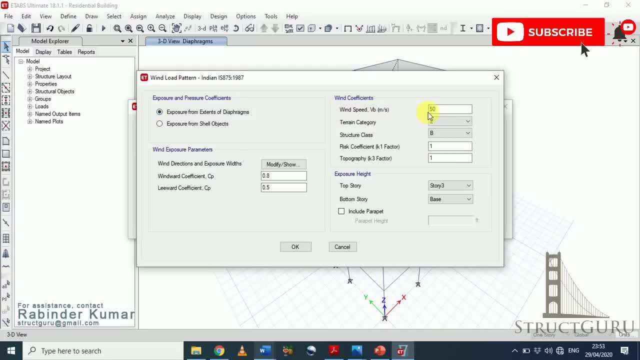 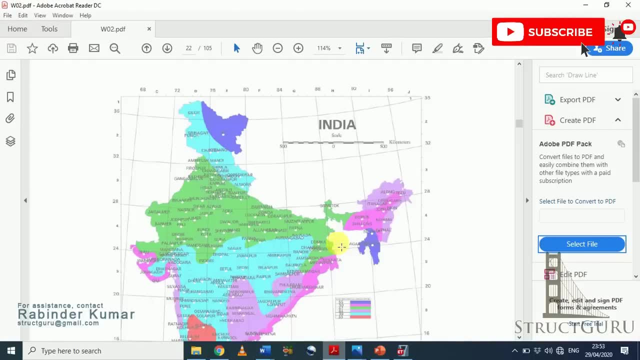 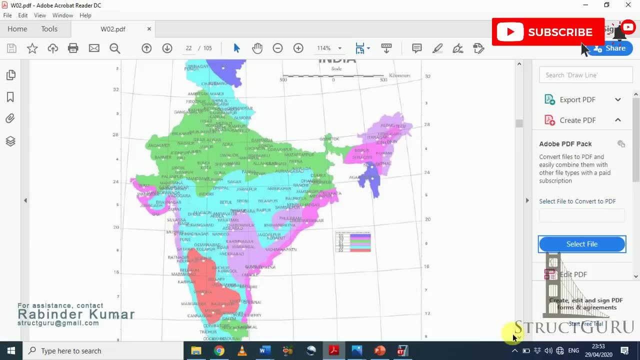 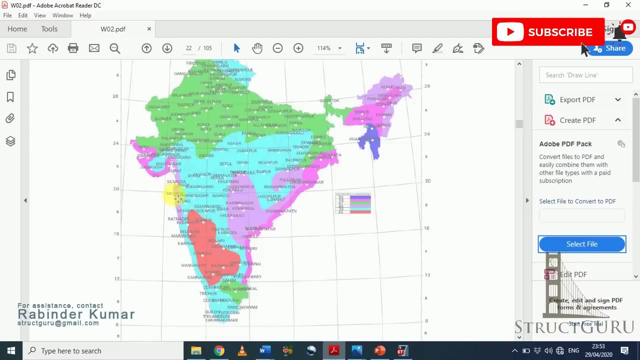 So first we will discuss the first option, Now, wind speed. So from code book you can specify the wind speed According to the area where the wind is coming from. For example, last time we discussed where structure lies in Bombay region, So Bombay is somewhere here in purple area. 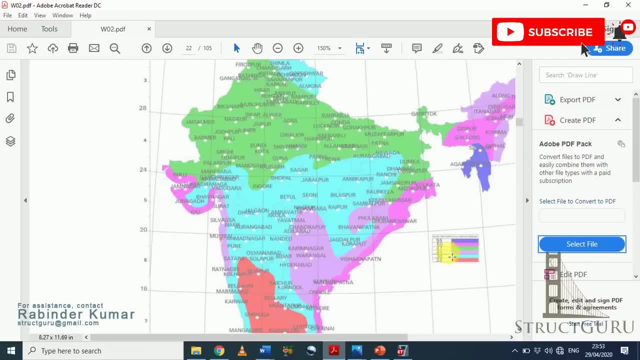 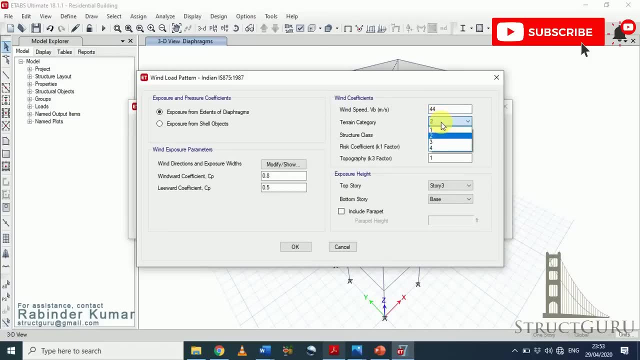 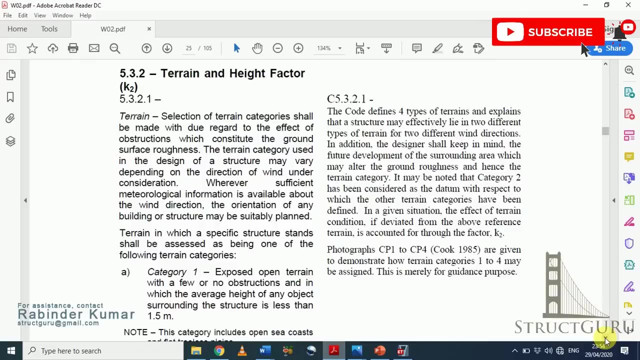 So for purple area the wind speed is 45, 44 MPH. So we will type 44 MPH. Now tearing category: similarly. So tearing categories specify whether your structure lies in sea areas, whether it is near to the obfuscation or it lies in a plain area. 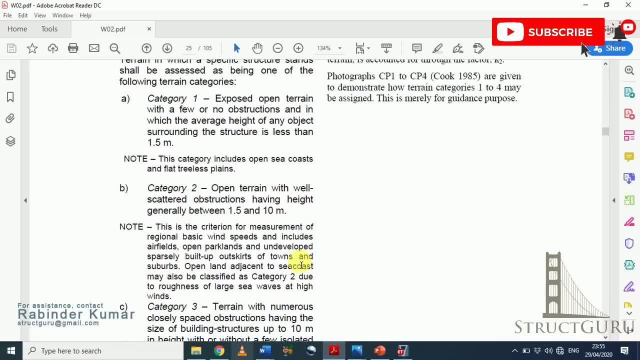 So from here you will define this criteria for the pavement of regional basic wind. It includes open land adjacent to the sea coast may also be classified as category 2.. So, for our case, we will choose category 2.. So, for our case, we will choose category 2.. 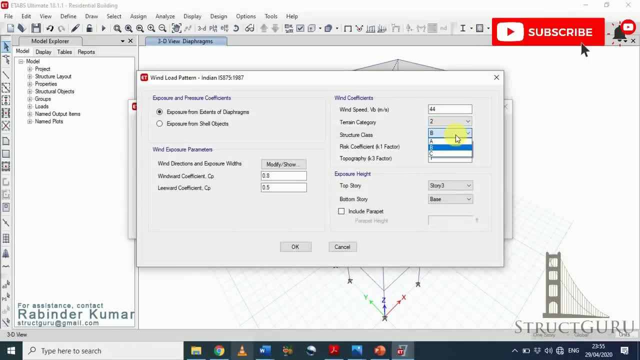 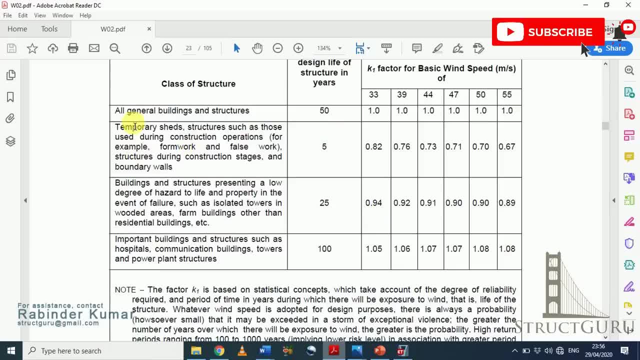 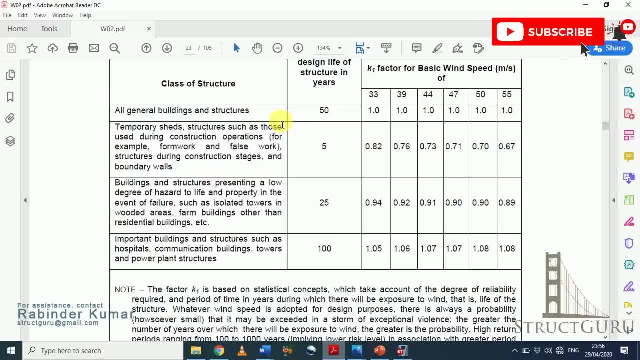 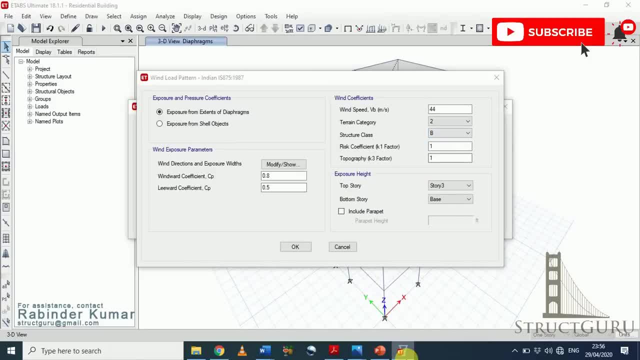 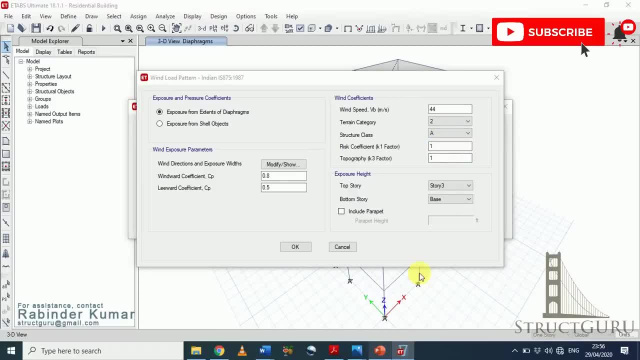 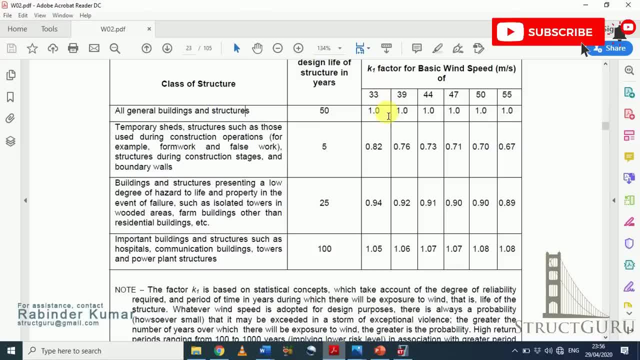 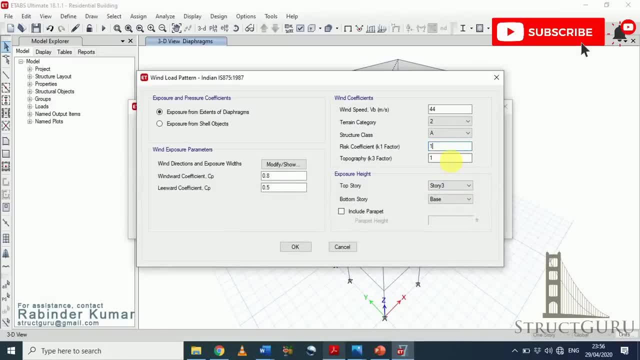 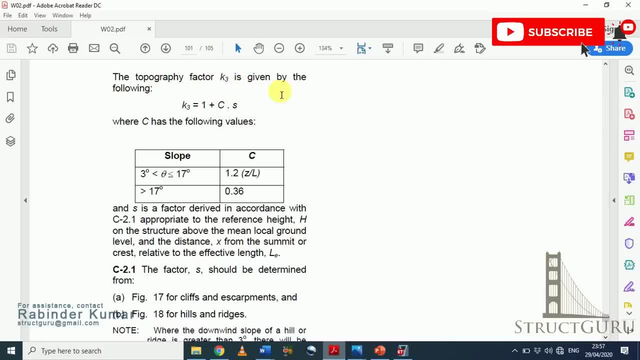 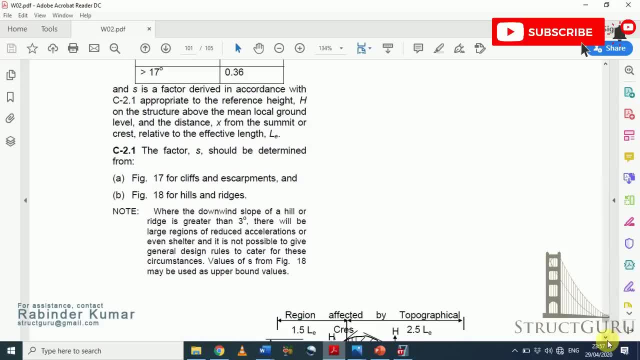 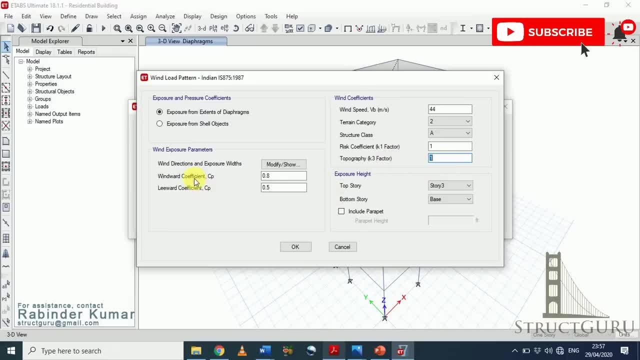 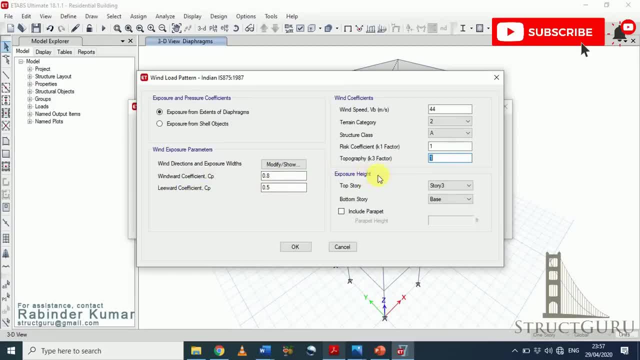 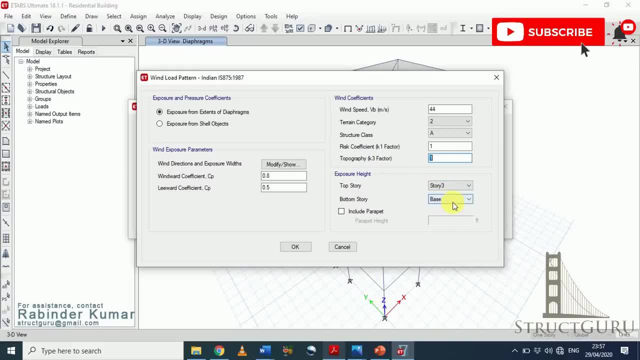 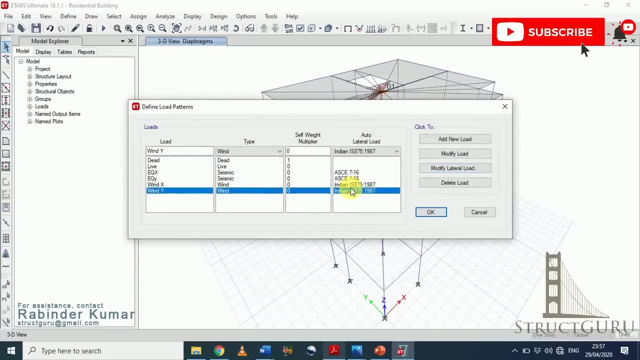 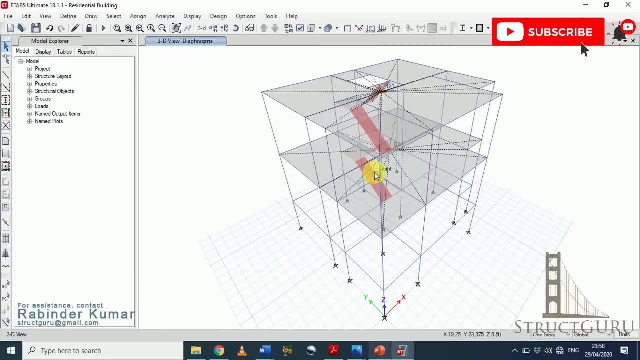 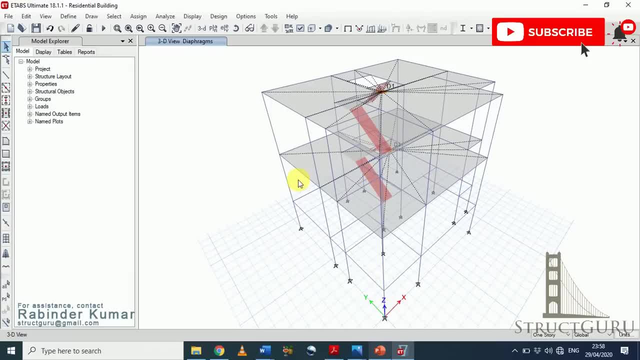 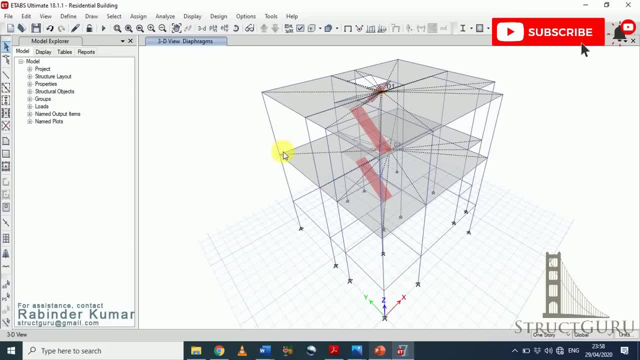 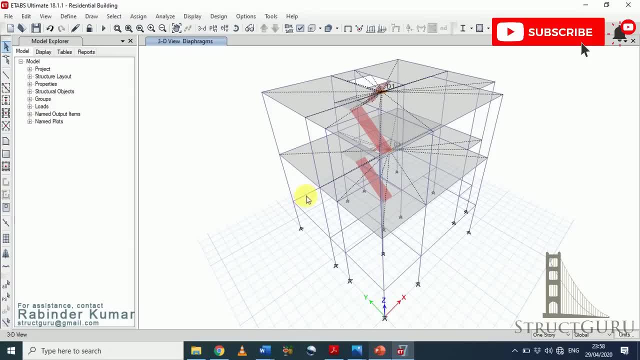 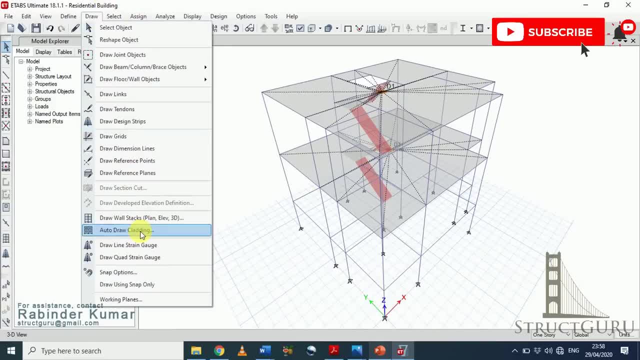 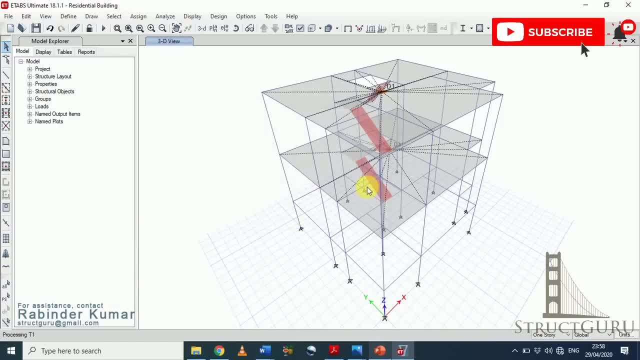 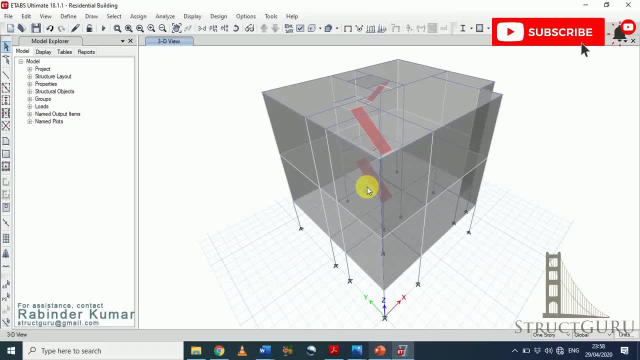 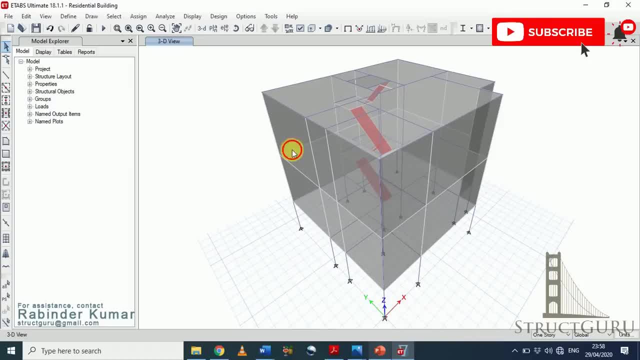 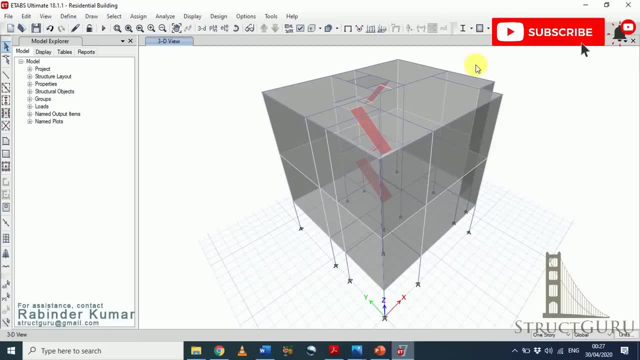 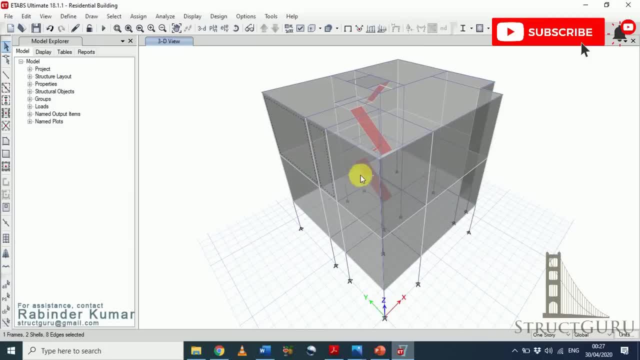 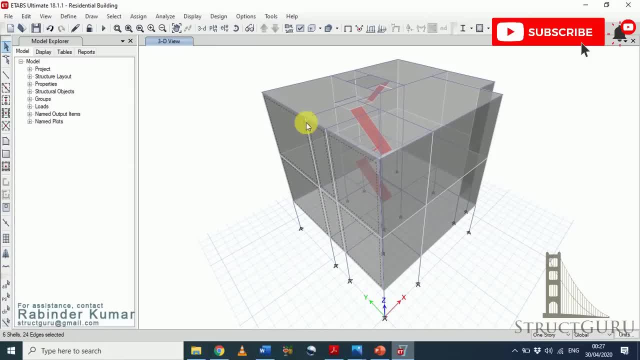 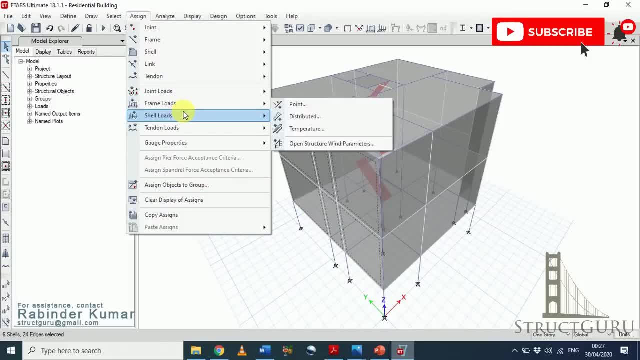 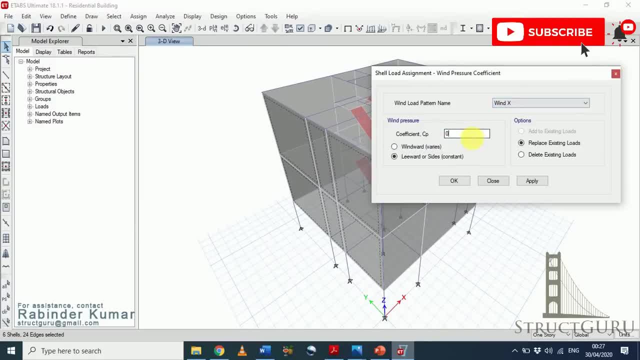 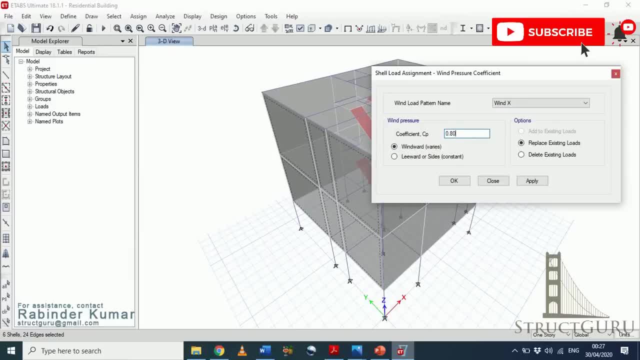 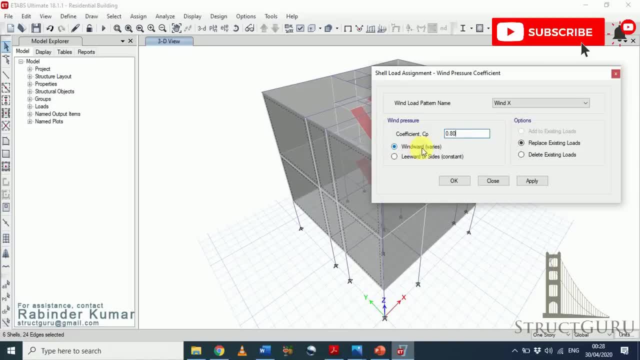 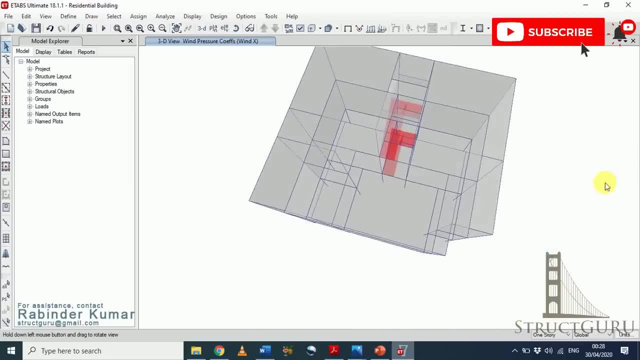 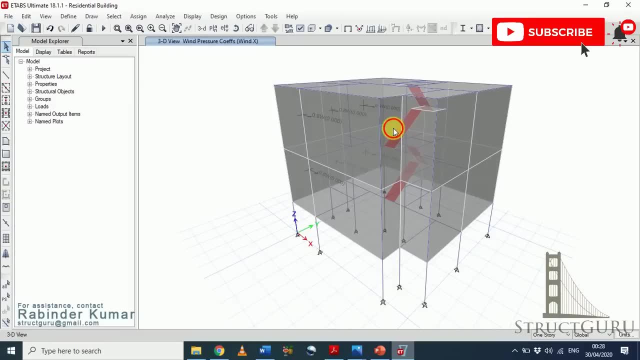 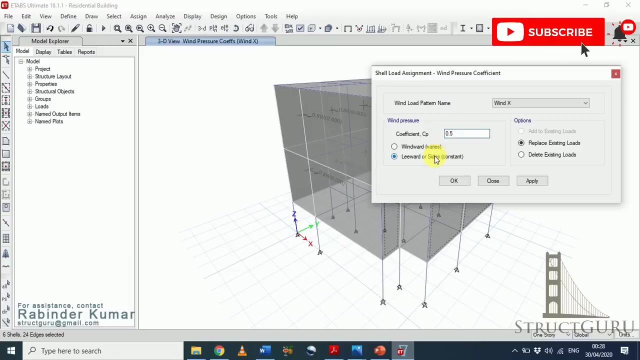 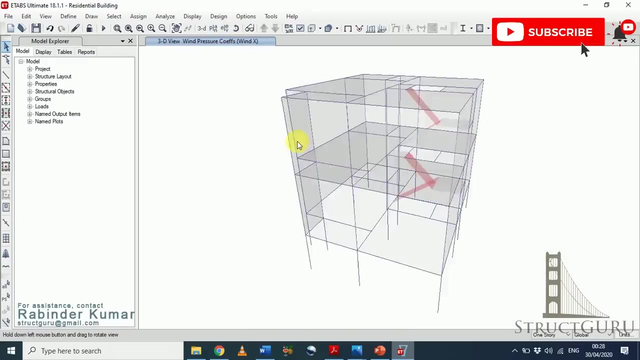 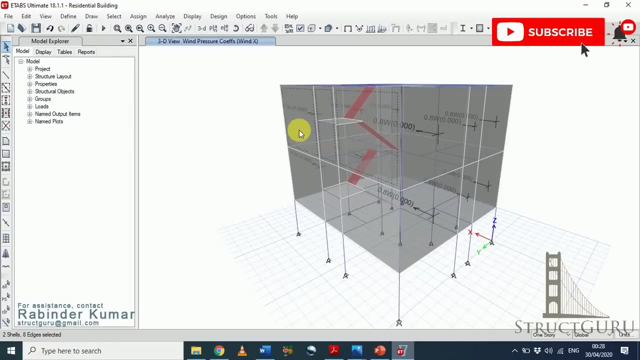 direction now leeward side. so leeward side will be. this is leeward side, this wall. so select the walls. go to assign menu share loads. wind pressure coefficients. put 0.5 on leeward side, click OK. similarly, you have to do the same in wire direction as well. for wire direction, select the walls. 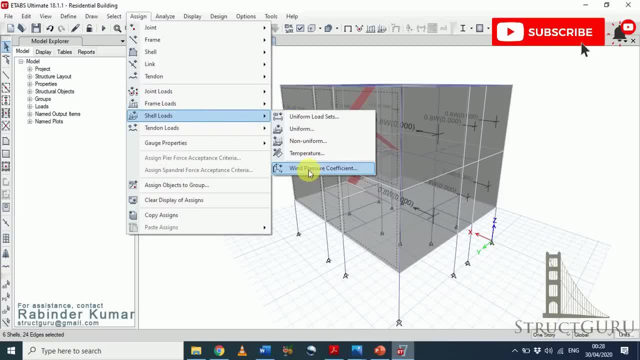 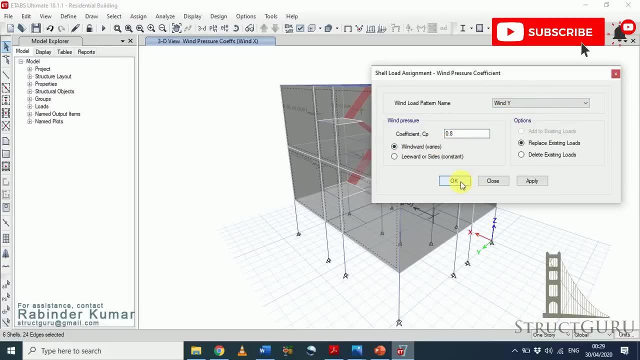 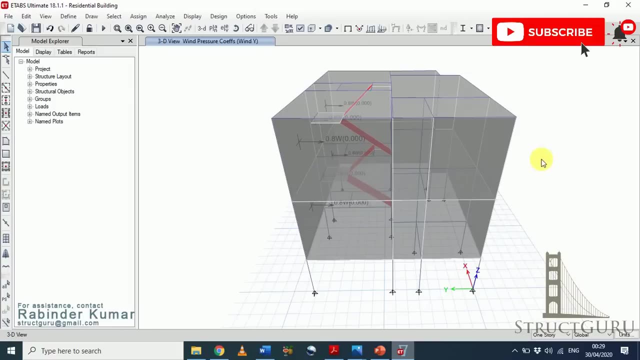 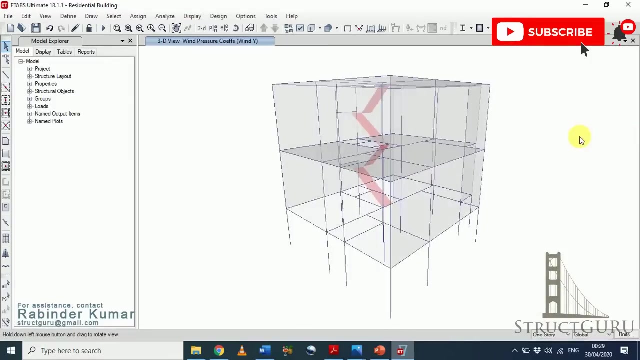 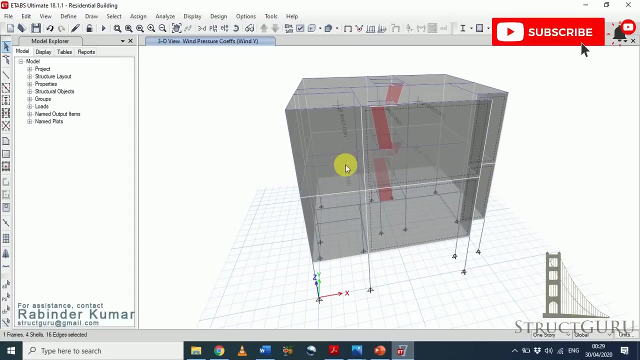 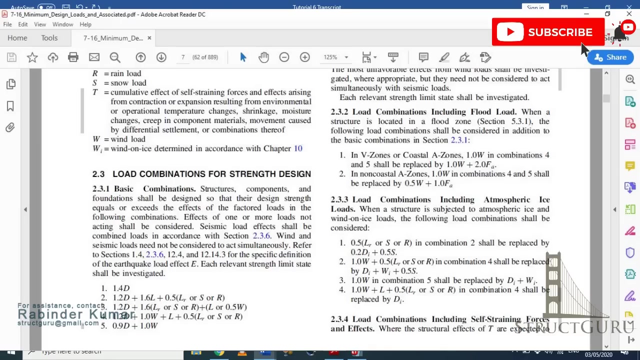 go to assign menu share loads- wind pressure coefficients 8 on windward side and click wire from drop down list ok, and do the same on front walls. go to assign menu share loads- wind pressure coefficients 2.5 on the website, click. That's Now let's begin how load combinations are defined. So first refer the code book. 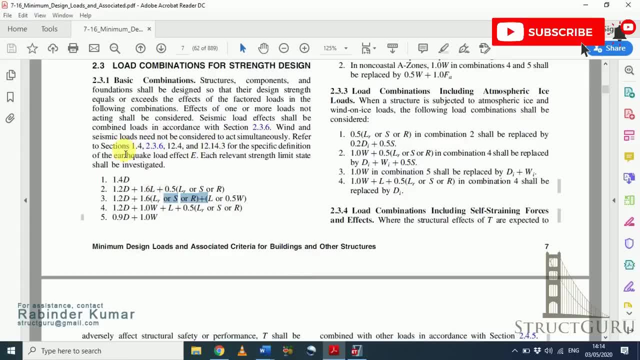 So the ACI ASE 716 Has defined five basic load combinations for strength design. so we have to follow these and we Follow these equations and we have to generate many Load combination considering the load Patterns we have defined in our ETABS model. So there are two ways to do it: go to your ETABS model. 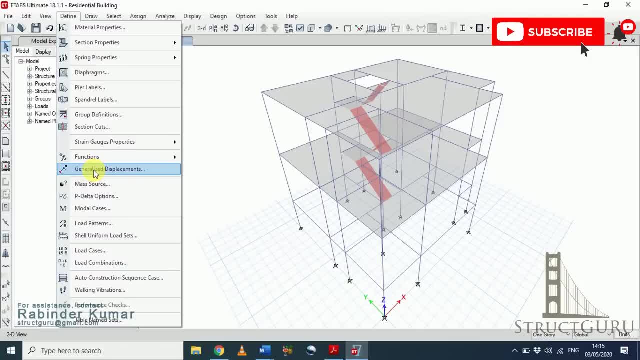 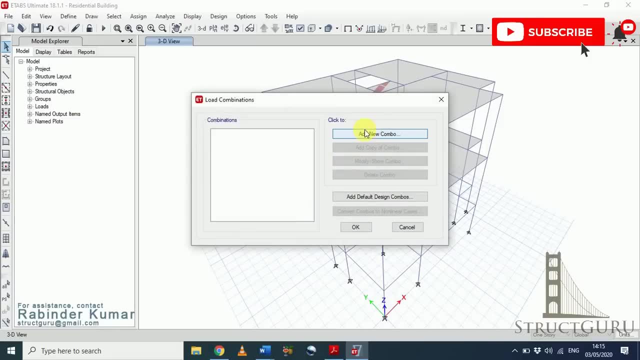 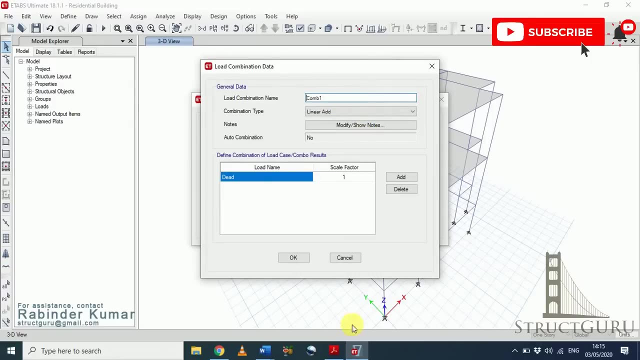 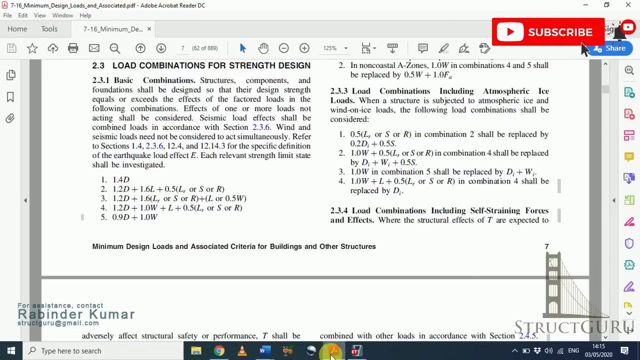 Click to the define menu, So here you will see load combinations. Click load combinations. There is add new combo. So click add new combo. You can name it according. accordingly, for example, The usual practice is if you are generating load combination using first equation. So what will you do? 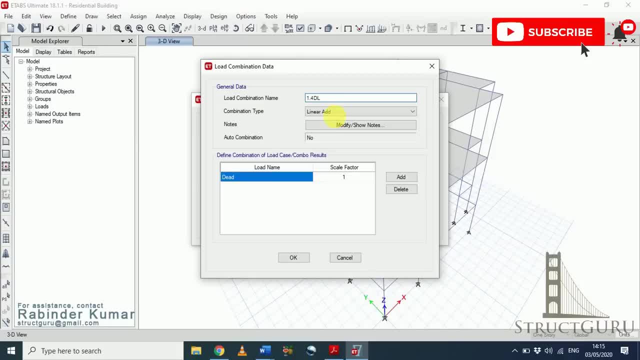 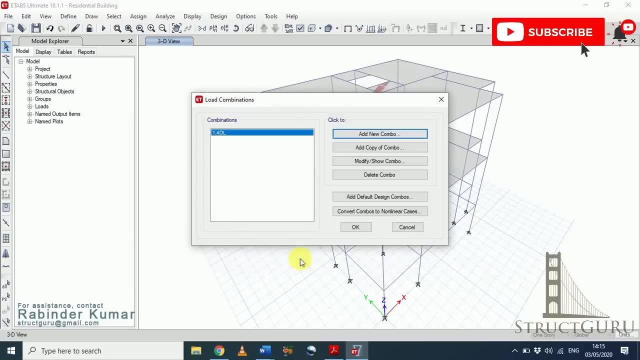 1.4 dead load. So dead skill factor, you have to give 1.4 click. Okay, so we have successfully defined a load combination. So we have successfully defined a load combination. similarly, if you want to add a new combination, refer code book. so the second equation is 1.2. 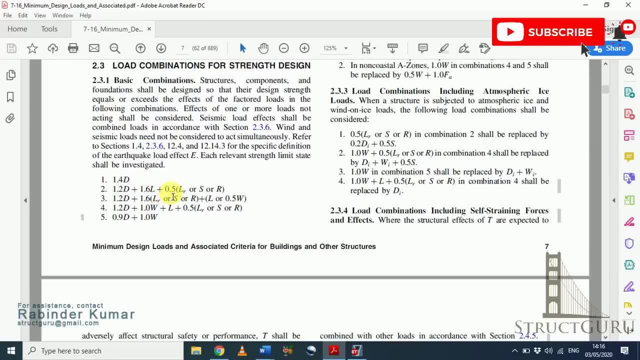 of dead load plus 1.6 of live load, plus 0.5 of roof live load or snow load or rain load. as i have not considered roof life load, i have just added the default value of live load in all this lab, so i will use mine up to these two mathematical terms. so 1.2 of dead load plus 1.6 of live load. 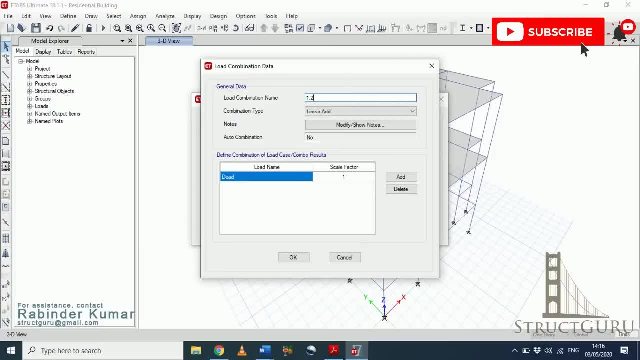 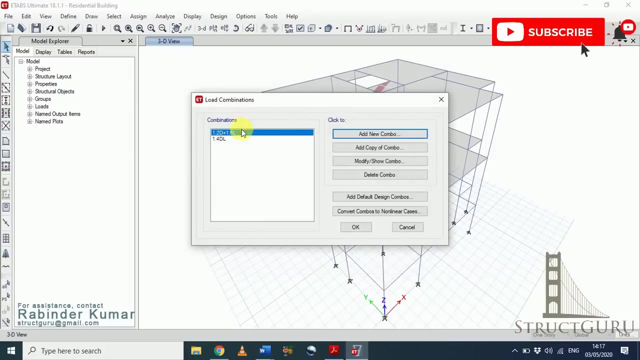 so click add new combination. name it 1.2 of dead load plus 1.6 of live load. similarly, combination type should be linear and dead load is 1.2. click add. from here you change the load type. click to live and 1.6 of live load, click ok. 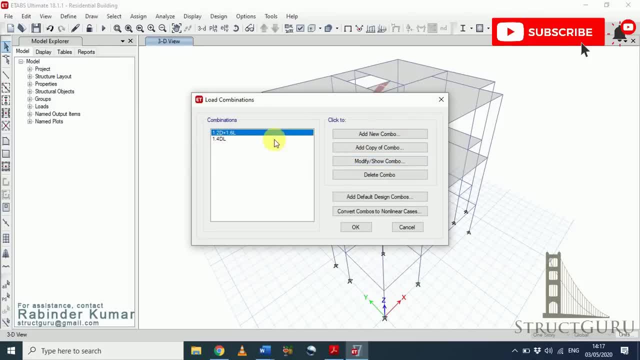 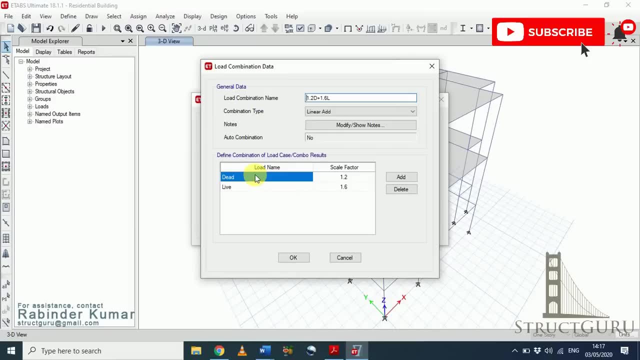 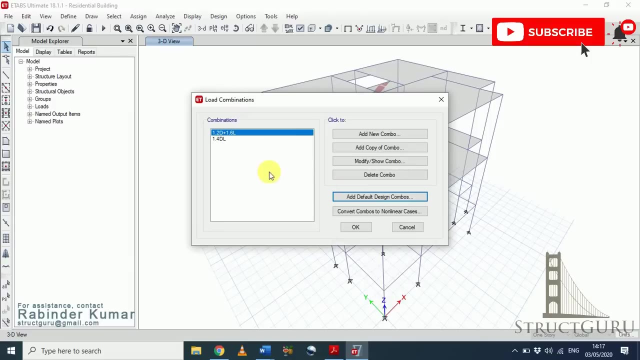 if you want to see the load combinations, click and click modify. so here we have successfully defined a combination with 1.2 skill factor of dead load and 1.6 skill factor of live load. so this is a manual way to define the load combination. there is also another way. 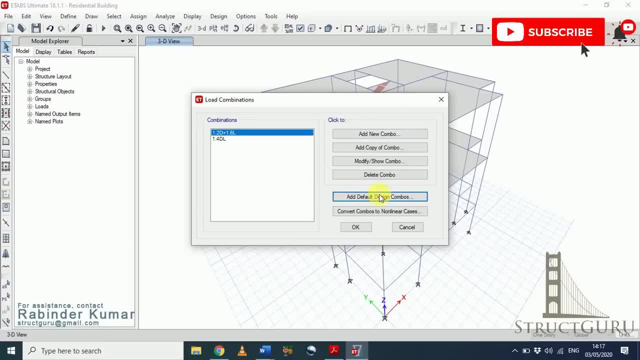 to define load combination. so in this dialog box you can see eight default design combos. since we are using as a ci318 building code which takes all the loads and loading criteria from asce716. so etab by default knows according to your load veterans what kind of load combinations should be. so if you just click eight, 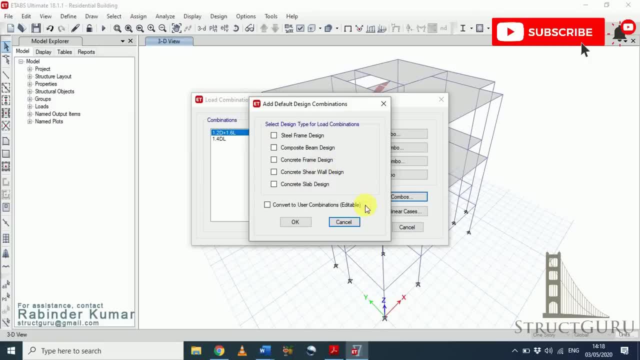 default load combinations. so a dialog box will appear. so there will be six checklists and from this six checklist you have to choose one or two according to your design type. for example, if we are designing for concrete frame design, so we have to check this dialog box. so, concrete frame design. 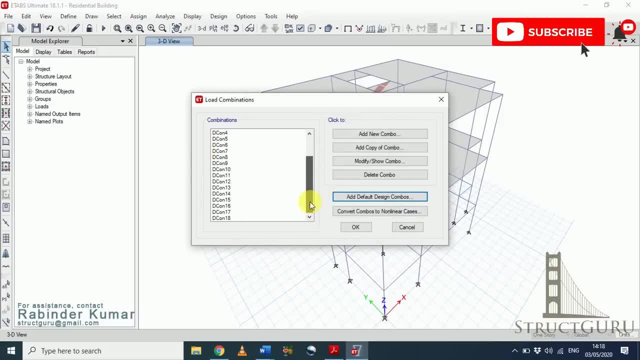 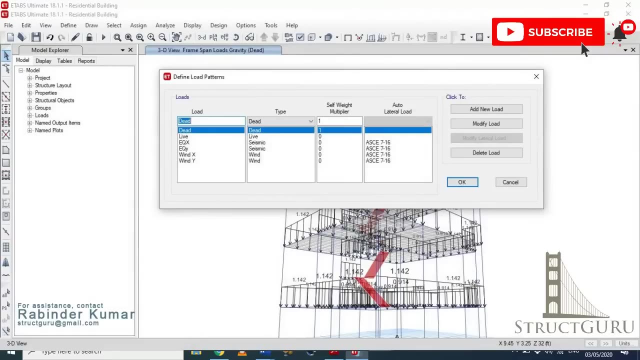 click ok. so, as you can see, etabs have defined almost, i think, 19 load combination based on our load patterns. so let me remind you we have to use six load patterns: dead loads, live load, earthquake in x direction, earthquake in y directions, earthquake wind load in x direction and one load in y. 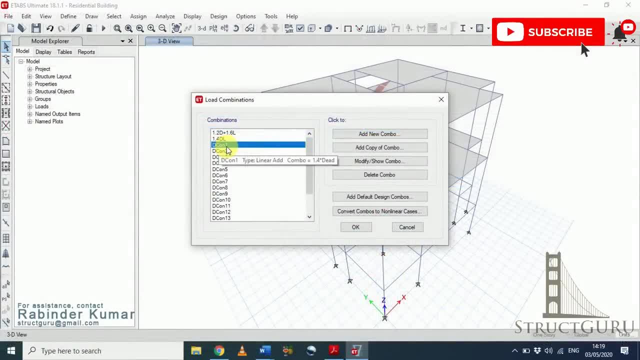 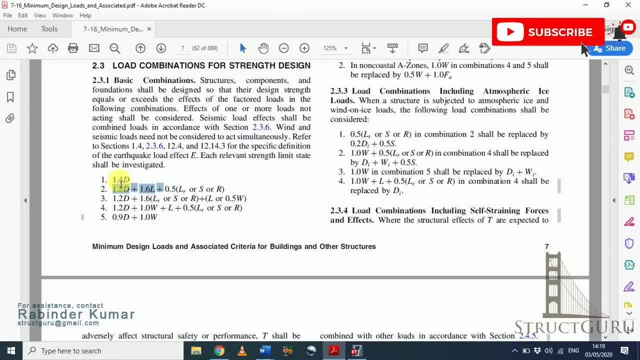 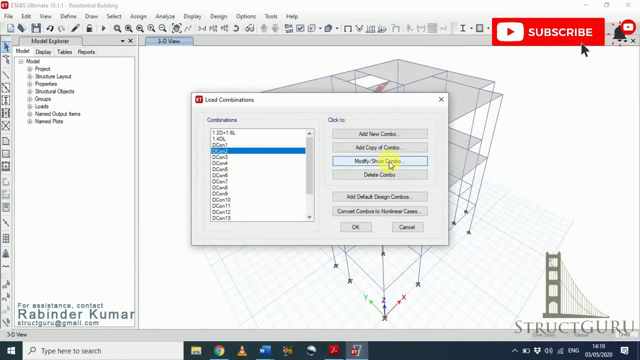 direction. so if you open this combination, default combination, which is generated by etabs, you will see 1.4 of dead load, which is given in the basic equation of code book. similarly, if you open default combination 2, so it will be 1.2 of dead load and 1.6 of live load, as i said earlier. 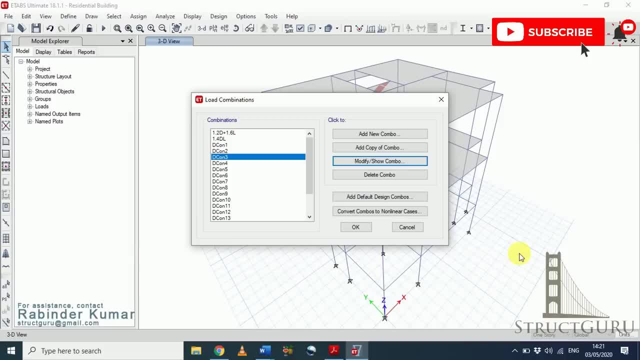 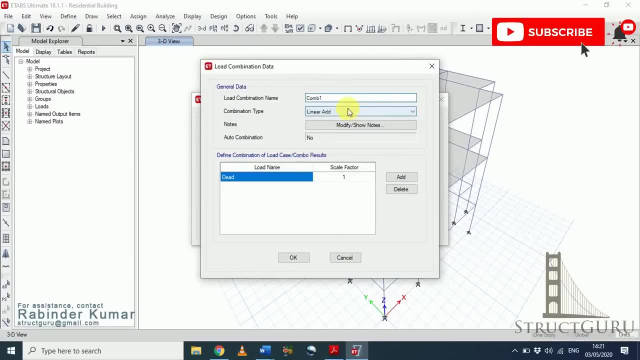 in our profession sometimes we have to increase the load factors which are given in our code book. so i will recommend you you define combinations. name it as my combo, so where you increase the del loaded by 1.4 live load as 1.8. earthquake load x 1. earthquake load in y direction is 1. 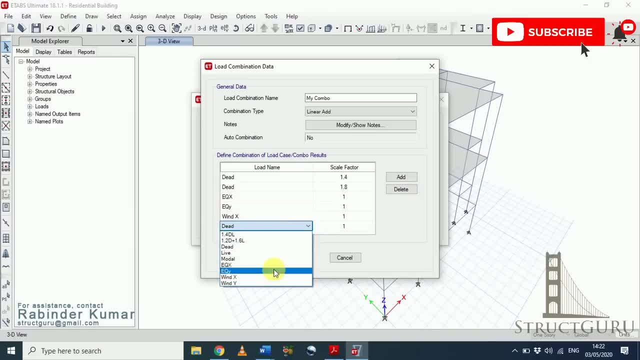 wind load in y direction is 1 and wind load in y direction is 1. you can also change these values. so if you put here live, okay, make it 2.. so this is my combination. that means i will design a building using this combination, which somehow overestimates the design. 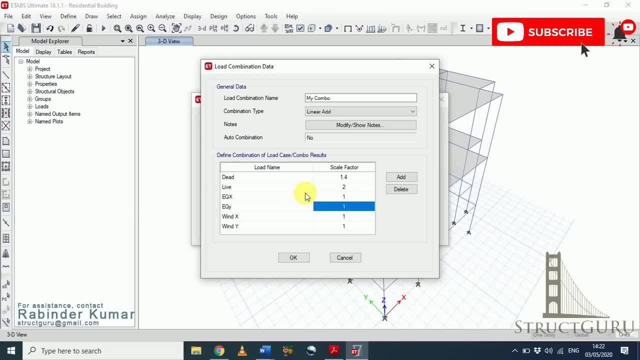 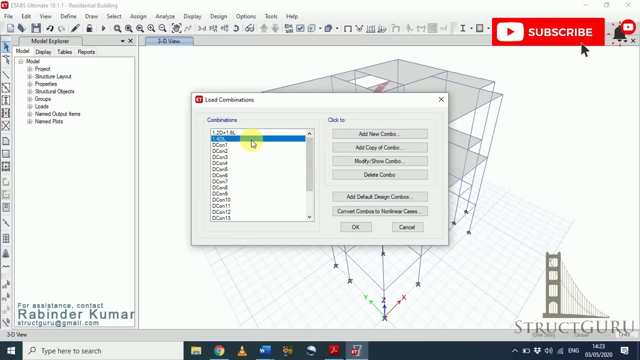 but we will be on the safer side, and this practice is recommended for the beginners who have just started their consultancy. so it's better to go on safe side always. so click OK, I'm going to delete these two combinations. of course, we will use the default combinations which are generated by etabs for over. 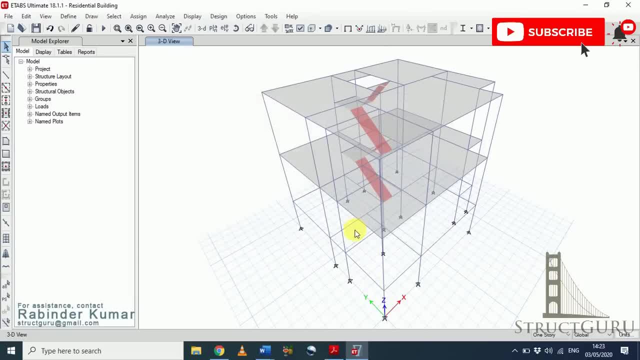 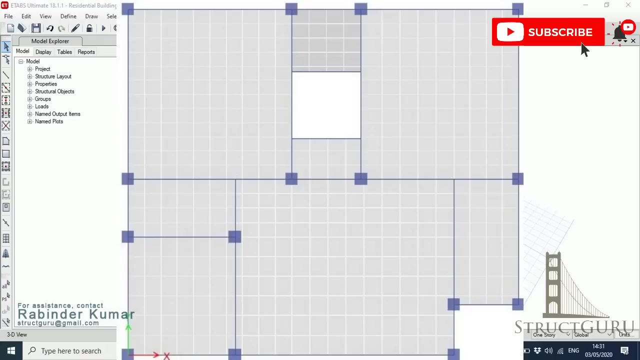 design, click OK. this is the simple way of defining the load combinations. now let's move to our second topic and which we will sign: the mashing service. left now the question is why mashing is done so mashing is done to break a large element, which is slave in our case, into number of small elements to develop a 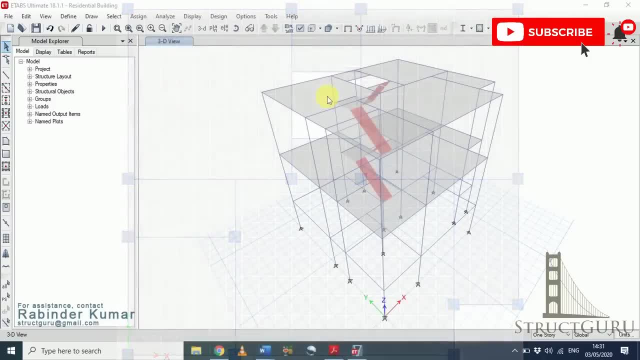 precise, correct and uniform load distribution pattern from slaves to beam. this is very important to do during modeling of structure. so there are two ways to do the mashing of slave. number one is manual method and number second is auto mashing method. in usual practice auto mashing method is widely adopted. but first I will start from the manual. 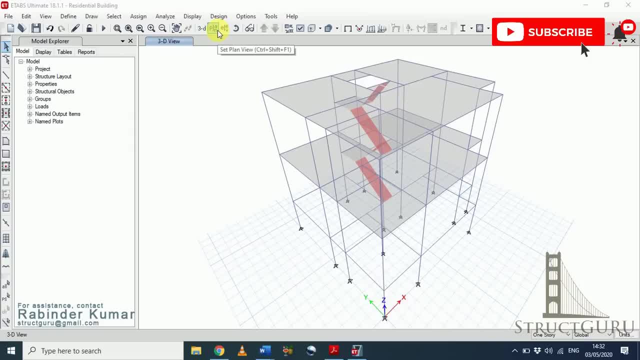 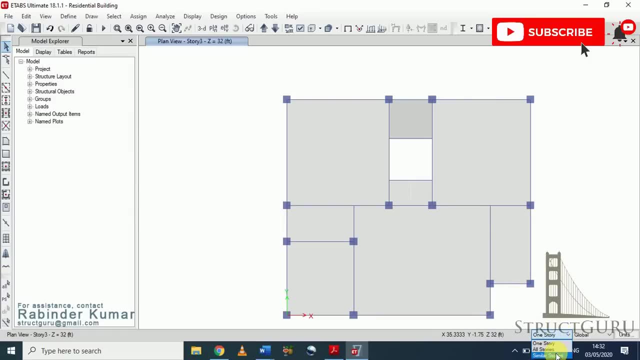 mashing method and then we will switch to the auto mashing method. now switch to the plan mode. from here you can also refer to all the stories, because all most of our slaves are uniform in both stories: kept at the same places. now to do the manual. 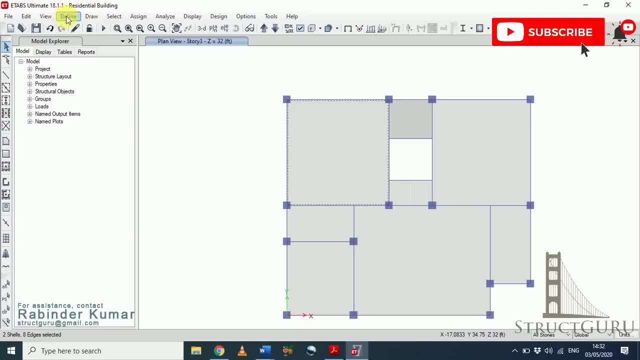 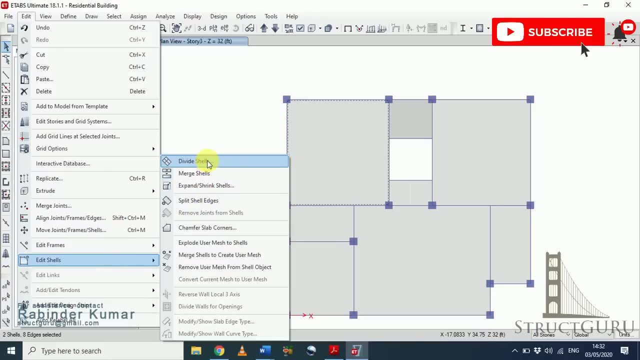 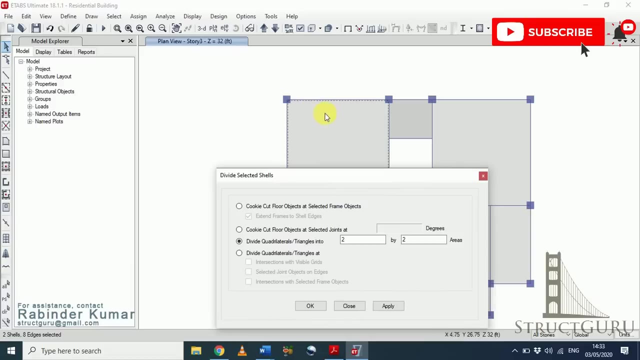 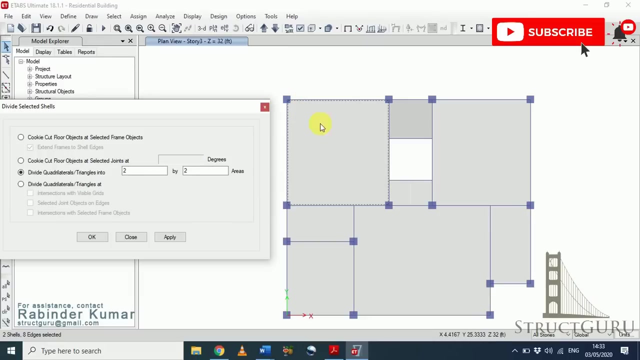 mashing. first you have to select the object, select the slab, go to edit menu, edit shells. now you have to divide shells. so from here you have to do now you have to divide into, into in number of squares. for example, if I want to divide into ten pieces in x-direction and twelve 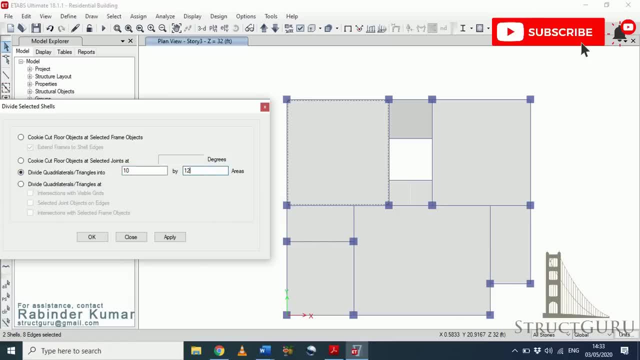 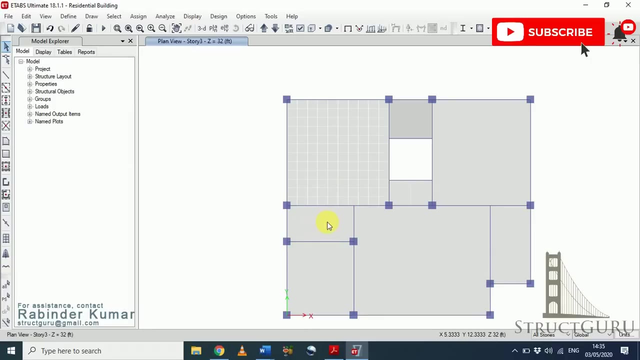 pieces in y-direction. so I will just put the ten into twelve. click ok. so in this way, we have to divide the shell off objects into number of squares. now, from here, we have to also divide this slab into number of square pieces, following the same continuity. for this, what we 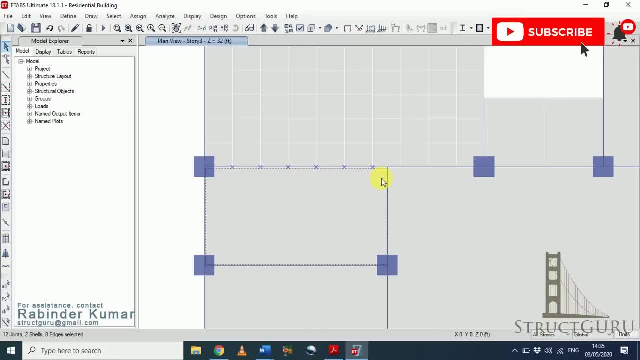 have to do? we have to select this object and also select these points. go to edit menu, click edit shields. divide chains. so from this option we have to choose selected joint objects on edges, click over. as you can see, the line is in a continuous manner. now you have to divide these shields in Y direction into number. 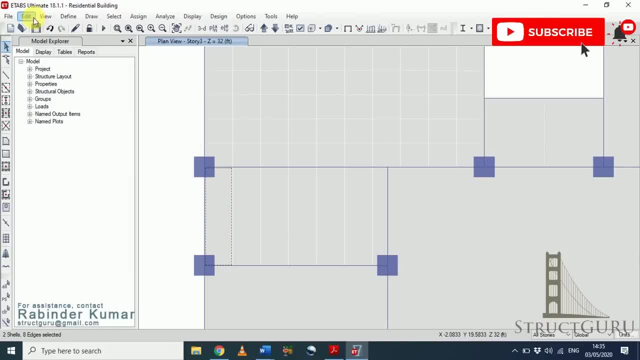 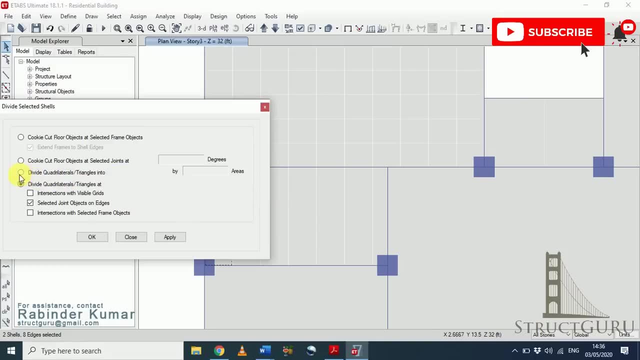 of squares. for example, I'm going to divide it into five squares. go to edit menu, edit shields, divide shield. now you have to choose this option. so from here we have to select this object and also select the joint object. so from here, we have to select this object and also select the joint object. 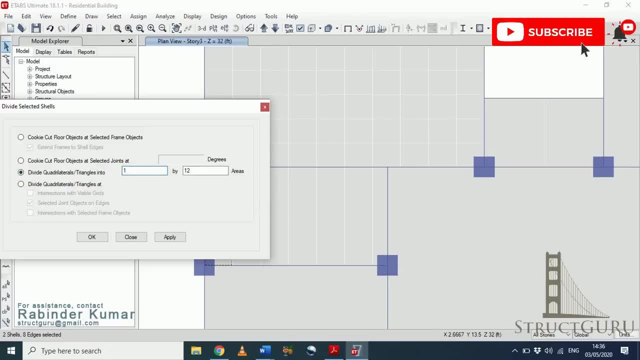 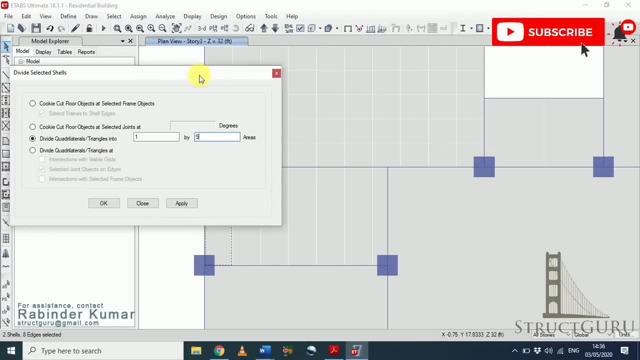 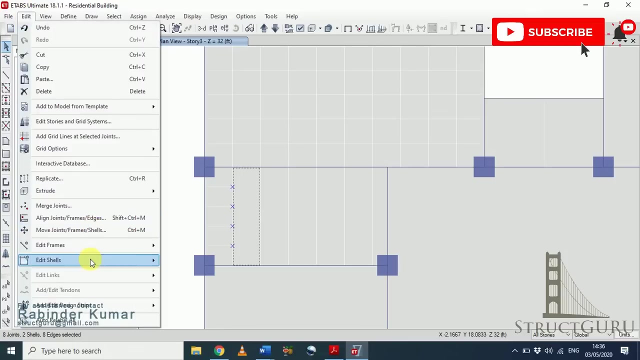 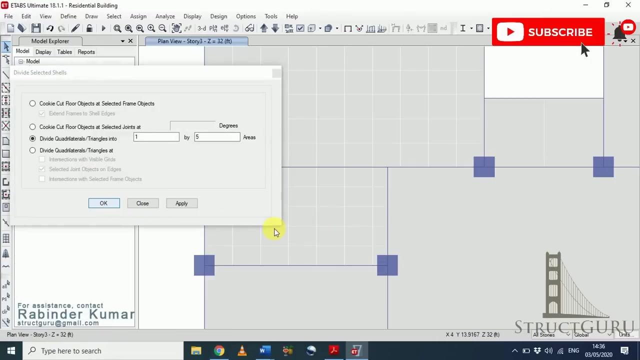 so I don't want any. this division in X direction, so I will put one. so I want five divisions in my direction. put five and click OK. now, similarly, select these corners and the following shield: go to edit menu or choose all the shields. added shields. similarly, one by five, click OK. so in this way we have to divide. 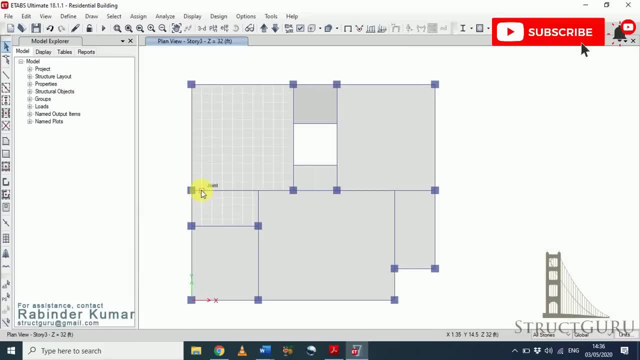 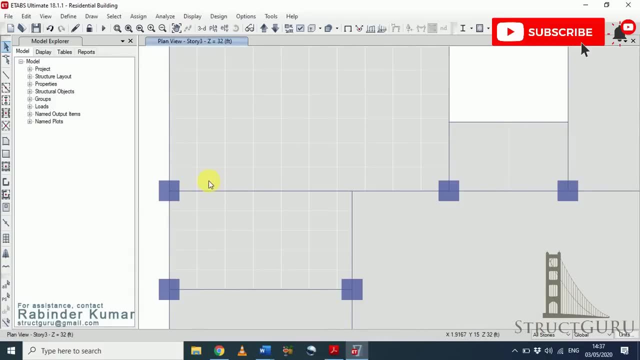 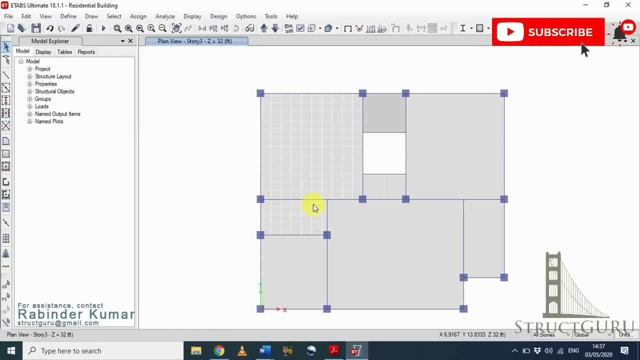 the shell objects into a number of squares. following that, following the continuity of the slabs, because the load will be transferred from this slab and this slab. in this way, we have to divide the shells. so this is the manual method of mashing the slabs. now we will move to the auto mashing. 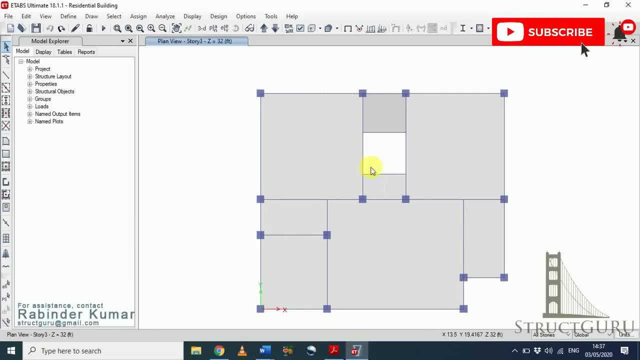 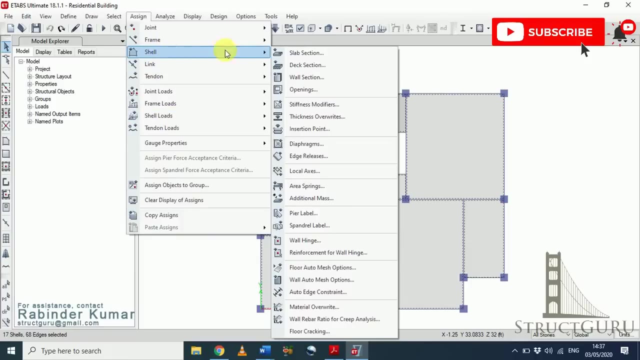 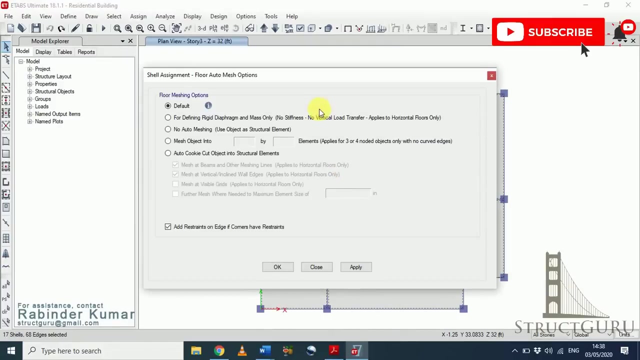 method. so for auto mashing method, what you have to do? you have to select all the slabs, go to assign menu shell. from shell, you have to choose floor auto mesh options. okay, so if you don't mesh, if you forget to mesh, and if you run the analysis, 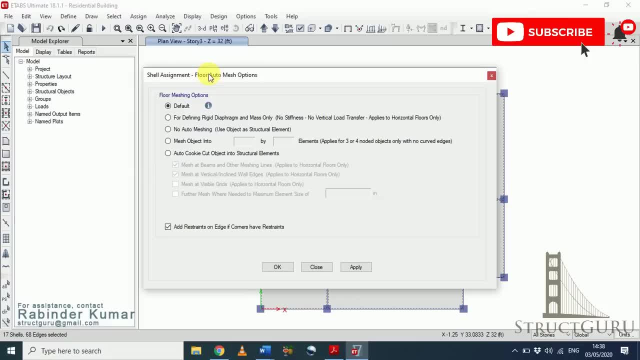 ETABS by default will divide the slab into number of square sections. so in this way you can measure the size of the slab to get the maximum size of the slab. so it's better you always do it by yourself. so now you have to click auto cookie-cut object from structural elements. so mesh at visible grids- no I. 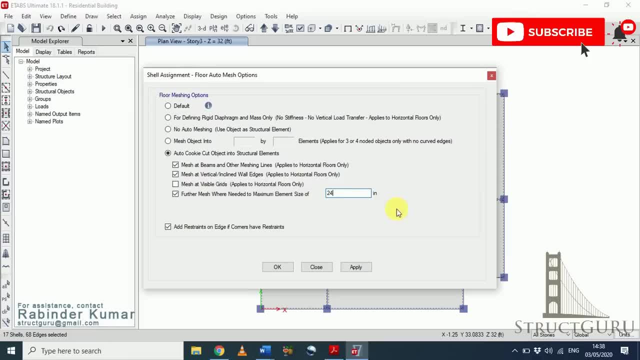 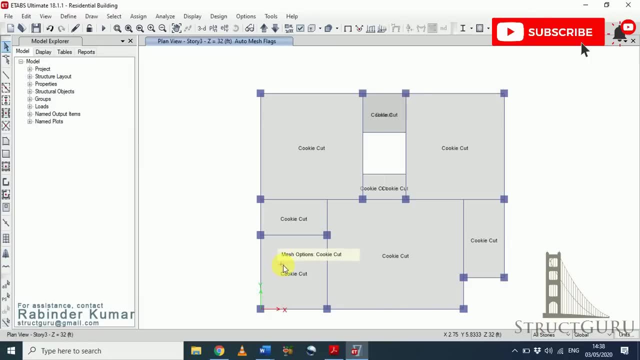 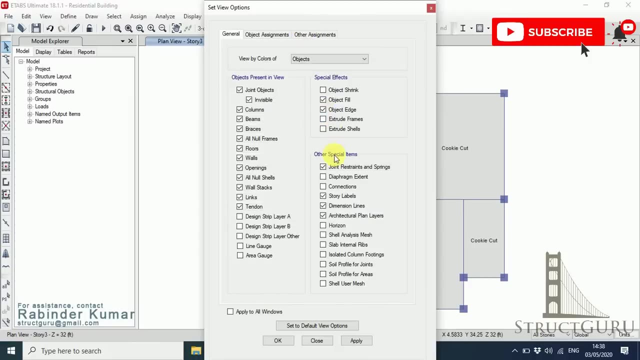 don't want to mesh at the visible grids, so further mesh we are needed to the maximum element size. you have to check this option. reduce this size, make it 24 and click apply to see the meshing go to set display option. from here you check she'll. 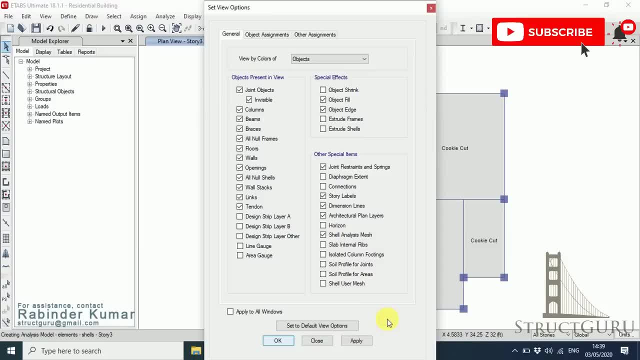 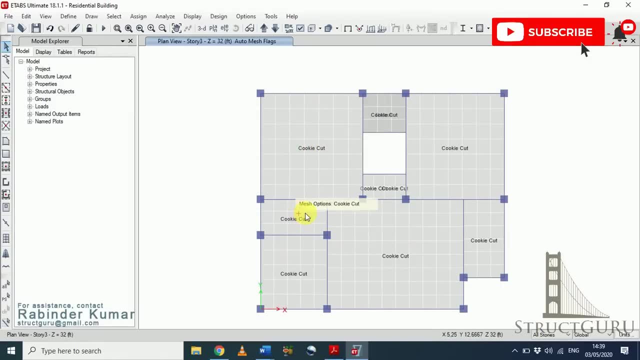 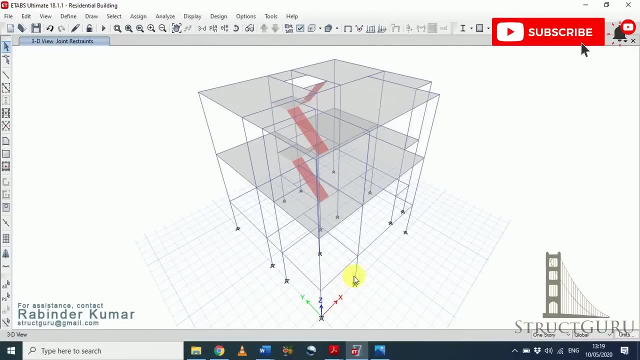 analysis mesh and click OK. so, as you can see, the meshing has been done automatically. for all this, before we go for analysis, we will give fixed support condition to the structure. to do so, go to assign menu. first we have to switch the structure into the plan. 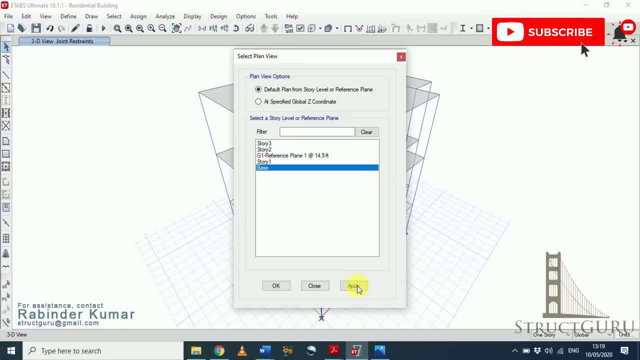 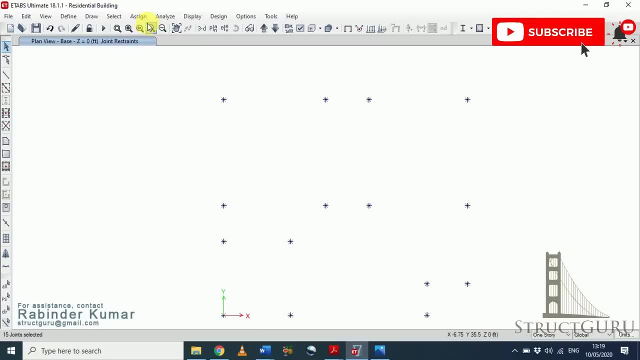 mode. from from plan mode, click on base, select all the joints. go to assign select joint and from here you have to select the restraints, as a base is always fixed in the ground. so we will choose this icon in order to make pin support to your support conditions. you can click on this icon similarly for 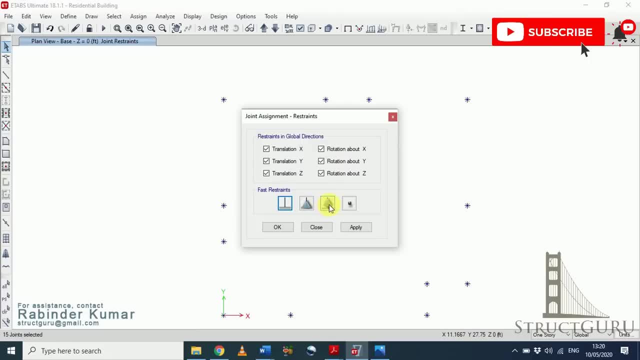 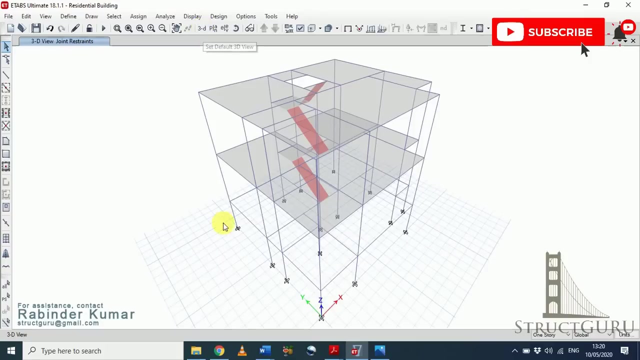 roller support. you have to go to click this icon and you can also select your support conditions manually according to the degree of freedom which you want to restrict. for our case, we just want to click fix support, to click on this icon and hit apply. switch to the 3d venue. as you can see, our support I can change is from: 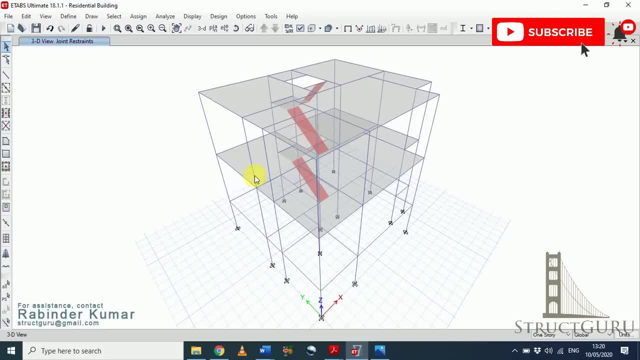 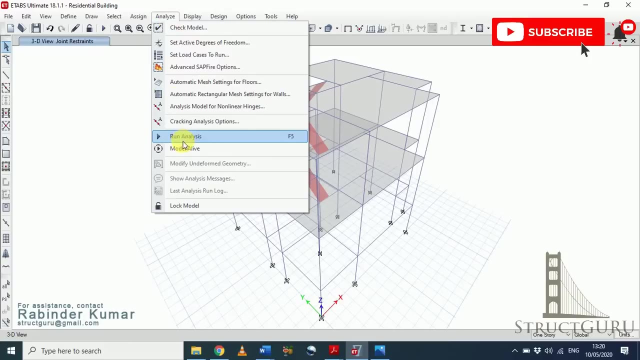 pin support to fix a hole. in order to analyze the structure, go and click this button, or you can also press a five from your keyboard. or you can also analyze your model by clicking the analyze and then click run analysis. but normally we go and clickати and run analysis, or 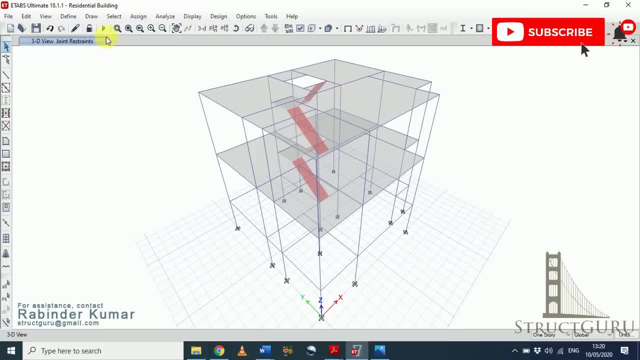 then click run analysis. but normally we go and click differ and that takie to any. click this play button for the analysis of the structure, so click. so here you will see, within fraction of seconds our model will be analyzed. if we have gone for hand calculation or manual calculation, it would have taken days to 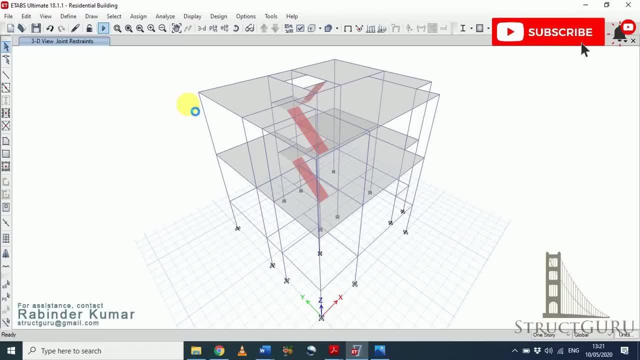 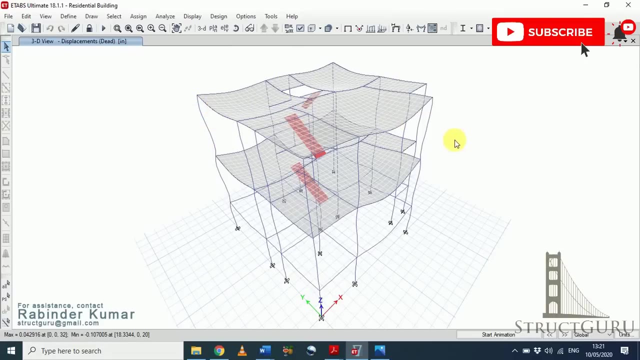 analyze such a structure. so this is the real power of software and that's why we use the structural design software: in order to reduce the time and get the accuracy in our our analysis. yes, our analysis is complete. so to check how our structure is displaced, let's go and click. show deformed shape by clicking. 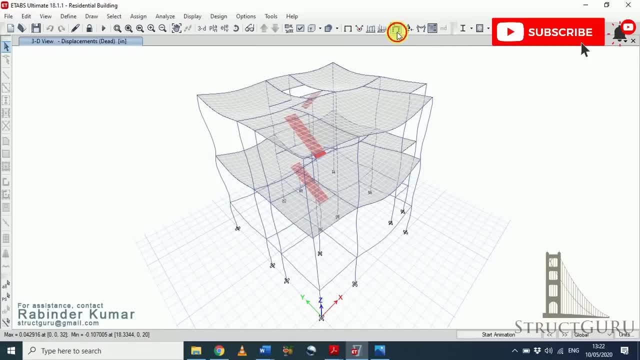 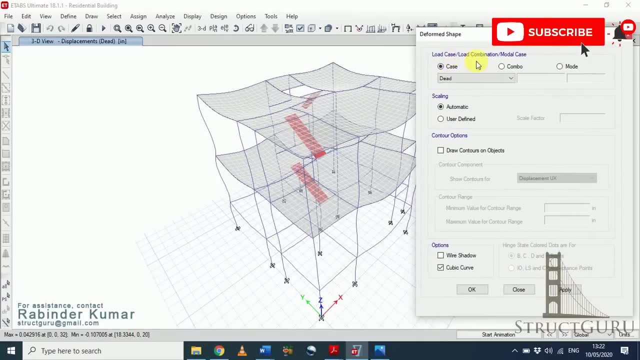 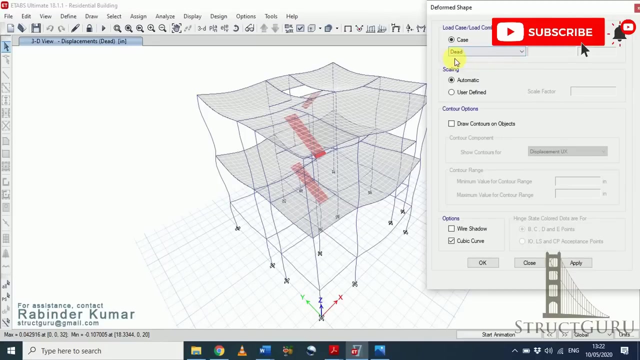 this icon or you can also press f6 from keyboard button. click on this icon. so from here we choose a load pattern or a special load combination which we have defined in order to see the displacement of a structure for a particular load pattern or combination. if you want to see, however, displacement is occurring on 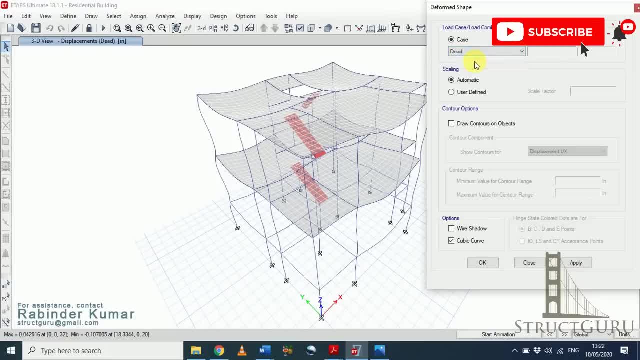 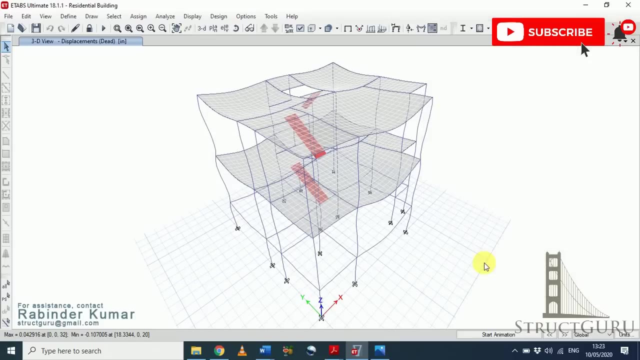 dead load case. so go and click dead load from here. you must click wire shed so we can see how much our structure is displaced from original position and click OK. so, as you can see, our structure is displaced downwards under the action of dead load, which is what should have happened. similar should be the case for 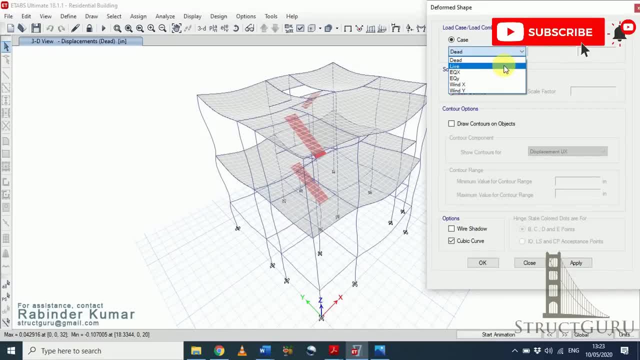 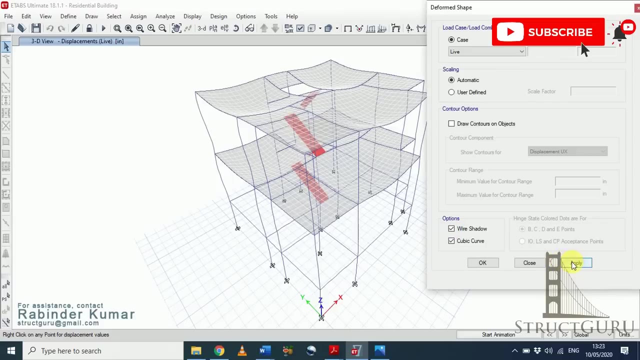 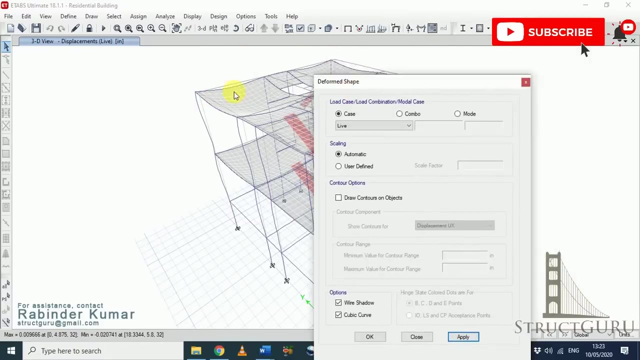 live load, but the deformation should be less because of a live load is much less than the dead load which we have applied. go and click apply and yes, so must click wire shadow. in this way, you will be able to know how much our structure is displaced from original position. if you want to check the displacement, you can. 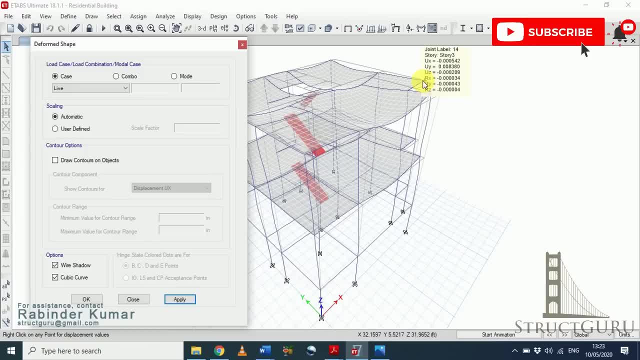 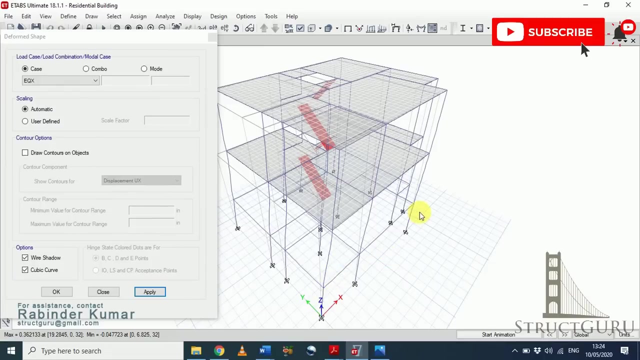 move your cursor along the joints, so in this way you will be able to know how much your structure is displaced. so for EQ X direction, our structure should deflect in positive X direction. so let's see whether it is happening or not. click EQ X and then hit apply button and yes, our structure is displacing on positive. 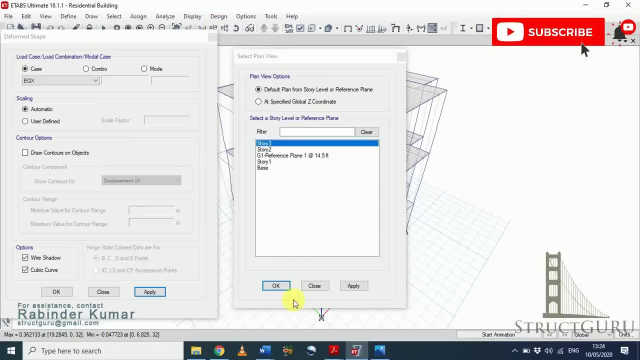 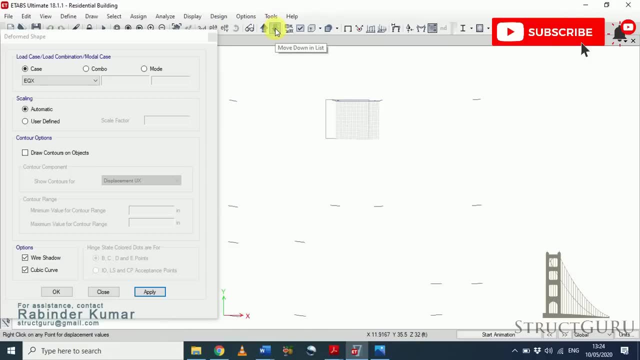 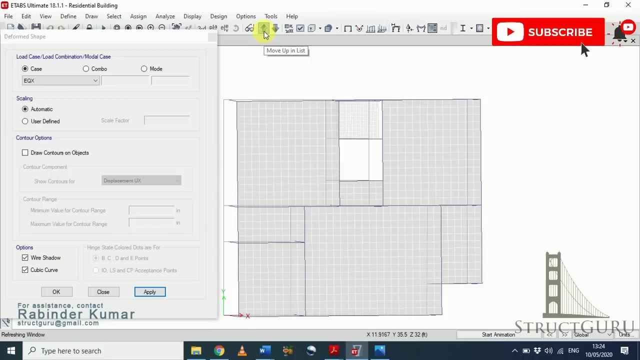 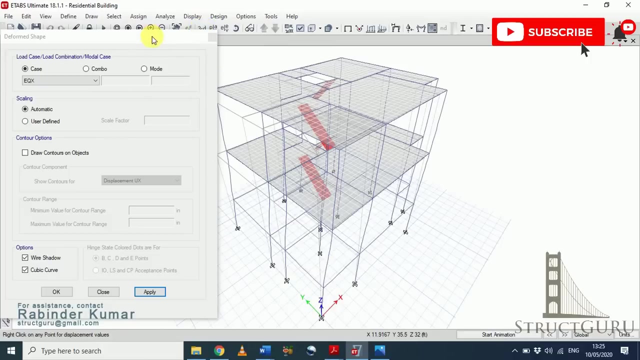 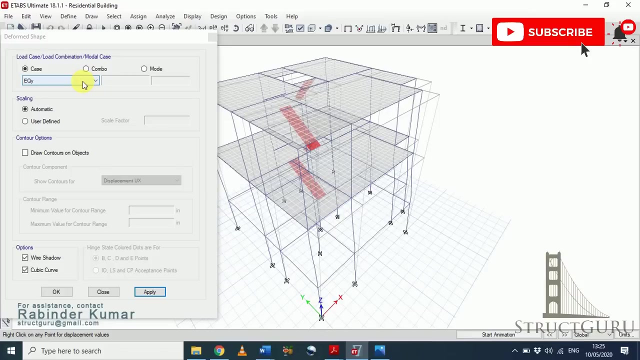 X direction. go to plan mode and yes, this is what should have happened. on bottom story, the displacement should be lower. in the top story, the displacement should be higher. similarly, for EQ Y direction, our structure should have displaced on rear side of the building. so select EQ Y and hit apply button and yes, the structure is. 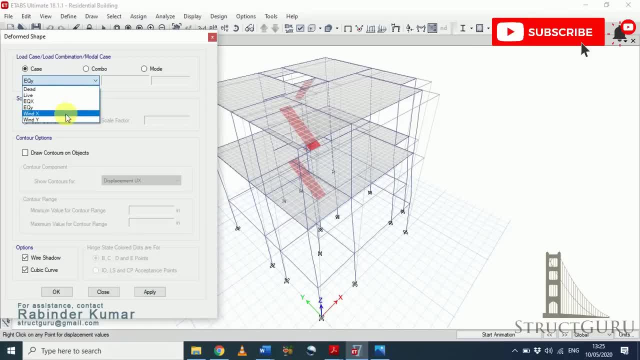 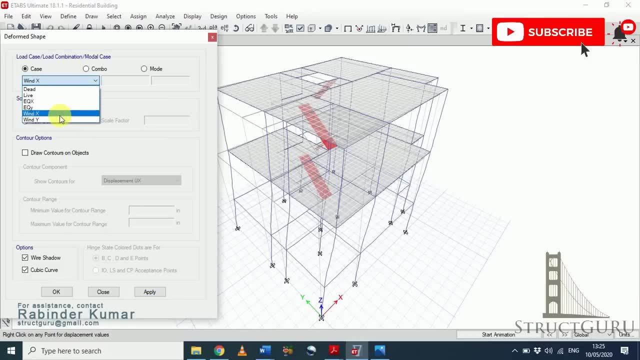 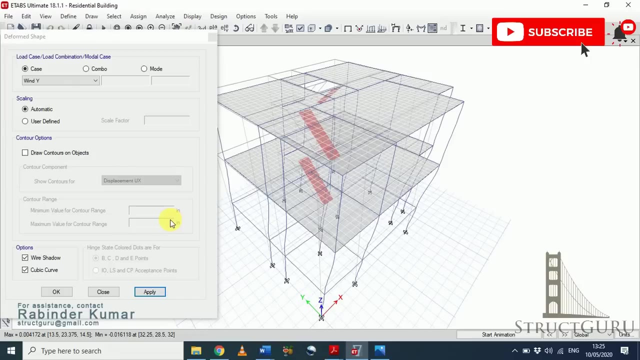 deflecting on the rear side of the building. similarly, for wind X it should displace on positive X direction and for Y it should have displaced on negative Y direction, because we have applied wind load from this direction. so that means whatever the load pattern we have applied, our structure is displaced. 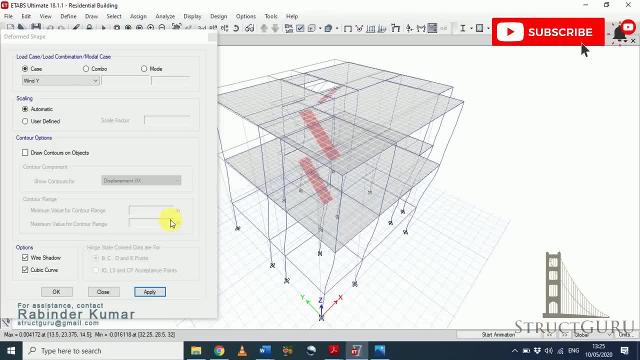 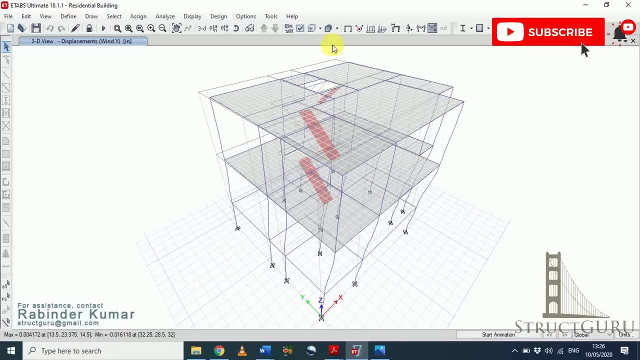 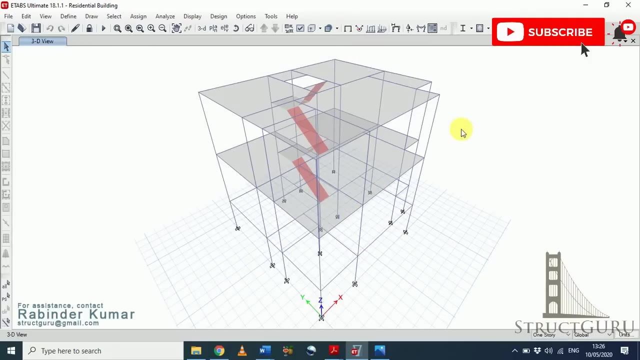 displacing accordingly. so this shows that our load applied on the structures are correct. if you want to switch it to the undeformed shape, go and click this option now. the most important point in our analysis is to see bending moment, shear force and axial force diagram. so 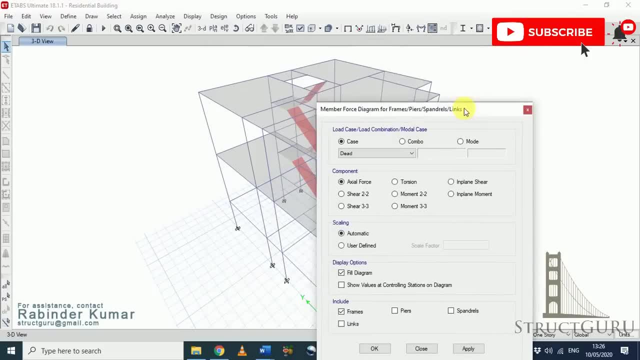 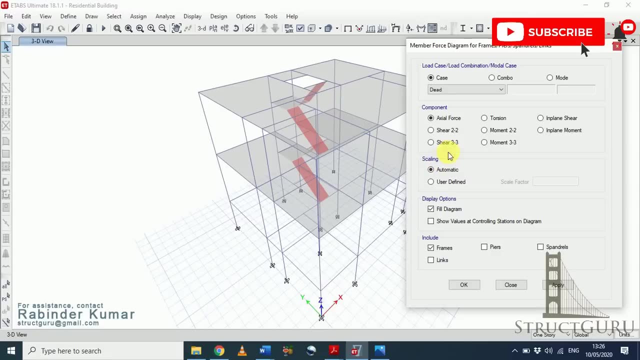 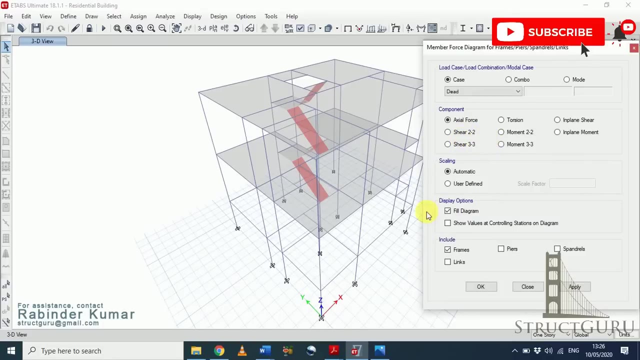 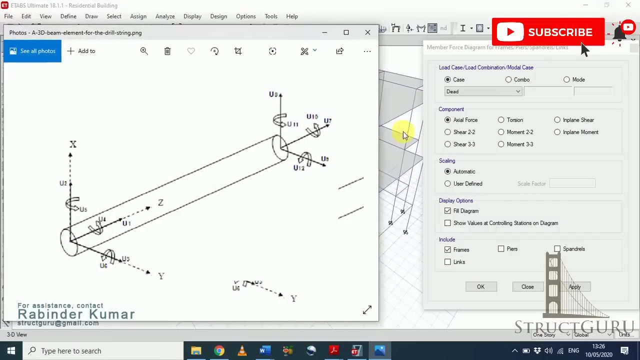 for this you have to click this icon. so once you click this icon you will come across with lot of force components and let me tell you which component to choose and which components are important in our design. so for this I will explain these component from the diagram. so in our design we give importance to V2. 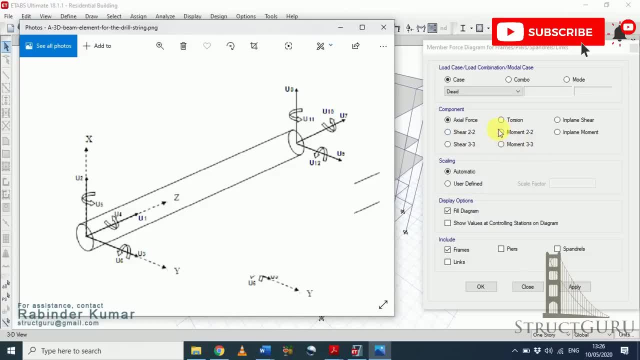 shear in V2 direction. similarly moment in M3 direction. we will importance to torsion in axial force. so let me show you from this diagram how the force behaves. for axial force that means the force along this plane or along this z-axis along the length of beam. so it should be. it could be in beams as well as in columns. 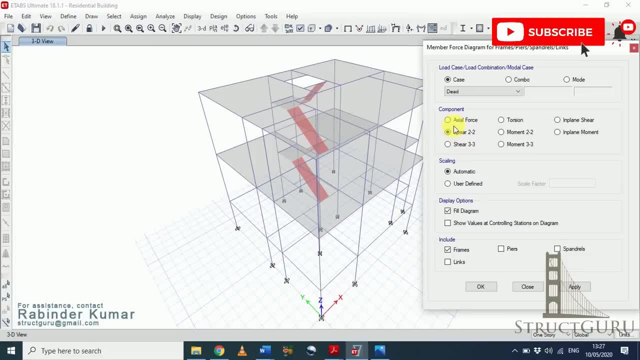 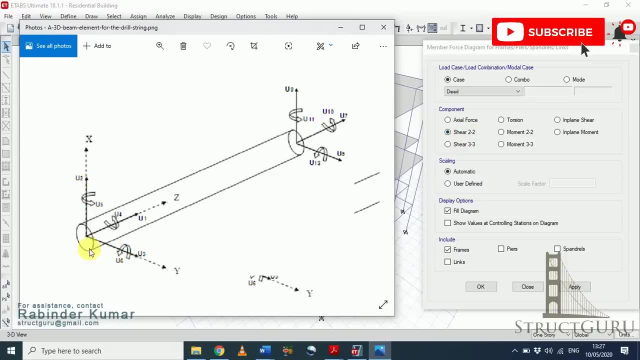 but it should be along the length of the beam. similarly, shear V2. shear V2 to means shear along two plane, this u2 direction. similarly, and this is considered the major shear force in our design. so we will take great importance to shear 2- 2. similarly shear 3, 3, that 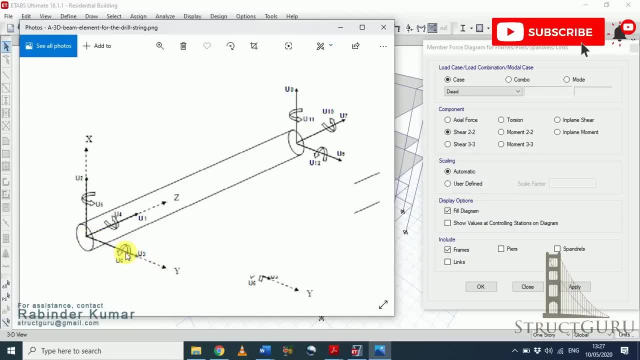 means shear in this direction and this is considered as minor shear. force input will give less importance in our design. and for moment 2: 2 now we have to use the x's. for m2 2 now the x's will be in u3 direction, so this is considered as minor moment. so this will deflect our beam in this. 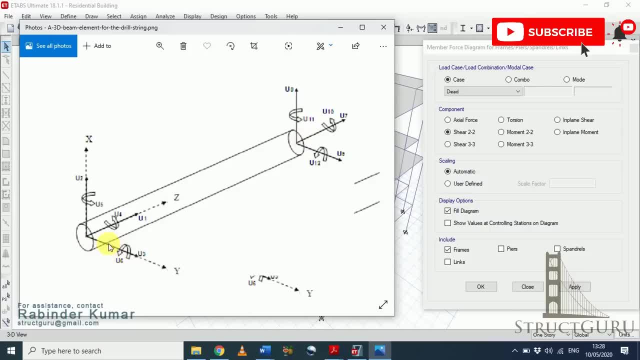 way in this way: for m3, this is the moment in u2 direction and this is going to deflect our beam in this direction. so this will is considered as major moment and we will give great importance to this moment. and for torsion, that is, the twisting effect, twisting effect along u7 or u4. so again, we will give importance to the torsion as 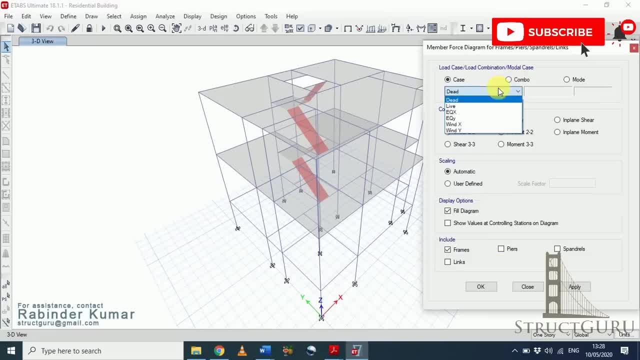 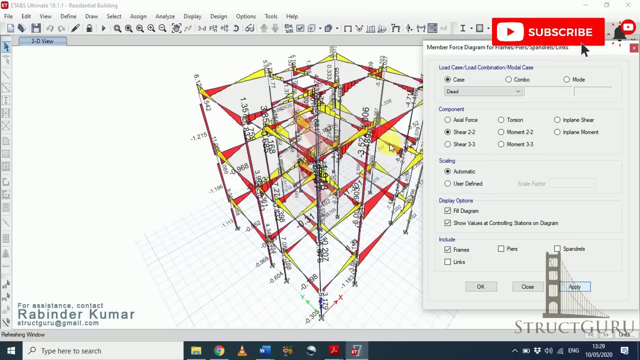 well. so for dead load, let's see click apply if and you must click show values at controlling station and this way it will give you the maximum values of bending moment along the beam. so click apply, so we click shear force. so our shear force is behaving linearly, as we know that shear force. 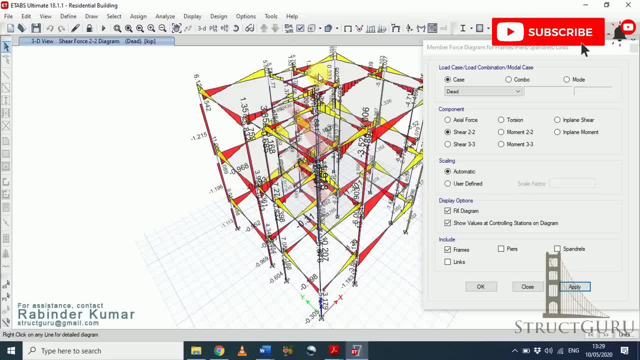 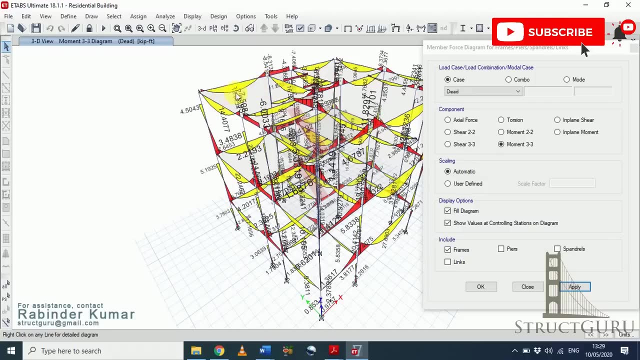 at the support is maximum, so that means our structure is behaving correctly. in order to see the moment diagram, click m33 and hit apply. once you hit apply, you will see the bending moment will be maximum at the mid and you will see hogging bending moment at the supports. 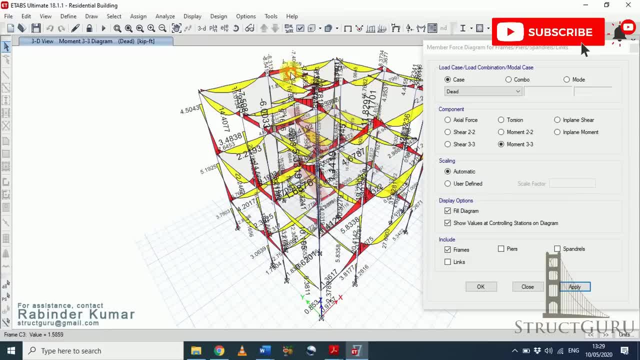 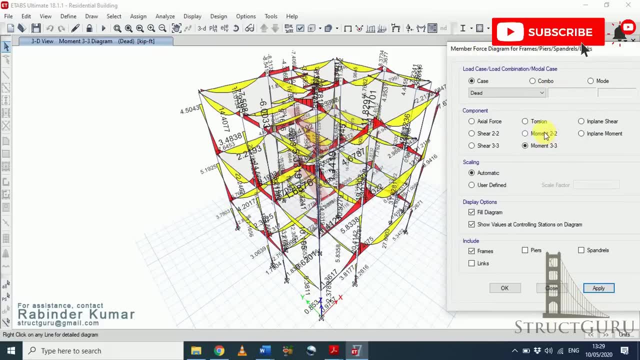 and that means you have to provide an extra reinforcement at the top of the beam. so in this way you have to go for the analysis in order to see in eq x direction. that means our moment diagram should behave linearly in x direction. so let's see whether it is happening or not. 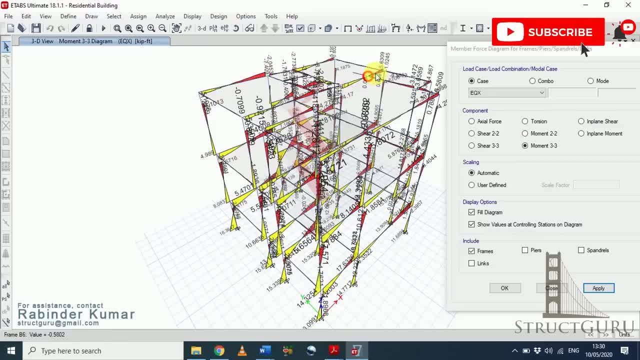 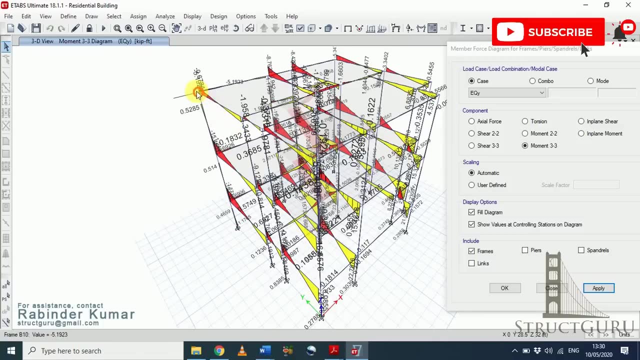 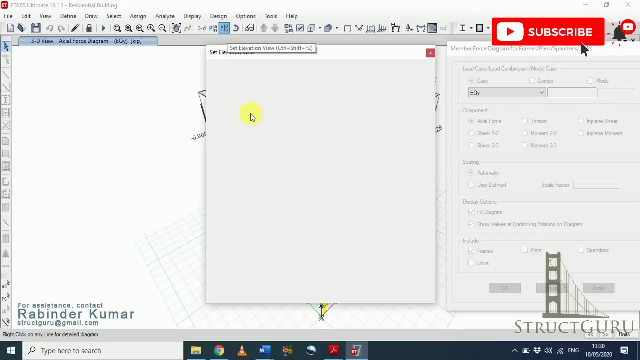 click apply and yes. so the bending moment is behaving, moving linearly along the beams. similarly, for y direction, click apply and yes. for axial force. so go and click axial force and then hit apply. so, as you can see, let me switch it to the elevation mode. so from here you can see. 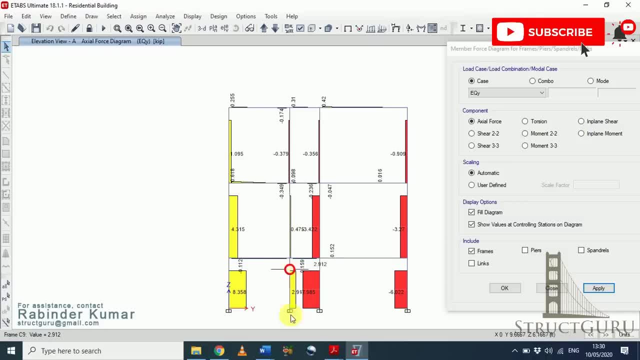 the tension force and the compression force. so these two columns are under tension. when the earthquake is applied in y direction and these two columns are in compression, and at the top story force is less and at the bottom is the way the force is high because of the 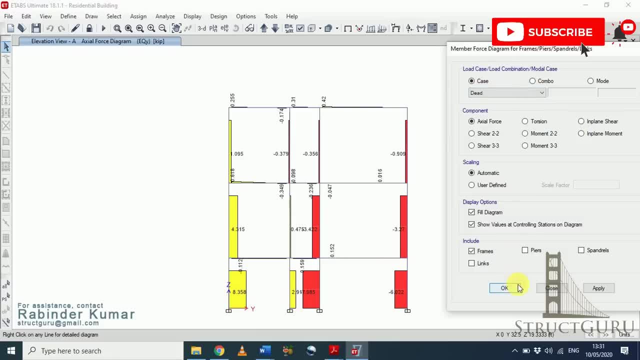 bottom is stories of first major load. similarly, if you click dead load you can also see from the dead load pattern our top story is experiencing less loads. the bottom story is experience experiencing high load because all over all the load coming from top story needs to be bear. 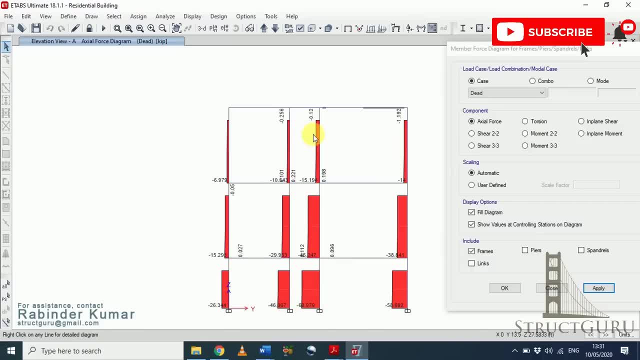 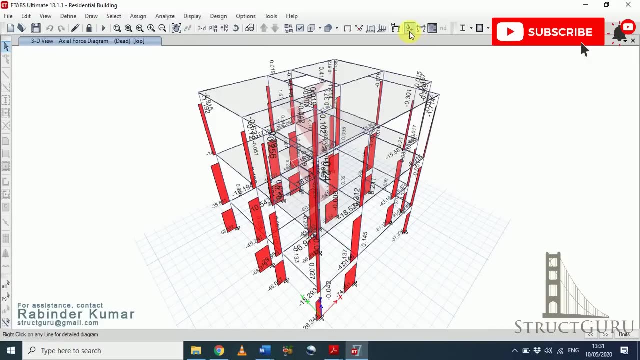 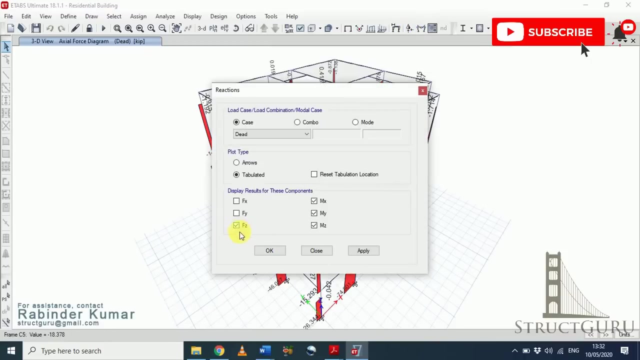 by our the bottom story column. so that means the model is behaving perfectly fine and click ok. now let me show you how to see the reactions. in order to know the reactions, you have to click this icon: display support spring reaction. we want to see the reactions. in order to know the reactions, you have to click this icon: display support spring reaction. we want. 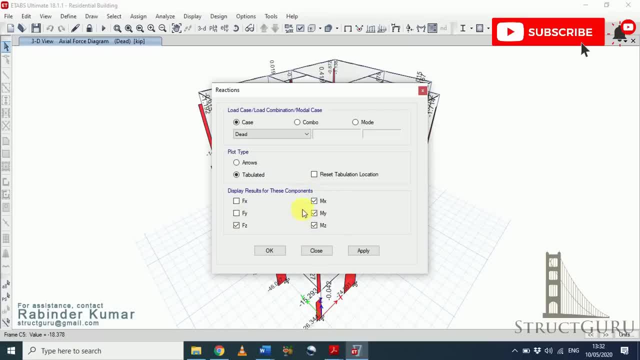 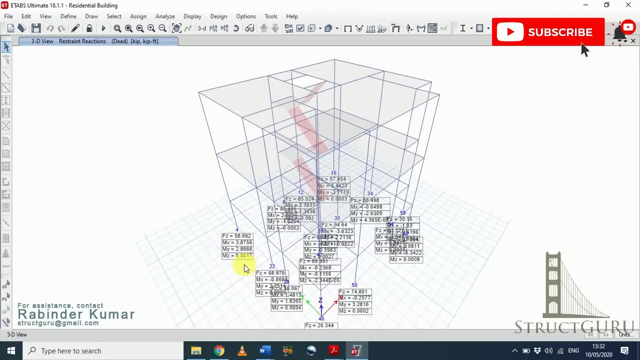 reaction in FZ direction and we will give all the importance to the turning facts moments and also click tabulated from this icon. so click apply. so once we go for the designing the foundation, we will be needing all these values. so this is, for example. so this column is: 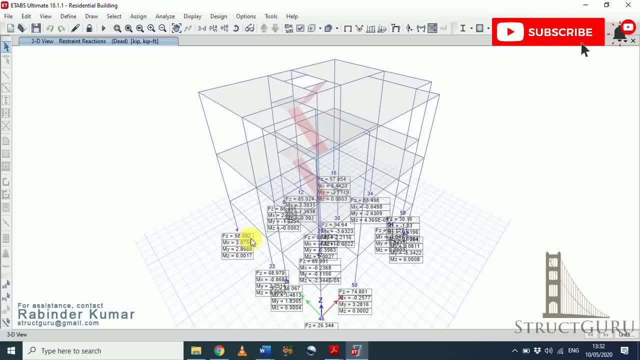 going to resist. fifty eight point six, nine two pounds keeps sorry. fifty eight point six, nine two kips of the load which is coming from all the stories. similarly, this column is experiencing sixty eight point nine, seven nine kips of the load coming from the first stories. so in this way we have to go and 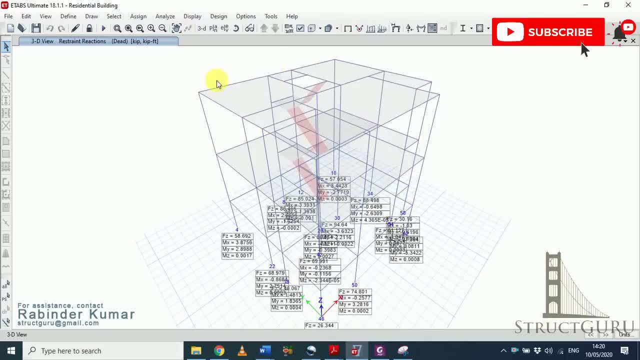 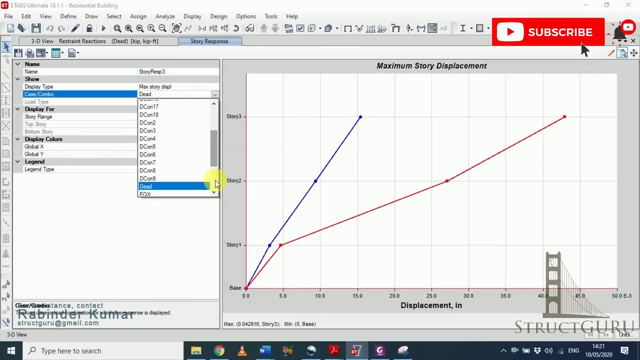 interpret the results. so, in order to see the story response blocks, so we will go to the display menu and from here we will choose the story response blocks. so this will show us how much our story is displaced under various load conditions. so mostly we will see our story displacement in EQ X. so from here, 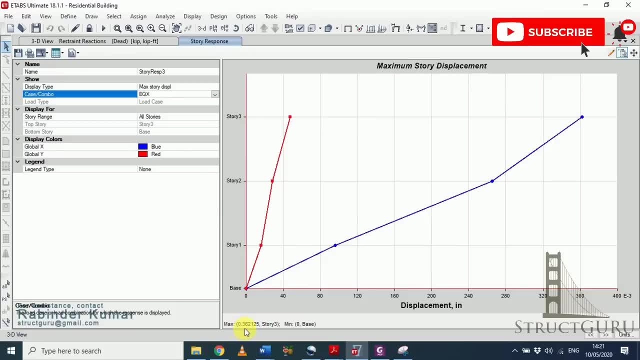 you can see the maximum story displacement is zero point six, three, six, two, one, five inches in X direction. similarly, for EQ Y it is three, zero point three, six, three, two, same in both the direction. so how to check whether it is within the limits which is suggested by codes? so in order, 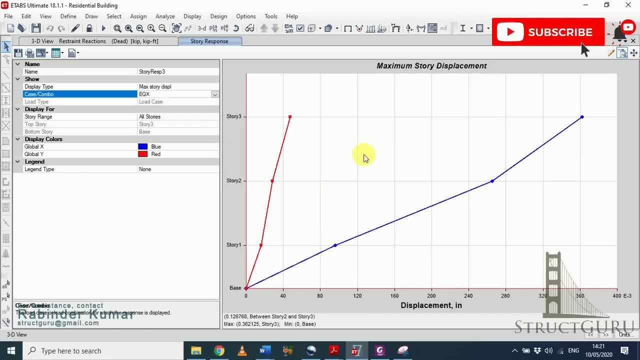 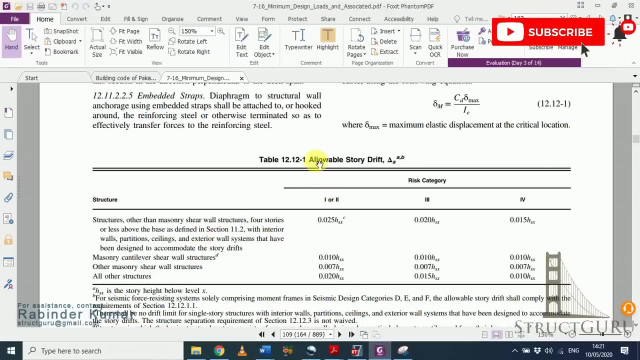 to check the limits. if you are using American code so you have to multiply. so here the allowable story trims are given based on the structure type, and this category you can show on the display too. so now I have visible elements which are given, but very getting busy just a later to find them, even though there are only few elements. y or seedlings, examples of today's method. so, for example, sorry that one that has integrated will bepress or broken. he is not just an example. but, for example, you will choose no for your towards non. follow the lineари. you can also choose theig as step under. 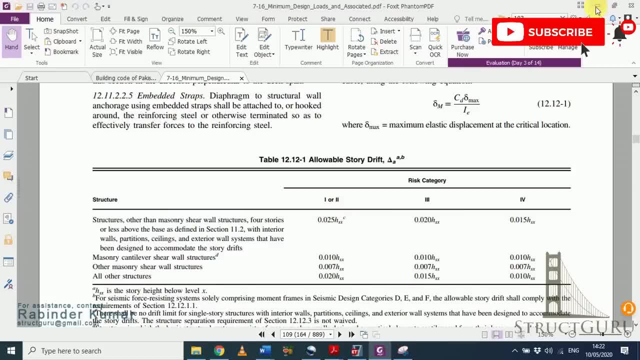 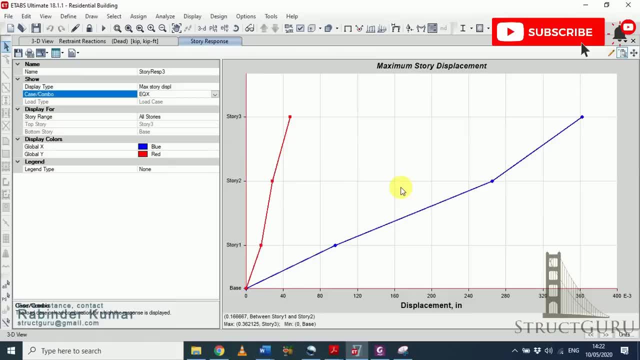 for example, i am taking this value 0.025, so 0.025 multiplied by story height, for example, i am considering 24 feet. i am not considering the base part of the structure. in order to convert 24 feet, i will multiply it by 12, so i am getting 7.2 inches is the maximum story displacement from. 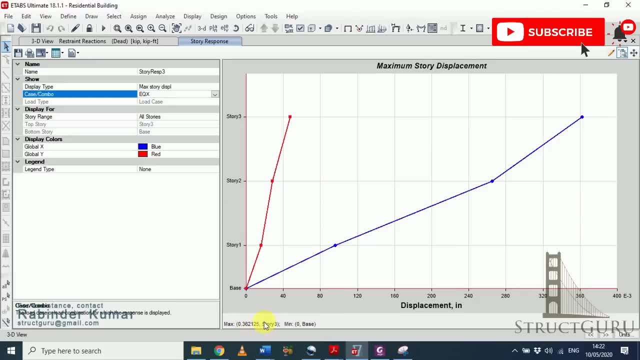 code and in this case we are only getting 0.36. that means we are within the allowable limits which are suggested by codes and if you are using is code, so in this is code this: we have to multiply story height with 0.004, so this will give you the maximum allowable story displacement. 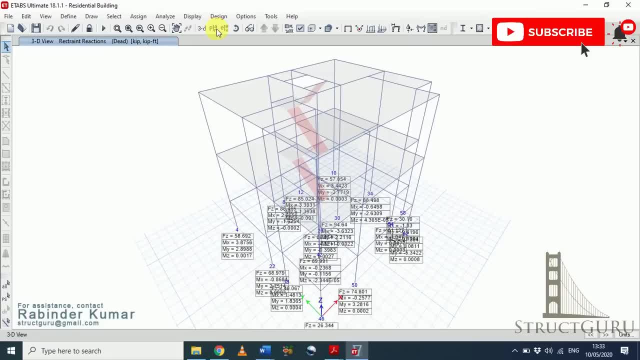 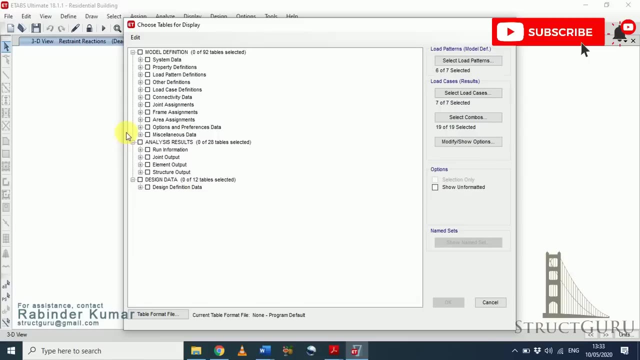 suggested from the codes. in order to see the other parameters, you have to go to the display menu and click show tables. from here you click analysis results and in this way you you can find many parameters as per your requirement. for example, in order to see the value of the base reaction, just click base reaction and from here you select the load pattern. 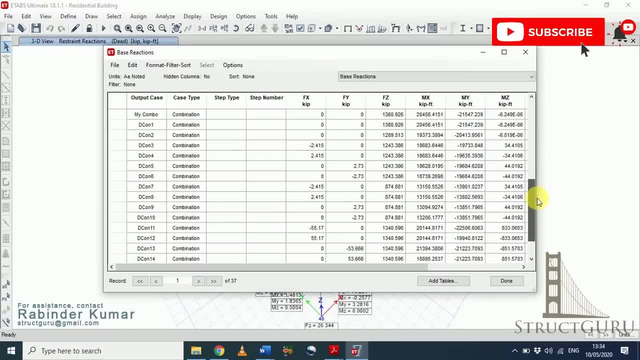 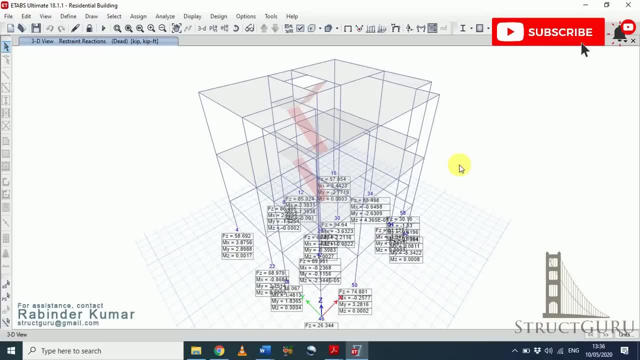 and click ok. so this will generate the base reaction according to the load conditions you have defined. so in my next video we will design this structure and i will show you how to verify whether our design is economical or not. if it is not, so how to make our structure economical. 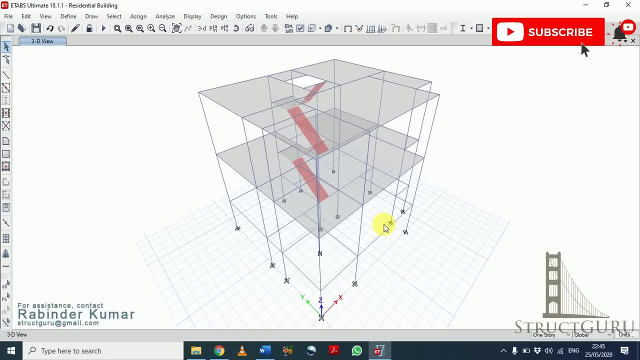 so, before designing our structure, let's see and check the material properties, whether we have added the correct values of compressive strength of concrete and all the related values of steel. so let's do it. go to define menu, go to material properties, and we have selected 3000 psi. 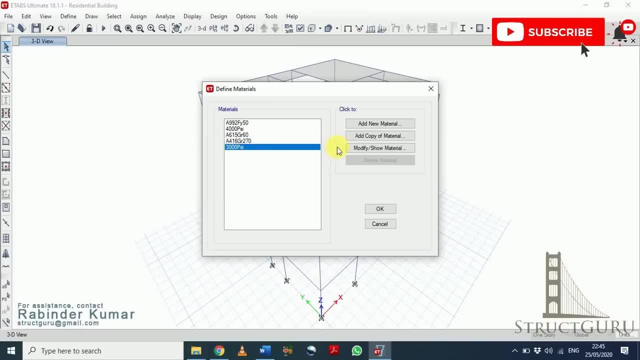 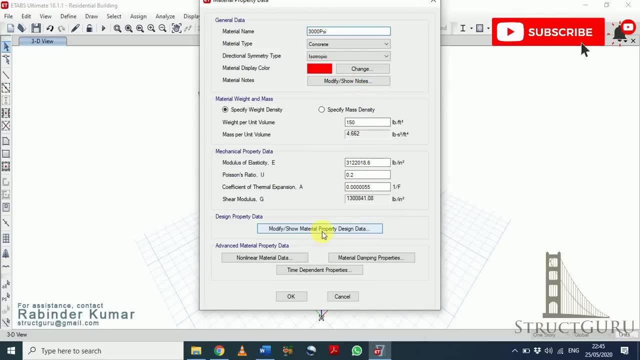 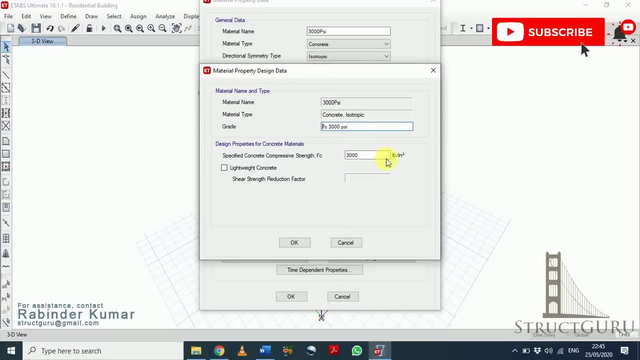 as compressive strength of our truck or the value of our truck concrete. so see. go to modify show material from here. click to modify show material properties. now, here you can see we have already added 3,000 pound per inch square as specify concrete strength, as our building is residential building. 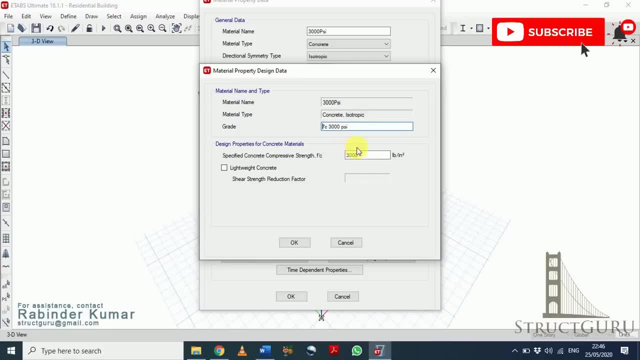 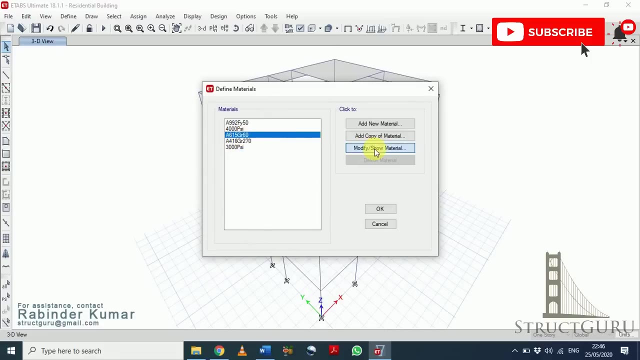 so it's not a heavy structure. that's why we will design all the components considering this much compressive strength of concrete members. click OK, let's check for steel. so for main bars we are going to select 60 grade of steel and let's see what are the properties mentioned. so click modify show. 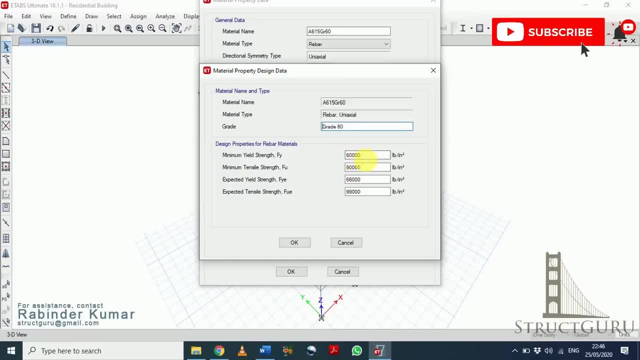 properties. now here you can see: 60,000 pounds per inch and the ultimate strength of the steel bar which we are going to use in our structure, which is 90,000 pound per inch square. you can also get these data from the supplier or the from testing laboratories. now this: 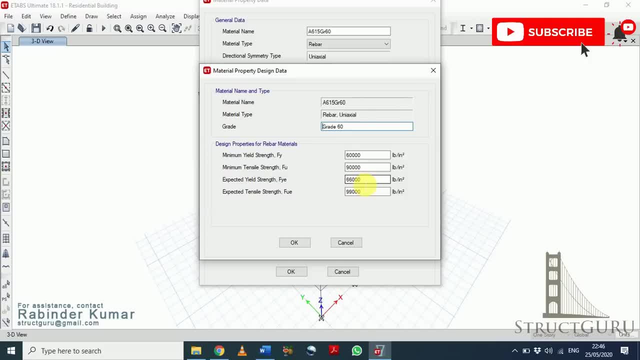 is expected yield strength. to find expected yield strength you have to multiply minimum yield strength 60,000 by 1.1 factor. so this is basically used for plastic analysis, for elastic analysis. we are not going to use these parameters, but you must know from where these values we can get. you just need to multiply these. 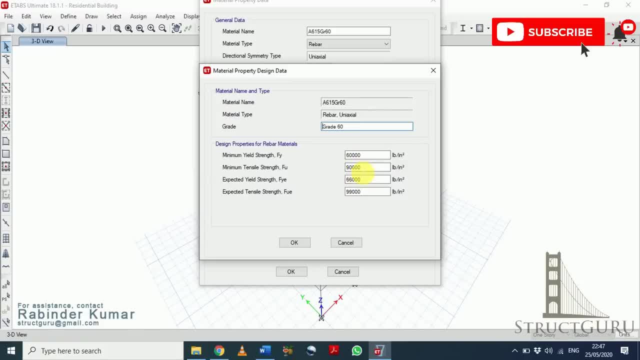 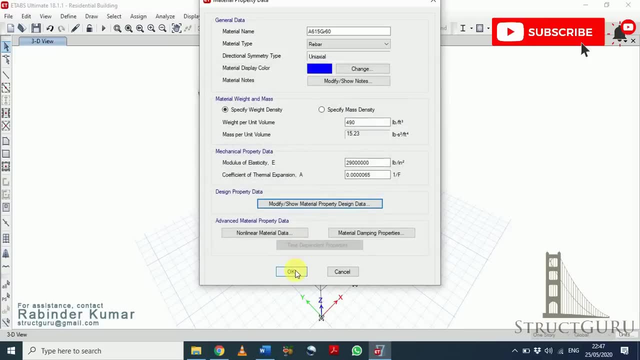 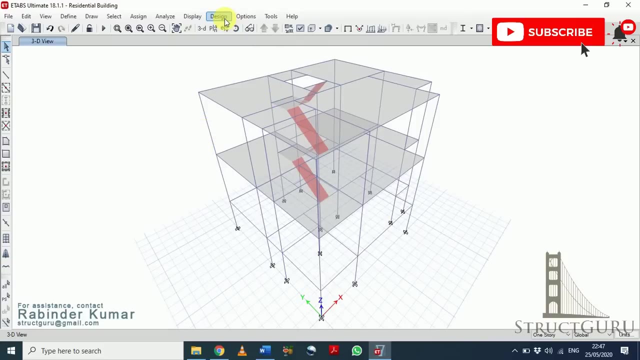 parameters by 1.1. so in this way you can get expected yield strength and expected tensile ultimate strength. so click OK and click OK. then click OK. in order to design our structure, you have to go to the design tip from the top and from here, as our building is concrete frame type. 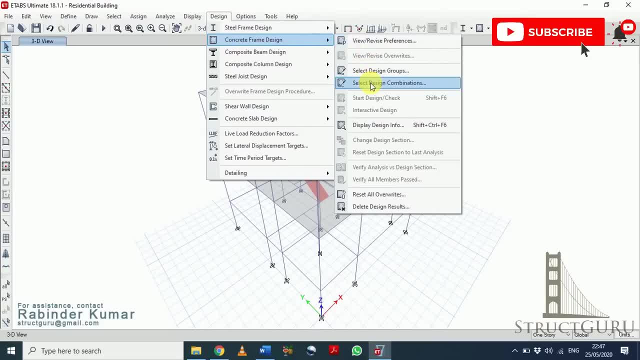 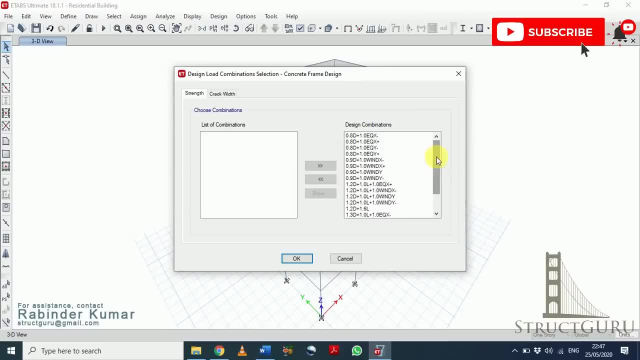 building. so click concrete frame design and then select design combinations. so here you have to add all the combinations which are suggested by code books. you have to put all this combination in this dialog box. so in total we have defined 18 different combination containing different load patterns with various magnitudes, which are mentioned here after. 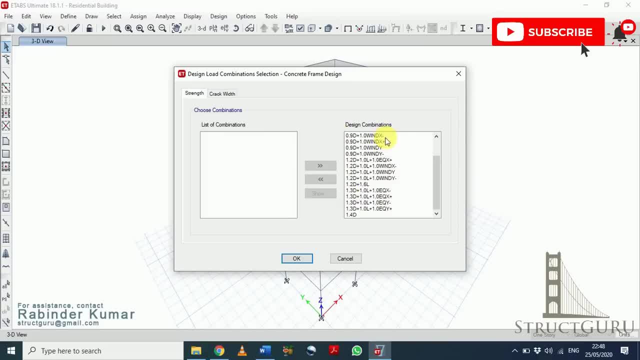 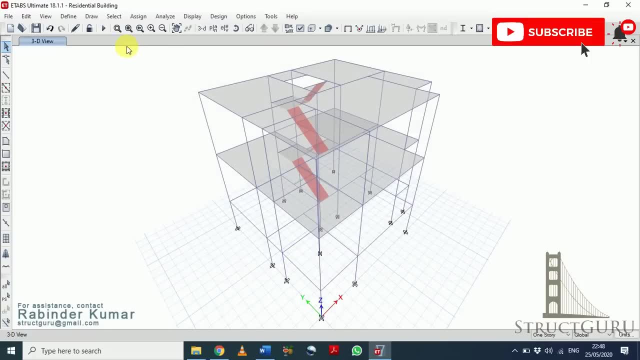 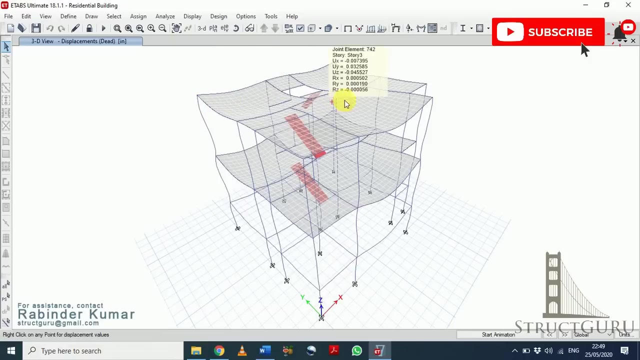 adding all the design combinations, and this right inside of the box. click OK. as you have checked all the design combination, now you have to run the model. so for running the model, click this play button. you, you, you, you, you, you, you. so our model is analyzed. to know more about analysis, you can refer to my 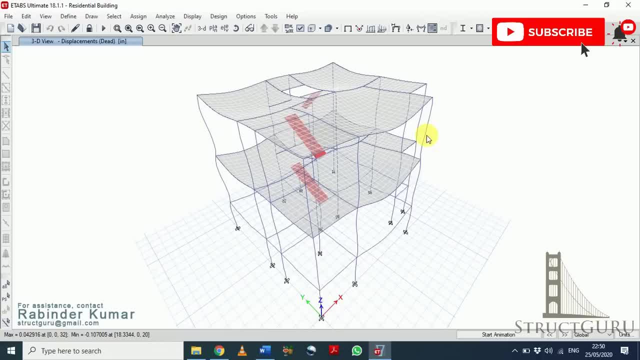 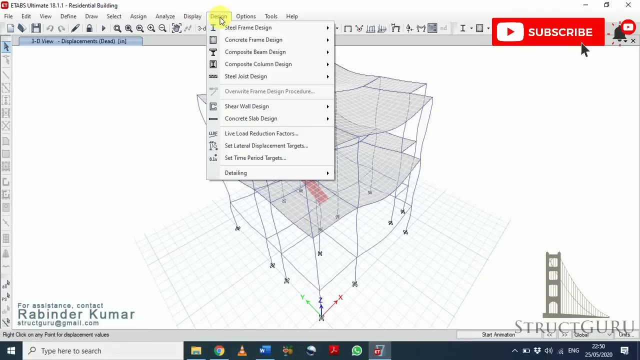 tutorial 8. here I have explained each and every parameter in detail about analysis for design. either you click this icon which says concrete frame design, or you go to the design tab from the top menu. from here you select concrete frame design and then click on the design tab from the top menu. from here you select concrete frame design and then 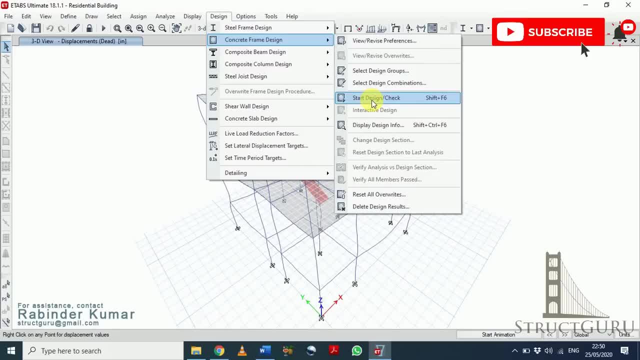 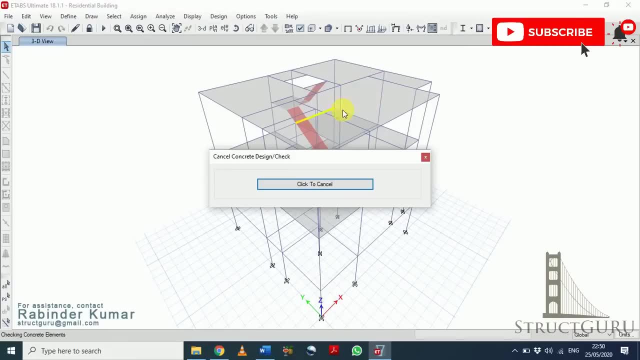 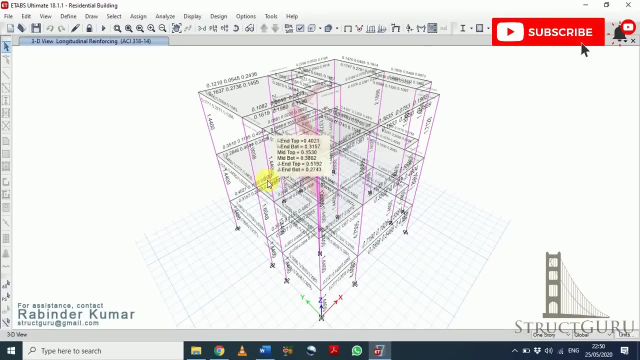 then select a start design flash check. so here you can see the model is going beam to babe and column to column to design each individual member in this structure. so, as you can see, our design is be in the order of Mitsuba. so here you can see. this is a really a pretty chill look like a machine from the same setting. so this is birthing system, which is built by Microsoft and here you can see this is being designed for each. when we are displaying 2011 standard dean, say, we are maximum time starts, there are some options to use. that this is for each individual and so, as the module has been designed for each individual person, there are six którzy that AI's designed within seconds, the core structure of our demonstration and everything you can see. 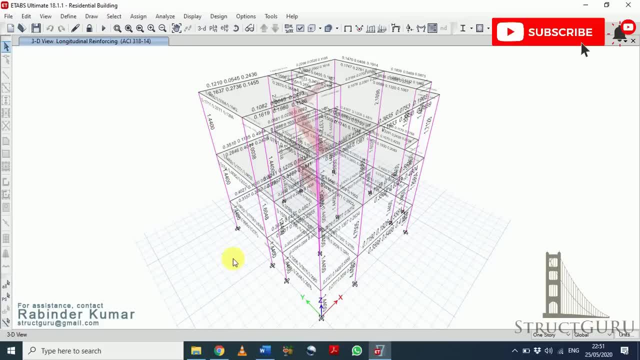 has designed all the structural components. now let's see, let's check whether is there any member which is failing the load which we have applied. to check that, what you have to do, you have to click this icon- concrete frame design. from here, verify all member passed. you have to select this option after that. 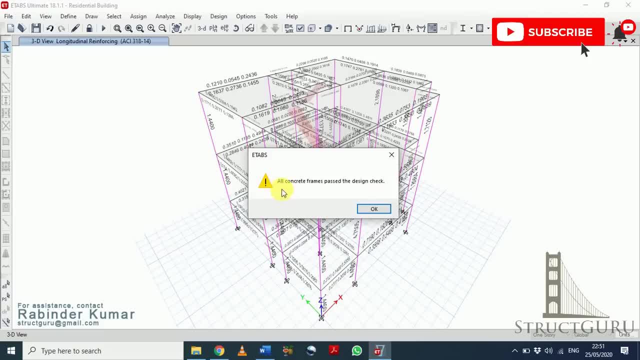 dialog box will appear where you can read all concrete frame path design check. that means whatever the loads we have applied and earthquake conditions which we have modeled in our parameters so against all types of loading and loading patterns, our structure is responsive, will considering the section sizes and the material type which we have. 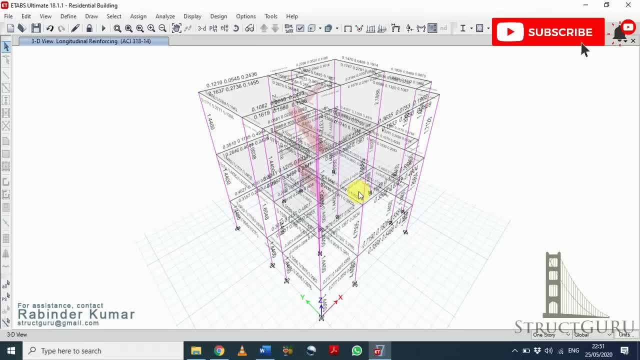 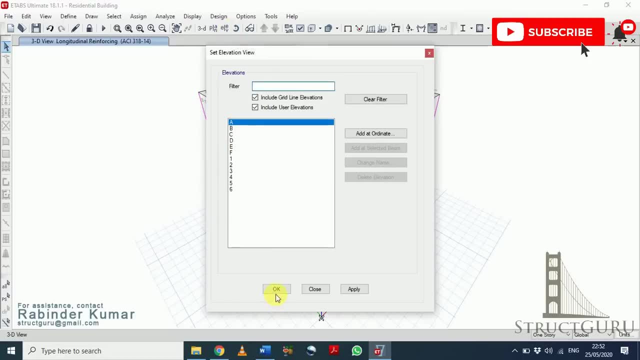 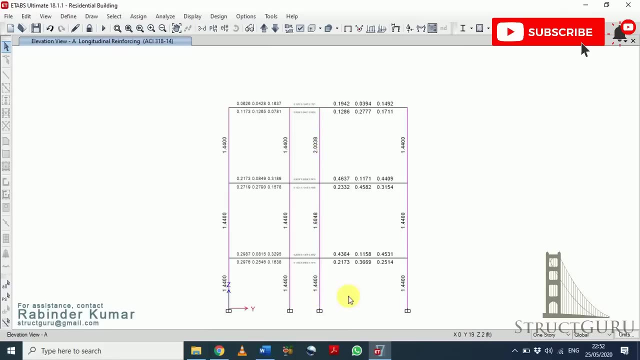 defined to design this model. now let's see the design in detail for this. go to the elevation view and select any kind of elevation. if you remember from my analysis video in axial force diagram, the bottom story columns were experiencing more loads than the top story columns, but here you can see the middle story. 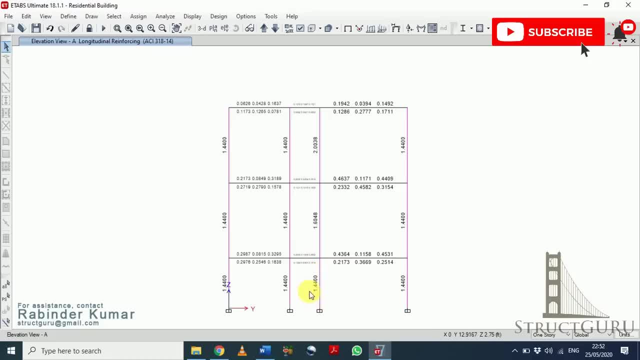 column requires more steel than the bottom story column. and again, the top story column requires more steel. so what is the reason behind that? to understand these numbers, let me switch this data into the percentage, so it will be very easy for us to interpret. so for this, you have to click. 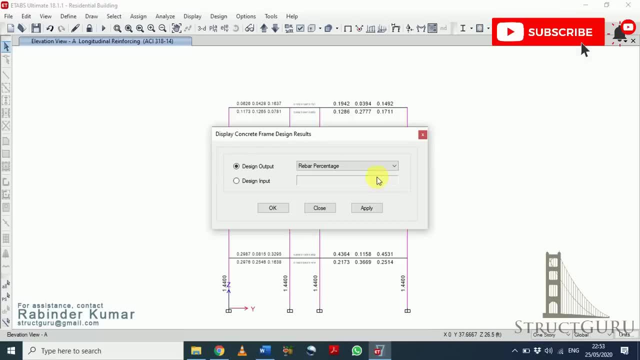 this icon and then go to display design info. from here you have to select 3 bar percentage and then click OK according to ACI code. so the minimum greenGH- I've added the Boole value每 reinforcement and column is required one person and the maximum is eight percent. so for example, 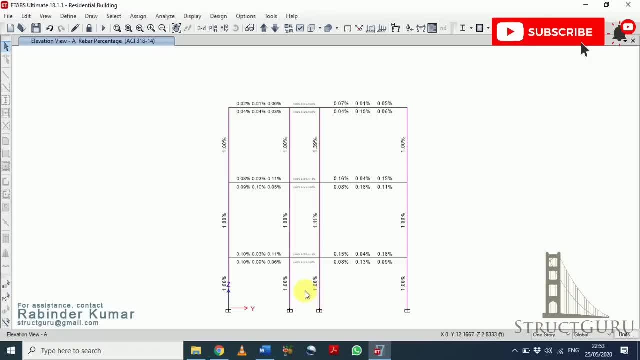 here you can see, the minimum reinforcement by default is one person. if, for example, design calculation suggests the minimum reinforcement should be 0.8 percent, but etabs by default considers the value which is suggested from the sei code, which is one person. now, at the above story again, the percentage of steel increases and at the top story the percentage. 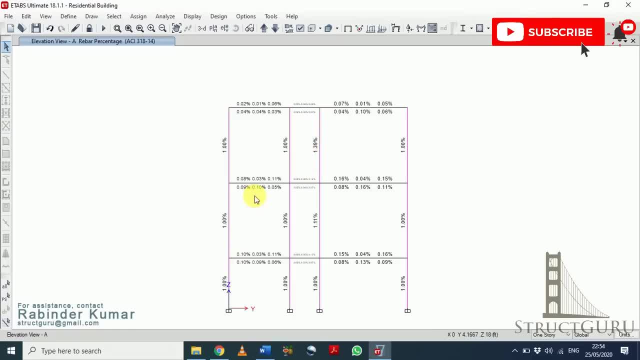 of steel increases. similarly, if you consider these types of column, the percentage of steel is uniform throughout the stories. let's see the other elevations now again, the percentage of steel at first story and second story is higher compared to the bottom story. now, what's the reason behind that? because, based on the axial force diagram, 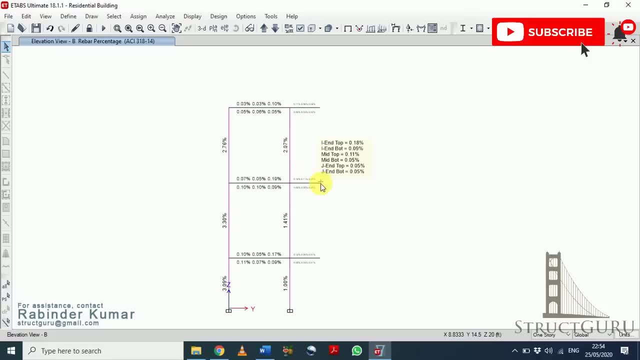 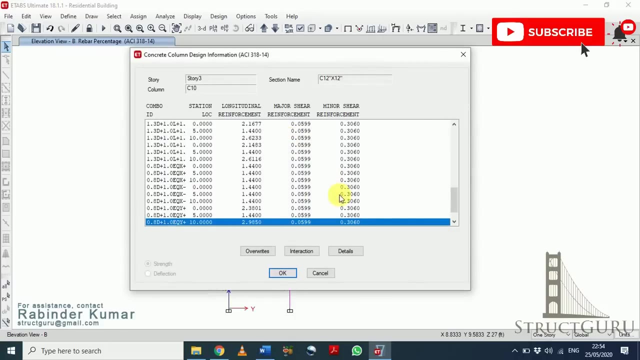 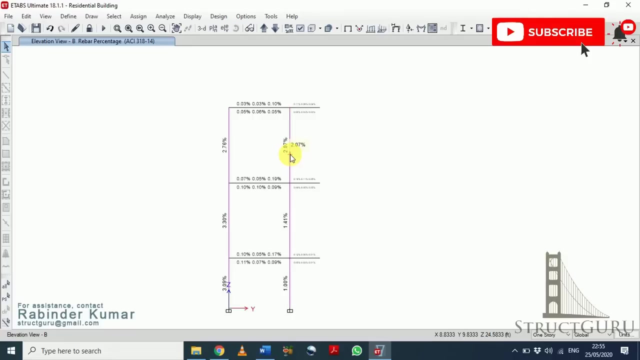 top story is experiencing less loading and the bottom story is experiencing more loading, then why the steel percentage is required higher in the top story. so let me tell you: the percentage of steel in columns is decided on the based on on the movements, by axial movements, movement. now, if you want to see the details, why, at what load combination, this percentage of steel is. 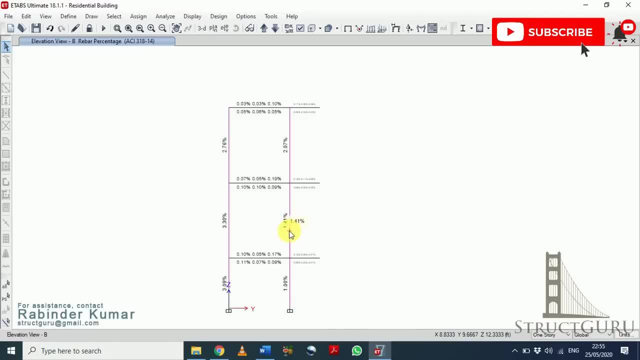 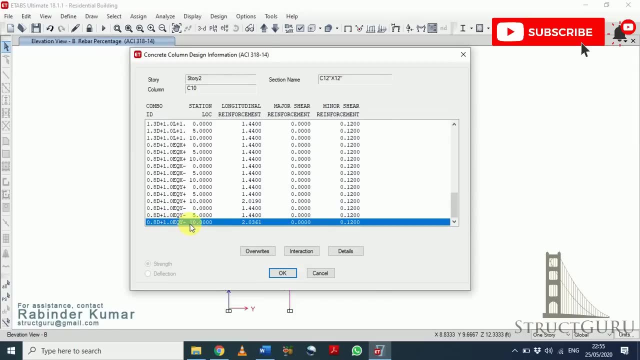 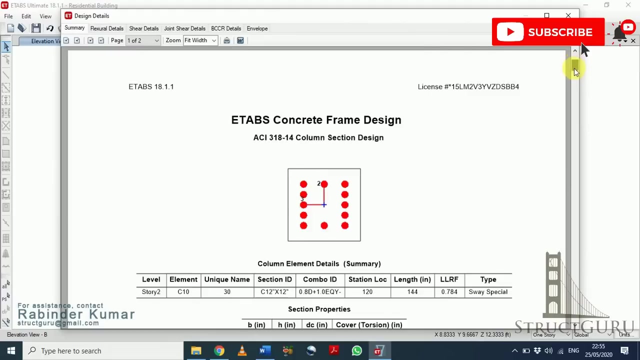 calculated. so just put your cursor at this column and press the right click from your keyboard or mouse. so here you can see, on this loading combination you are getting higher longitudinal reinforcement. so if you want to see more details about this column, click the detail button. so here you will see the entire frame design for this column, particularly at this story. so for 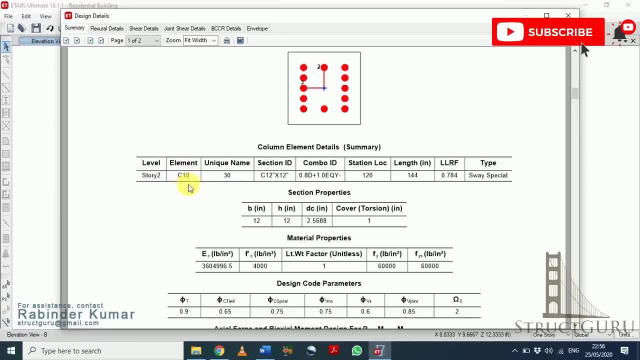 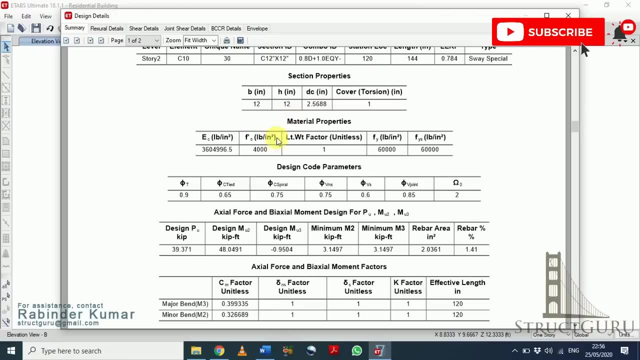 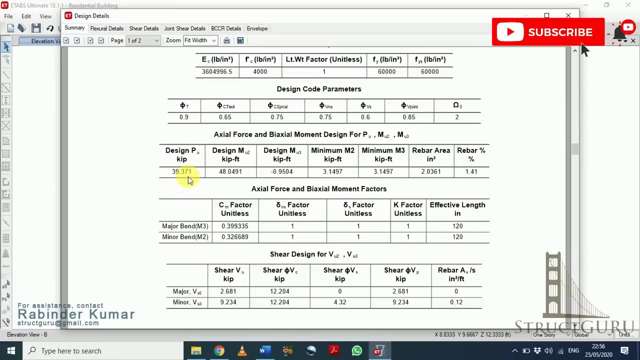 story 2. the column id is c10 and the section size of the section is c12 by 12 at this load combinations. so this is the design based on this loading combination. now from here you can see that the top story is coming on. this column is 39.371 kip. 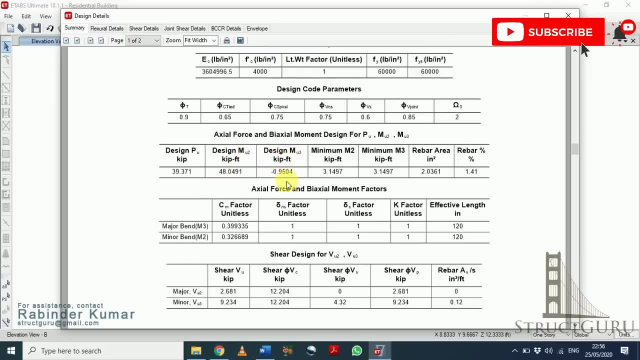 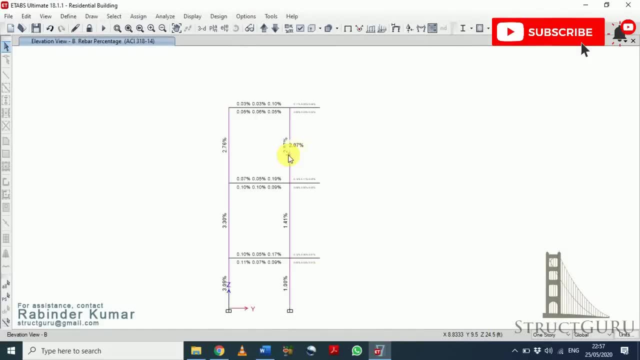 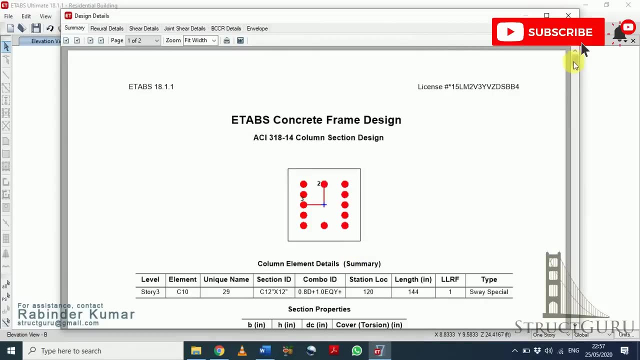 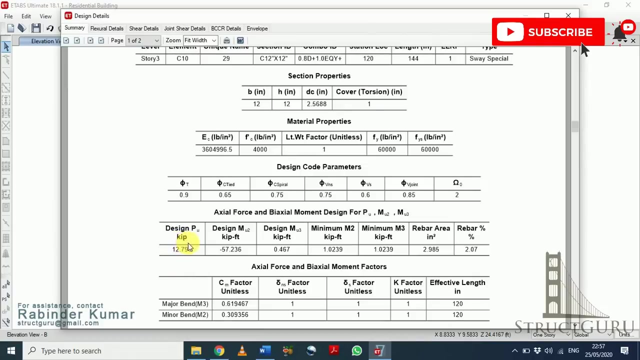 moment in two direction is 48.09 and moment in three direction is 0.950 kip. now let's look for the design parameter of this column. so for this you have to go for the details. now you will see this top story is experiencing less load. 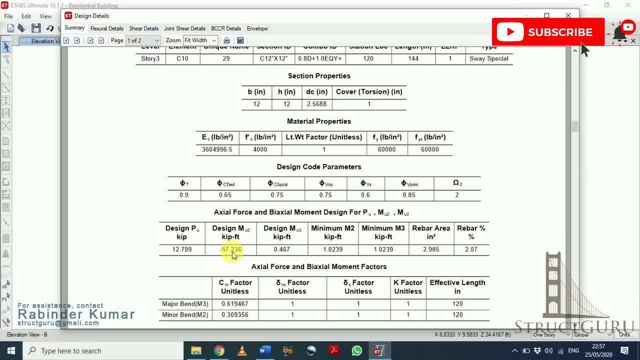 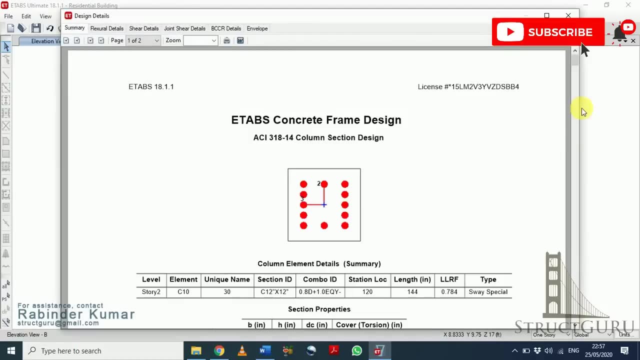 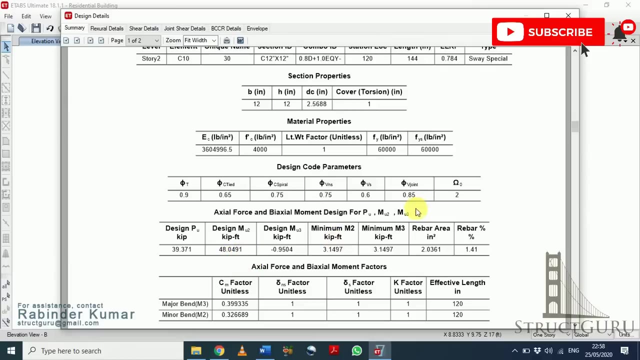 the moments are higher, so the moment will be the deciding parameter for calculation in area of steel. so here you can see, minus 57.236 kip fit and here you can see the moment is 48.049 kip. so in this way, and this column is also experiencing more load than the 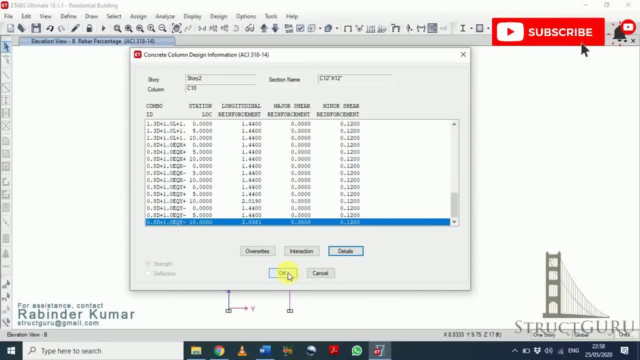 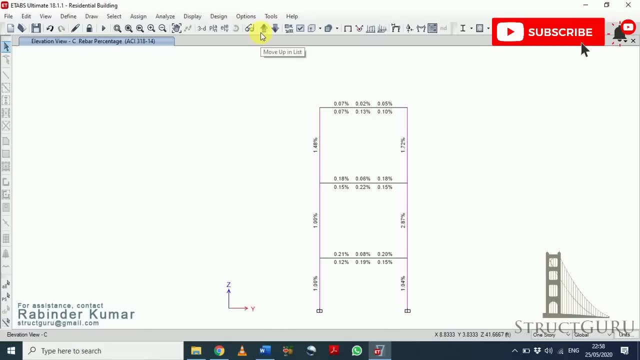 upper story column. so the moment will be the deciding parameter for area of steel. so if you face this kind of behavior in your model or in your design, so don't worry, just take for the moment calculations. now let me explain you the data for the beams. so this data denotes the reinforcement at middle. 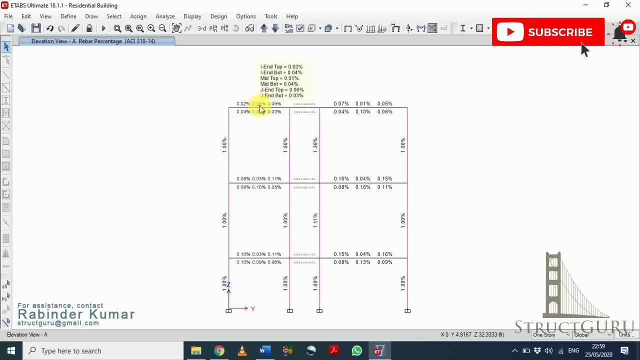 of the section at the bottom and this data denotes reinforcement at middle of the section at the top. this is at the left side of the beam. this is at the right side of the beam, so the bottom- the numbers written at bottom of this beam- represents main steel or 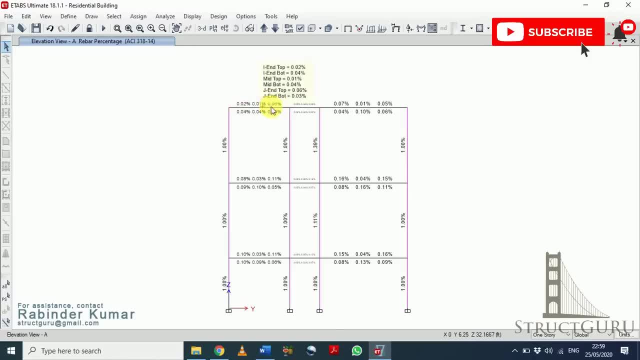 bottom steel and the number represents at top of the beam represents the top steel required in this, required for this beam. similarly, you can see at the sides, the top reinforcement is small compared to the bottom reinforcements. so why is this? so you must remember from an analysis video we were experiencing.